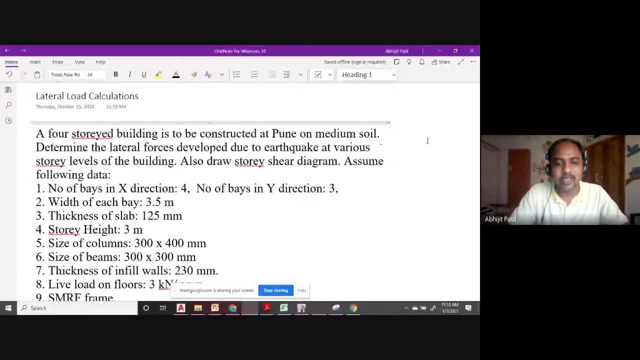 effect is generation of waves inside the ground. so that is the major cause of concern for civil engineers. so that is causing damage to our buildings. so after understanding this, we also have seen that different parts of country it is divided into different zones. those are called as seismic zones. 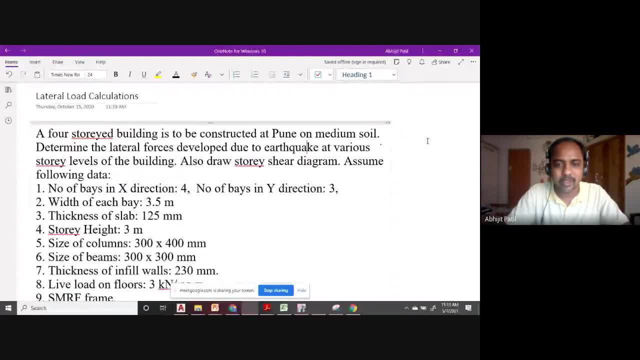 okay, so, as I told you that, I will elaborate that more when we solve the problem, so, uh, that zoning is necessary because some part- we have seen some part of Maharashtra will face lesser earthquakes, because these zones, if you see, it depends on the geological features. okay, so the Himalayan region is. 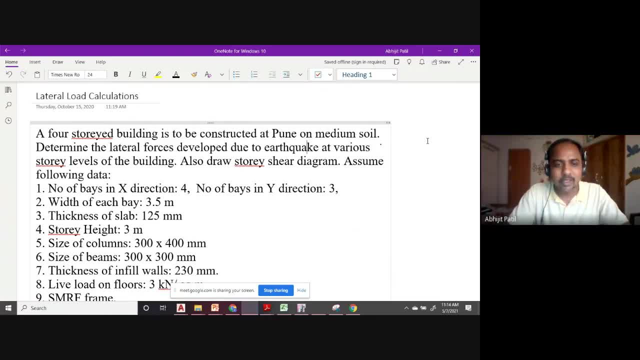 prone to more earthquake as compared to the Deccan region, Deccan Plateau. we know that most of the Maharashtra is on Deccan Plateau, so this is seismically less active as compared to the Himalayan region and some part of Gujarat. Kutch is seismically active because there is a fault present. 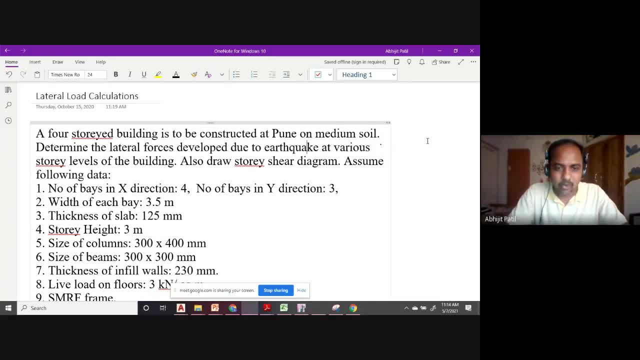 there. so earthquakes do happen at that region. so we have seen that and we have also seen how the earthquakes are measured. so seismograph or seismometer, these instruments are used and basically, uh, the magnitude, uh is measured with the hip-hop Richter scale, so it is nothing but the amplitude, so that wave is recorded in. 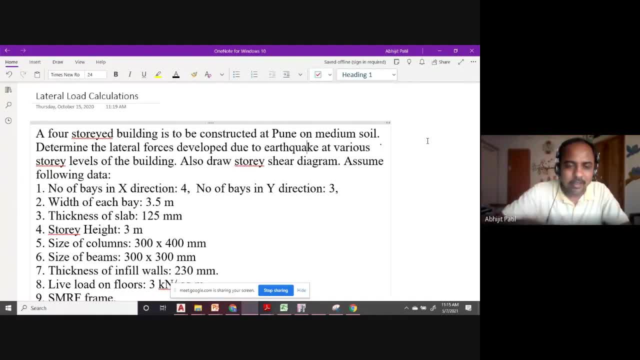 seismograph maximum, uh, you can say displacement of the ground or acceleration of the ground is recorded and that either acceleration, displacement, velocity that can be converted to displacement back, and that displacement is used to calculate the seismic magnitude and that is called as this is magnitude okay, and another. 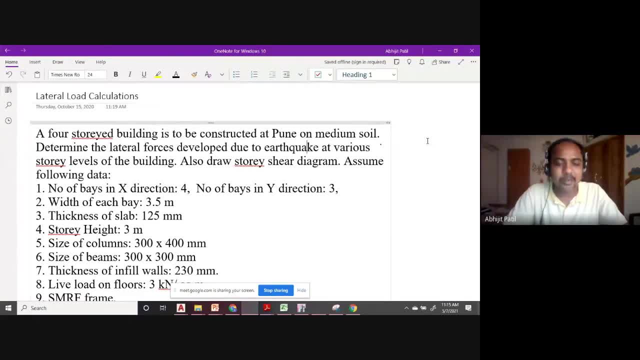 which I forgot to mention yesterday. another parameter is used that is called as intensity. so intensity is nothing, but you measure the destruction. so you can refer to any standard textbook. there are two good books I will suggest at the UG level. so these are: and design of uh buildings by sk dude, and another is punk Jagarwal and Manish recondite. 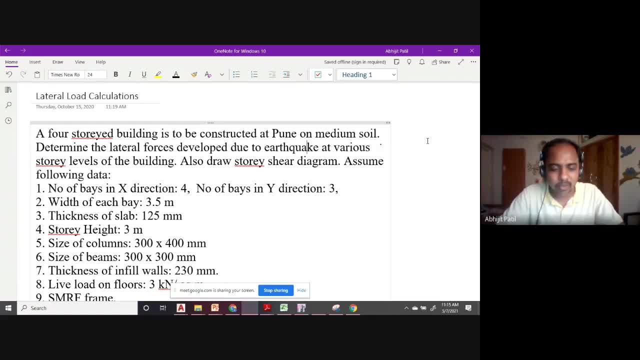 so these two books you can refer even for if you opt for PG, these books are good enough to help you in your PG courses also. so so there you will find the intensity different, different New lawsuit, chilérian- we're not going in detail, but the amount of destruction. 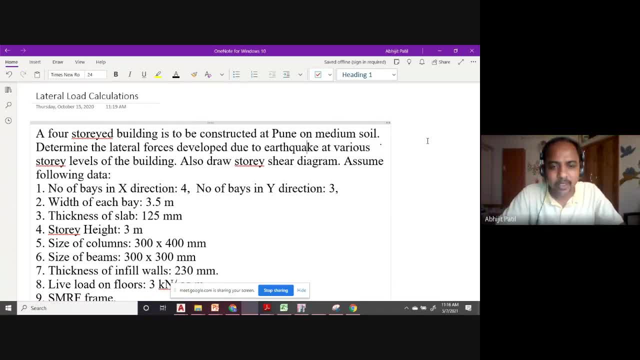 is measured, or whether the humans fail the vibrations or not, whether only upper story people felt the vibrations but the first two, three story didn't fail. so depending upon this, the categories are chosen for intensity and the intensity map. just like contour map, we have intensity map. so generally, at nearby source, the intensity will be more obviously and 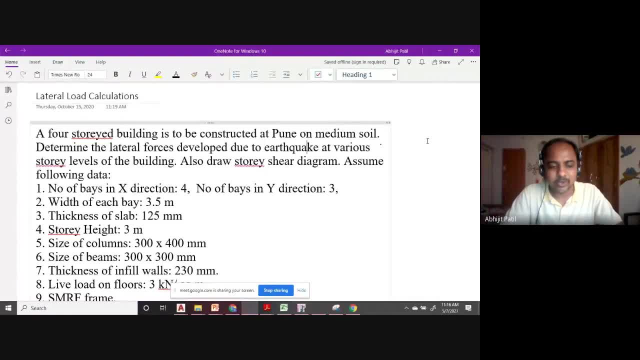 as you go away from the source, the intensity will reduce. so these maps are called as iso see small maps. so these are different methods to so. basically, magnitude is actually the amount, where it measures the amount of energy released or related to amount of energy release, but the 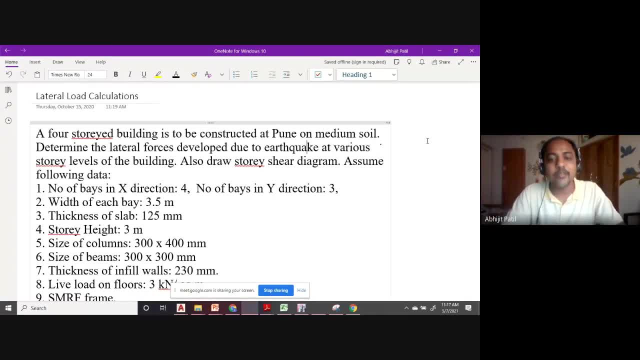 intensity is. it is the effect of earthquake on human beings and buildings. okay, so this is the basic difference. so, technically speaking, magnitude is- more, you can say, appropriate parameter to measure an earthquake. but from cylinder in point of view, intensity is also that much important because it includes the building damages. okay, so our in our hand. 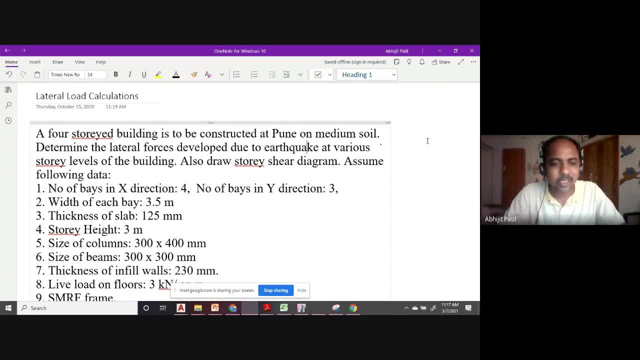 magnitude is not in our hand, because that is seismological activity happening inside the earth which is not in human beings hand, but the intensity we can reduce by applying some- see- earthquake resistant designs and experience principles. okay, so for that. so that is again some advanced part, but before that we must know how to Thank you. 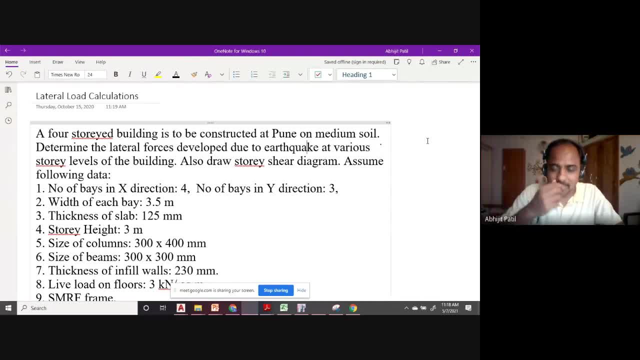 for taking this session. if you have any further questions, please e-mail to podtronplaycom. are actually now into the effects of earthquake on our buildings, and that too, infact, quantitative 평신계속 reminder- okay, because we will actually calculate how much force is going to act. 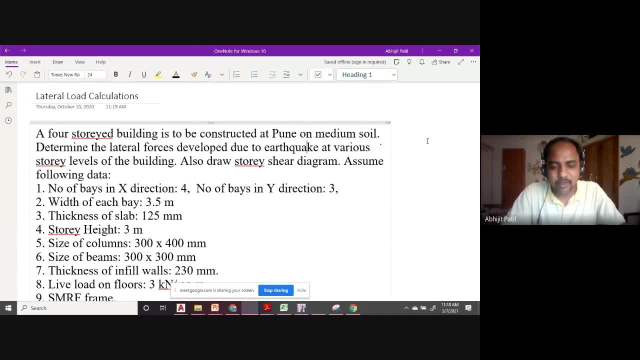 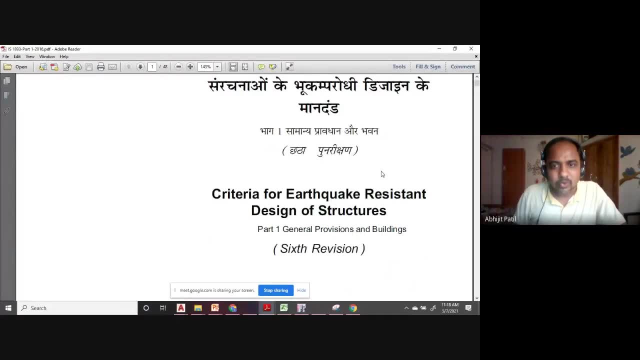 on a typical building and for that we have some guidelines from this Indian standard. so this is criteria for a resistant design of structures. part one: general provisions and buildings. so there are actually four parts, but part one is most widely used because this is basic general provisions plus few. 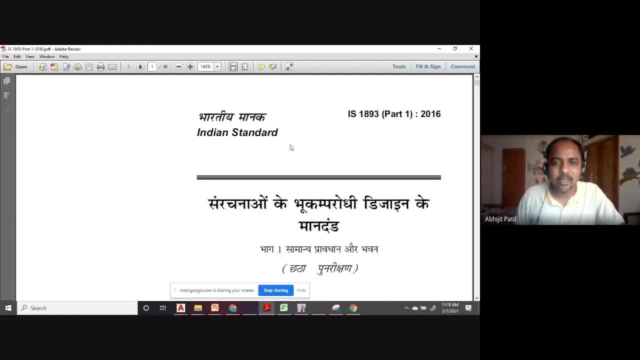 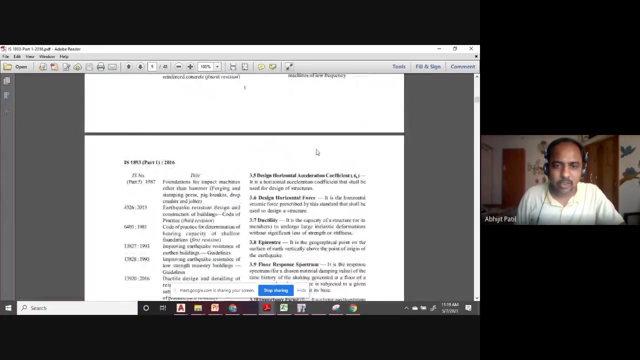 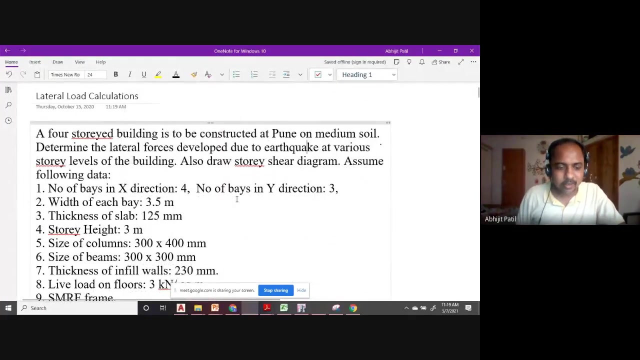 specific provisions related to buildings are provided, and the standard number is is 1893, part one, and it has been recently revised in 2016, after the Nepal earthquake. okay, so we will be referring to these as a guideline for calculating the earthquake force. so just a second, yeah, so I hope that everybody has written this formula and 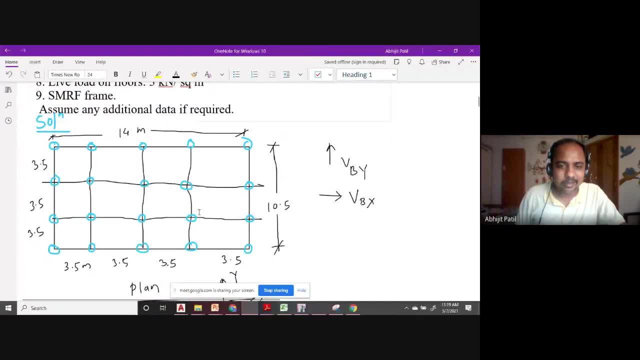 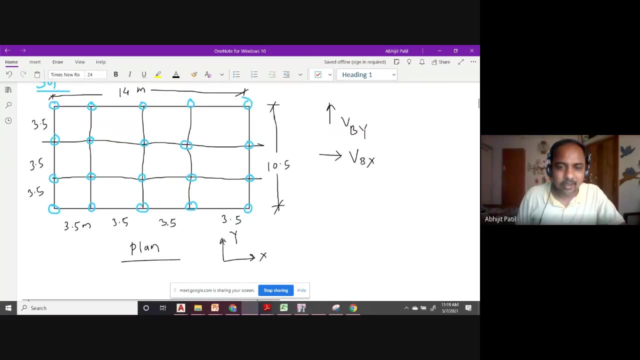 sorry written. this problem and this scale related to the numerical. so basically, this is a building with overall dimension: 14 meter by 10.5 meter. okay, so this is plan. so in plan, this is X direction. this is Y direction. this is just for our assumption. 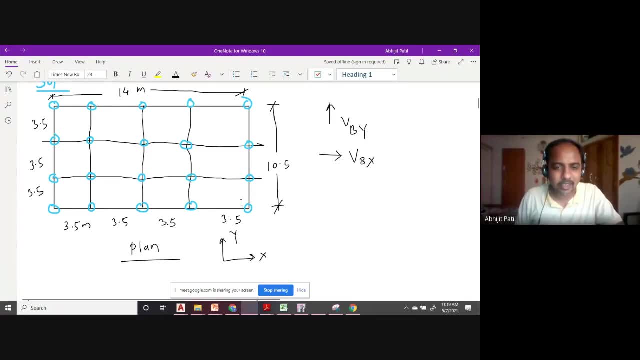 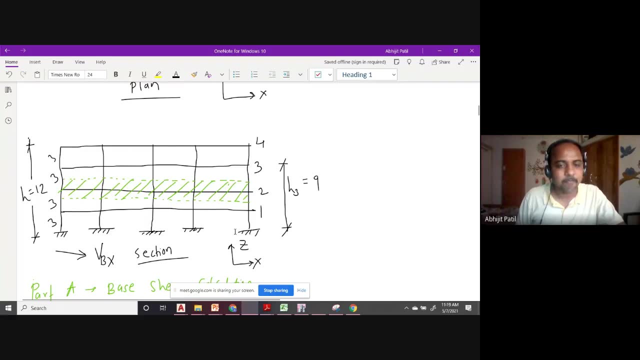 can assume anything, but this is generally accepted: X, Y and vertical Z and this is a cross-section. so this is in X direction and this is the vertical Z direction. okay, and whatever lines are shown, these are beams and the circles, these are columns. similarly, here, the vertical lines are columns, the horizontal 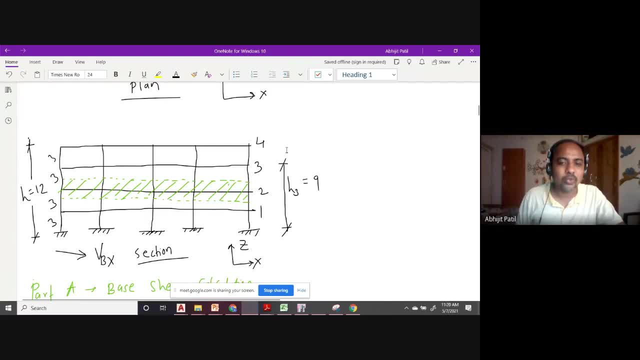 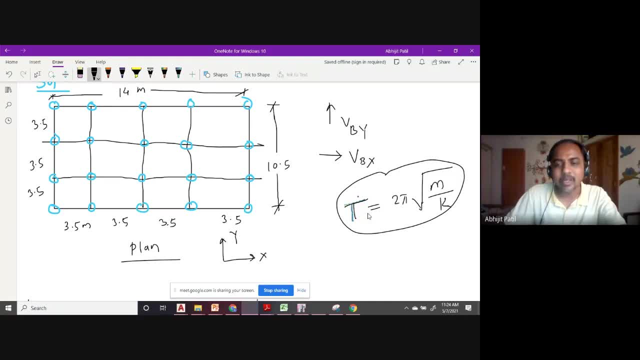 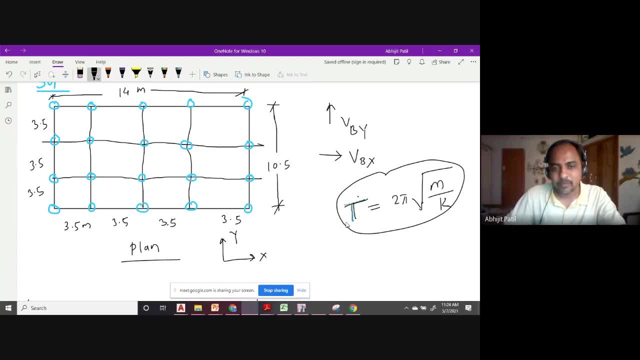 called as inertia force. okay, if you change the mass or stiffness of the building, the earthquake force coming on the building will also change. okay, that is the thing to be remembered: that other forces are external factor dependent, but this earthquake force depends on the properties of the structure itself. okay, 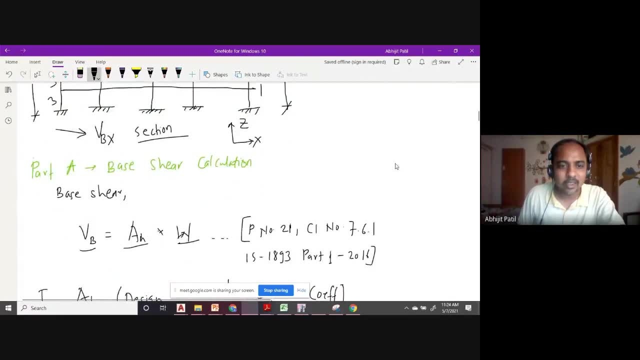 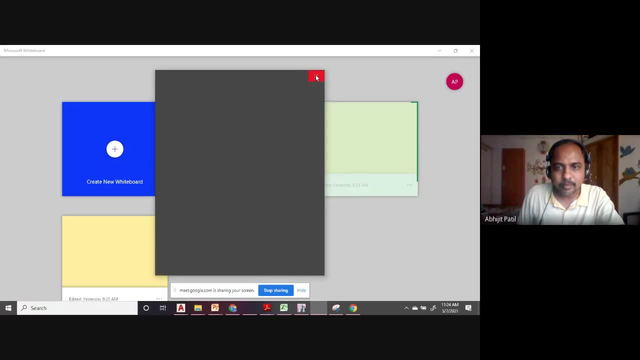 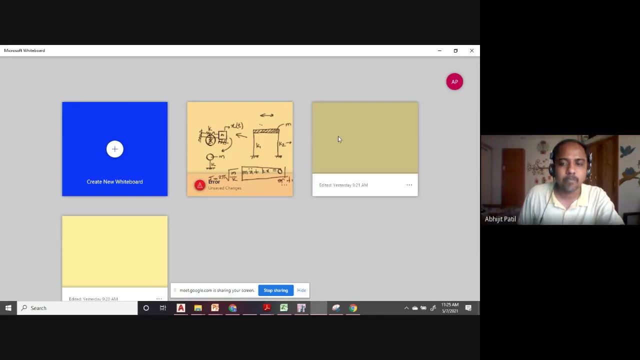 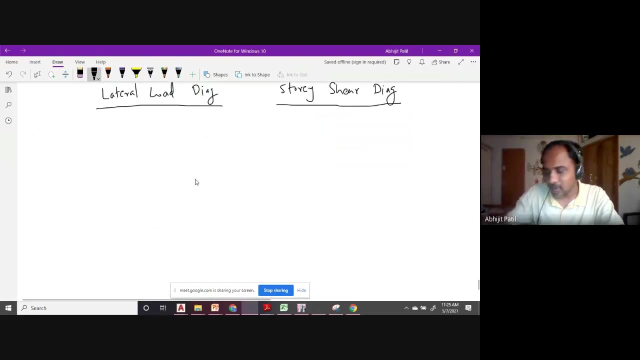 so now we will actually go and see how to calculate the earthquake force. so before that, let us project about this. I will explain here. it's called as inertia force, okay, so now we will actually go and see how to calculate the earthquake force. so before that itself, okay. so basically I will draw cross section of a building like this. so 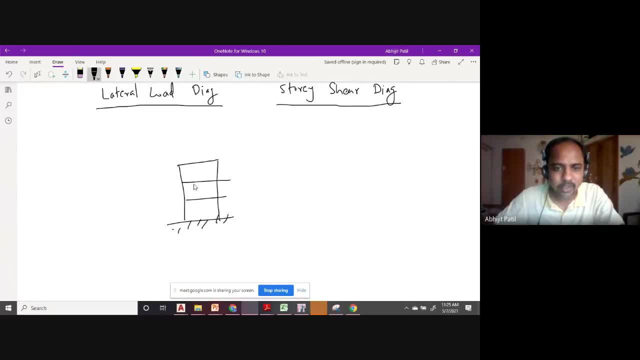 there may be a number of stories, number of columns, etc. etc. okay, so this is elevation of the building, so the earthquake force will act in this direction. okay, so this ground will vibrate like this, okay, and the building will vibrate in this direction and because of this vibration or motion, this 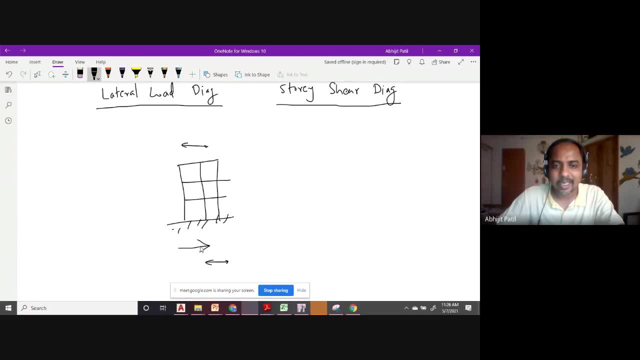 building will experience a force in a direction opposite to the direction of motion. so that means, if you remember, inertia forces, okay. so suppose you are traveling in a bus, okay, and the bus is moving in this direction, somewhere inside you are sitting here. it make say you are sitting somewhere here and the bus is stationary. 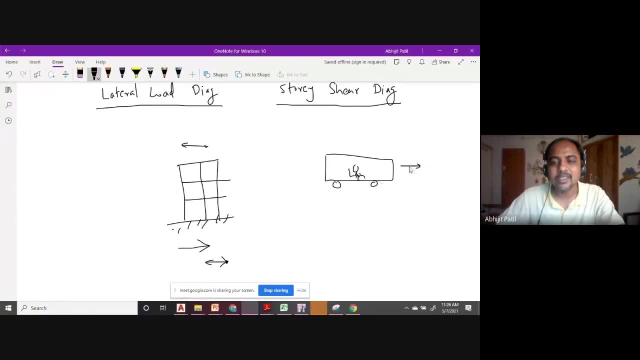 for example, and then firstly see the tama of심carry pistons in it and then smoking energy forces over here and then suddenly the driver pushes the accelerator and it moves in this direction. so what you feel? you feel that somebody is pulling you back. 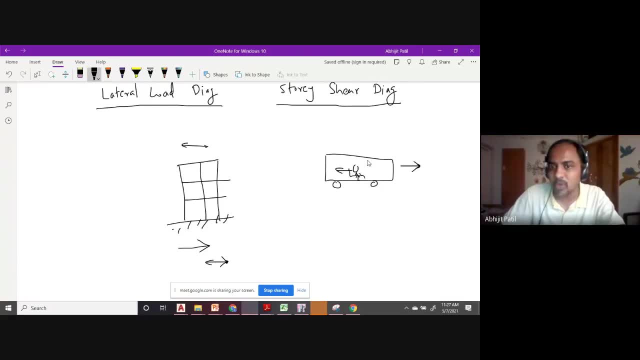 right. if you are standing then you will experience this force more because the cg of the bus and cg of the your body, that distance will increase as compared to the sitting position. so this is called as inertia force from newton's second law of motion, f equal to ma, and the direction of this force is always: 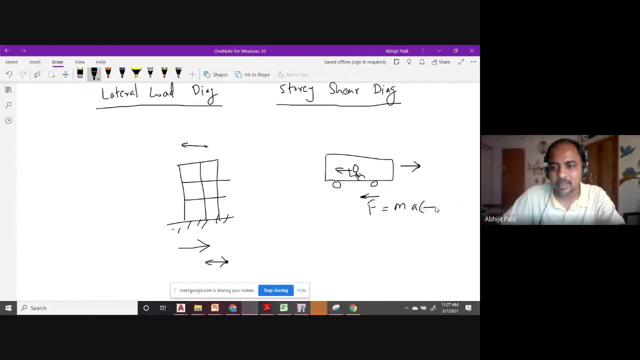 if this is the direction of the force, this is the direction of the acceleration. so in the direction of uh, opposite to the direction of acceleration, you will experience this force. so this is called as inertia force. okay, i hope you have understood this example. so uh, building- now building is stationary for 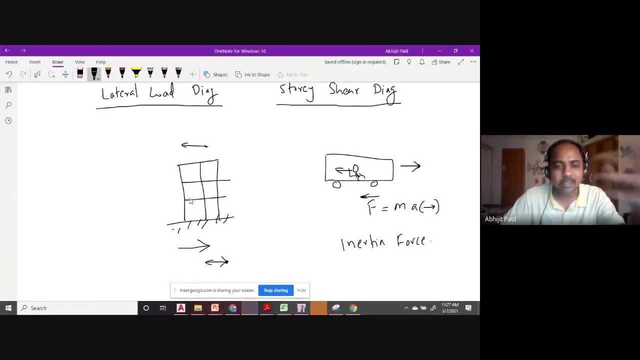 5 years, 10 years, 50 years it has been standing on the ground and the ground is stationary, so it is relaxing, no tension, but suddenly the driver. so here it was the driver. okay, so here who is the driver? okay, so here is the driver. this is the driver. the earthquake the driver. 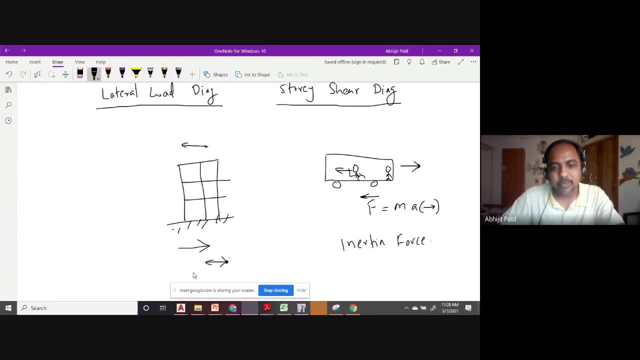 pushes the accelerator- okay, and seismic waves pass through this because of that earthquake. okay, and these waves. now this bus is traveling in one direction, but this driver is very skillful: it travels forth, back, forth, back, forth, back. so imagine you are sitting in this bus and the driver is suddenly accelerating in. 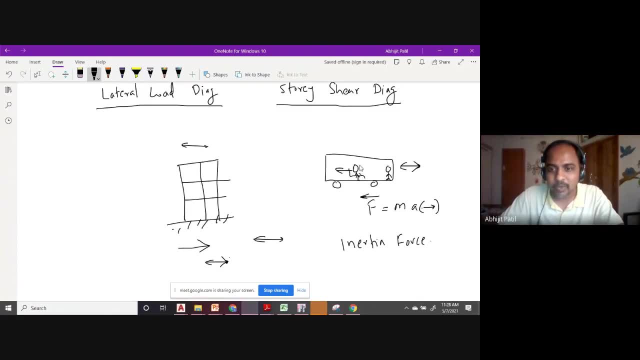 forward direction, backward action, forward, backward. so what you will feel, you will also experience: somebody is pulling you, pushing you, pulling you, pushing you, but it is in the opposite direction of the motion of the bus. so same thing will happen here. this ground motion bus is traveling back and forth. 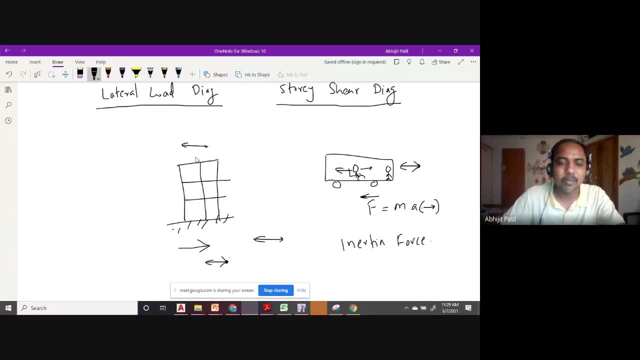 back and forth, and this building will also experience that somebody it's pushing it backward, pushing you forward, back and forth, back, helpful, but that somebody is nothing but mass of the body itself. okay, so your mass, let's say you are of 50 kg and another person sitting beside you is off 70 kg. so obviously, 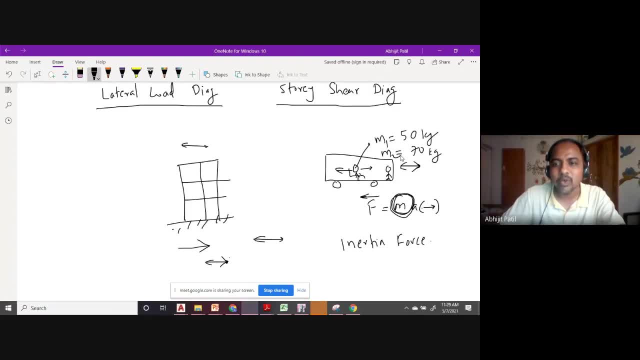 this second person, m2, will experience more, more force than you if you are of 50 kg, Understood this. So this building is also experiencing same force, And who is pushing it? Nobody else but its mass itself. So I jokingly say that this Newton's second law. 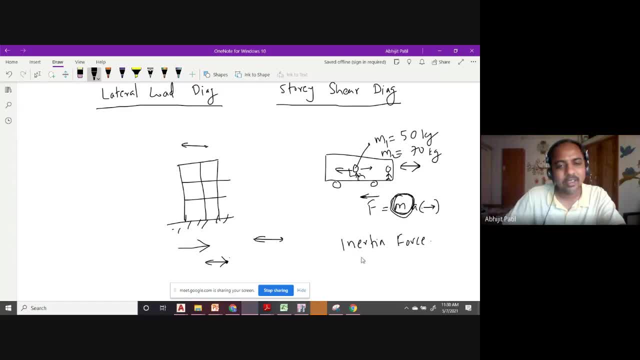 or the inertia force is nothing but laziness, Why it is experiencing laziness. Suppose this is traveling in this direction, in the forward direction, And what is happening? This part of the building, because it is attached to the ground, it has no option but to travel. 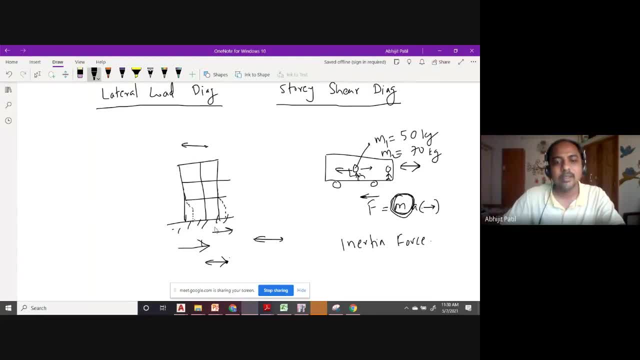 with the. Let me Use another thing. So this is the position when the ground is moved by this small distance during earthquake. So what has happened? The columns, or the structural frame part, which are the part of building and attached to the ground. 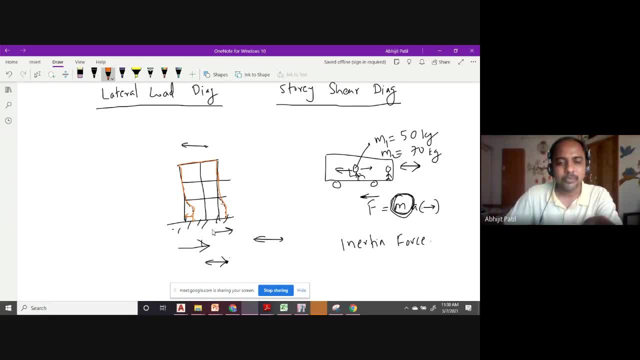 they have no other option but to travel with the ground. OK, But here at top what is happening? They are lagging behind, They are reluctant. The mass is very lazy If you remember the first law of Newton's, first law of motion. 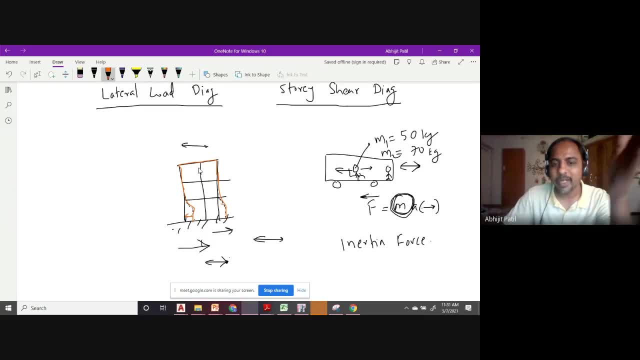 every body or mass which is in state of rest or motion will continue to be in the same state unless some external force is applied. OK OK, OK OK. But this means that the mass is very lazy. It doesn't want to change. 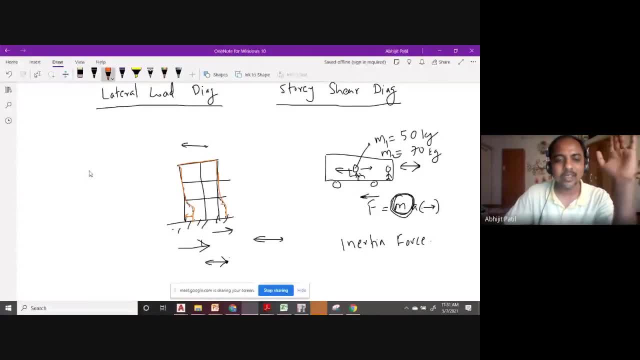 If it is traveling, it wants to travel continuously. If it is at rest, it wants to rest there itself. OK, So if you are sleeping and in the morning your father or mother are calling by your name to wake you up, but you want to continue the state of sleep, you don't want to wake up. So this is a natural, inherent property of living as well as nonliving. The state of sleep is when you are still in the same place, The same things. If you are playing a game, you want to continue to play. 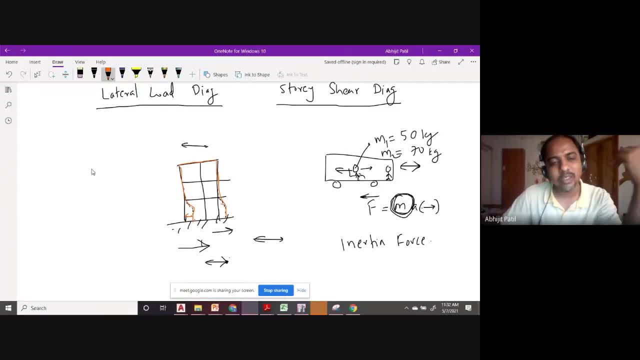 You want that your time should stop there and you should play continuously, Because you are enjoying that state of rest or state of playing or state of sleep And you don't want to end that state. The same thing happens with the mass. 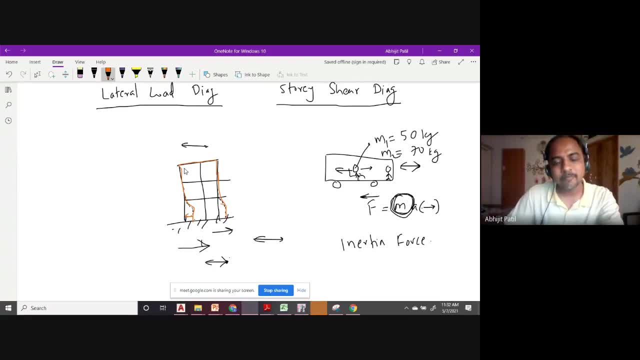 So this mass is not ready to move, the nagging of your father or mother will start. so you think that instead of listening to all this nagging, it's better to wake up. so you wake up. so same thing happens here. it resists the motion as far as possible, as far. 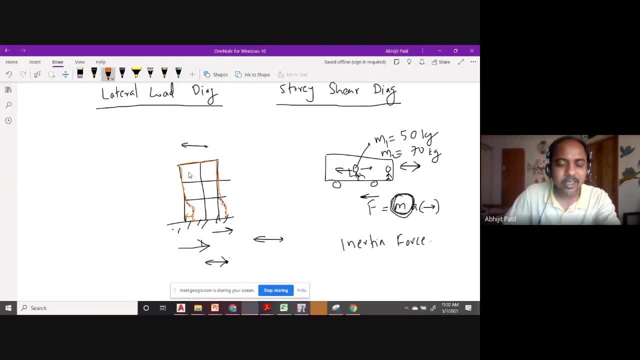 as it can be here. but then it understands that it has no other option. otherwise what will happen? this building will move, some part will move ahead and some part will stay behind, and the building will get damaged. okay, so it decides that there is no other option and i have to move with this mass. 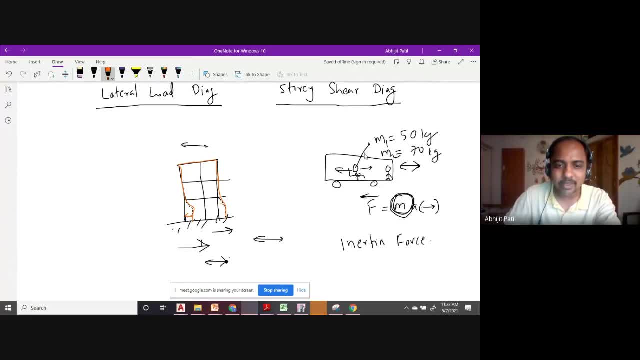 okay, so it starts moving forward. but by that time what happens? because earthquake. if you see the records, they are like this: so this is the mean position, so it will go in this direction, then in this direction, in this, in this positive x, negative x, positive x, negative, x, like that. so by that time it decides to 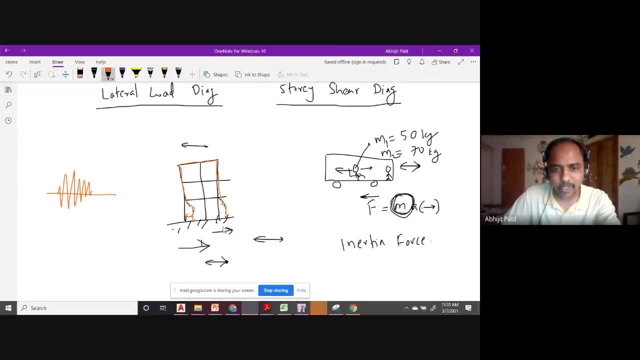 go forward. the building or the ground has already started backwards, generally okay, but it lags behind, so always there is lagging. same way happens in reverse direction. so it is, and because of this this building is experiencing the earthquake force. okay, so if you have some material, 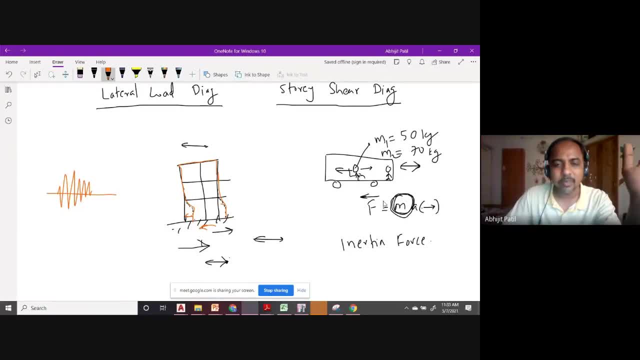 if you can defy this inertia force. that means what? if your building is ready, sorry, if your building. if your building is ready to move with the ground, okay, so there is no lagging here. what is happening- the upper stories are lagging lower, so is moving with the ground. if the entire building moves with the ground, there will be zero. 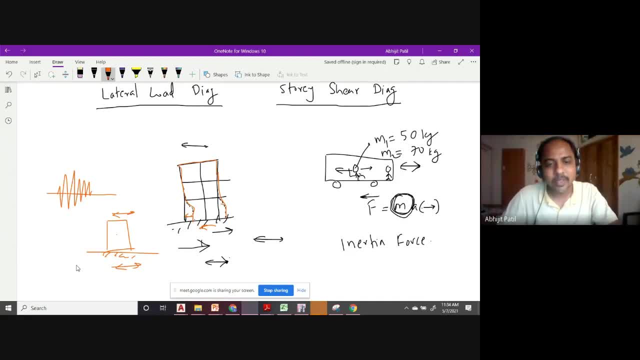 earthquake force, there will be zero earthquake force. even this concept has been tried and that is called as base isolation. so this is something advanced. if you are interested, you can search on this, this isolation. so technically this is possible to do. okay, but for normal of course, the cost involved is very, very high currently. so for normal buildings we have to. 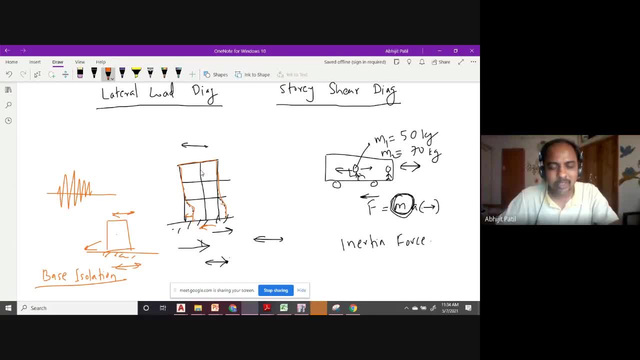 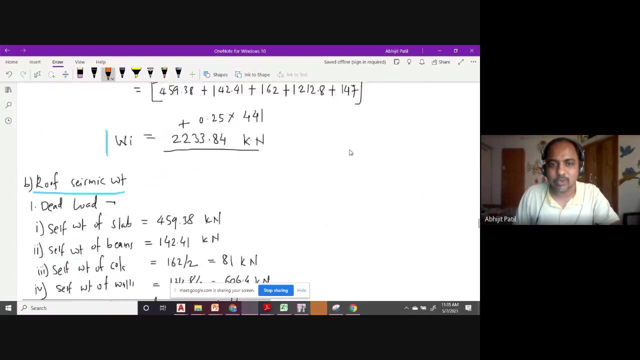 follow this inertia force and we have to understand why the force is induced. so i hope that this is understood. because of this newton's first law and second law, the body experiences and because of its laziness, structure, experiences the inertia force. okay, now coming back to numerical 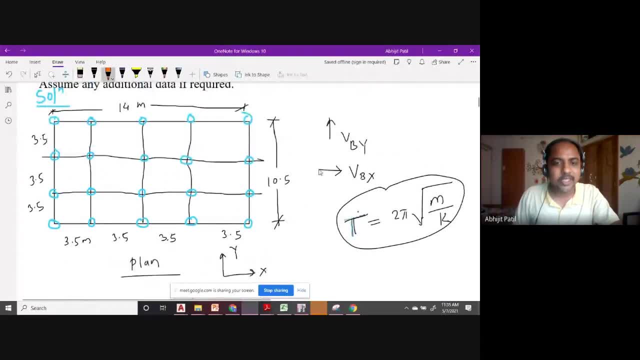 now this force is acting. always we consider, because we don't know- earthquake, from which direction it will come. it may come 45 degrees or 20 degrees. you want to find out what is the force. the Tran fragrance plane has gone there because if you want to get accurate, you can design it there. and then final failed here starting. it should fly different protractions. if this force move from one direction to the other, it is actually kind of worse like ruff. from which direction it will come, we cannot know. it may come 45 degrees. you can see that bad force disappears because of it. 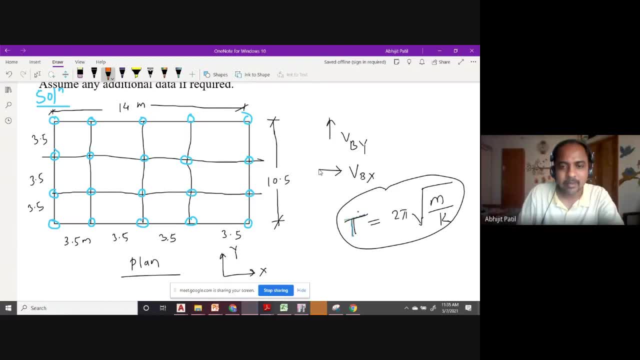 which is blunt forces going how itیrctly is brought back through the structure. you need a few local forces. this may be to X, it may come 30 degree to Y. okay, so what is the solution? we cannot just go on calculating the earthquake force in every possible direction. so what is the 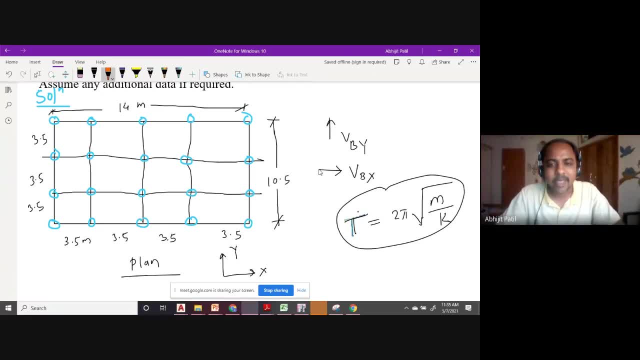 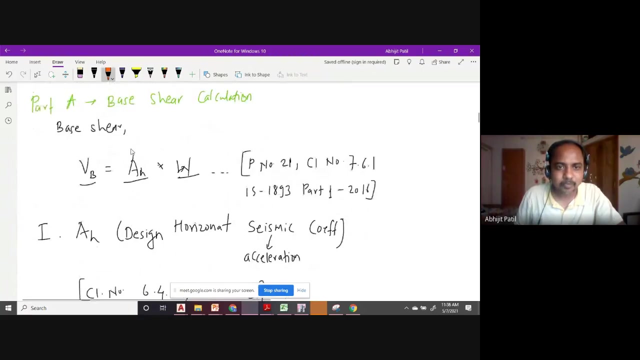 solution suggested by code. we have to calculate maximum earthquake force in X direction, maximum force in Y direction and design your structure for these two directions separately. that will be enough. okay, so this earthquake force is called as base shear. the base shear means the why it is called as shear. 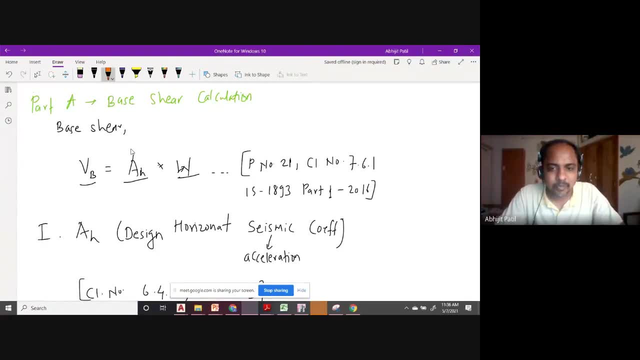 because it is in shear direction. lateral direction- okay, it is not vertical. vertical force is called as your axial force and this is shear force. so base shear means the total earthquake force acting at the base. so that is the part A of this solution. so we have to calculate the total earthquake force acting at the 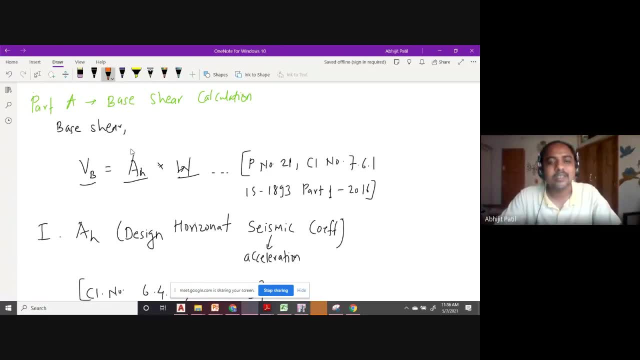 base of the building and then it gets transferred at each story level above. so that will be part B. so first we will just calculate what is the total earthquake force that will be acting at the base of the structure. so this is the formula. please start writing. okay, so where, from where I had got this formula? 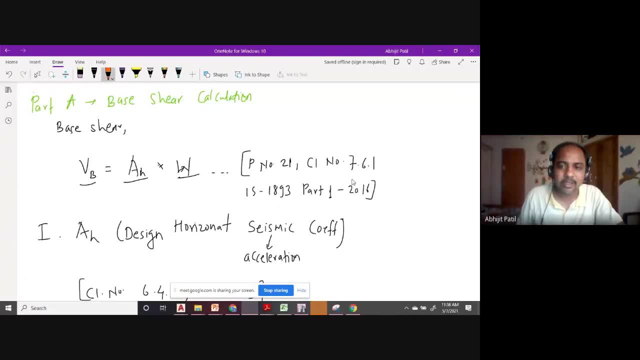 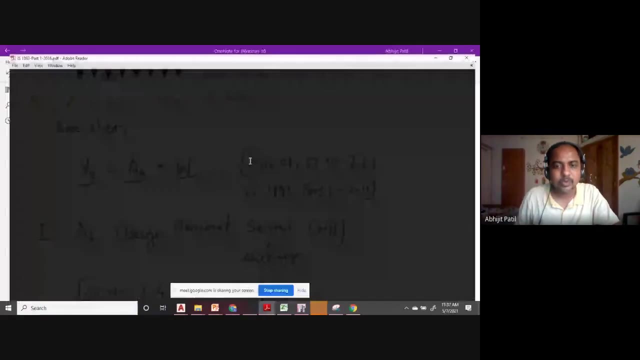 so page number 21. you may have a habit of writing this page number, clause number, so that in future you get to know from exactly where that part is taken. so we will go to page number 21 of is 1893. so this is is 1893, page number 21. 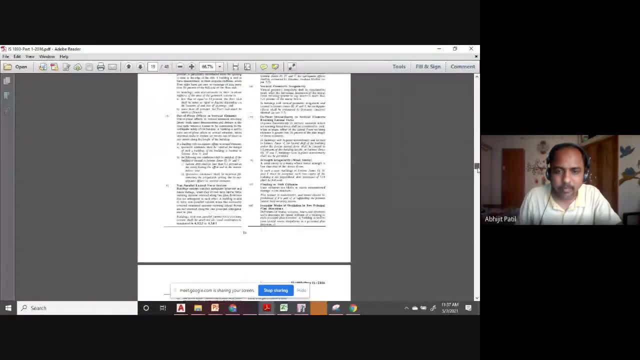 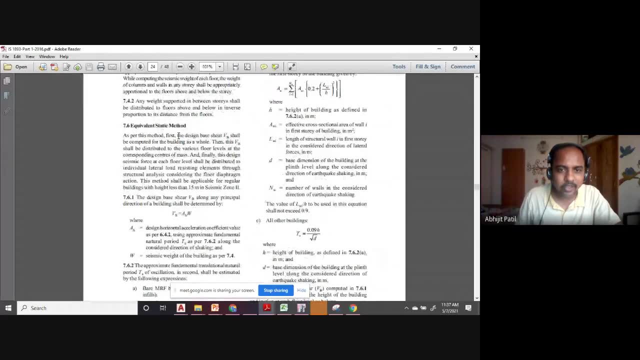 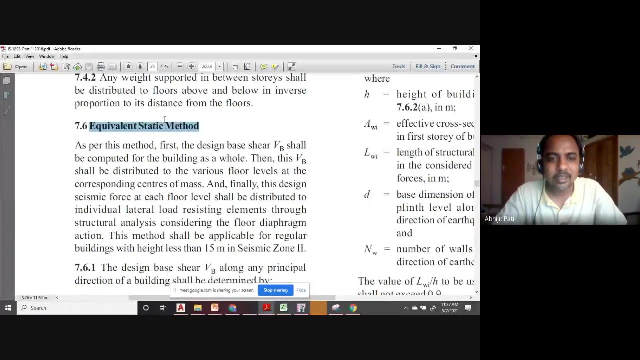 1893, page number 21. you have a that comes out of page number 6. okay, man 8". okay, this line is also in our Tubos of most. so how are you getting this correct? okay, I think we have got it right, all set. so now, if you take that particular page number, 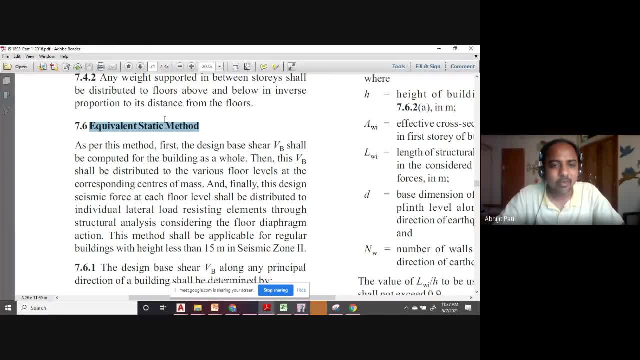 then again there are dynamic methods. that means what is static and what is dynamic. the difference is the force or the response of the building. both they change with respect to time. okay, so dead load or live loads, the load of the wall- it doesn't change with respect to time, so that 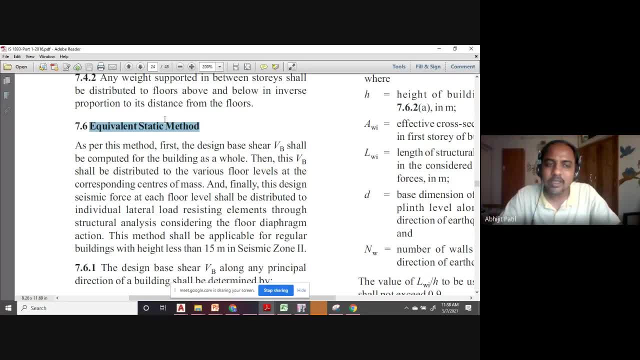 force is static force. wind load: it is dynamic force. it changes with respect to time. earthquake force: it is a dynamic force. it changes with respect to time, but it is very time consuming to calculate the exact time variation. so what is done? we agree to some solution that we will consider maximum wind load. 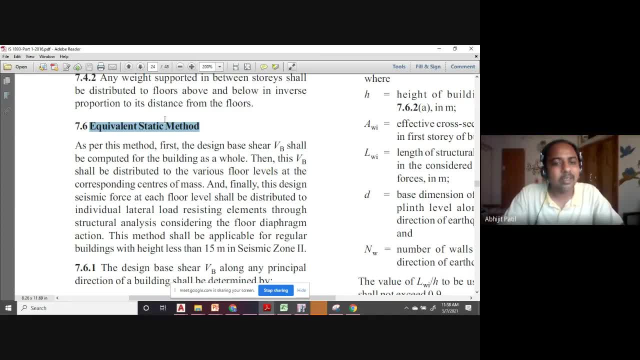 or maximum earthquake load, its time variation we will not consider and the maximum force we will apply, and then we will analyze our structure using static method. so this is simplified solution and now a lot of uh sophisticated software are available, so dynamic methods are also used for high-rise buildings or even for normal mid-rise building also. 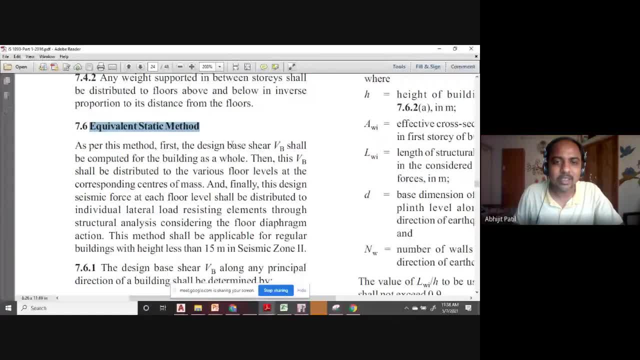 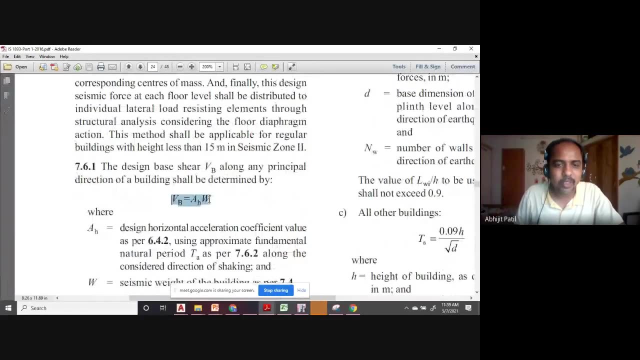 okay, but uh, to understand the basic concepts, we will. or even your syllabus is mentioning this equivalent static method. so for normal buildings, this method gives good results. so, coming back to this formula, vb, equal to so, vb is your design base share for which building is to be. 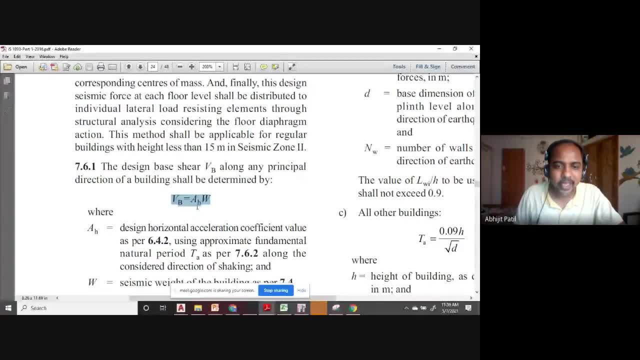 designed. so vb is equal to ah into w. so you can see there are again two parts: a, h and w. so ah is design horizontal acceleration coefficient as per clause 642. so to calculate h we have to go back to clause 642, using approximate fundamental natural period. 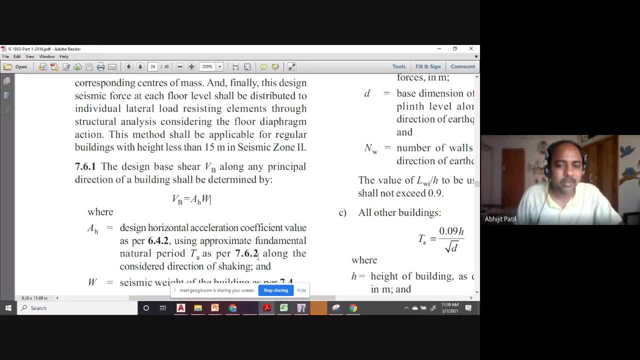 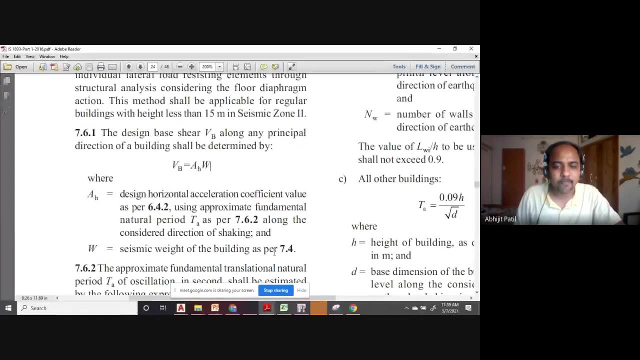 ta, as per clause number 762, along the right hand side, we will consider direction of shaking. that means x direction- we will have different time period, y direction, we will have different time period, and w is seismic weight of the building, as per clause number 7.4. okay, so try to understand. 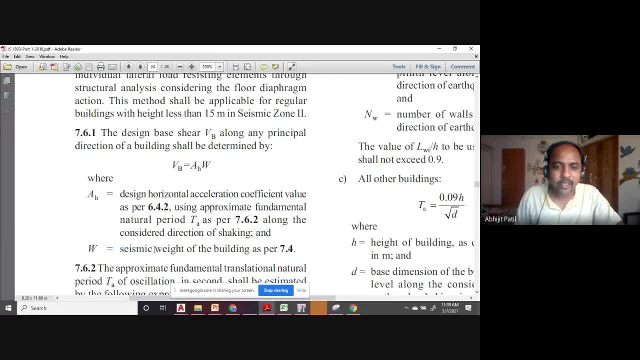 w is your seismic weight. this is not normal weight. so seismic weight is something different than normal weight. so we will see what is that and ah is some coefficient. so basically, if you see we are considering some percentage of seismic weight will be acting as horizontal or lateral earthquake force. so that is the basic concept to be. 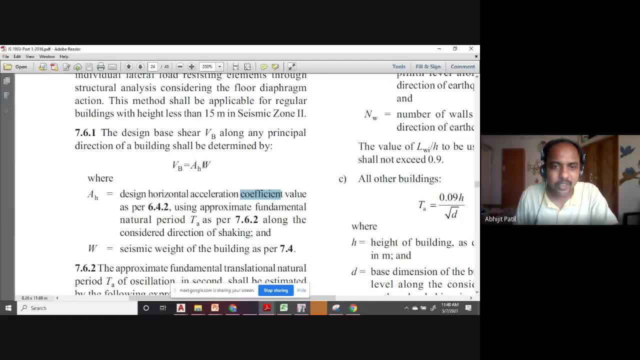 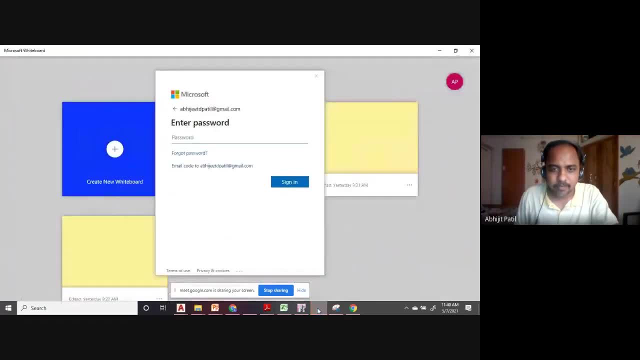 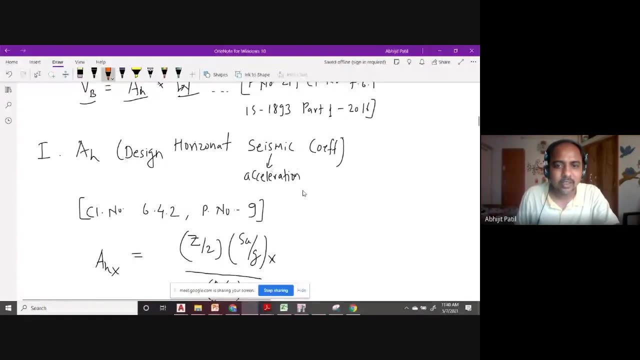 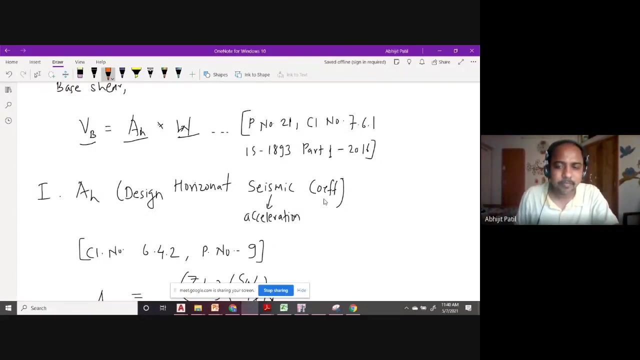 understood here. okay, so we will see how to calculate seismic weight and we will see how to calculate this coefficient, a, h. okay, so this is is i have written here. so in that we will firstly go with age design horizontal seismic coefficient, or it is also called a design horizontal acceleration coefficient. 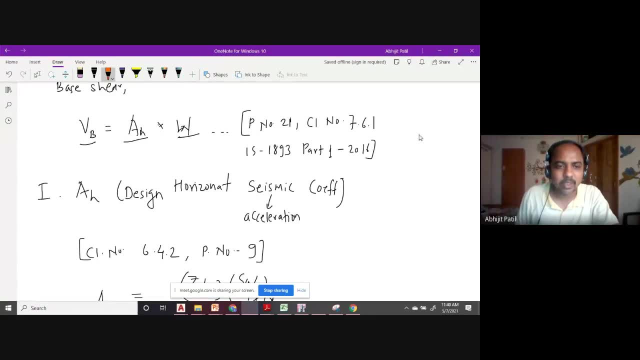 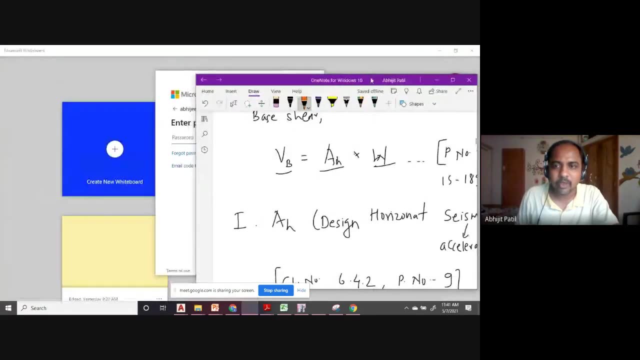 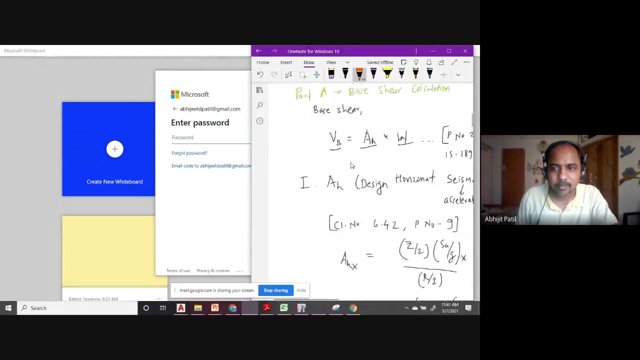 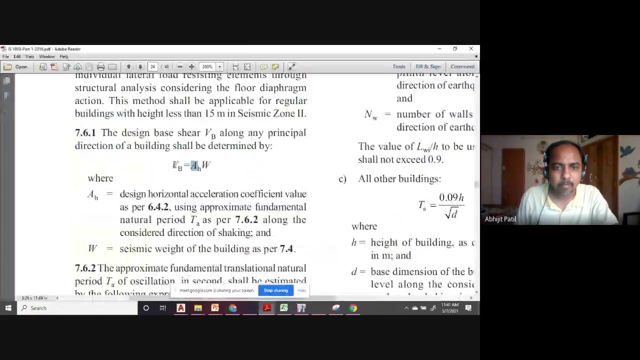 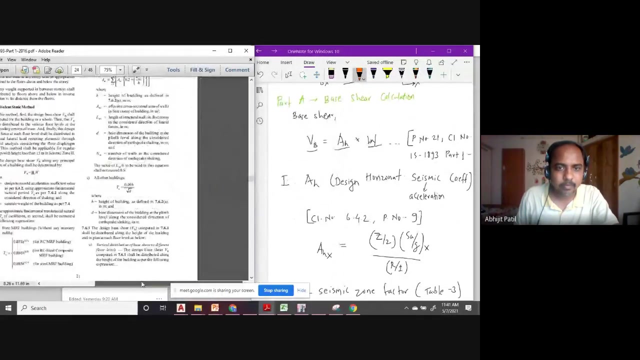 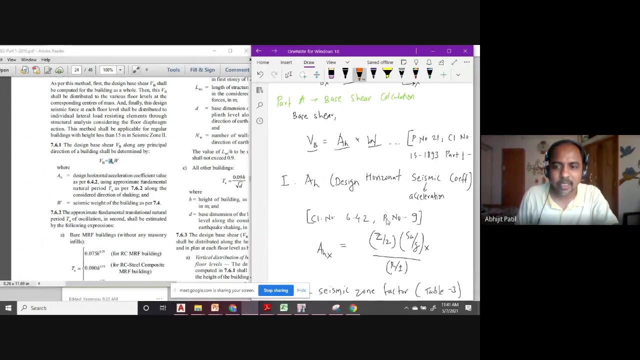 so for this, please write this formula, write the clause number and again write this, what i will do. i will parallely try to show both the screens. and here for h, we have to go to clause number 6.4.2. it is on page number nine. here i have written: 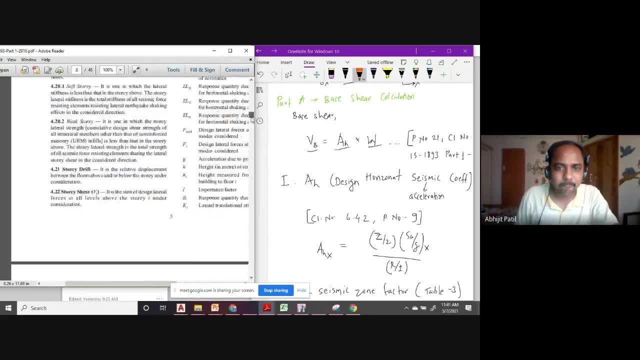 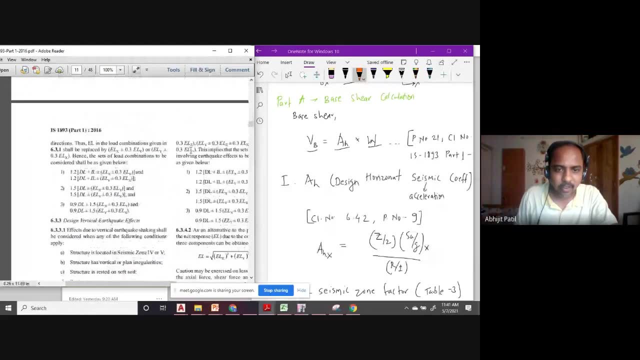 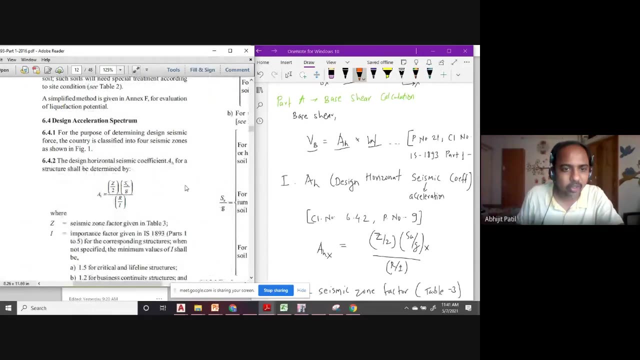 page number nine. so we will go back to page number nine. six, four, two, seven, eight, nine. okay, so clause number six, four, two: the design horizontal seismic coefficient for a structure shall be determined by using this formula. so please write this formula. so here you will notice that h is written. i have written a, h, x, because in x direction. 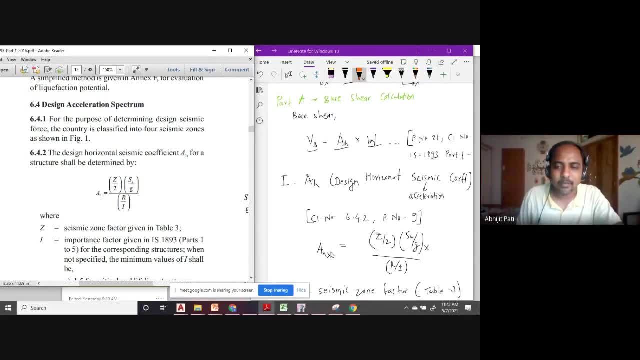 it will be different. in y direction it will be different. okay, so what is this? this is z by 2 multiple, divided by sa by g, x direction, divided by r by i. so you will notice that this z, r and i will be same in both directions. only this sa by g value will be different. 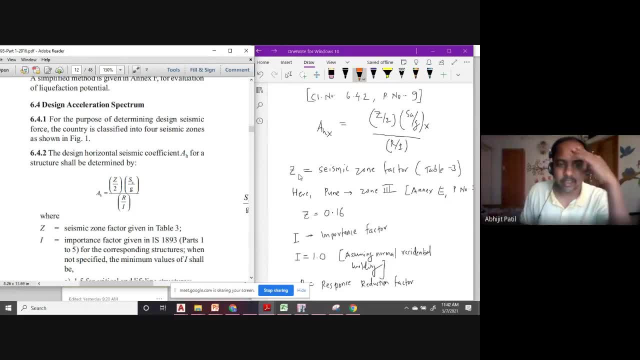 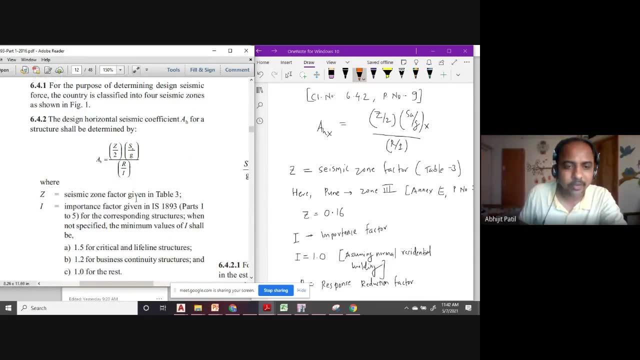 okay, now this z here one by one. we will see each and every term: import. you don't have to remember anything. in code, everything is given. so z is seismic zone factor given in table three. so this zone factor is nothing, but this factor will depend on the seismic zone. 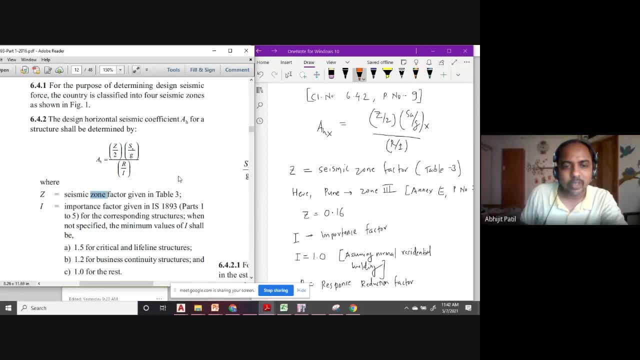 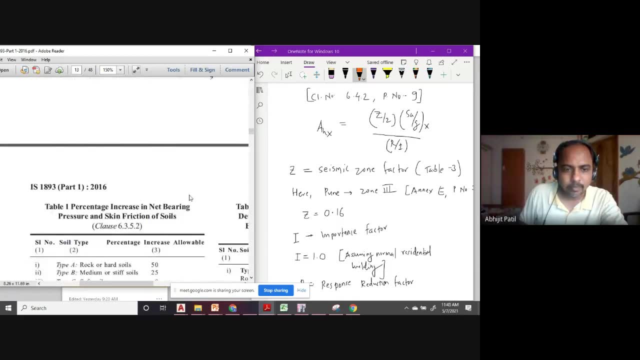 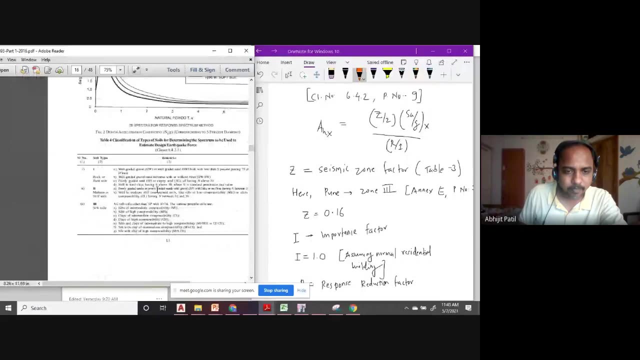 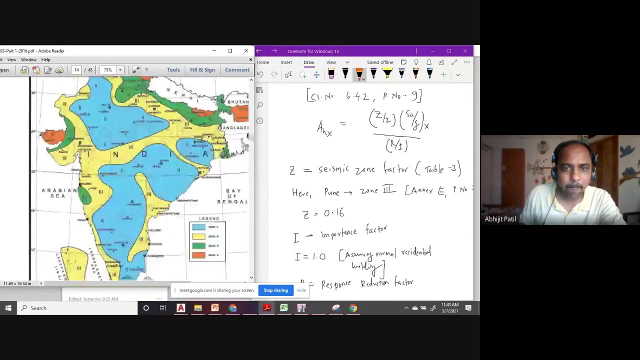 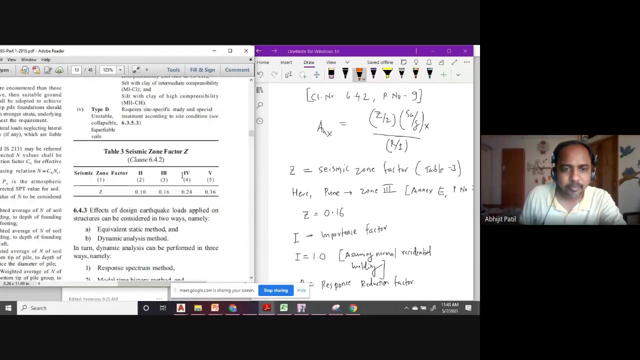 of your location. okay, so we have to refer to table three. so table three, this is table one. table five: sorry, okay, it's here itself. table three on page number ten. okay, so what is given here? the seismic zone factor and the seismic zones two, three, four, five. 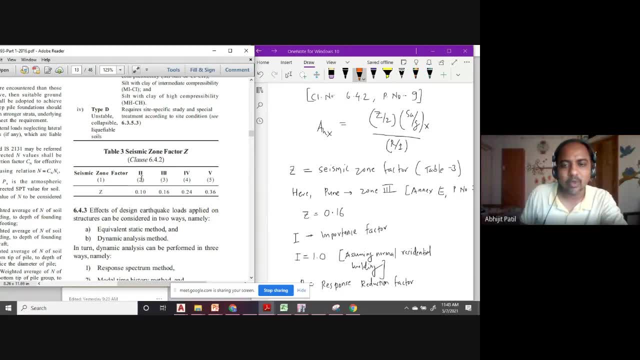 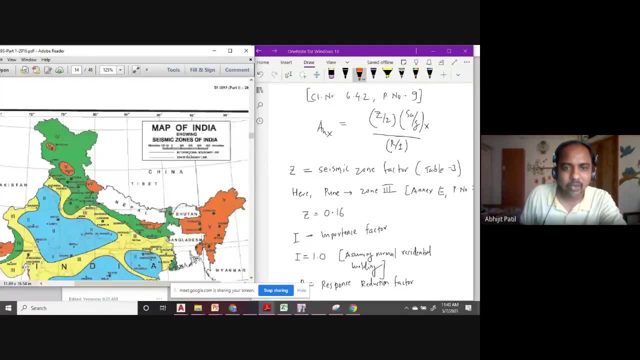 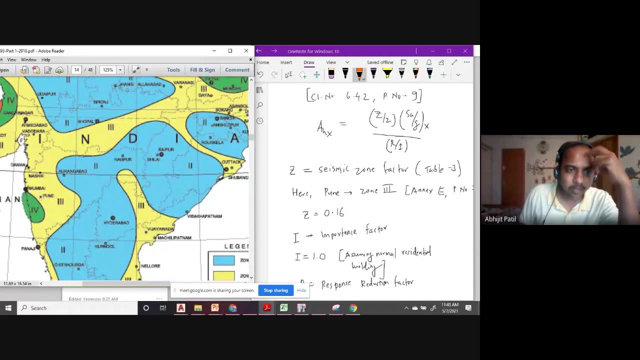 so we must understand, or we must know, our location of the building is in is in which zone. so there are two methods. one, you directly refer to the map. okay, so here we can see. since pune is metropolitan city, it is available here. okay, so this is the yellow region, yellow belt is zone three, or there is an extra e given. 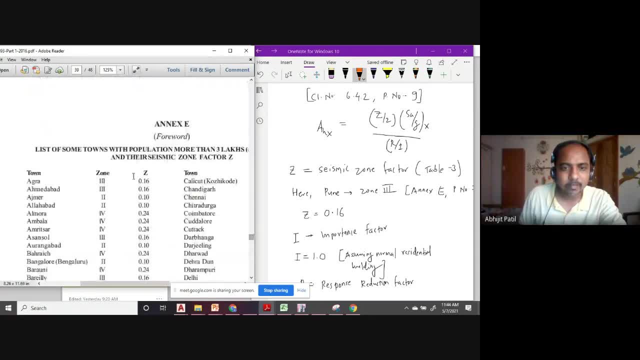 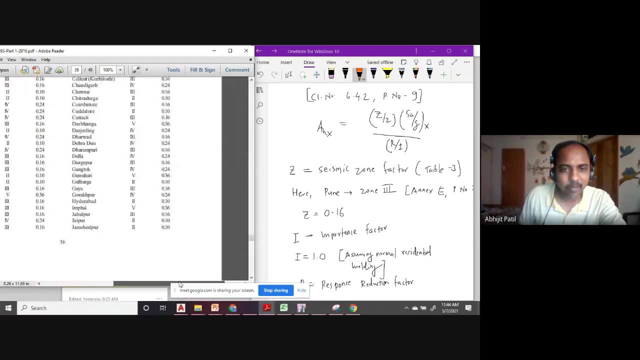 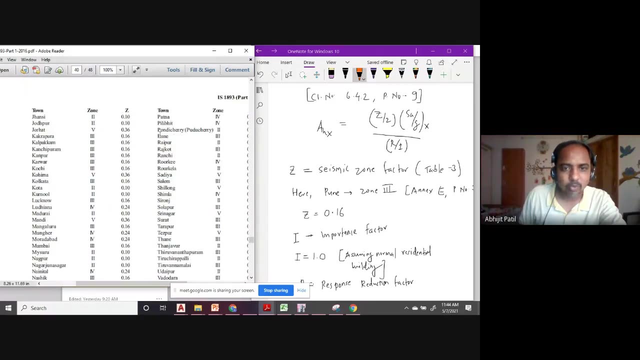 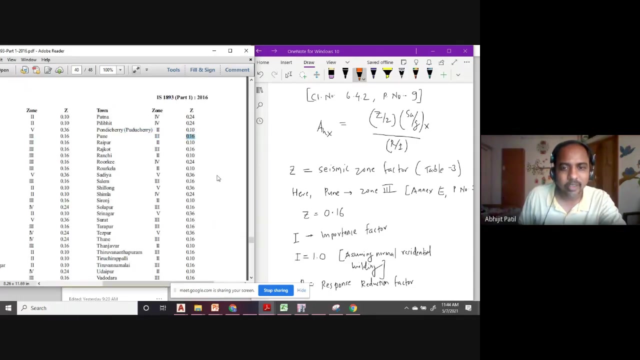 at the end. so annexures are always given at the end where name of the city, zone and zone factor- everything is mentioned here. also you can search alphabetically. so Pune is here, zone 3, and the zone factor for zone 3 is 0.16. okay, and next is E at the end of the ice code or we can refer to table from: 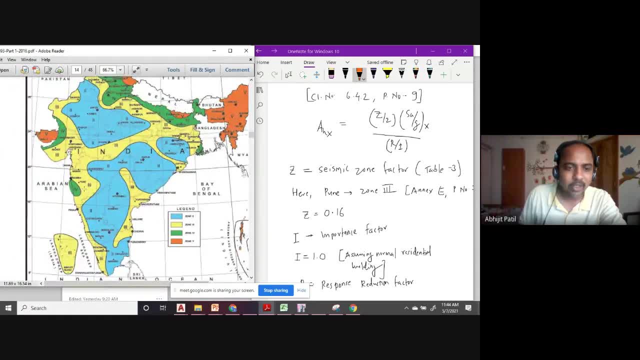 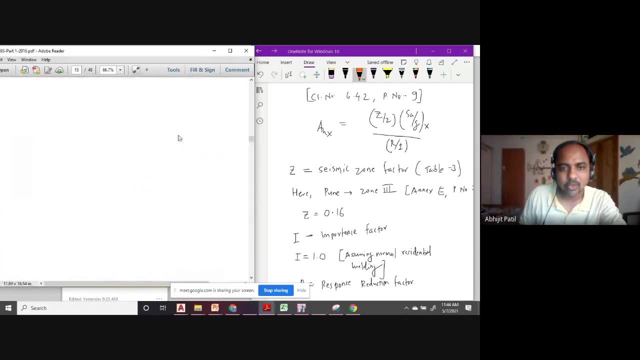 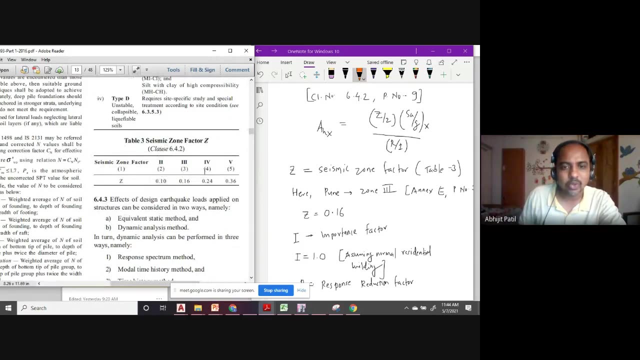 this seismic zoning map of India. we understood that Pune is in zone 3, table 3 here. okay, you have the seismic zone factor for zone 3 as 0.16. okay, so seismic zone factor, you have to refer to seismic zone map of India and then locate your location in that map. understand which zone is that and for 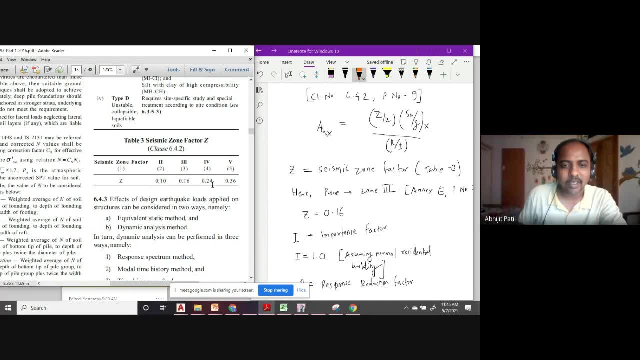 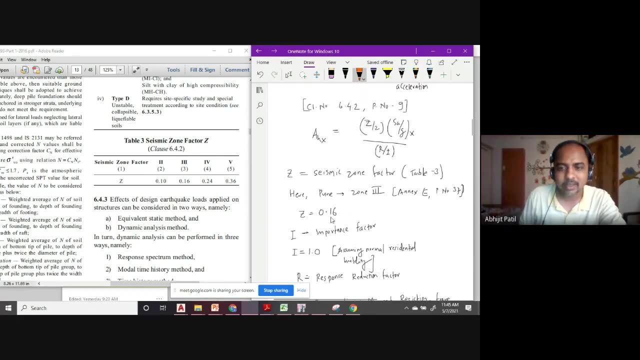 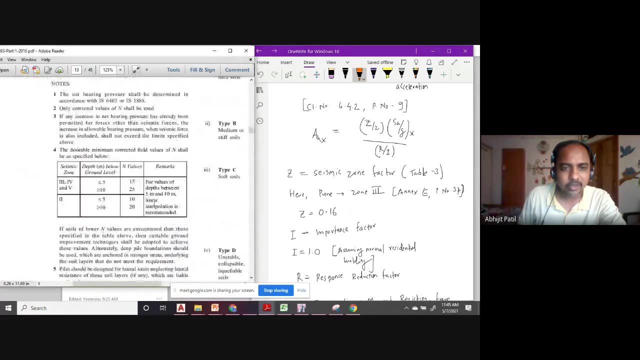 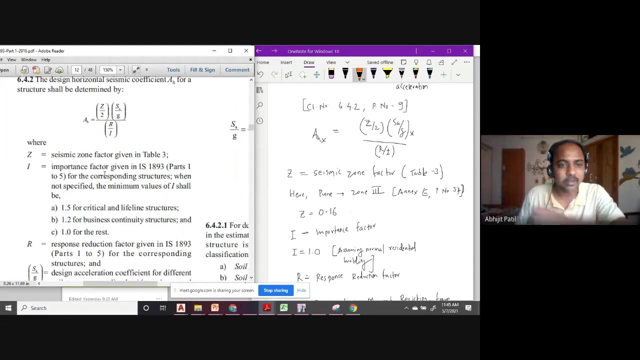 respective zones. you have to take the zone factors value of Z here. so I have written here: Z is equal to 0.16. for zone 3 it is 0.16. then second, is I coming back to page 9? I is importance factor for corresponding structures. okay, so here you will see the 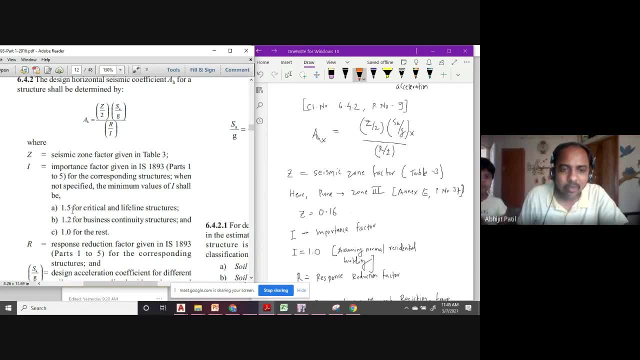 value of I is mentioned 1.5 for critical and lifeline structures. so what are these critical and lifeline structures? so what are the critical and lifeline structures? so you can understand the lifeline means, these can be the communication powers. okay, if the communication towers fail, then your mobile network will be gone, so very difficult to communicate with. 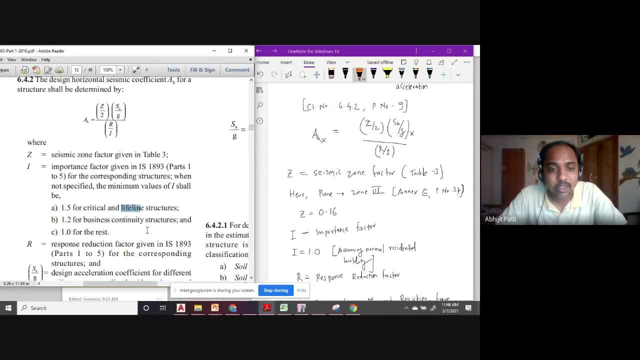 each other in the case of crisis, like earthquakes or floods, etc. bridges or main highways, then lifeline structures can be hospitals. okay, so you can understand the application of these structures. schools, where, in case of natural disasters, these schools are, even for this pandemic situation. we know that schools or hostels are being used as covid centers, as hospitals. okay, so these public 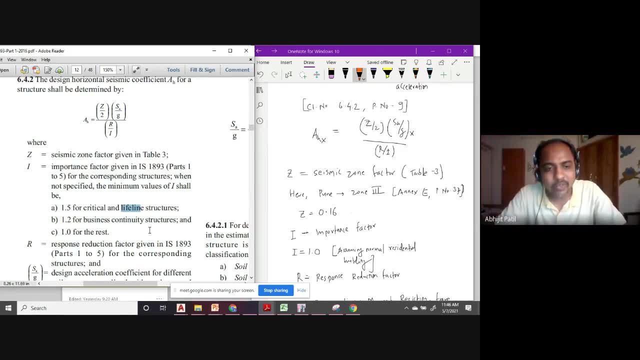 buildings or the government offices. so all these come under this: critical and lifeline structures. then 1.2 is business continuity structures. so these will be just like high-rise buildings where most of the offices, commercial offices, business entities are housed, and for other buildings it is one okay. so importance factor in our case it is assuming that it is a residential. 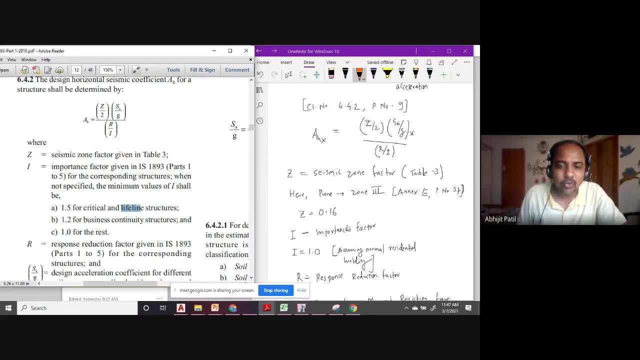 building, we can use i as equal to one importance factor as equal to one. okay, so in our case- it is assuming that it is a residential building- we can use i as equal to one importance factor, one. so understand that this i is r. by i, that means actually more. the value of i, more will be. 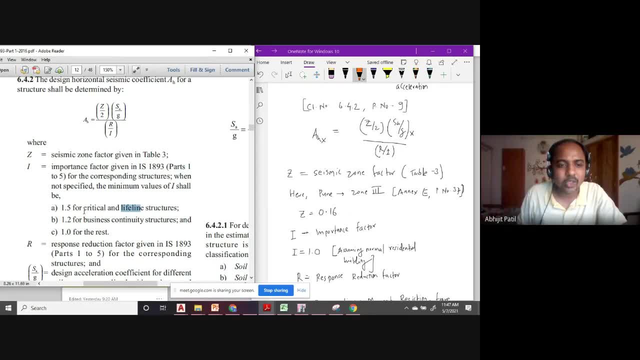 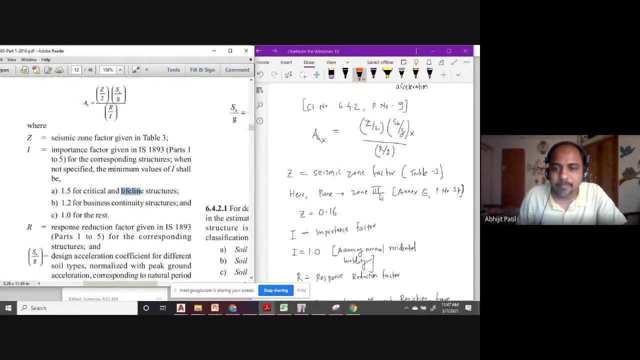 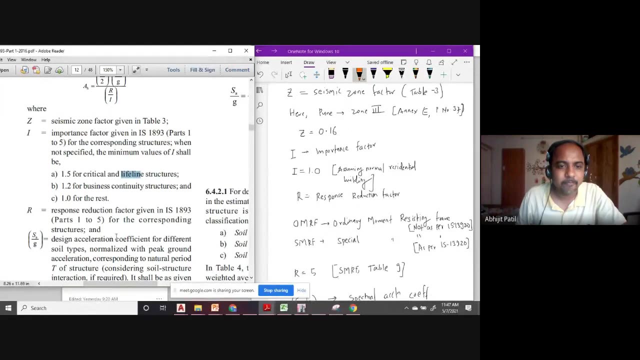 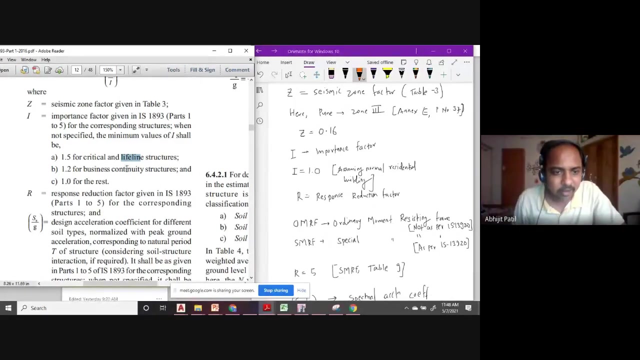 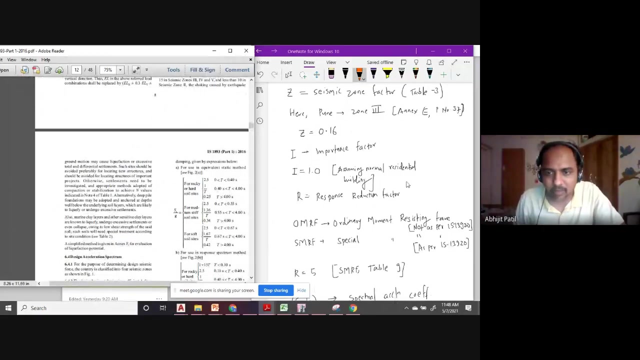 the earthquake force. so indirectly, code is saying: for hospitals etc. you consider 50 percent more earthquake force. okay, then you have response reduction factor r. okay, so this response reduction factor, okay, then you have response reduction factor r. is to be taken just a second. i have mentioned here the 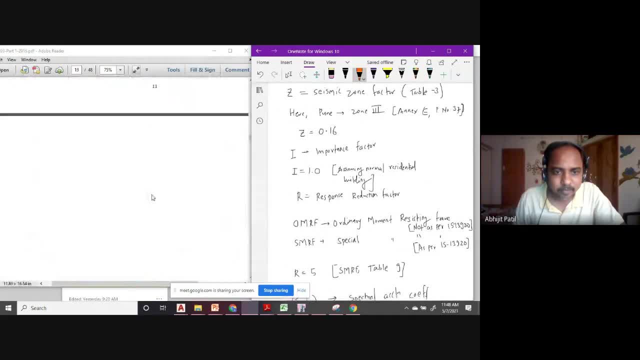 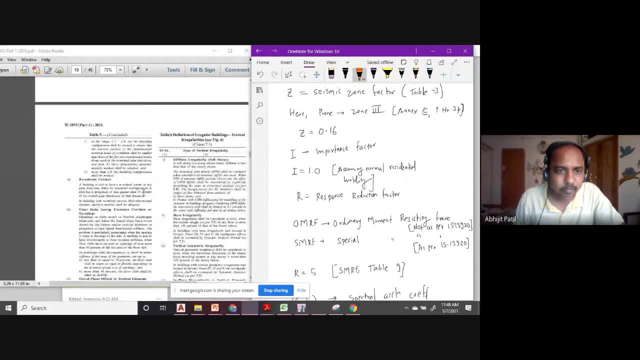 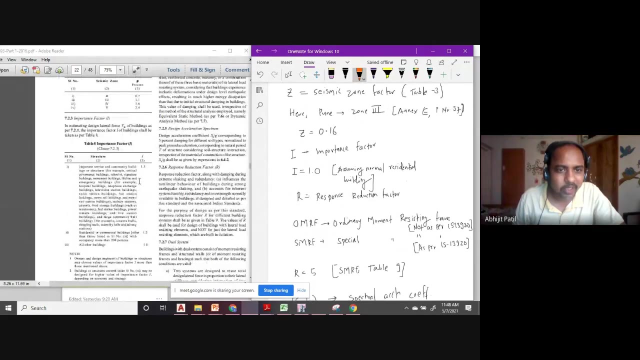 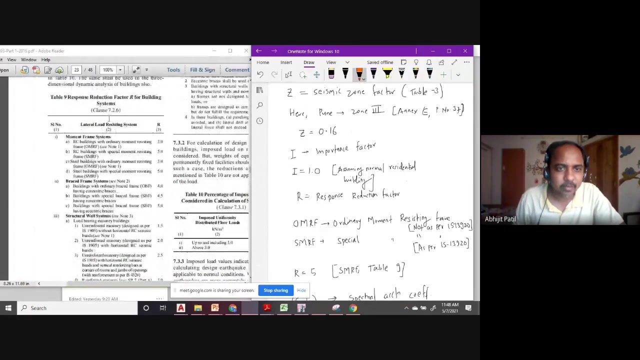 actually there is a table. actually there is a table. actually there is a table. okay, so this is the table. okay, so this is the table. again, importance factor: you have table eight separately for that, yes, and this response reduction factor, it's in table nine, so i will mention that here. 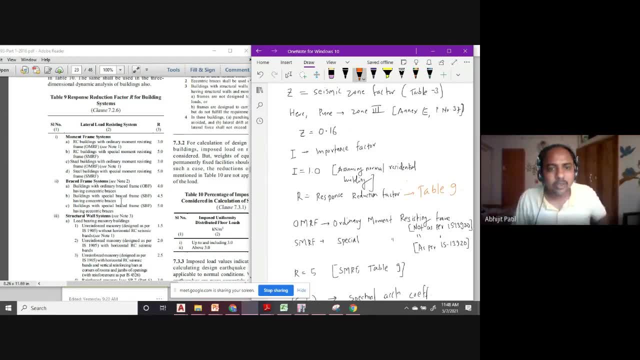 table. okay, so, uh, this depends on the stiffness of the structure. so you have moment frame system, that is, your regular beam column system, is called as movement frame system for rcc, and you have braced frame systems, that is, the steel buildings, particularly having this cross bracing or a bracing, the different types of bracings, and then structural wall system that 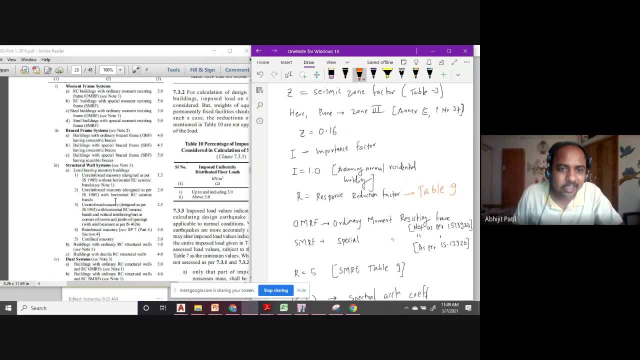 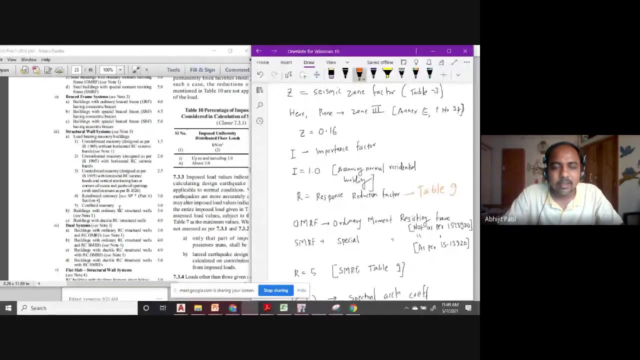 means the load bearing buildings. or instead of load bearing you can use the my one type of buildings. those come under this structural wall system, where all the walls are rcc walls, and dual systems where you have shear wall also and you have beam column framing also. and the last one: 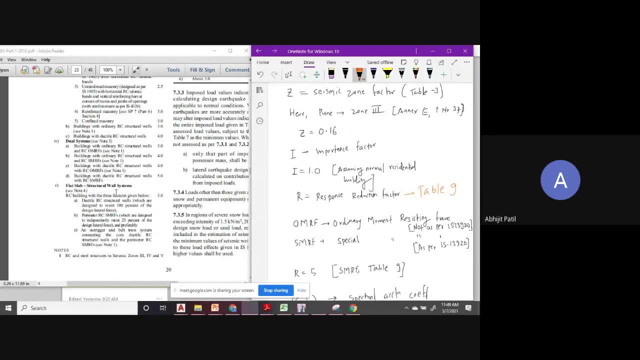 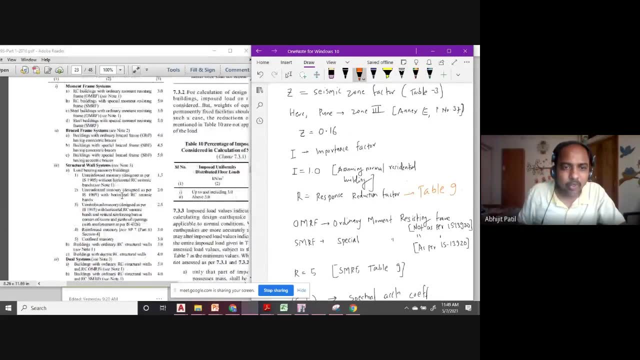 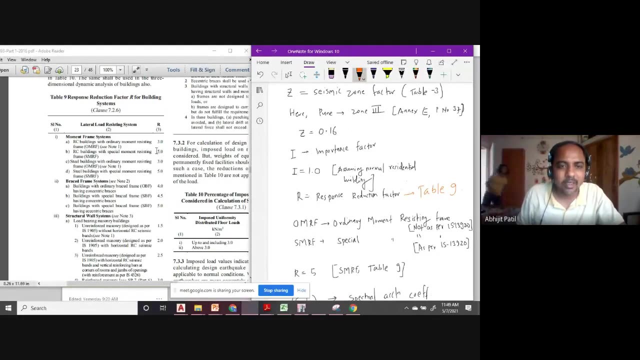 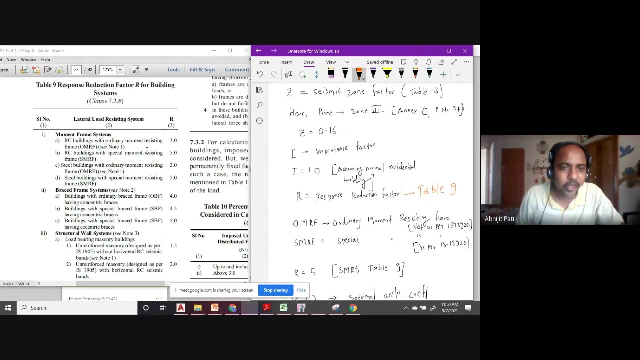 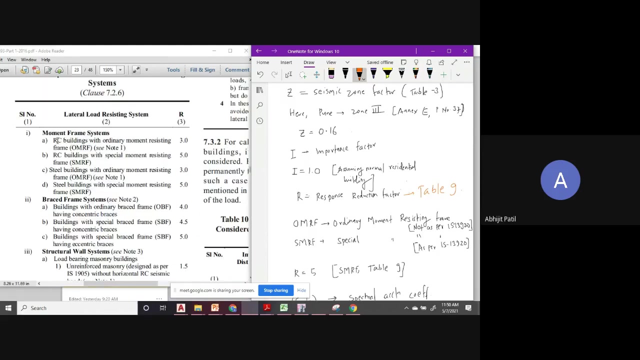 is flat slab, okay, so most of the high-rise buildings, they go for this flat slab. so, depending upon what type of structure you are having, you can use the value of r given. okay. so now will be movement frame system. okay, and there you have this omrf and smrf term. so here you can see rc buildings with ordinary movement resisting. 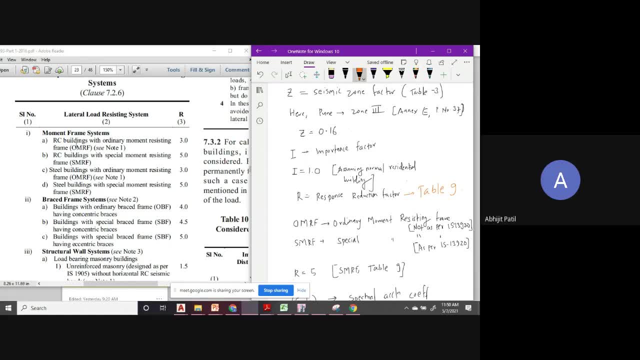 frame. so mrf is movement resisting frame. ordinary and special, these are the two types of frames: ordinary and special. so what is this ordinary and what is special? because for ordinary building buildings, r value is to be taken as three and for special moment resisting frame, it is to be taken 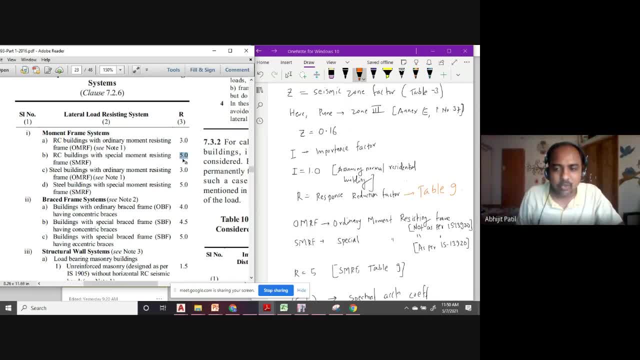 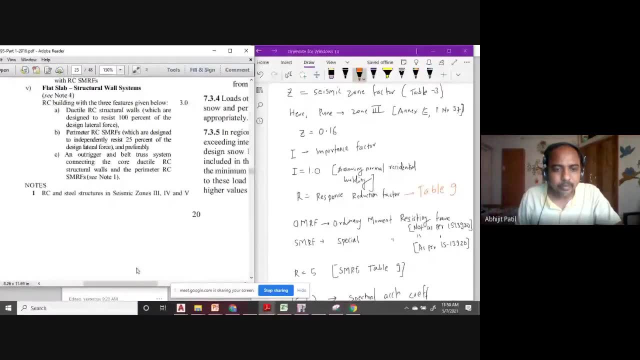 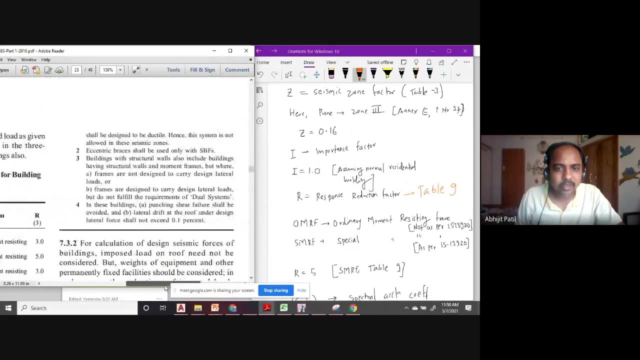 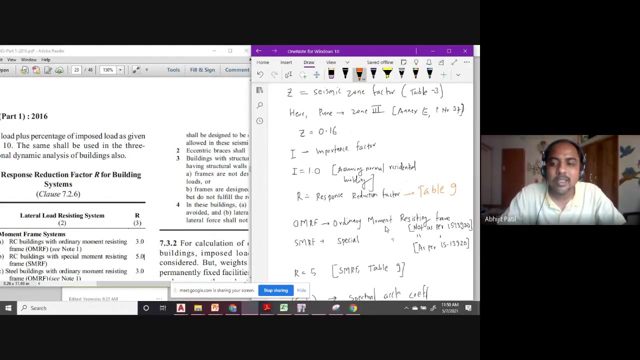 as five. so there is a huge difference. so what is this omrf here? not one is given below. okay, so the explanation was in old code. so omrf is nothing but uh, you have another code of is13920, so that is for ductility detailing. that means you have to follow some spatial detailing. 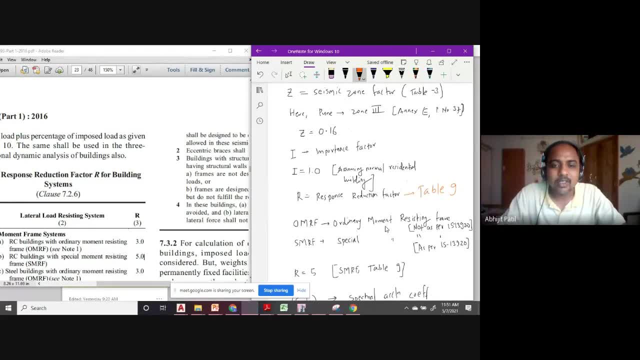 in rcc buildings so that the earthquake force effect of earthquake force is reduced with the help of ductility of the structure. so quickly i will explain the concept of ductility. imagine that you are standing here like this and somebody punches you. okay, i hope you can see my video also. so if somebody punches you and you stand rigid, 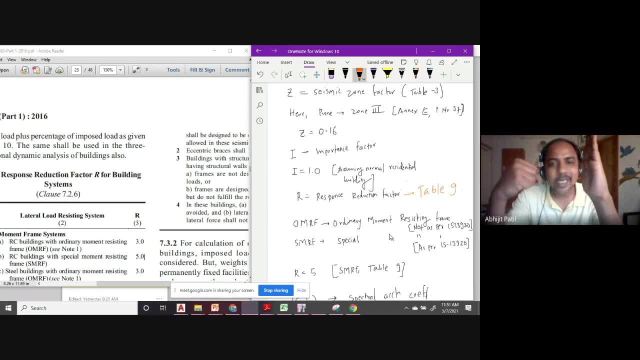 okay, you stand rigid. so what will happen? you will experience a lot of force, but if somebody is punching you like this and you just bend, okay, you just bend. what will happen? some amount of energy, which was, uh, in the form of punch, will get a lot of energy. 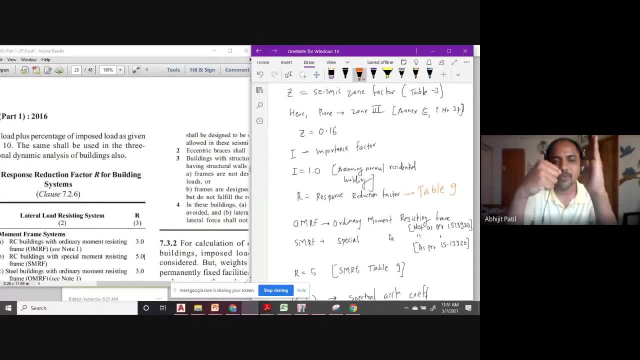 transferred in the deflection. okay, and the that means the amount of force experienced by you when you are flexible will be less as compared to when you are rigid. okay, so this is the concept of ductility. so in ductility we allow our structure to damage. okay. so if you are having some hundred percent energy, a few energy, almost 60, 70 percent energy, 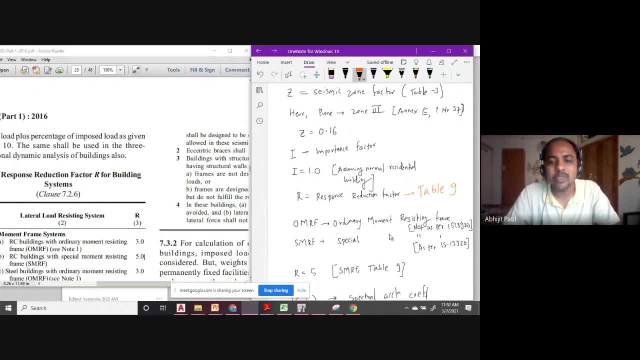 from the structure is transferred in the form of damage to the structure. now you may say how a structure can be damaged. in earthquake design philosophy we allow our structure to get damaged because practically it is impossible to design a structure as 100 earthquake proof structure. we never say earthquake proof, we say earthquake resistance structure. i hope you understand the if. 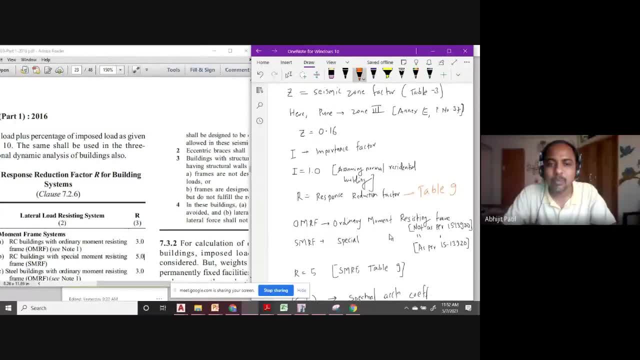 you are wearing watch. two types of watches, sorry: waterproof watch and water resistance watch. so waterproof means you can wear that watch and go for swimming, no problem. but water resistance means if you're wearing that watch and sometimes during rains it gets weighted. okay, that much it can bear. you cannot put that in. 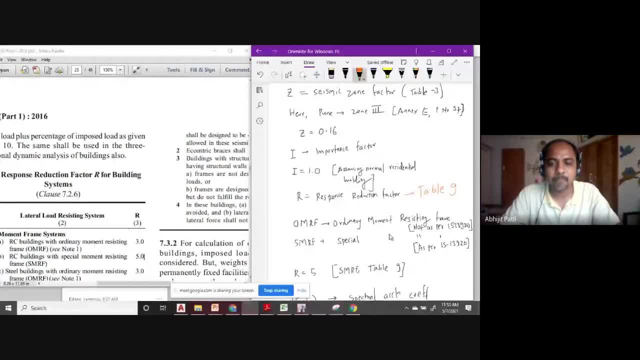 and deep in the water, it will stop working okay. so that is the difference in water resistance. similarly, water earthquake proof- we never do that, but earthquake resistance, yes, we allow some damage, but what this is. 13920 is. this tells us a few guidelines, okay, depending upon which we can. 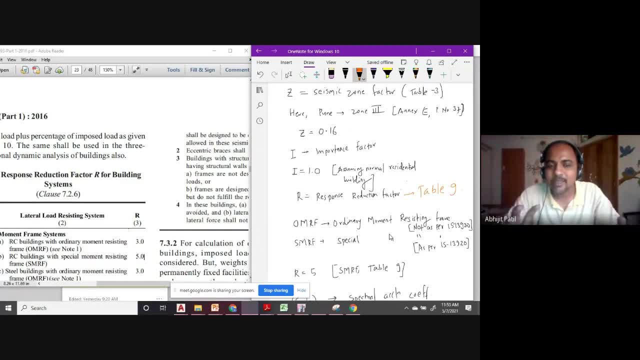 provide our reinforcement, detailing so that that damage is occurring at some particular locations, not at some critical locations. like the damage in beams can be allowed, because that will affect local floor, okay, but the damage in column is not allowed at all, because if you damage one column, the whole building can collapse you. 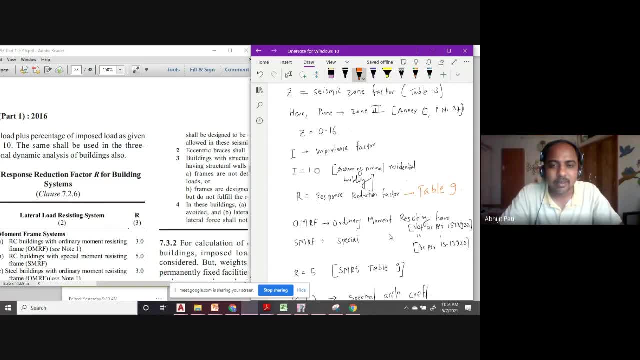 must have heard a few instances in near Borivali few years back that the ground it was something seven to eight storied building and there was, there were shops at the ground floor and while working some person bought the two, three shops in line and he wanted that space. 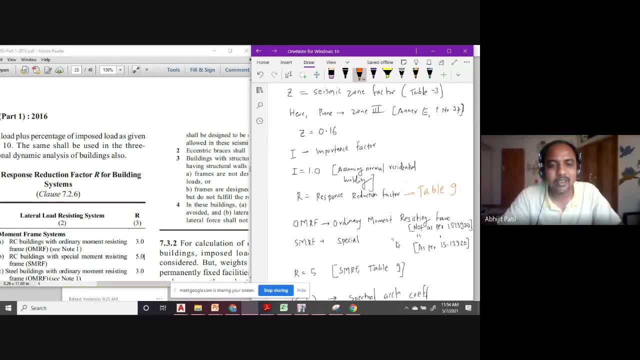 to be column free, so he is, without consulting any technical person. he started damaging column and one column was damaged. the whole building collapsed. it was an very unfortunate incident. so these things happen if only single column gets damaged. okay, so in one, three, nine to zero, we follow strong column. 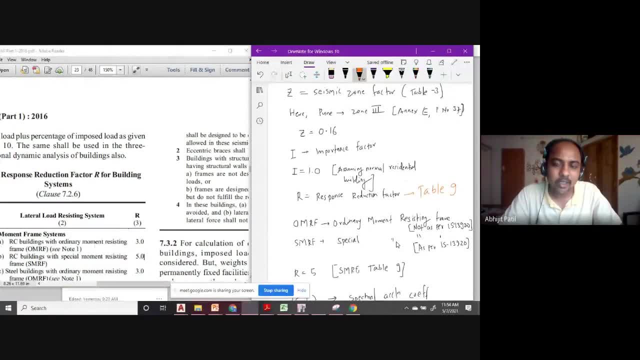 weak being philosophy, so we, our beams, can be weak whatever columns should be strong, so the detailing is done in that fashion. so if you follow those guidelines, then only this: we can take the advantage of ductility, we can divert the energy of earthquake to damage a few previous. 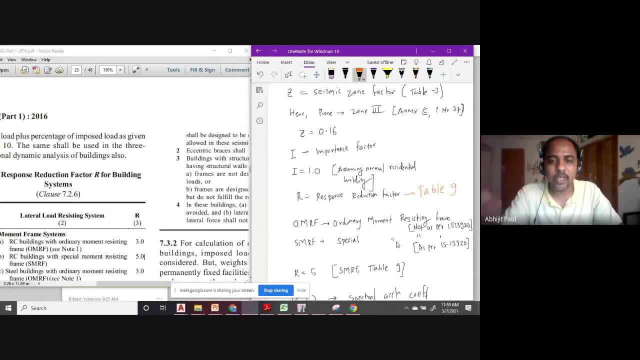 you identified, or few specific locations where we want our structure to get damaged. There is going to be a loss, So there should be a loss where the overall structure, even in wars- okay, this term is used, that of course it is beyond topic, but if you have seen movie Laksh, okay. so 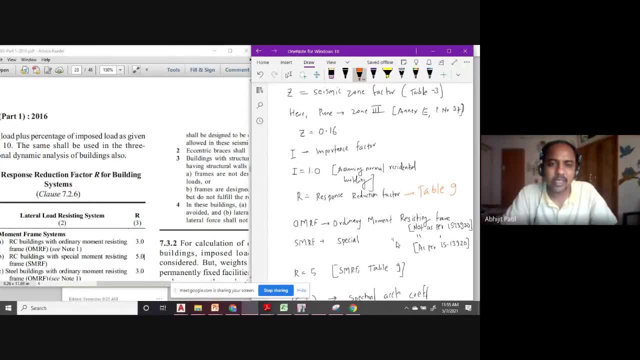 to this is a war tactic: to understand what ammunitions- ammunitions means chest, rastra, what ammunitions the opposition is having. so what they do, they just start firing blindly. okay, and when they respond, when the opposite party responds, they just record hearing the sound of the weapons fired. they just 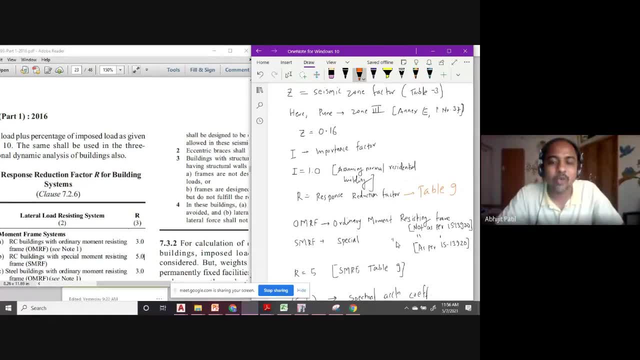 record how much weapons they are having a and which type of weapons they are having, what can be its range and accordingly they plan their. so they attack and they know beforehand that what damage can be done by them to us. okay, so like that we have to. there is a word. I am not getting that word. they 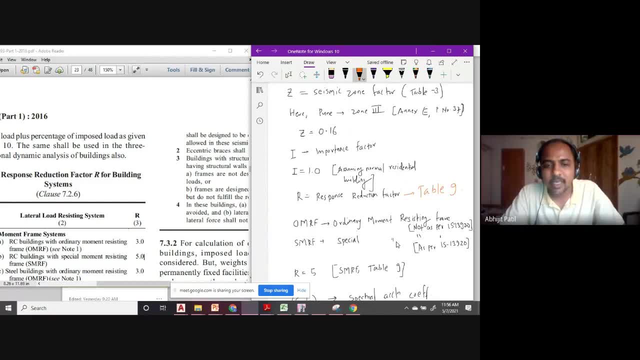 have to predict where the damage can be and we provide detailing in such a fashion that that damage is going to be announced in such a fashion that on the building is not damaged, it is standing still. the people inside the residing that building will remain safe or they can safely. 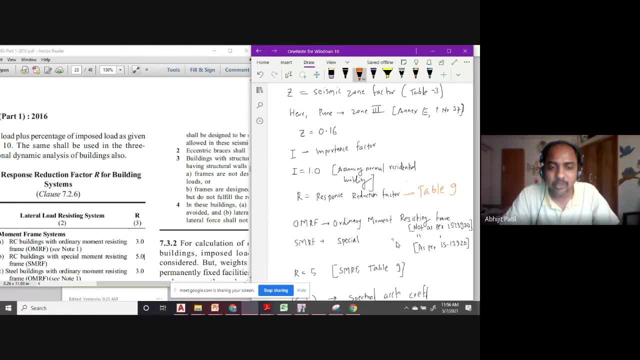 be evacuated during the earthquake. okay, So that is. this is the basic design philosophy of Earthquake Resident Design. so this r value will depend on whether you are following that guidelines 13920 or you are not following that guidelines. OMRF means you are not detailing as per IS 13920.. 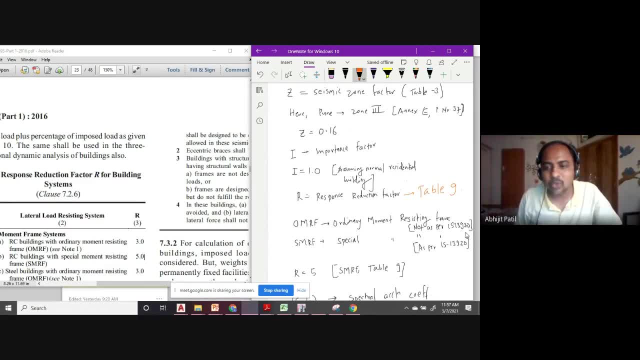 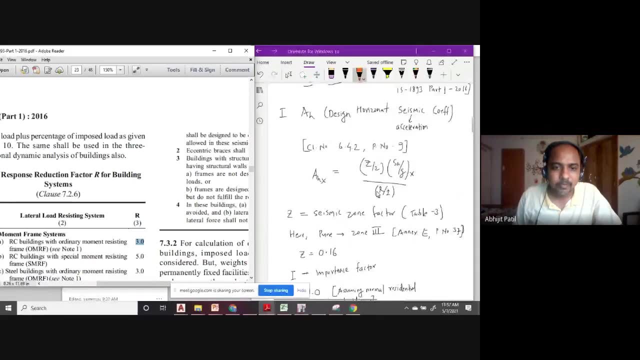 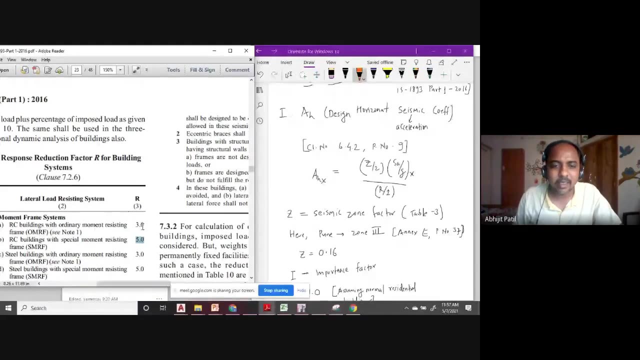 So that is the basic philosophy of earthquake resistant design: three, nine, two, zero. so code says: okay, you don't want to detail, okay, you take our value as three. so if you see here the R is in denominator, so higher the value, lower will be the force. okay, and if you are ready to detail like that: 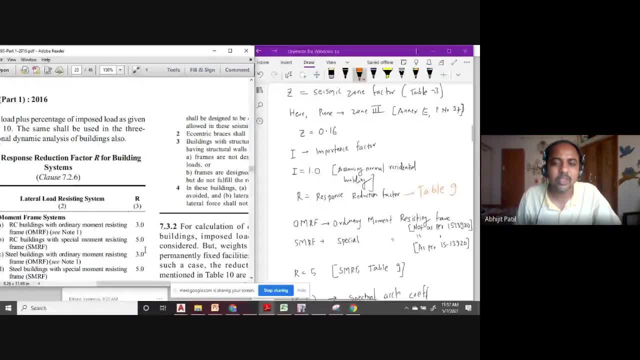 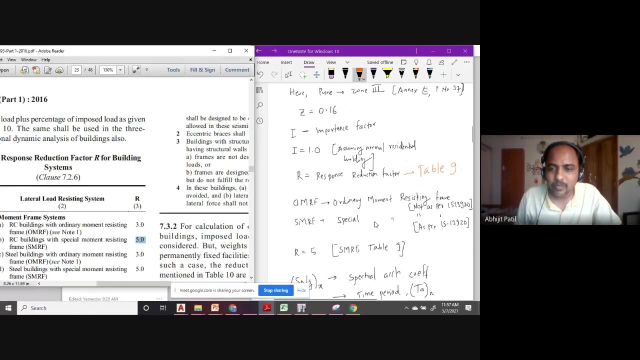 okay, then code says you can reduce your earthquake force by some more percentage and you can use R equal to five. okay, so I hope this clears the understanding of response reduction factor. so it is a reduction factor, okay. so if you are following again in numerical now, you will understood that. 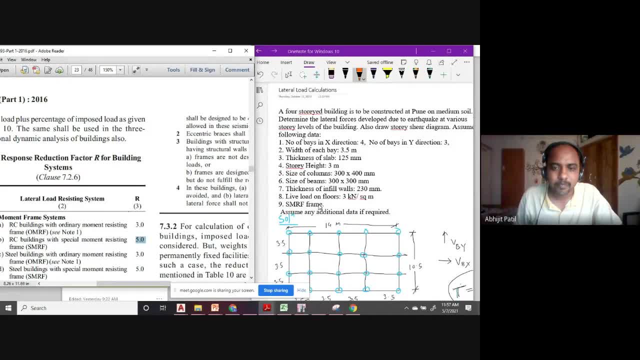 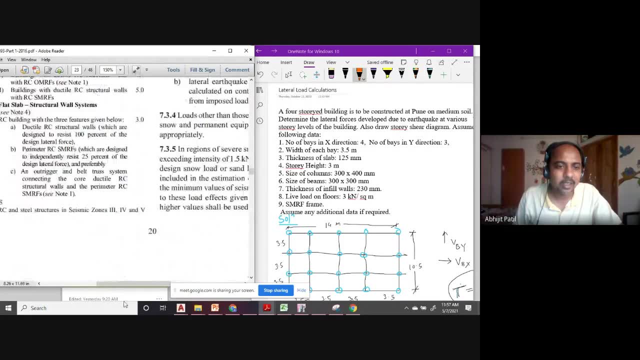 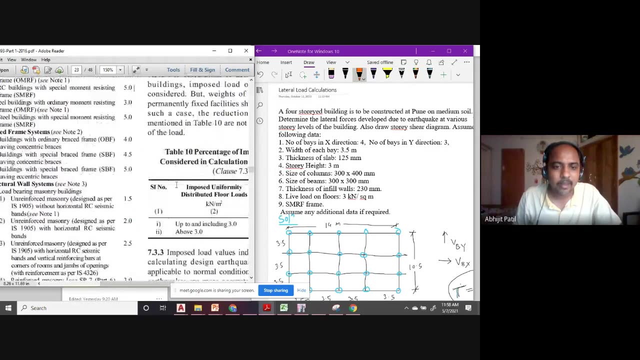 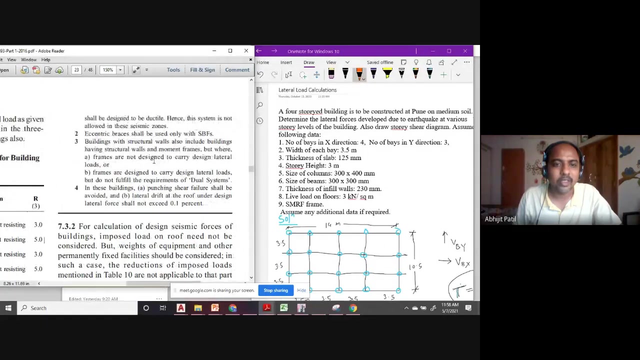 why this information is given. SMRF frame. okay, so, although it was a of choice earlier, but now, this note one says for RCC and steel structures in seismic zones three, four and five shall be designed to be ductile. hence this system is not allowed in these seismic zones. so 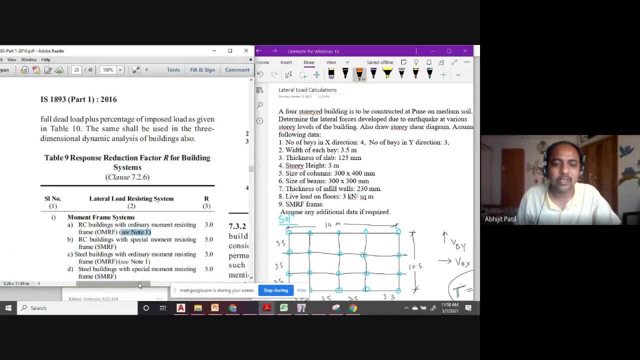 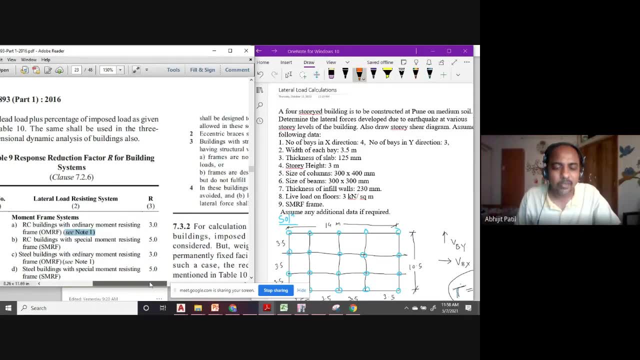 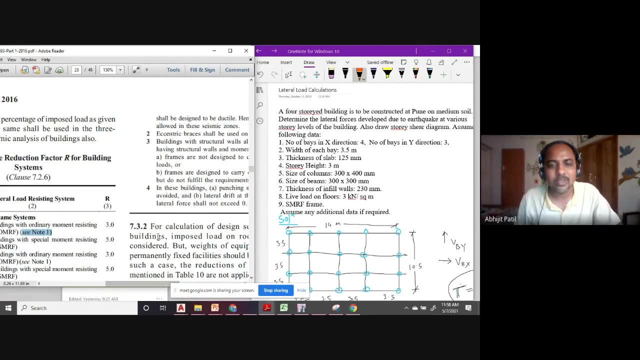 this system is this: note one: OMRF. it's not allowed in zone three, four and five. so earlier this clause was not there, it was compulsory for only zone five. but now, if your building is in Pune, Mumbai, which come under zone three, you have to compulsorily provide is one, three, nine, two zero provisions and our value will. 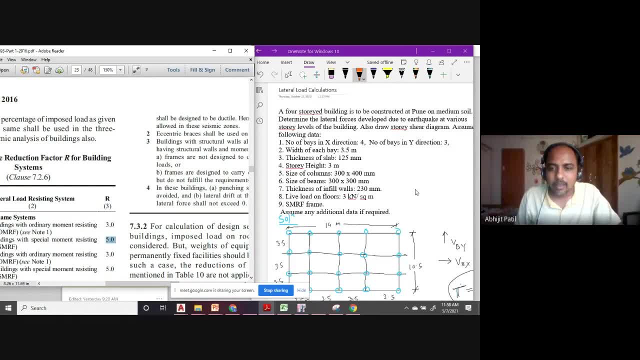 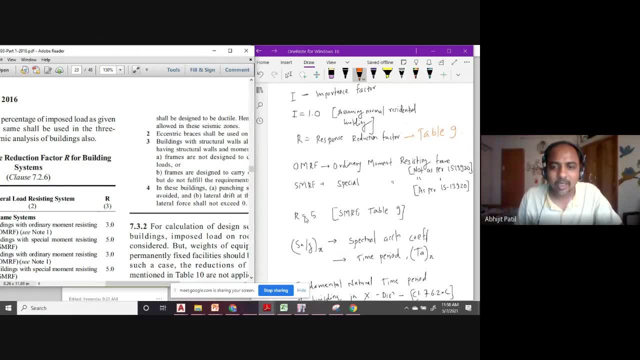 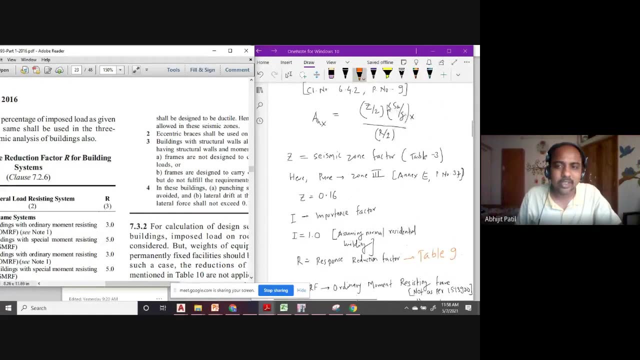 be five in that case. okay, so R we will take as five, because this is SMRF frame, R is equal to five. next thing: SA by G. okay, so it is never expressed as SA separately and G separately, it is always SA by G. so G here is acceleration due to gravity and 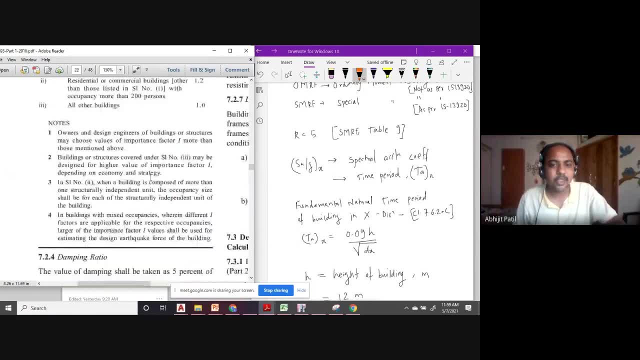 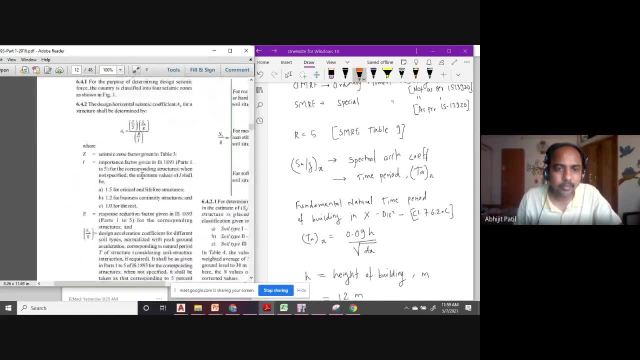 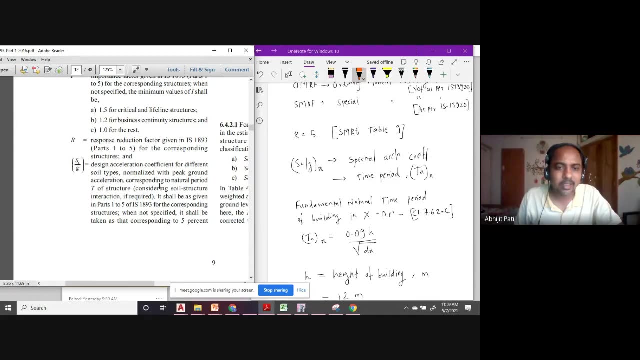 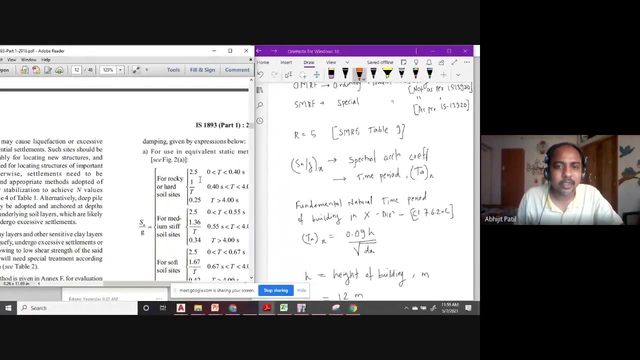 SA. coming back to page number nine, I guess next. so it is design acceleration coefficient for different soil types, normalized with peak ground acceleration corresponding to natural spirit T of structure. okay, and you can find that using this expression. so they have given some expression here for SA by G and 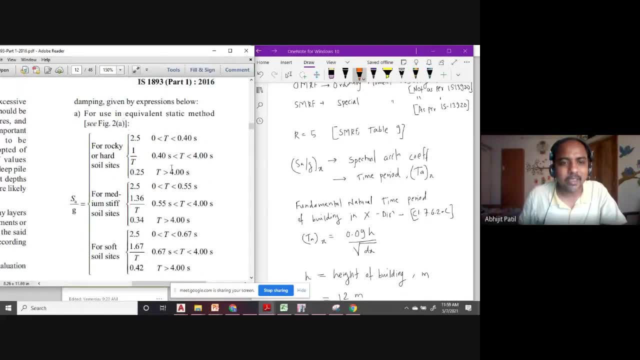 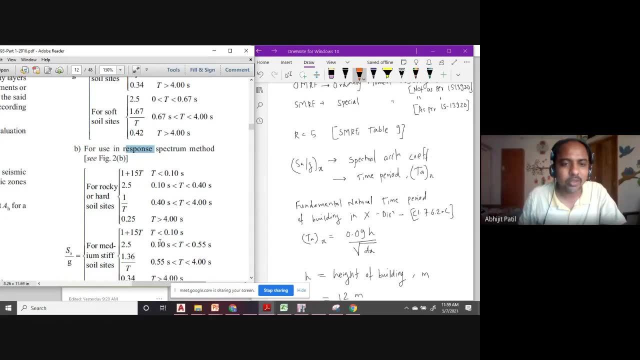 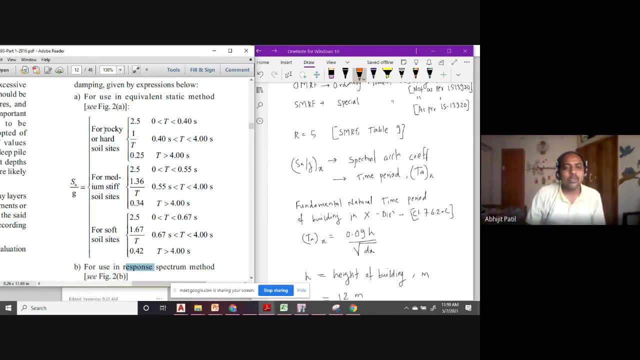 So for using equine static method, we have to use this A, and for using dynamic method, which is called a response spectrum method. so this, for time being, don't go into this. so this much is sufficient. so if you see here, it depends on whether your soil is hard rock. 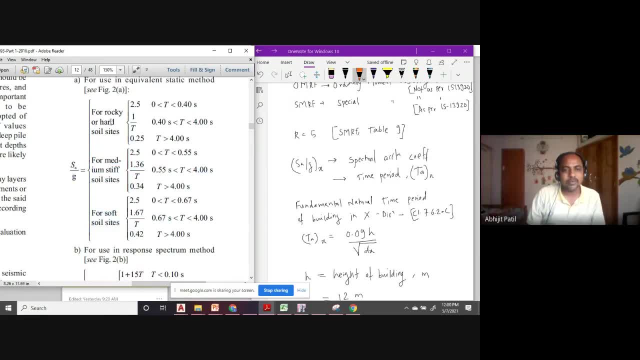 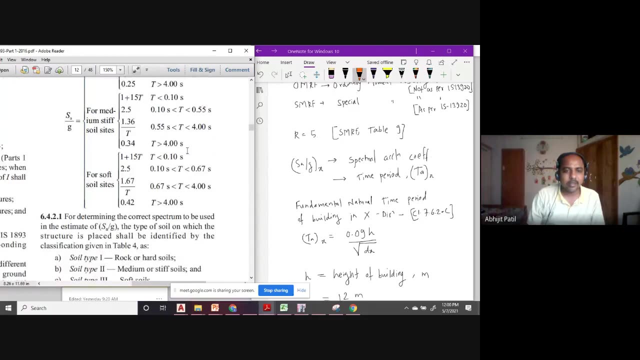 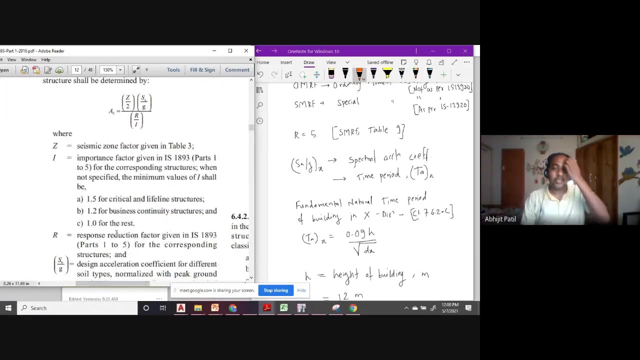 or medium steep soil or soft soil. okay, so this SA by G formula depends on these three type of foundation strata or soil and the time period of the building. okay, So time period of the building. we had read that the time period is to be calculated using 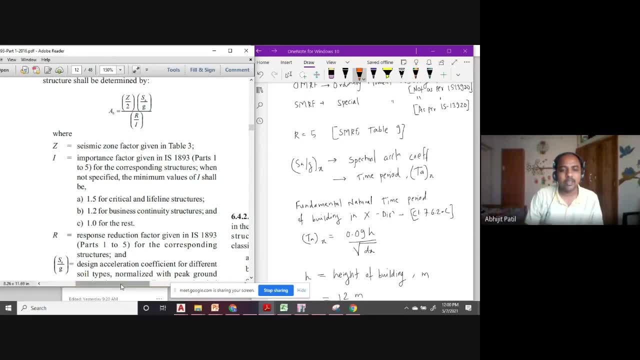 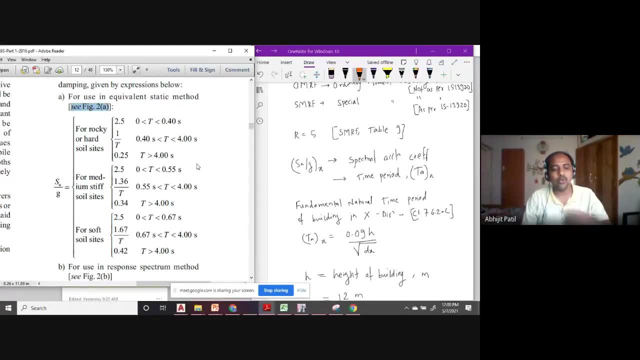 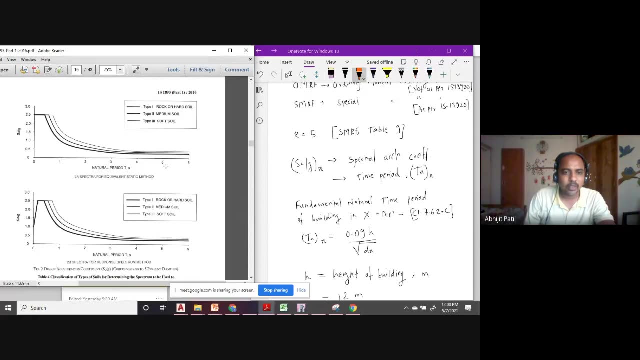 some clause, so we will go back to that clause. but again, this is also given in figure 2A. so if you don't want to do that, If you don't want to use formula, there is a readymade graph, given figure 2A, this one. 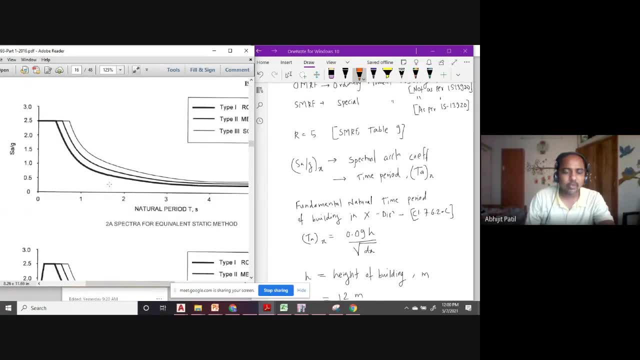 this is your figure 2A, so if your time period is one second. so there are these three graphs: one, two, three. okay, so type one is your hard soil, type two is medium soil and type three is soft soil. so we are having medium soil in the numerical, so we will use this middle. 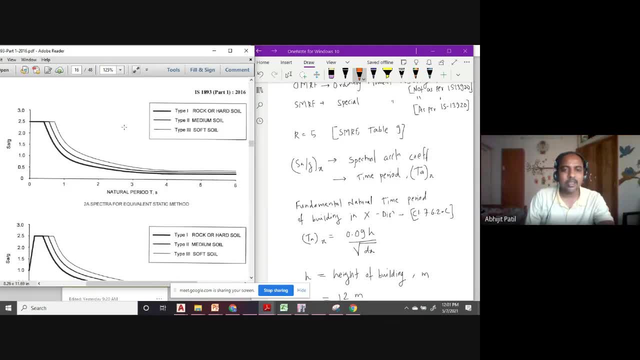 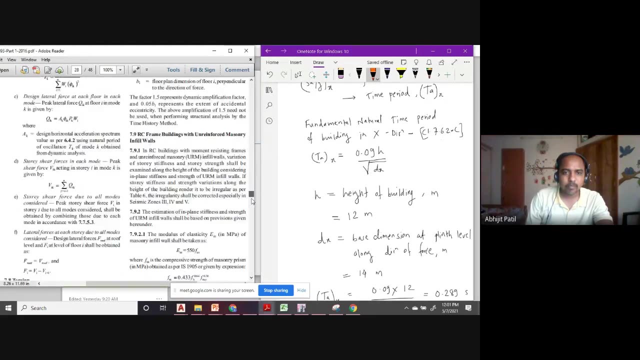 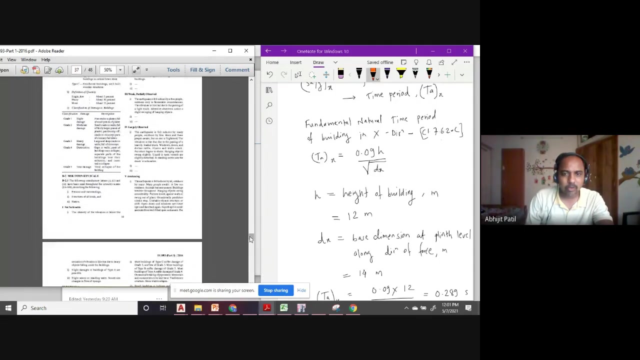 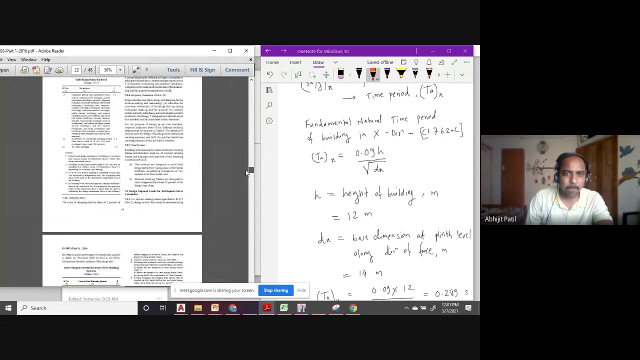 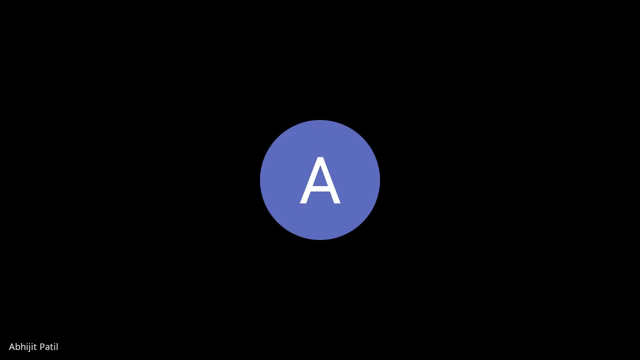 graph. okay, Now, the next thing remaining is time period. so here I have mentioned clause number 762, so we will go to that clause. Okay, I have gone too far. Okay, Okay, Okay, Okay. Six point four, seven, seven, six, two. 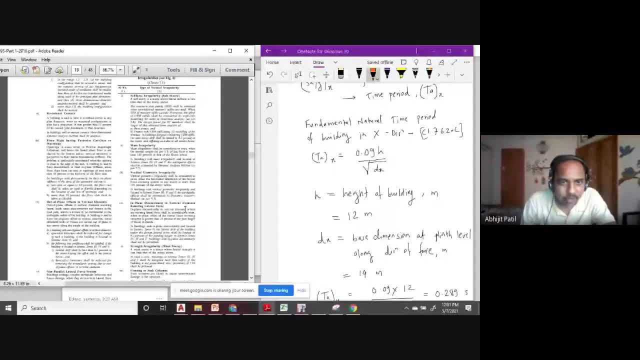 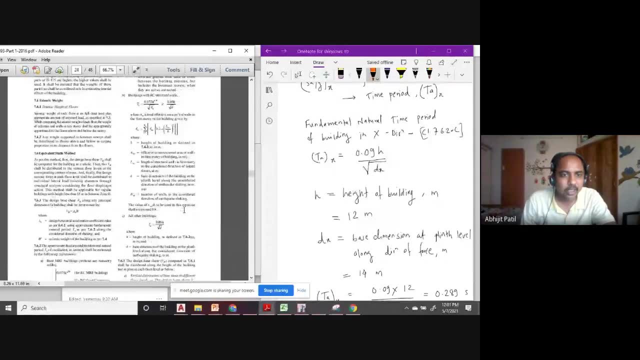 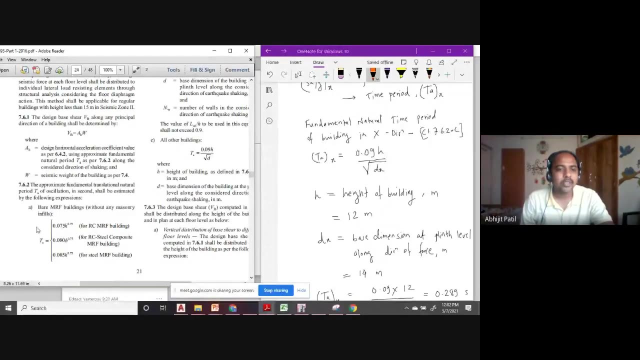 Yes, seven, six, two. okay, so you have again different, different formulas given you over time. So I have added a clause number here. okay, how many times must I have added? you know, this should be one here. so bare MRF, that is bare movement. resisting frame, that means without any. 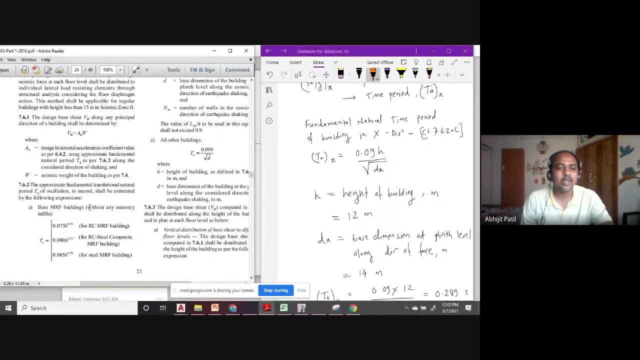 masonry influence. so this, the commercial buildings. if you see the IT offices or corporate offices, what do they have? they have just columns and beams and slabs and later on, using partition, lightweight partitions, they just divide the floor as per their convenience. so those buildings will come under this, but residential. 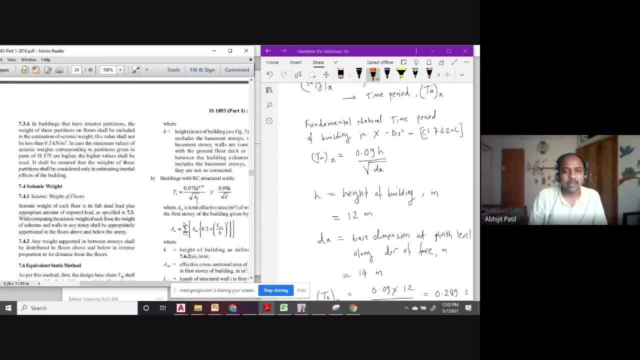 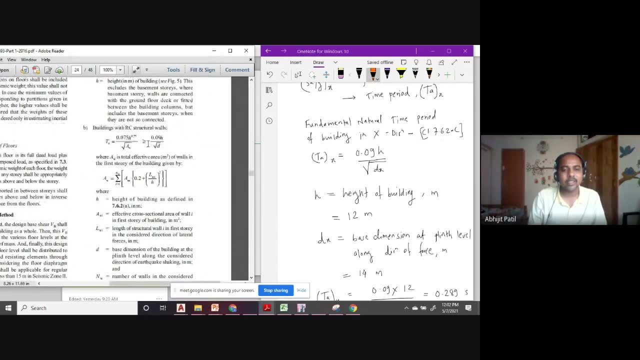 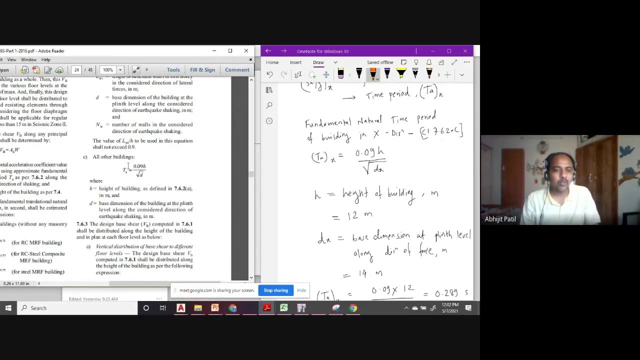 building will come under buildings with here or other buildings. so this is building with RSI structure walls. that means that my one buildings and here for all other buildings, so our building will fall under this category. what is the formula for time period? 0.09 h divided. 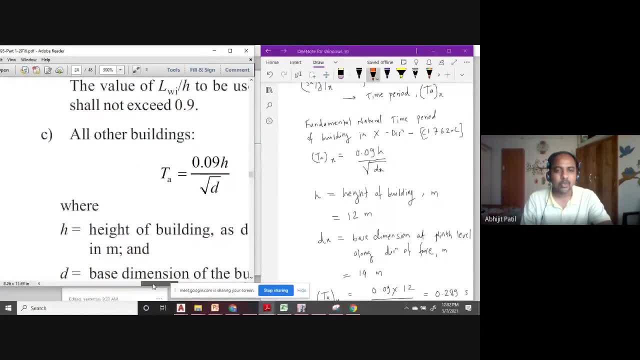 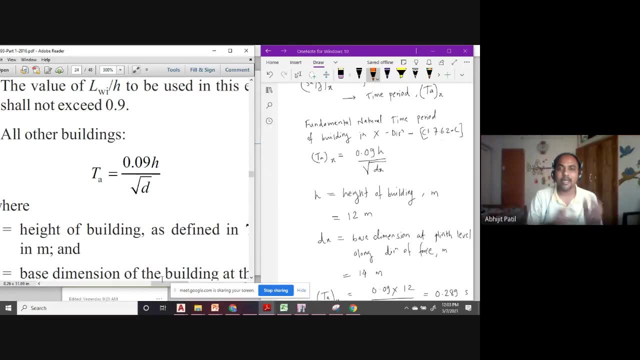 by square root of d. okay, so instead of we have seen that the time period theoretically is calculated as 2 pi and the M by K, but practically you can calculate M but calculate K. it is very difficult for large buildings. so code has given some formula based on experimental. 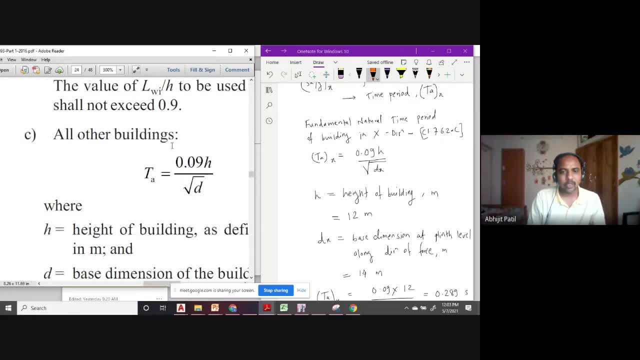 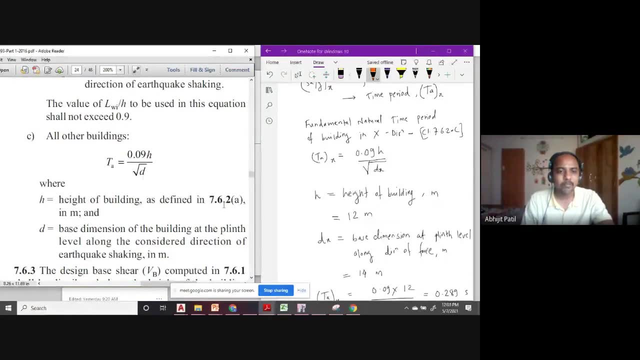 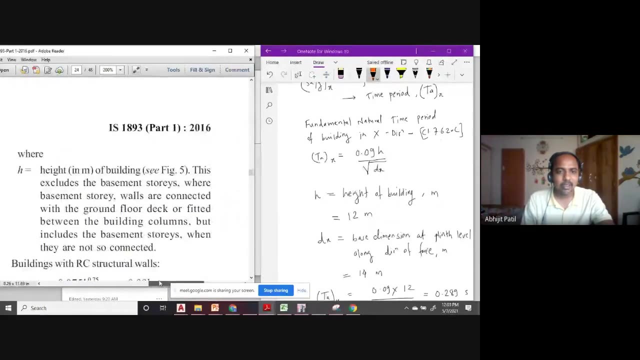 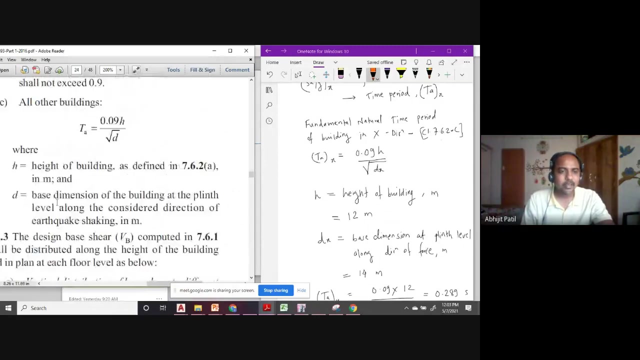 results okay. so this is more appropriate because this is based on experimental results. so H here small, H here is the height of the building as defined in 7, 6 to a. so 7, 6 to a is here. so height is excluding basement story. okay, and D is: 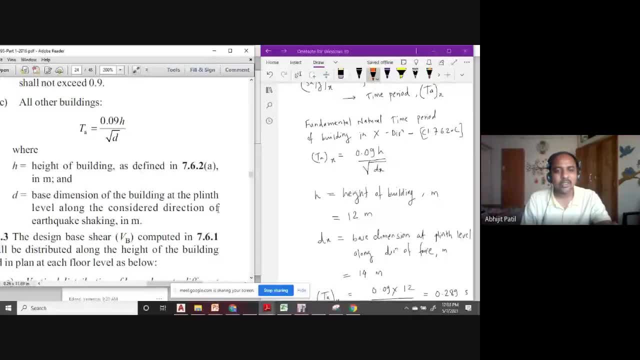 the base dimension of the building at Flint level along the considered direction of earthquake shaking. that means D will be DX or dy, depending upon time period in which direction you are calculating your time period. okay, so, having understood this, here I have written fundamental natural time period of building in X direction, because we have to calculate in what directions. 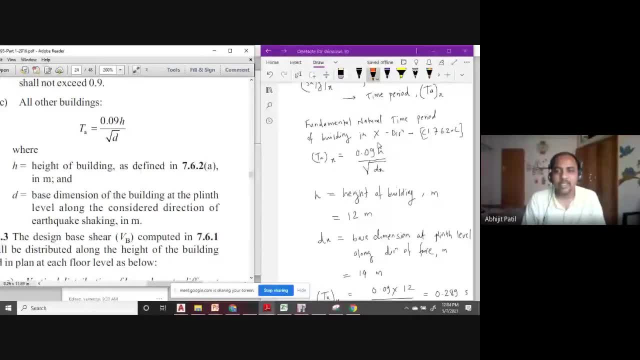 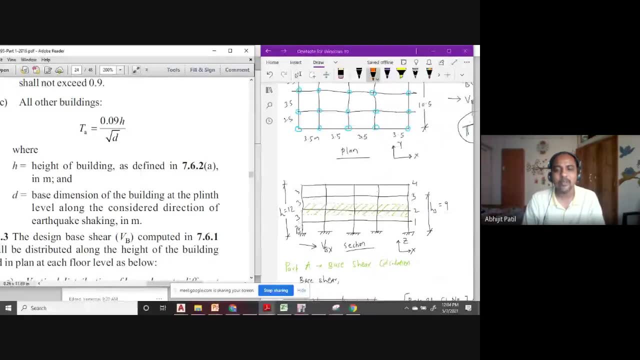 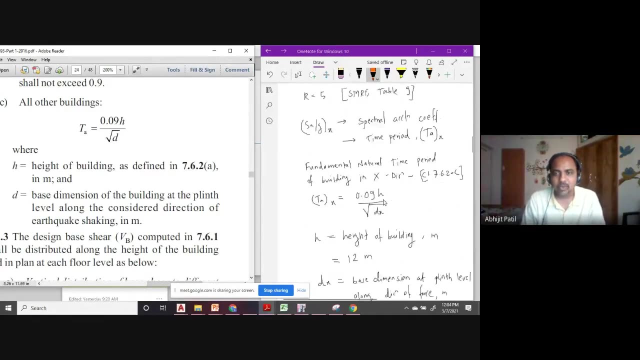 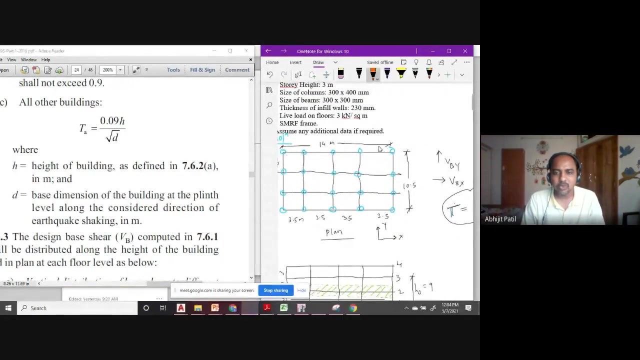 separately. so point zero nine H upon under root DX. so H is the height of the building we had calculated here for storage. so three meter each story. it is 12 meter. okay, so H is 12 meter and this is base dimension DX along X direction. so it is 14 meter. here in X direction, this 14 meter. so just put those values. 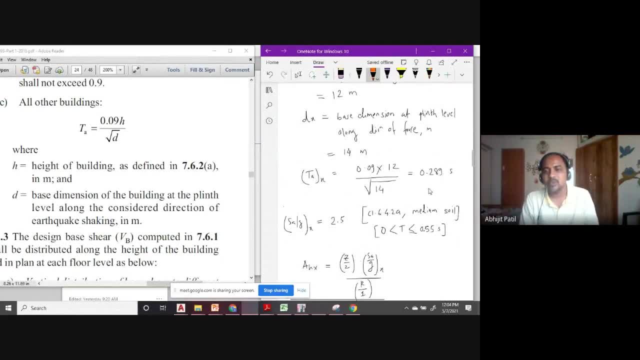 and calculate. so it is just save the time. I have already solve that problem. so point two: eight, nine seconds she's time period, and then put that in this formula. so for sa by g value for time period t less than 0.55 seconds for medium soil is directly 2.5. okay, so that has come from that formula which we had seen. 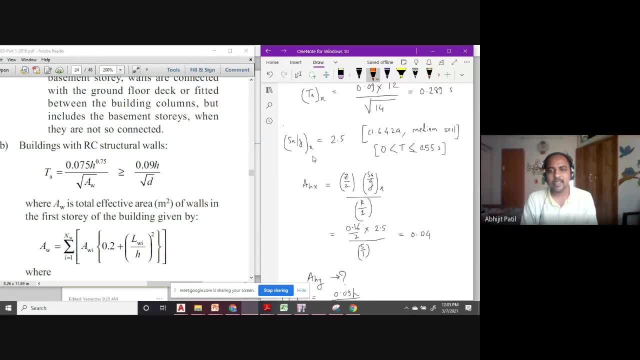 so this is all. data is with us. so ahx is calculated. just put the value of z, 0.16 sa by g is 2.5, r is 5, i is 1 and it will be 0.04. so on similar lines you can calculate. 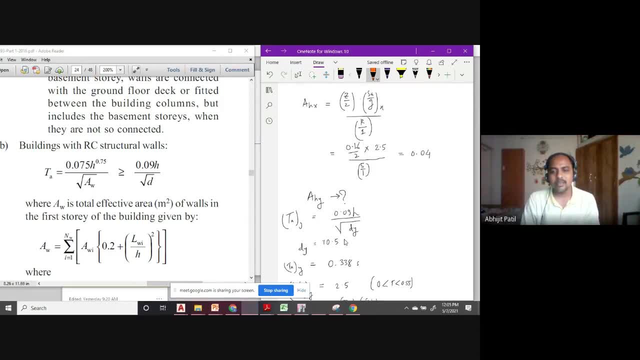 ahy. what is the difference? this time period will be different. okay, so dy, here is 0.5, the time period is 0.338 seconds, but still it will fall under the 0 to 0.55 category. so it is 2.5. 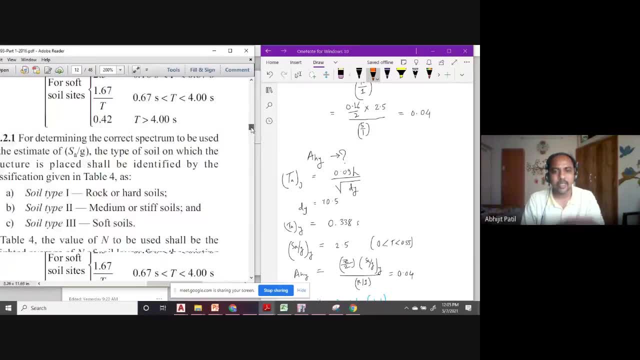 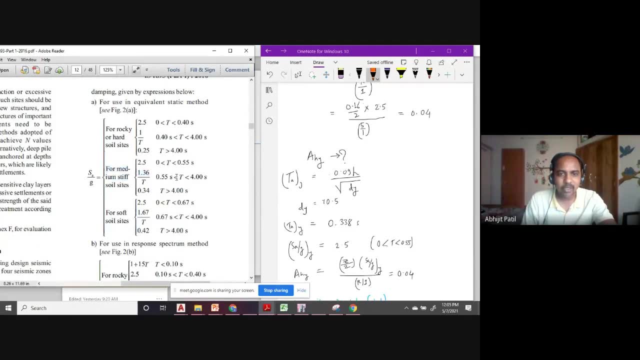 i will again repeat once you get the time period. just go to the graph or go to this here. and for medium soil the time period is between 0 to 0.67 seconds. sorry, we are here 0.55 seconds for uh, both x and y direction. so the value of sa by g is 2.5, obviously. so all the value. 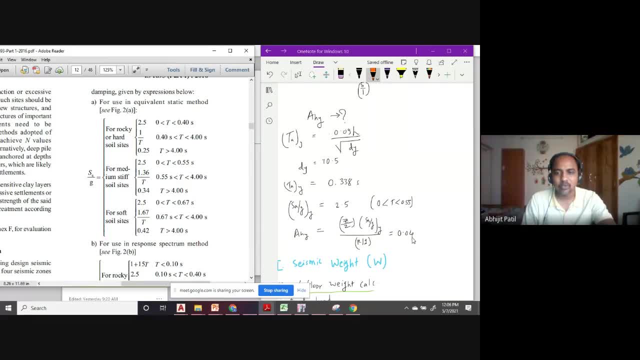 other values are same. so ahy is 1.55, also point zero four. okay, so this is one part: calculation of the coefficient. both the coefficients in this case are same: point zero four. now second part is how to calculate the seismic width. okay, so I will take just pause here, if you have. 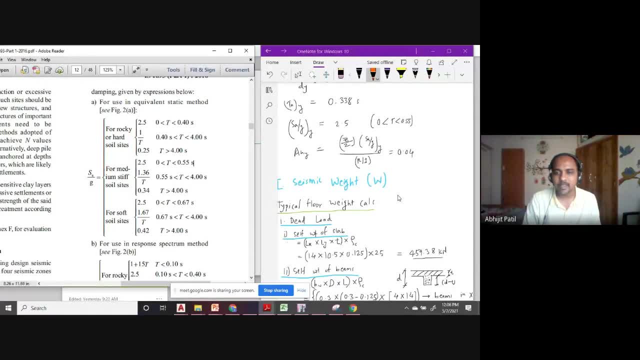 any doubt related to the first part, calculation of horizontal seismic coefficient, please ask. okay. Z depends on location. I depends on importance of the building. R depends on whether you are following one through nine to zero or not, say by G depends on time period. that depends on the height of the building and the dimension. the. 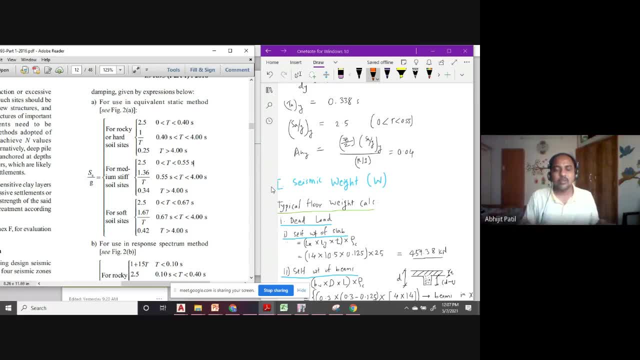 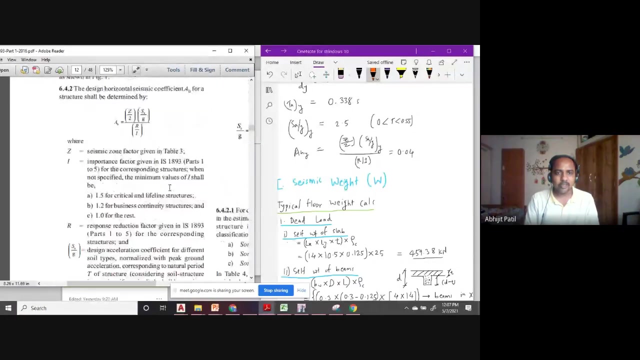 direction of the force which we are calculating. okay, so we have to just get the data and put the appropriate values in the formula now. second thing is seismic weight. so again we will go back to that basic formula, VB into a hitch. nothing that was on the basic formula. 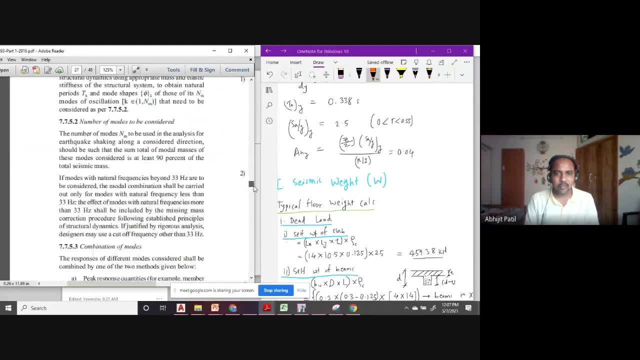 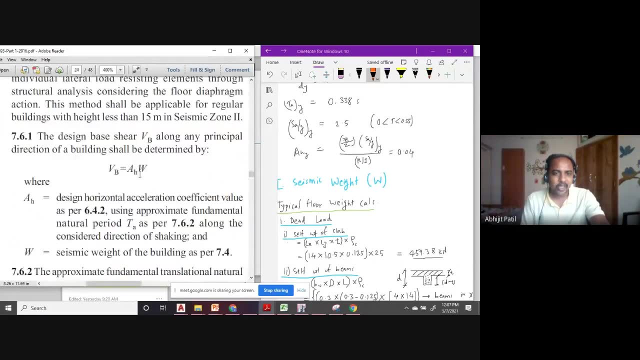 So again, we will go back to that basic formula: VB into AH. I think that was on. a second thing is seismic weight. so again we will go back to that basic formula: VB into AH. I think that was on page number 21. yes, so here will be. is equal to age to age. we are finished w. 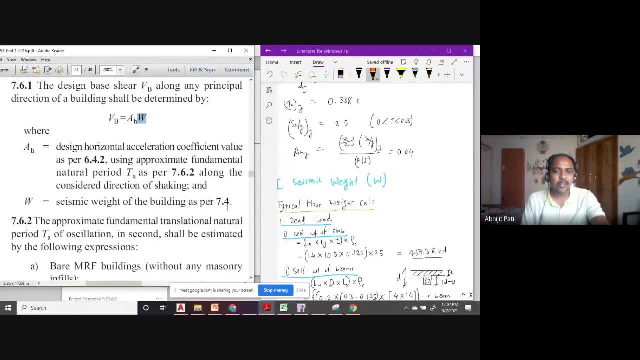 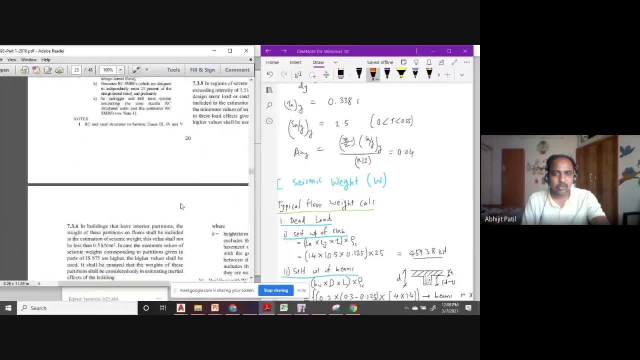 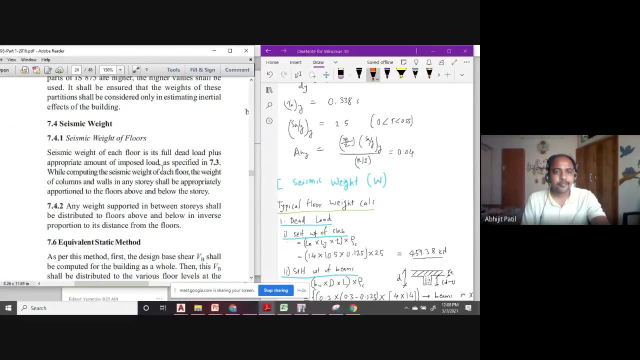 part is seismic weight of the building as per clause 7.4. so we have to go to clause 7.4. yes, seismic weight of flows. seismic weight of each floor is its full load. okay, full load plus appropriate amount of imposed load as specified in 7.3. so imposed load here. 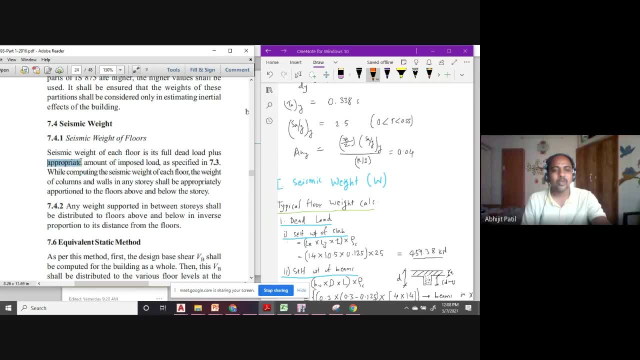 means live load. appropriate amount means we have to consider some percentage, and that guideline is given in 7.3, while computing the seismic weight of each floor. okay, at floor level we will have slabs, beams. okay, but what about walls and columns? so for that this next line. 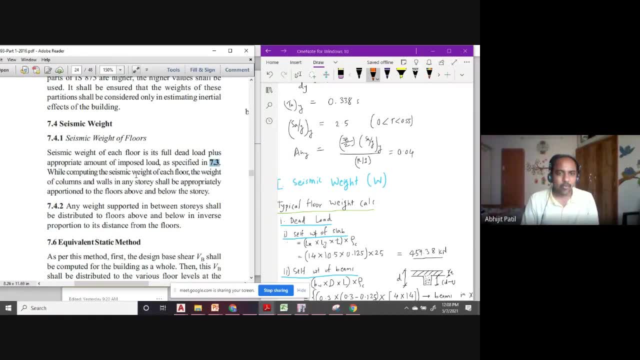 is there. while computing seismic weight of each floor, the weight of columns and walls in any story shall be appropriately apportioned to the floor, to the floors above and below the story. so appropriately here means 50% above and 50% below. we can distribute the weight of the columns and the walls okay, any. 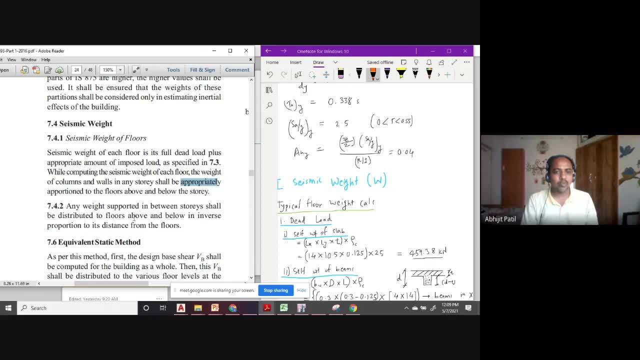 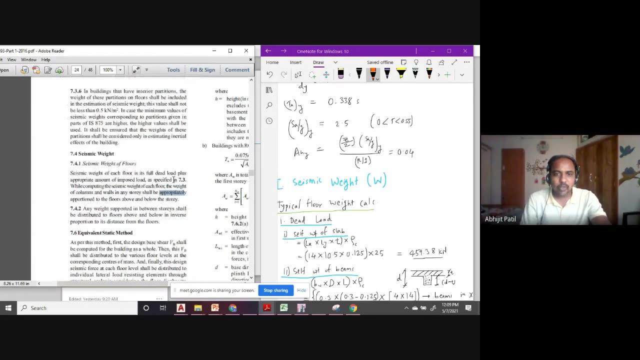 weight supported in between stories shall be distributed to floors above and below in inverse proportion to its distance from the floor. okay, so same thing, since it is symmetric vertically, 50% of one and 50% below. so full dead load we have to calculate and some part of lie load. so 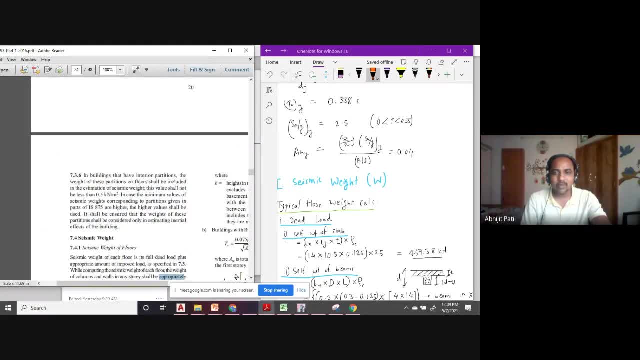 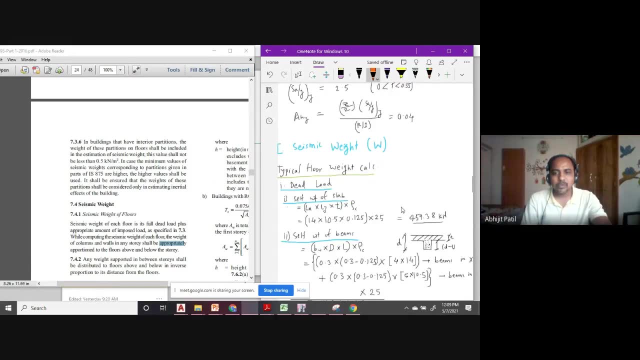 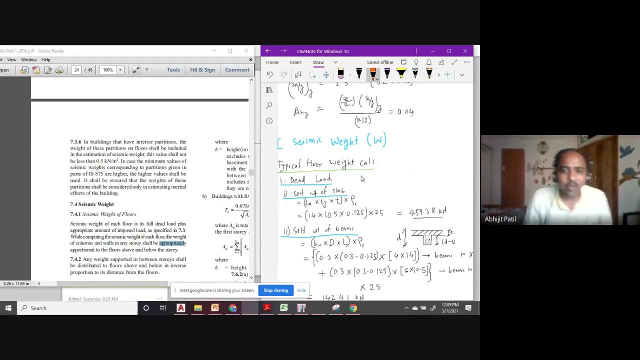 what is that? for that we have to go to clause number 7.3, but before that we will calculate the whole dead load. so for that we will consider a typical floor. okay, because it is repetitive flow, so we will calculate for one floor. so self rate of slab in this case. I will just maximize this now. 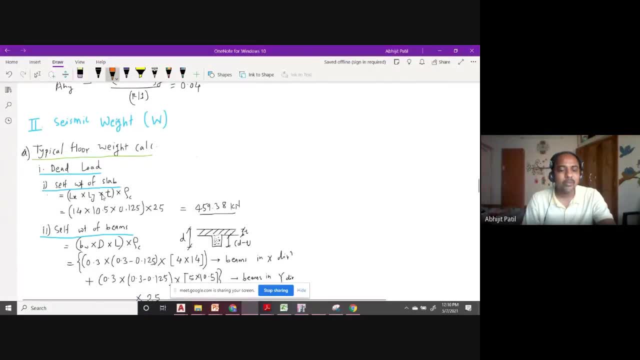 and we. so self rate of slab will be just length of the slab in x direction, in line direction, and thickness of the slab multiplied by the density of concrete. so we, or the total length is 14 meter, total width is 10.5 meter in data. it is given that the thickness of the slab is point one, two. 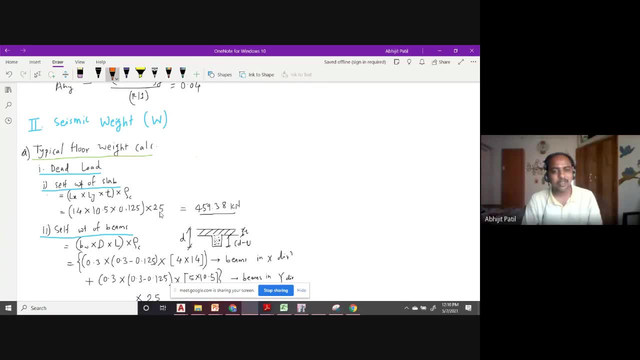 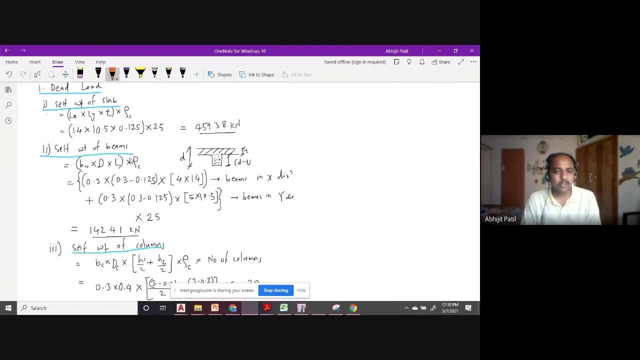 five. just multiply, you get the volume. multiply this with density, so this is the total weight of the slam for a single floor, typical single floor. okay then, uh, self-fit of beams. again we have to find the volume. so width of the beam, bw, depth of the beam and length of the beam. so here there are. 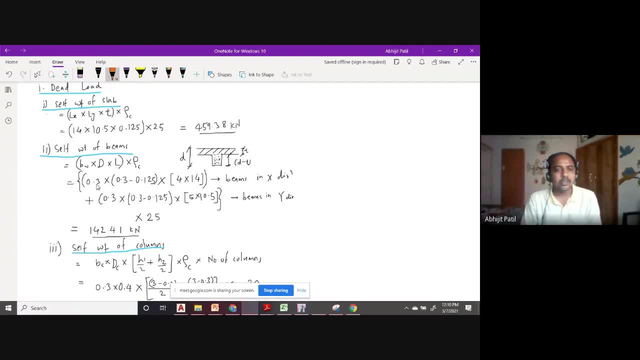 beams in x direction and in y direction. so width of the beam- 0.3- is constant. so i will take that out. depth of the beam: here you see this figure. so this is actually total depth from top to bottom. so out of that thickness of the slab we have already considered 0.125, so i will minus that. i will just 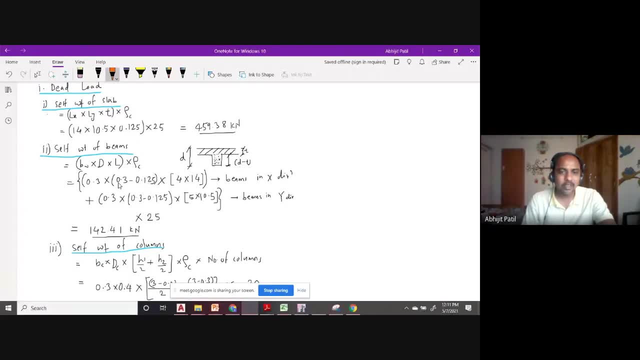 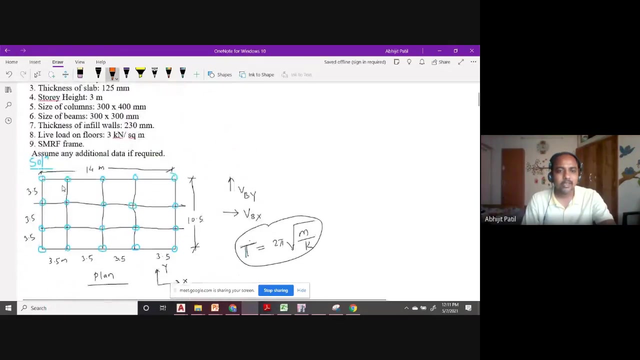 need d minus t. so this is 0.3 for and this is 0.125. the thickness of the slab is subtracted. okay, and multiply this with length of the beam. so length of the beam, how we are going to calculate. in x direction, next direction, you have, from here to here, total 14 meter length, and how many such 14 meters beams? 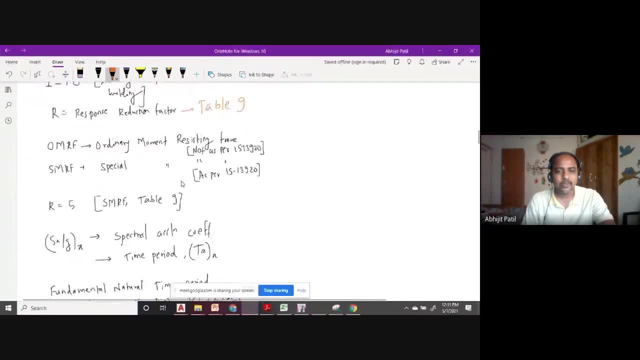 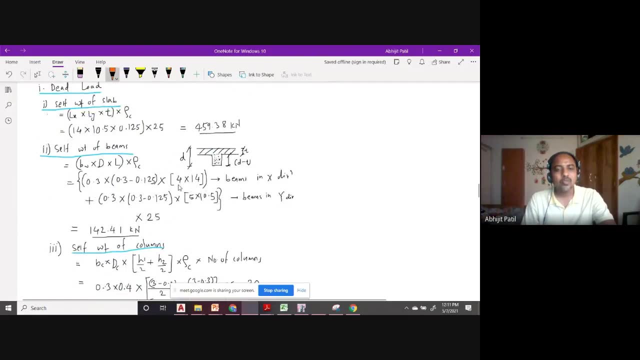 are there one, two, three, four. so that is why i have written yes. so i have written just a second here. that's four, four times 14.. so this is the total length of the beam and this is cross section of the beam. so we have got. 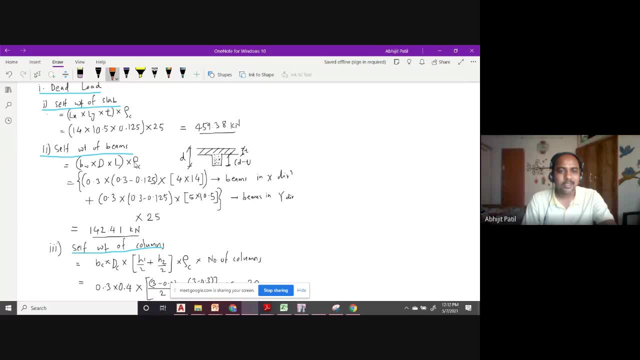 volume. okay, this density i have commonly written outside here, so this was in x direction. so remember, we calculate a h x and a h y separately. but weight is not direction. specific weight is acting vertically downwards, so we have to calculate the total weight. okay, so this is a general mistake. 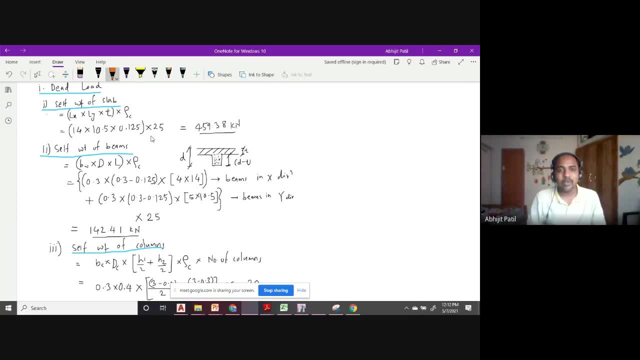 or mis concept. we are calculating the force in x direction. we have to consider only x direction of the. no, that is not the case. weight is not direction specific. it is acting vertically downward, so we have to consider the total weight. okay, so this was. this is just for calculation. i have 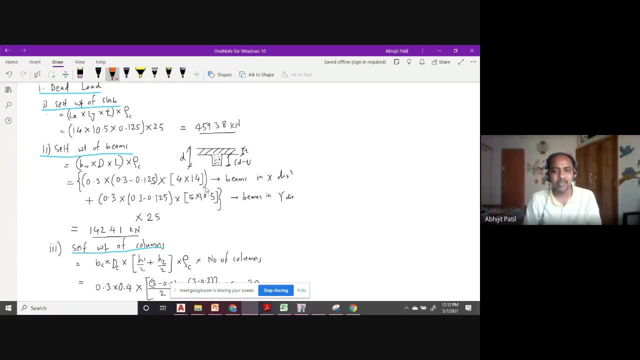 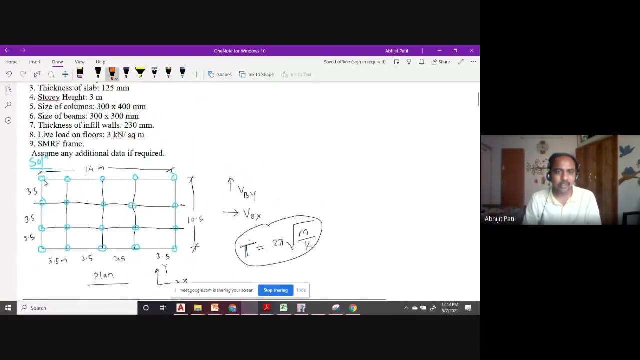 separated: x direction separately and y direction separately. so in y direction again, same 0.3 multiplied by this thickness. okay, and we have to calculate the total length of the beam in y direction. so length here is 10.5 meter and there are one, two, three, four, five. so 10.5 multiplied by 5 is the total length of the beam. 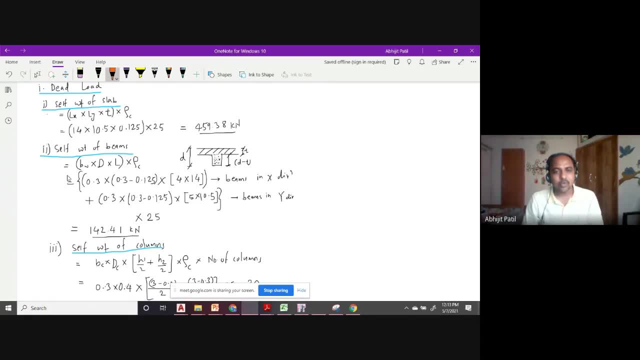 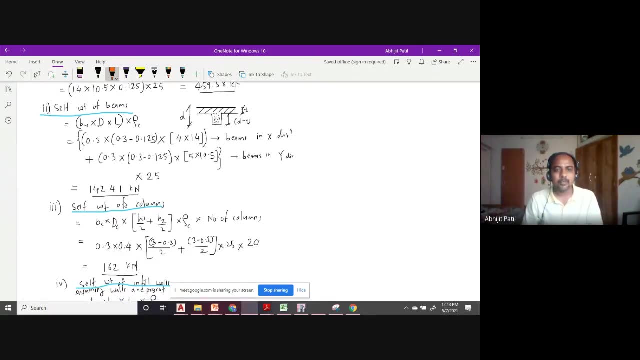 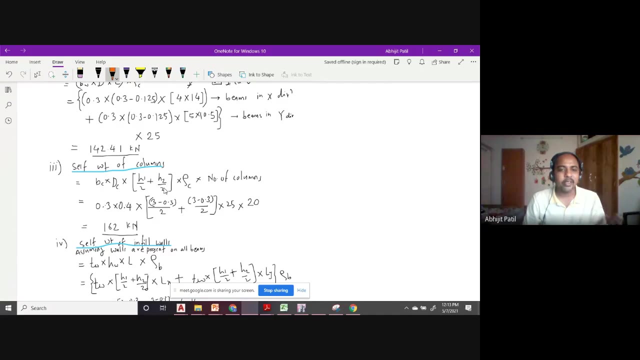 coming back here, yes, so 5 times 10.5. so if you do this, just multiplication, subtraction, addition, this is the total weight of the beam. out the beam, okay, then self weight of columns. so columns again. we have to find the volume okay and multiply that with uh density and into number of columns. 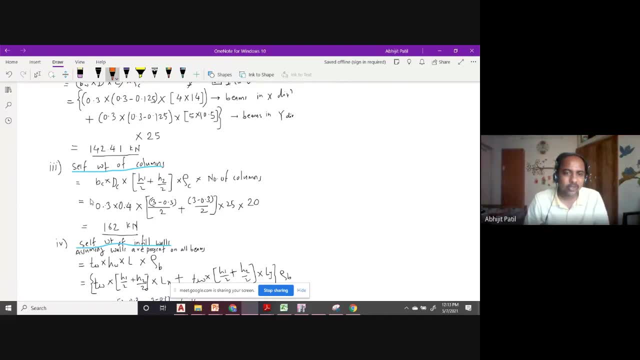 okay, so 0.3 by 0.4 is the dimension of the column, cross section dimension. now here, h1 by 2 plus h2 by 2, that means the height: 50 height from below, 50 height from above. now go to cross section here. 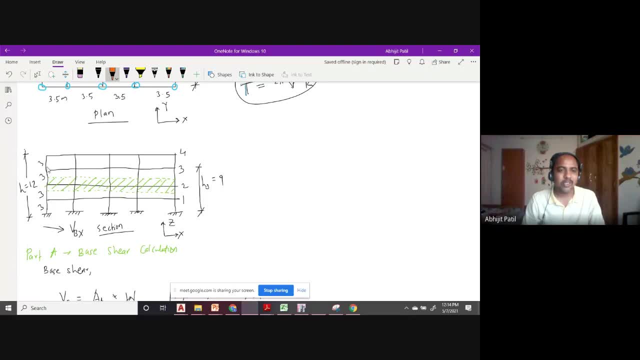 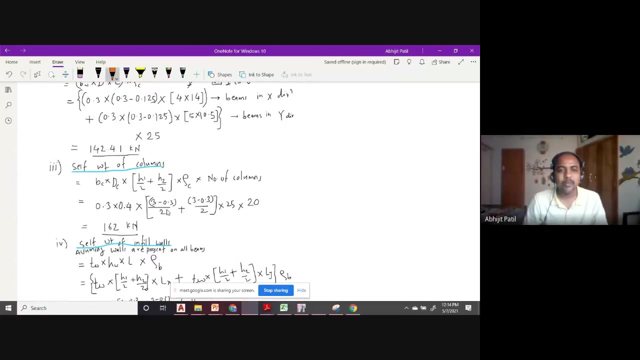 okay. so this is uh, obviously normally this will be the case that floor heights are same, so 50 from below, 50 from above. so that is why i have written h1 by 2, h2 by 2. okay so, and again, this h1, it's clear height, because beam depth we have already considered. so we will. 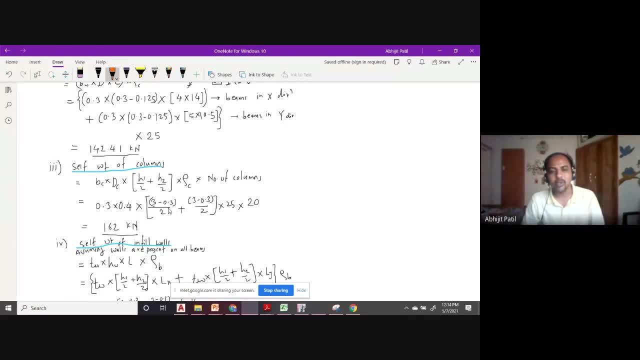 minus that from the total height of the column. okay, and then consider this by 2 by 2 and number of columns. okay, so this 20 is number of columns, so just count the number of. obviously this is 5 by 4, bay, sorry, uh, 3 by 4. that means number of base plus 1 will be your column number of columns. 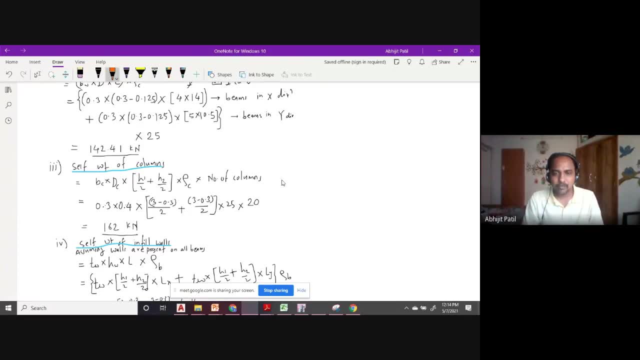 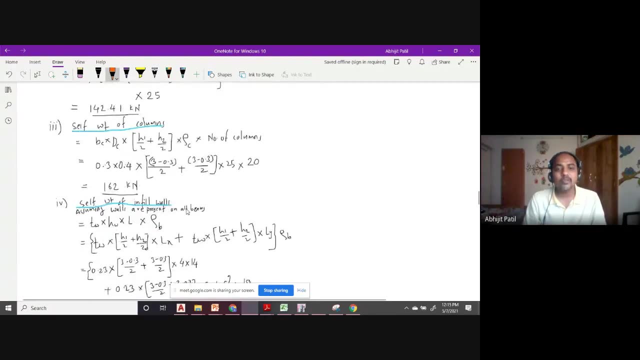 uh, grids. okay, so these are total 20.. so this is the total weight of column, then self weight of infill walls. that means average walls. so no data is given. so we have assumed that walls are present on all the beams. okay, sometimes they will mention that only outer periphery walls are present. 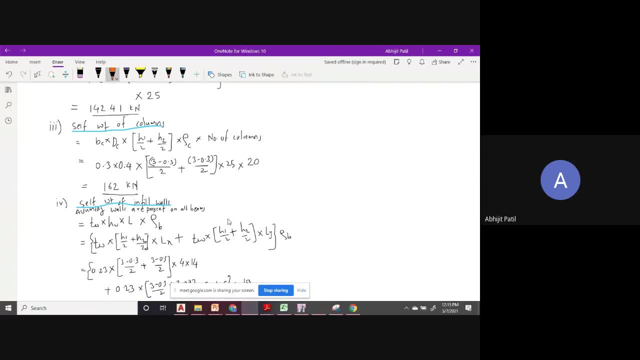 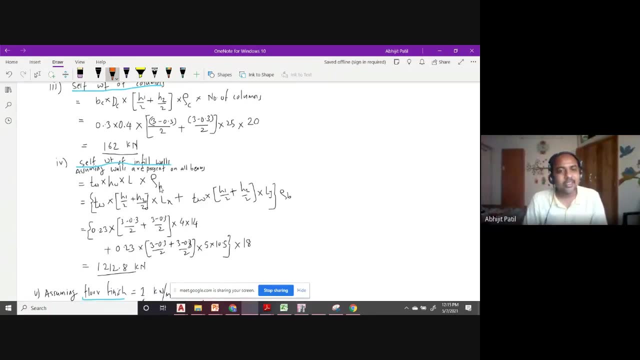 inside, no walls are there. so accordingly, you calculate the weight of the wall. so again, thickness of the wall, height of the wall, length of the wall and density of the brickwork. okay, and this height is again same as your columns. so that is why i have written h1 by 2, h2 by 2. 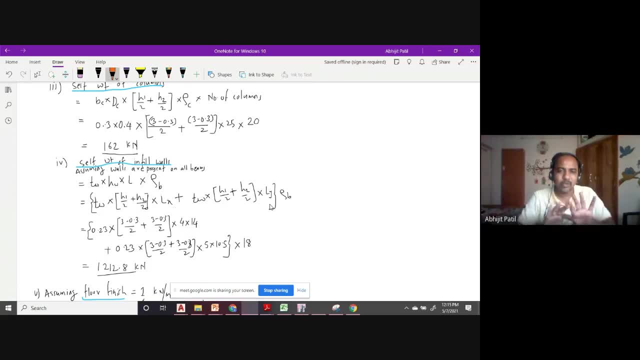 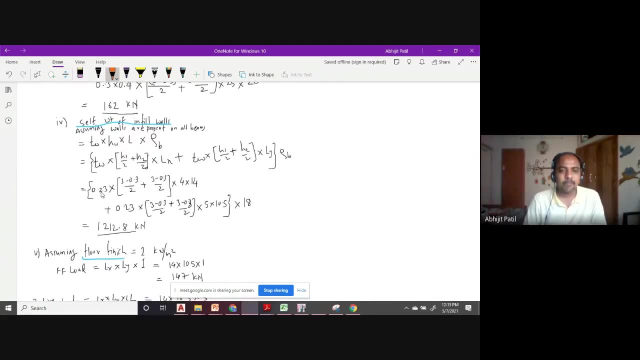 like that in x direction, separately in y direction, just for our ease of calculation. so thickness of the wall is 0.23 again here, if you imagine the wall is constructed up to the bottom of the beam. so i have, uh, subtracted the beam depth here. okay, and then? 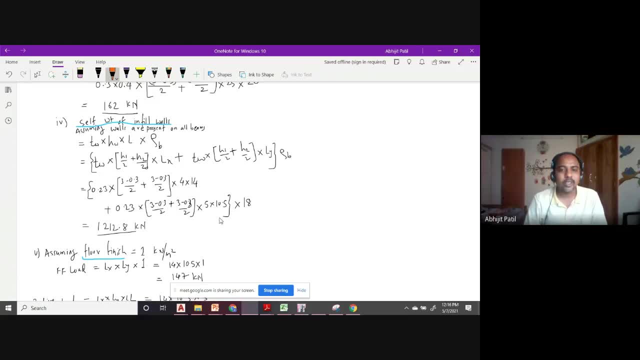 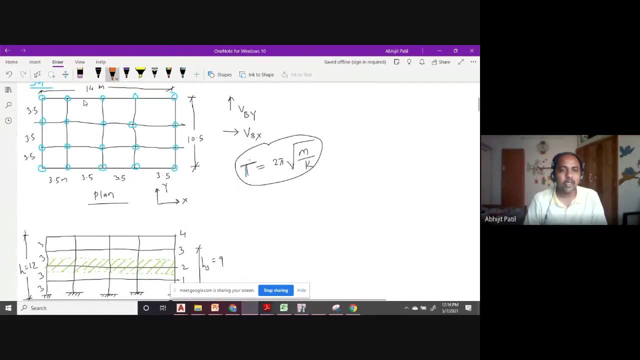 total same as your beams, so 4 into 14 and 5 into 10.5. okay, so 14 meter wall will be 1, 2, 3, 4, so 4 into 14 and in this direction: 1, 2, 3, 4, 5, 5 into 10.5. 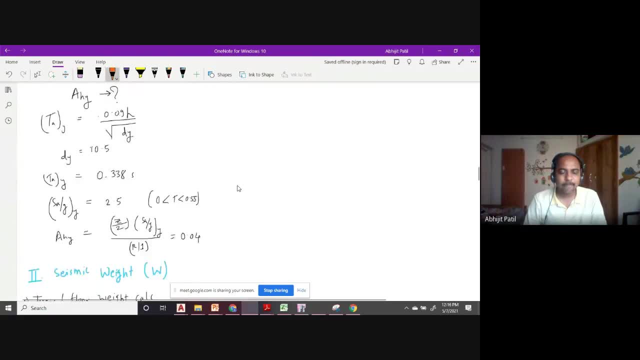 so a tube will be the same for both sides of the wall and then 1, 2, 3, 4, 4 into 10.5. so that gives us theta enclosed cap of the has is the crying triplet. we休it of h3. 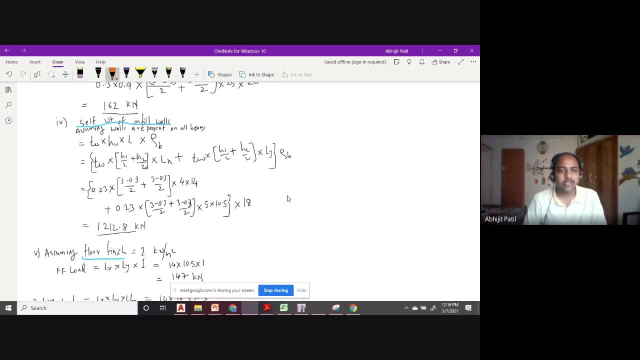 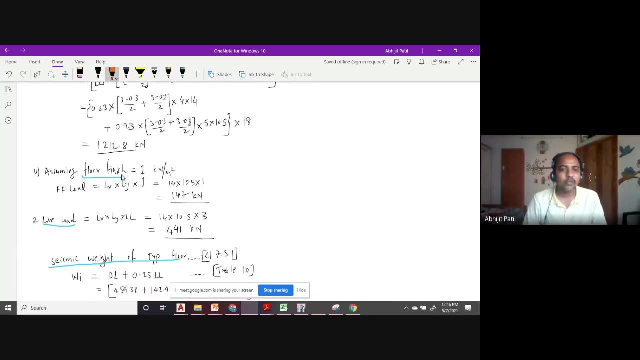 so on. so let me go to h幾 in person, okay, no problem, guys, and we can estimate this right. so we will start with some internal층 earthrolling. let me just put this in fine at once. okay, so let me just immumize and check this once in a while. 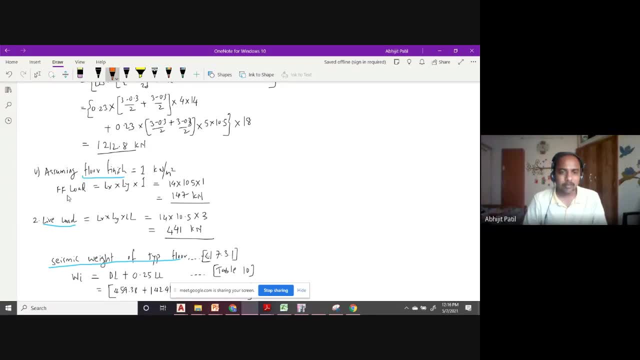 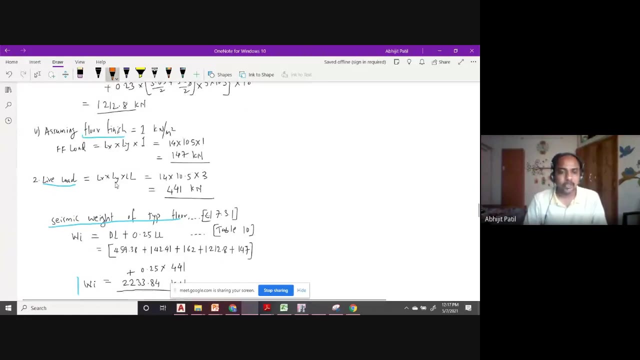 once in a while. Ugh islas d Ahora per square meter. so floor finish load will be simply area of the slab multiplied by this density, so 14 into 10.5 into 1. so this is the floor finish. lie load here is same as the area multiplied by the lie load intensity. so 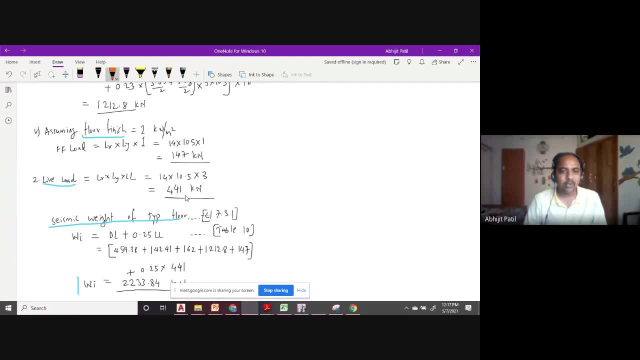 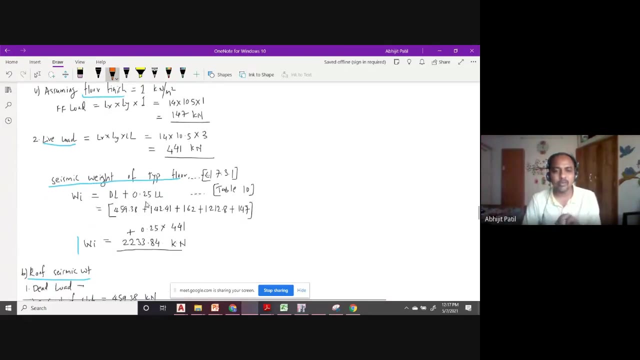 area into this. 3: this is the lie load commander now seismic weight of typical floor. so as per this clause, dead load, full dead load plus some part of lie load. so I have written here 0.25. so we will go back to code and see what it. 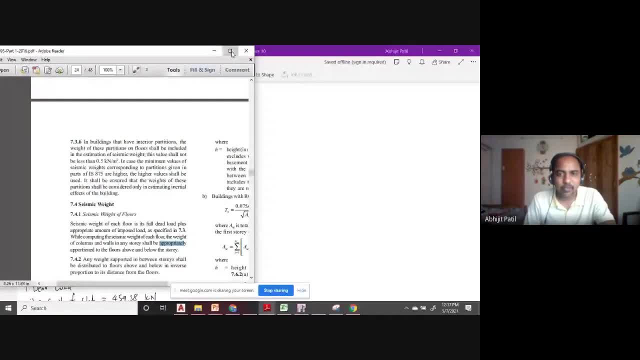 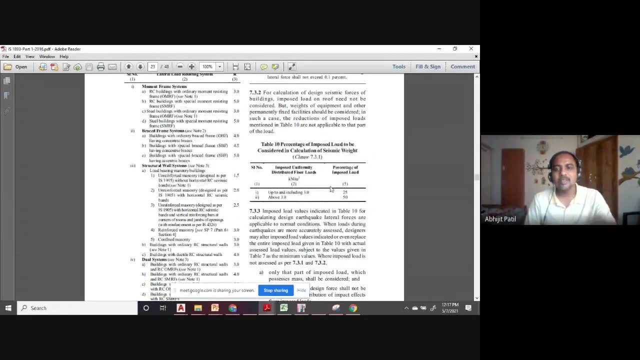 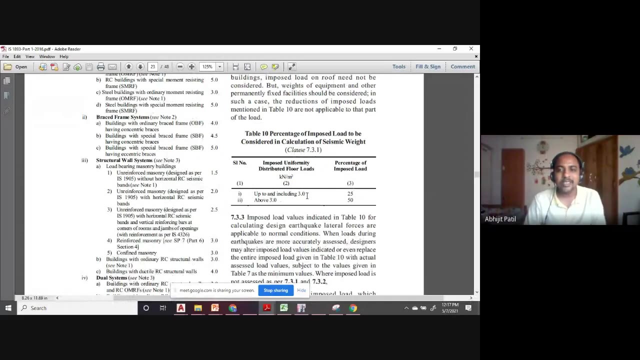 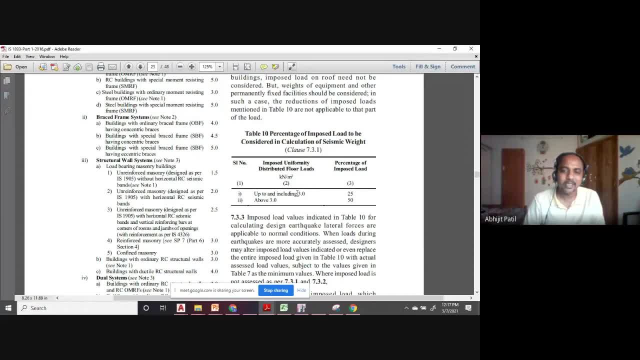 intensity is 3 in Newton per square meter or less than 3, you have to consider percentage as 25 percent. so don't we don't have to consider 100 percent, you have to consider 25 percent and your lie load is more than 3. but to 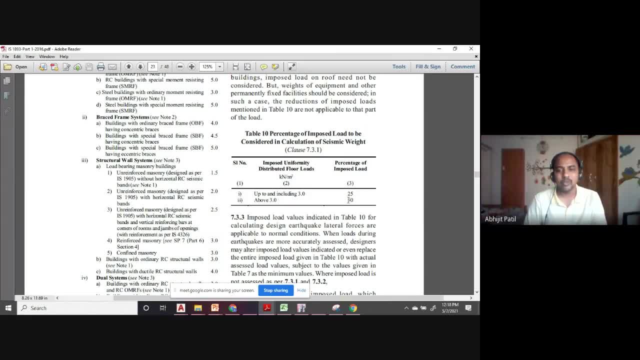 consider 50%. okay, so if you try to imagine why this reduced load we are considering- because, suppose you are, you are designing your college building, okay, of our weights, the moving load. moving load is what? the load of the people who are occupying that building? okay, so this load is not constant, it is always. 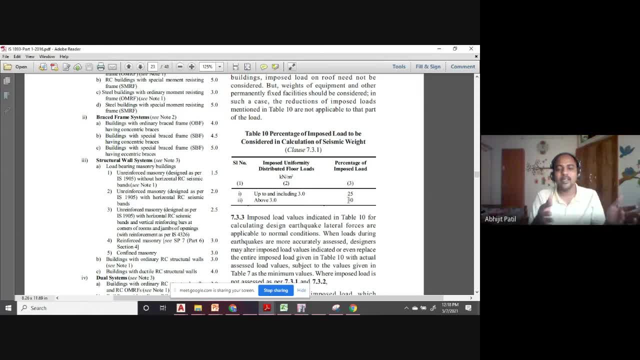 changing. so in during college hours it will be very high. during holidays or during non working hours it will be very low. okay, so this keeps on changing. so during an earthquake, it is very the probability is very low that hundred percent teachers are present. hundred percent non teaching staff is present. 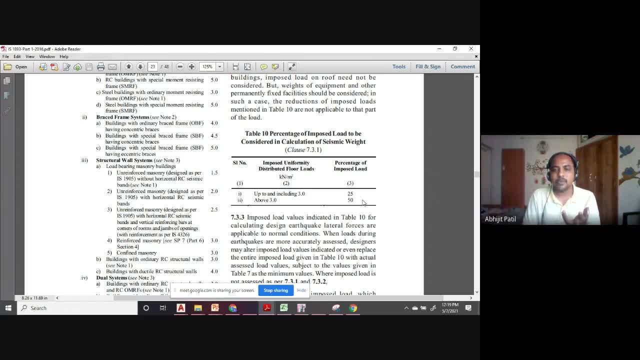 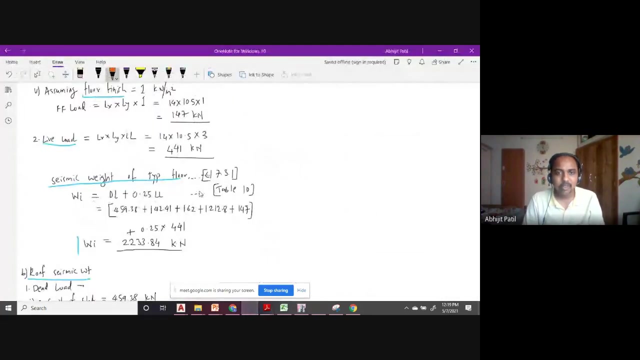 hundred percent. students are present, okay, and they are present on that particular slab, okay, and then earthquake happens. so this probability is very, very less. so that is why code allows us to use lesser percentage of light load. okay, so we are using- sorry, we will go to here, so as per that table- our light load. 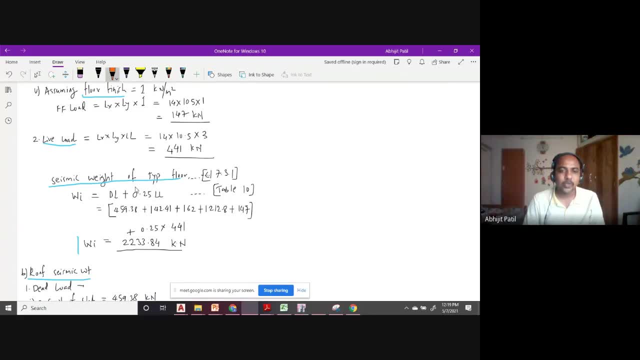 is three, so up to three we have to consider 25%. if it was four, we have to consider here 0.5 it. so just we will add all the loads. so these are all: slab weight, self weight of beam, self weight of columns, self weight of wall and floor finish load. 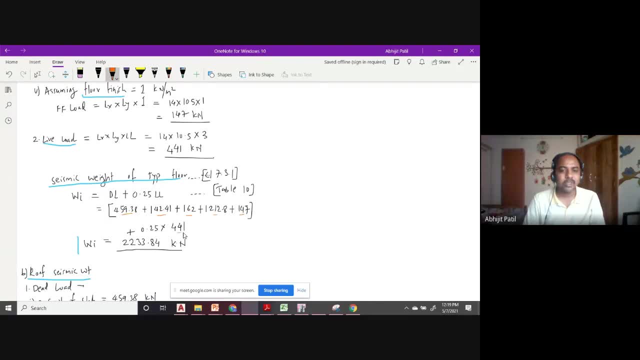 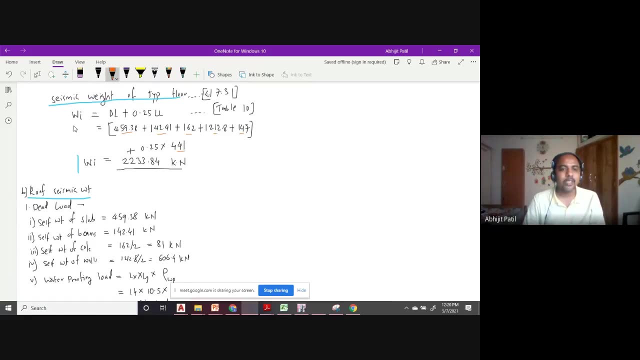 esque and two percent up here, sir, division line cherry, or three percent seconds between one the floor and each of the other side. okay, so basically this is: and l-7000 earth and same amount of standard, one brick and cedar, while we are adding the horizontal phase. now we are adding the horizontal example. 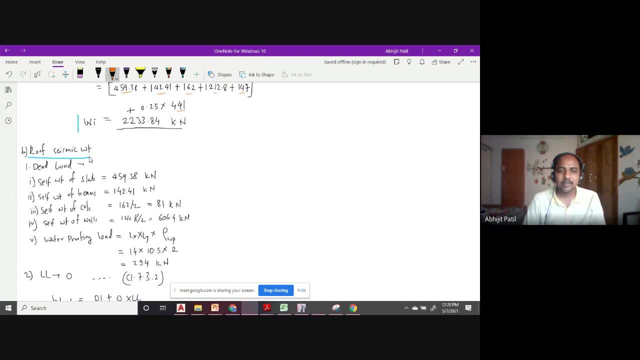 because the vertical phase ofquet is bad during lightning state. so we are using horizontal hyperontologies that i taught you all the time. so we are creating horizontal expected insane. The dead load of columns will be half. in that case, no column from above. Similarly, the dead load of walls will be also half. 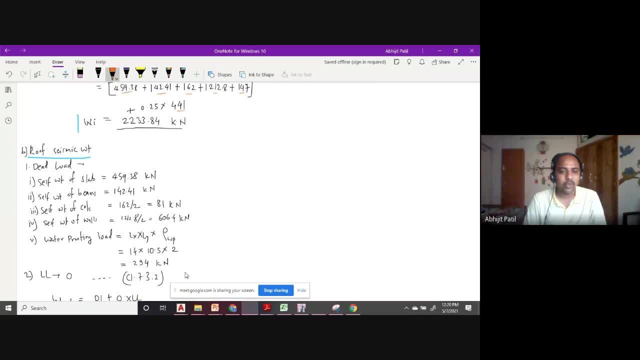 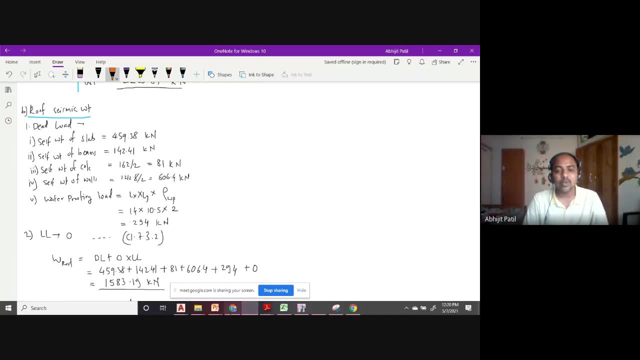 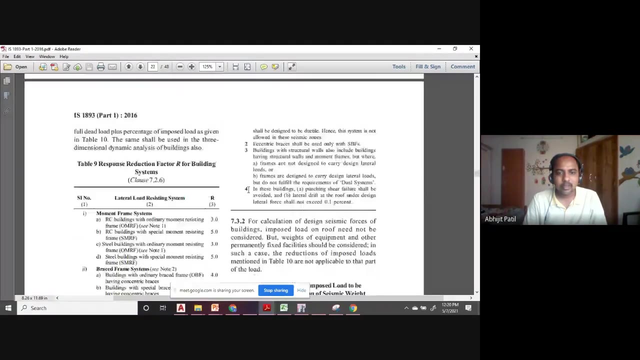 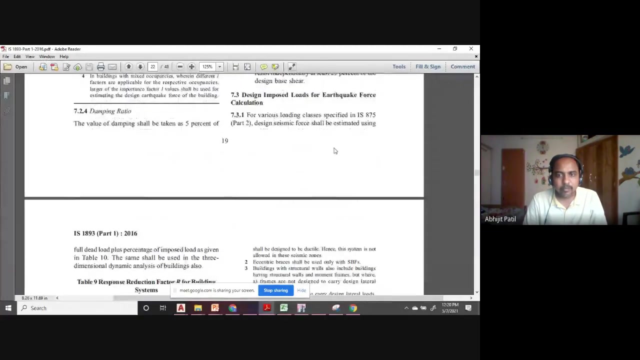 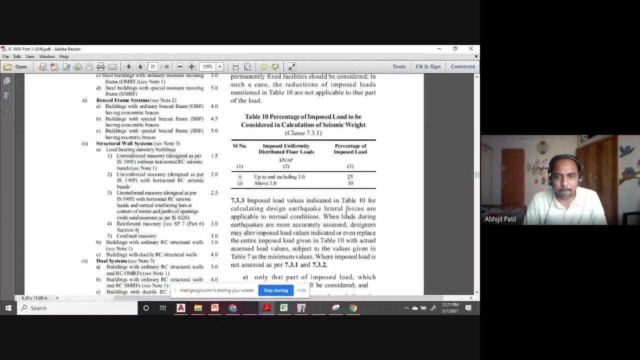 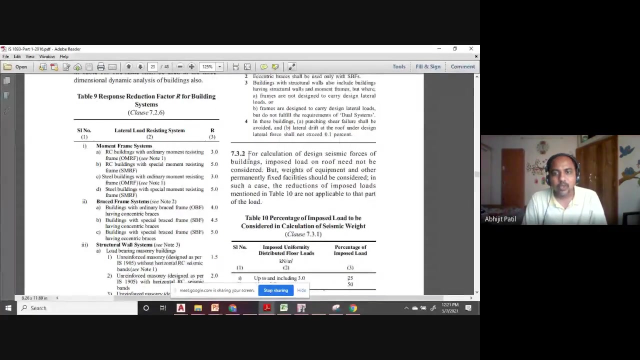 The waterproofing load will be different than the floor finish load And lie load here is considered to be as zero. So I will show that clause 7.3, point yes here. So for calculation of design seismic forces of buildings. 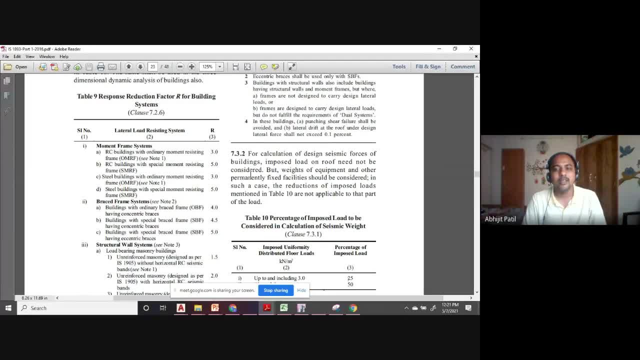 Imposed load on roof need not be considered, So we can consider this at zero. but some addition, waste of equipments and other permanently fixed facilities should be considered. So this can be if you have put a gym at the roof, which normally people do, or swimming. pools. Okay, So these permanent loads need to be considered, But other than that, if you are having normal lie load, that is, if you remember, if accessible roof is there, you consider lie load as 1.5 kilo ton per square meter. 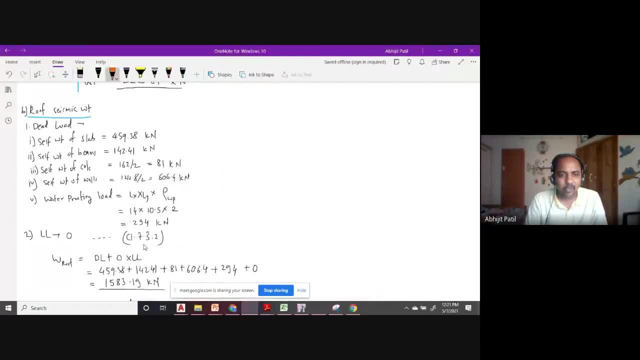 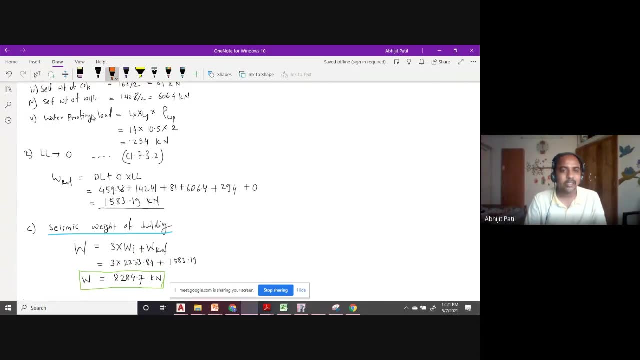 So you can consider that as zero in calculation of seismic weight of proof. So here you just consider a weight of proof as addition of all these dead loads plus no live load. So this is your roof load. So the total seismic weight will be. 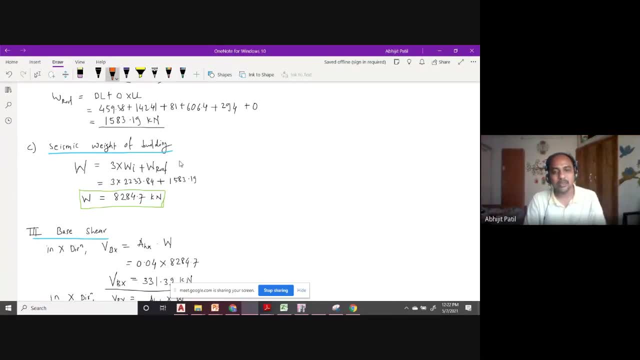 So there are, if you remember, four story. out of that, one is roof and the others are these three. So three times this weight of typical floor Plus one types the weight of room. So this is your total seismic weight capital W. Okay. 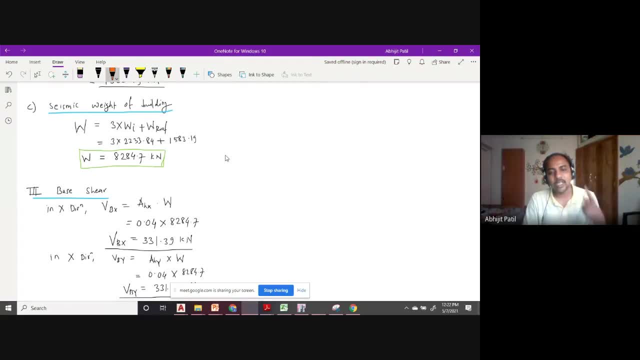 So we have got age, the seismic coefficient, and we have also got the seismic weight. So we have got both the entities. Now just multiply that to get the best year in respect to direction. Okay, So here it should be. So in Y direction and X direction. 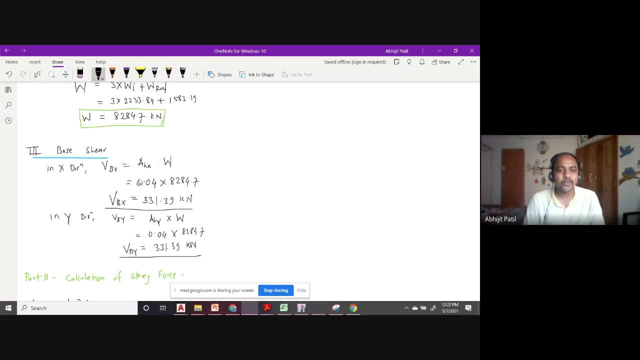 So fortunately here, in both direction, these coefficients are the same, but sometimes you will get different questions. That is why this value here and here they're coming out to be, say, 331 kilo Newton. Okay, So this is part a, the total calculation of the base year. 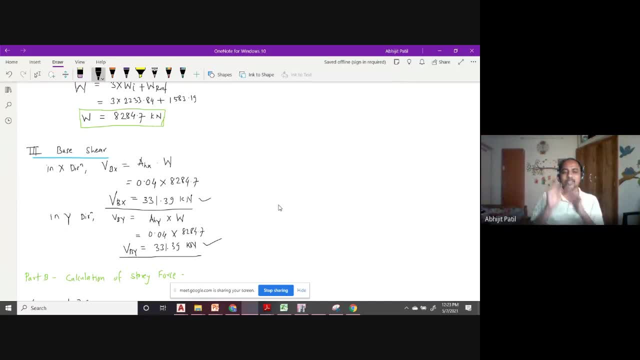 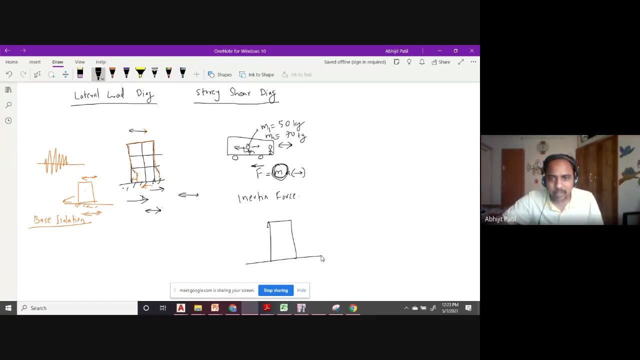 Okay, So this is part a. Okay, So base year. Remember, if you remember, I had told you that this is the force acting here at the. I will draw it again. If this is the building like this, this total force is acting at the ground level or at. 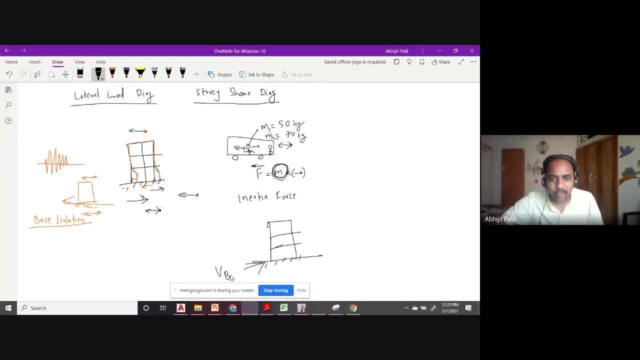 the foundation level. So this is in X direction, This will be X. This is in Y direction, This will be Y. Okay, So this part a we have finished. Now to analyze the building. you have to distribute this force all along this building. 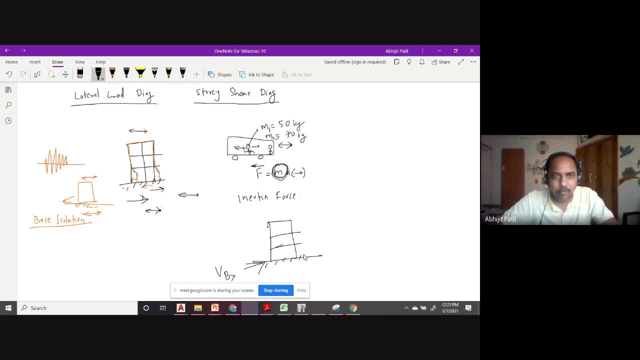 So there will be This floor force will be distributed along this Floors. So this force is actually acting at the floor levels, because just now we have- we had seen that mass is assumed to be concentrated at the slab level. Okay, And force F is equal to M into A. So wherever there is mass, this force will be present. 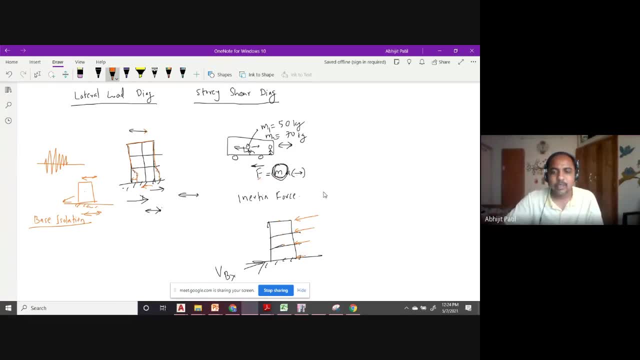 Okay, So mass is present at the floor level. So we will consider: at each floor level This mass will be distributed like this. So this will be: uh, if it is in X direction, so it will be X, four, three, two, one, like 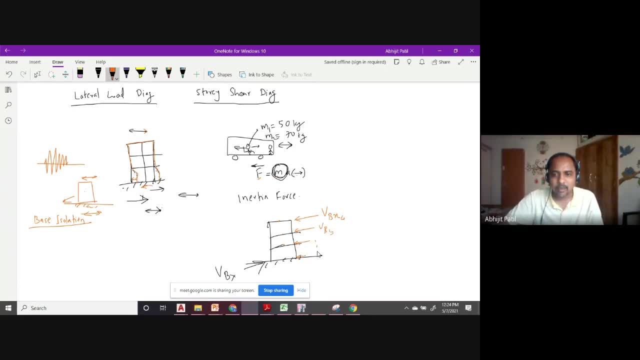 that, Okay, Like that It will be distributed. now, how to distribute that again? uh, this code helps us in doing that, But what is the basic, Uh, What you can see, um or fundamental behind that, uh, distribution or method? I will explain. 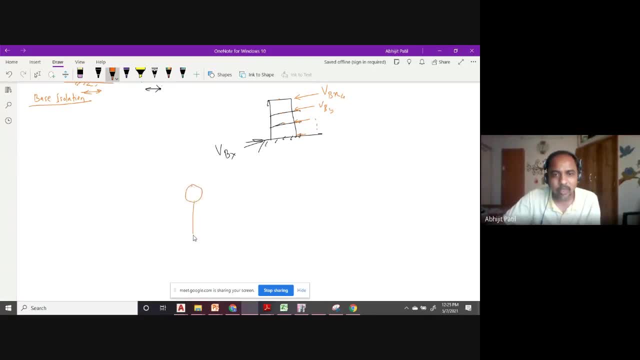 that. So you have, uh, we had seen yesterday one model, but this is all. this also represents a building, So this represents the total mass of the building and this represents the total stiffness of the building. Okay, So yesterday, if you remember, uh, one professor had demonstrated that different heights of 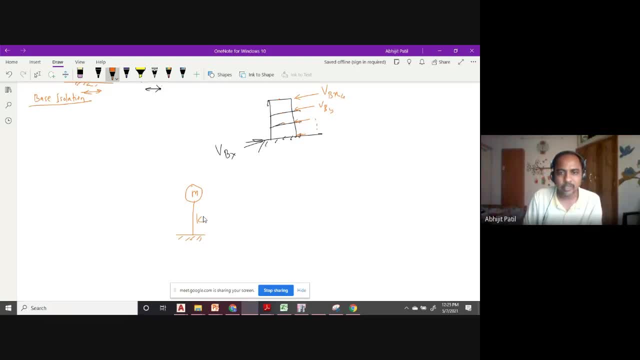 buildings. Okay, So in that case, that that is nothing but that mass is uh was attached at the top and some string was attached here. Okay, So this represents a typical building. Now, when earthquake comes, or if you just move this uh ground or base, this will start. 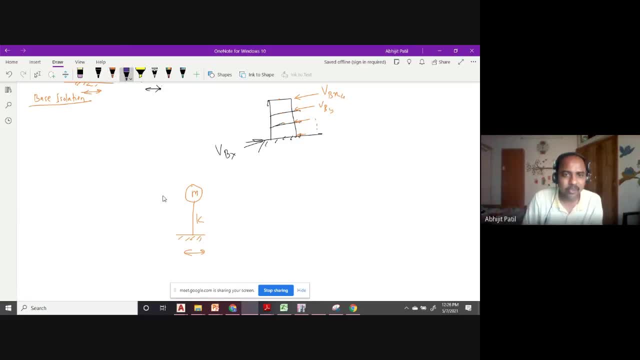 vibrating like this. What will be the nature of vibration? It will go here, Okay, So It will deform like this when it will move forward and it will also move backward. Okay, We had seen the demo yesterday Like this, Okay. 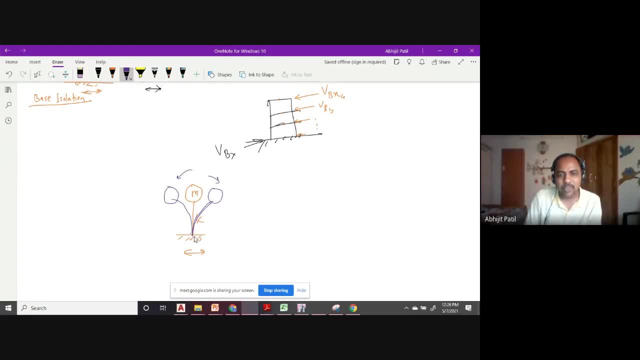 So forward, backward, forward backward. So it will move like this And, if you see, this is the nature of deformation, So it is in, It is in, Okay, So it will deform less here And as you go away from the base, as you go towards roof, the deformation rate will increase. 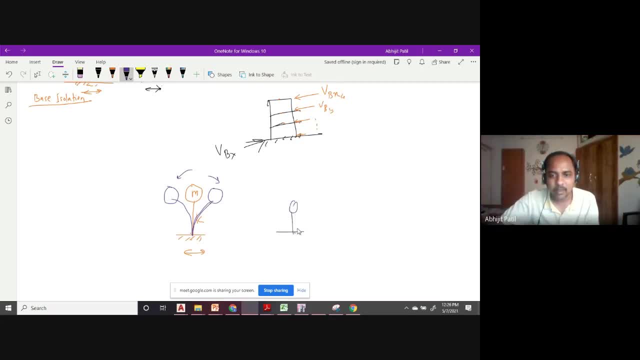 It is not a linear deformation like this. It is not a linear deformation like this, It is actually parabolic. So what is the parabola? this, This type? So? So, at lower level, the deformation is less, but at higher levels, The deformation is more. 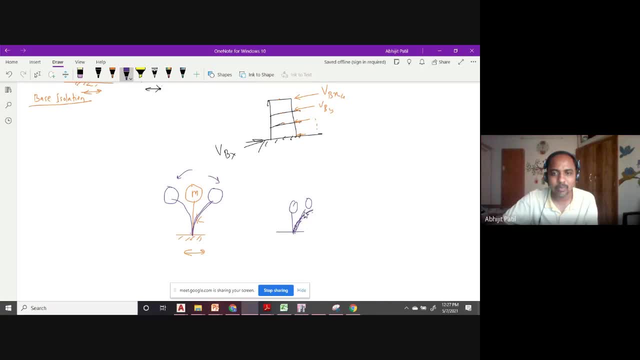 Okay, So, okay. Okay, formation is more. So this is the difference between linear and parabola. Okay, So, what code has suggested? because we know that the force depends on the stiffness as well as deformation. So more the deformation, more will be the force. Okay, So, using this fundamental, 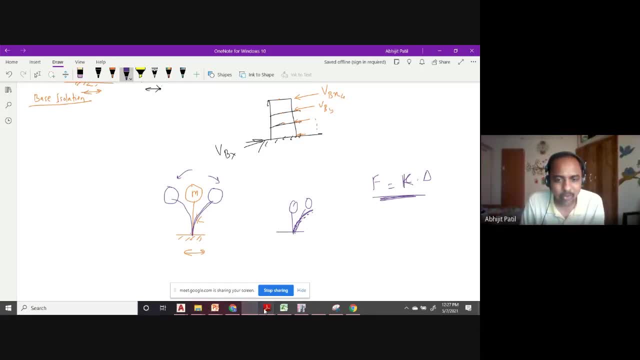 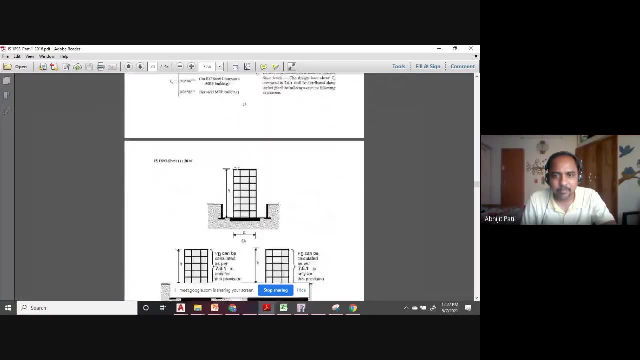 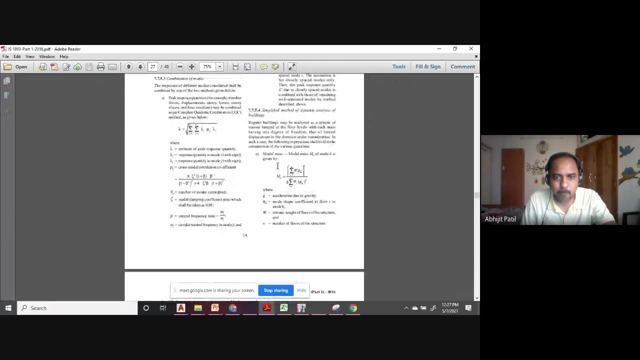 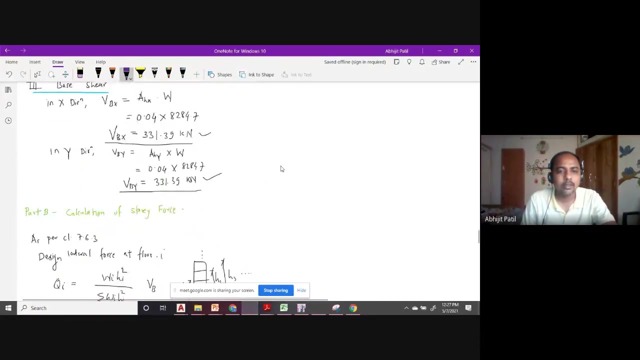 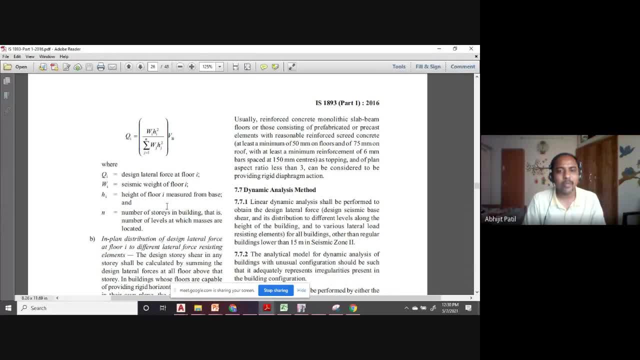 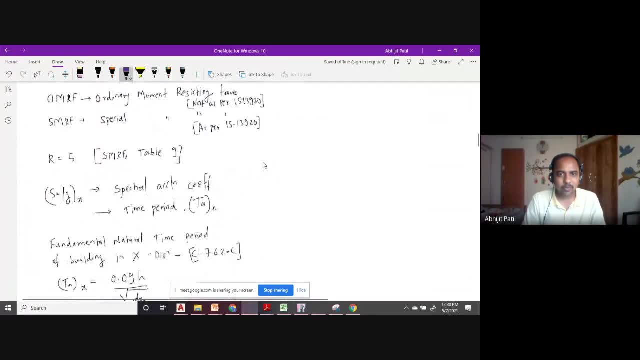 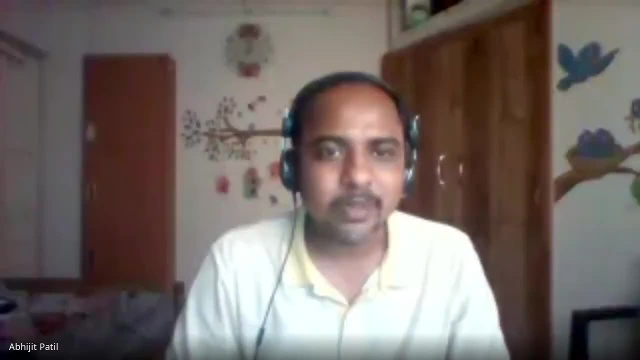 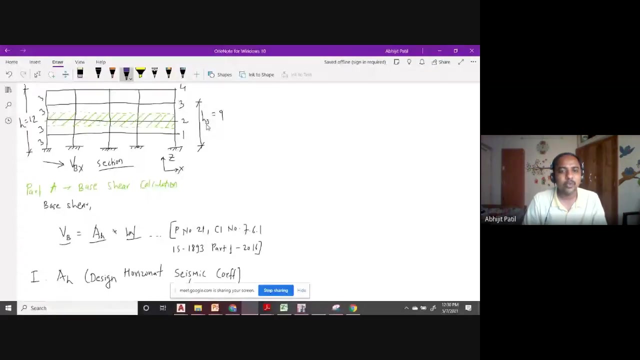 h i height of the floor. i measured from the base, okay, so i think i had mentioned it some. h? i for second floor will be six meter because you have to measure from the base. h? i for third floor is called h3. it will be nine meter, okay. so height of each floor from the 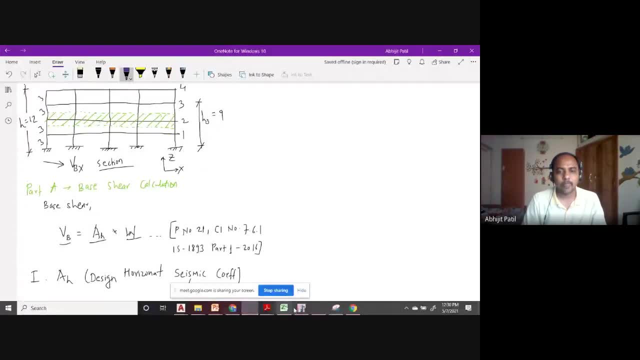 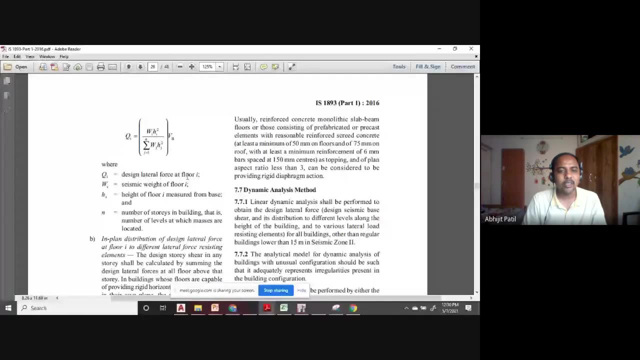 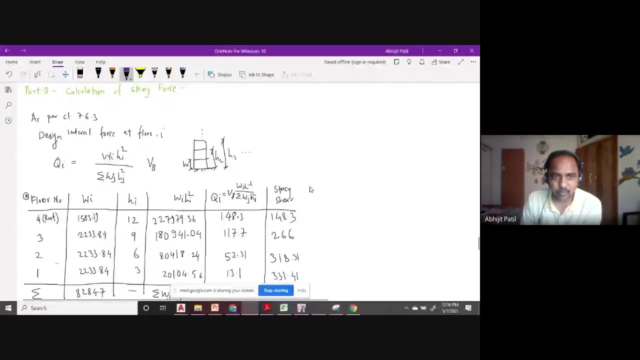 base and then n is number of storage in the. okay, or that is the number of levels at which masses are located. it's okay. so once we understand this, so again, we will come back to this formula and in a systematic way we can find this. so i have, uh, or not, i have also copied: 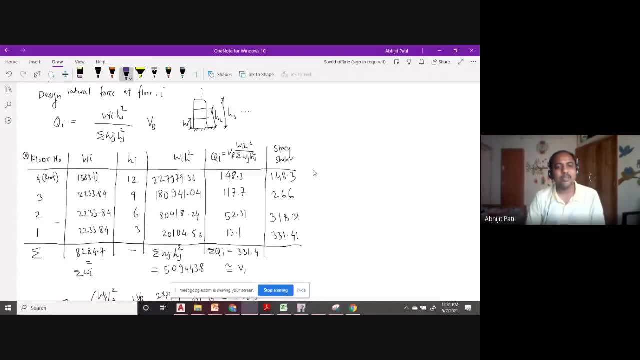 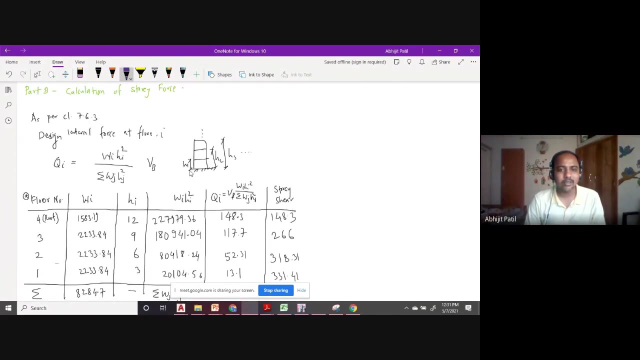 from a book. so in most of the books, uh this method, simple table tabular form is used, so it is very uh easy to understand and to calculate this. so this we have written from clause number seven, point six, point three, and uh, this h i try to understand, is: 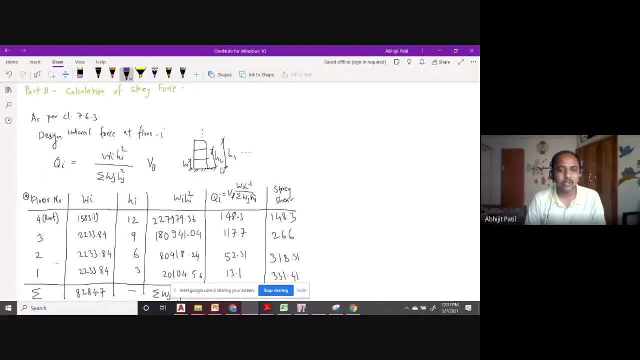 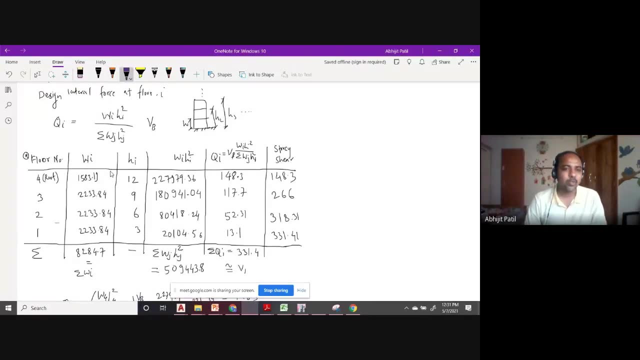 height of each story from the base. so h1 will be this, h2 will be this, h3 will be this, like that. so what we have to do, so we are, we have made these columns floor number wi, hi, wi, hi square. then this formula, qi into qi is equal to vb into wi h. 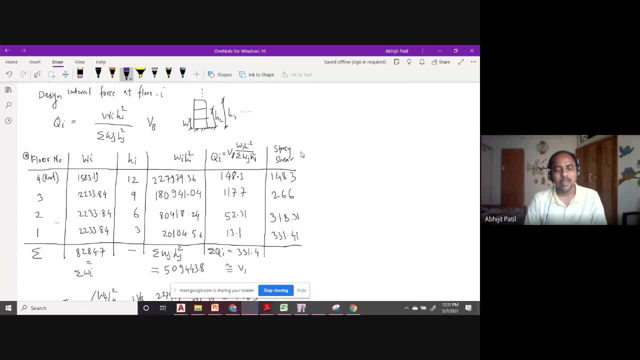 square divided by summation, wj hi square and this is the story shear. okay, so this is story force and this is storage here. so later on- uh, first just don't focus here. up to this point we will focus and then i will tell you what is this last column. 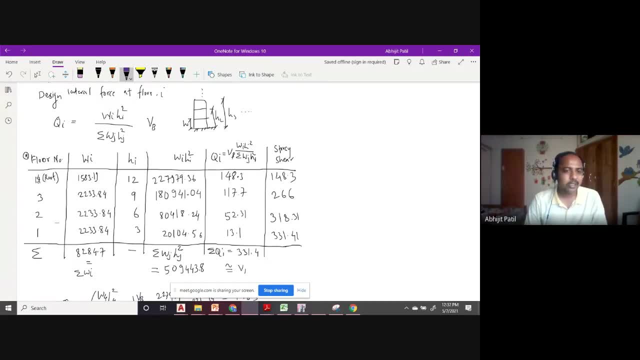 so once we have written this second step, just write in reverse order from top to bottom floor: three, two, one. so if you are having 10 solid building, it will start with 10, 9, 8, 7, like that up to one. then just write the uh seismic weight of that. 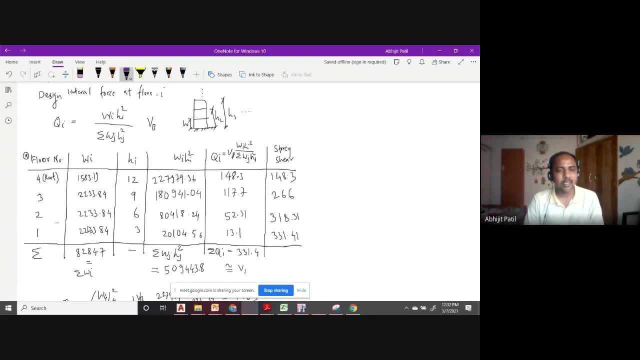 each floor. so if your building is typical, like, just like we are having here, each floor will have same uh seismic weight for roof. it is different. if it is having different, you can mention that different, different uh seismic weights. then hi, here is height of that particular floor from the base. so here roof is at the top, so it is 12 meter. 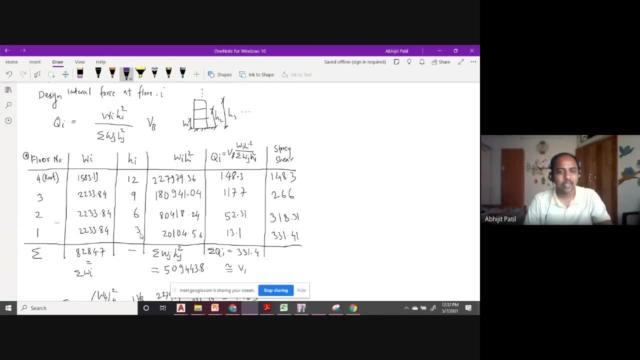 then third floor nine meter, second floor six meter, first floor three meter. okay, so this much we have to just input, then just make square of this hi and multiply that with seismic weight. remember this is in kilo newton, this is in meter. okay, so this value we will be getting for that respective floors. 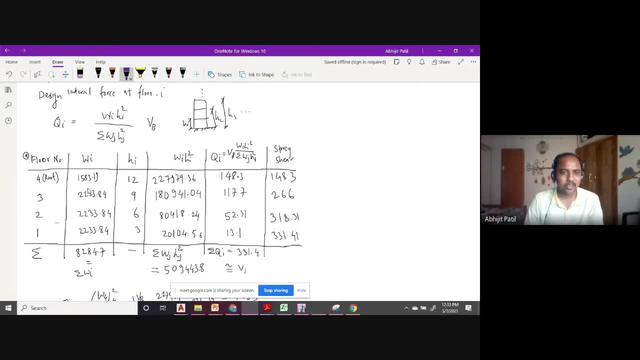 okay, and here you will get that summation. so obviously there, this seismic weight summation is summation wi here. this is summation wj, hi square. so just add all these values here, write down at the bottom and this qi. how are we going to calculate that? 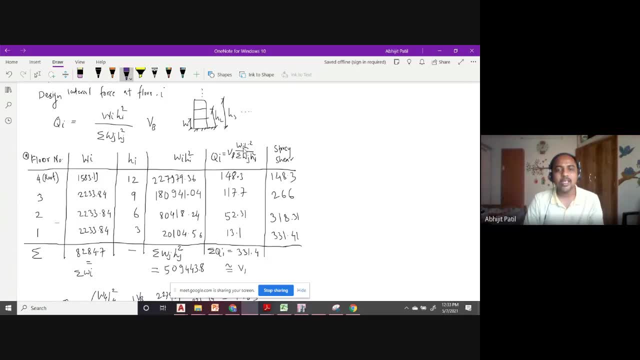 so summation: qi hi square. so above is wi hi square, so here it will be. for roof it will be just like this: w4, sorry, into h4 square divided by whole summation: wj chi square. okay, so for four story it will be like 22 000 or 22 000. 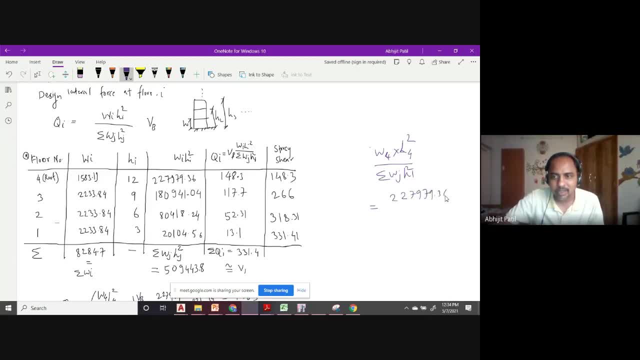 something- 22, 7979.36 something. so this value i have taken divided by the whole summation, 59443.8, and multiply this ratio with your vb base year 331, something we had calculated okay. so this is constant vb by this ratio. this value will go on changing as per floor. 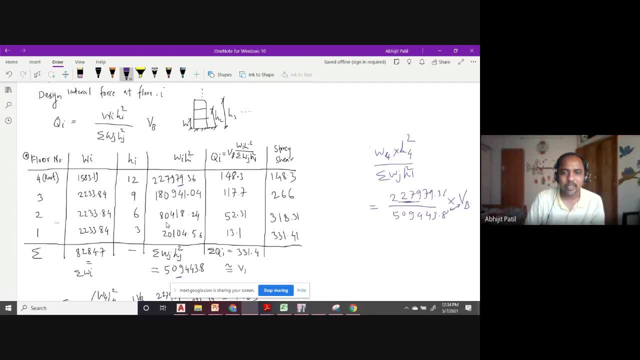 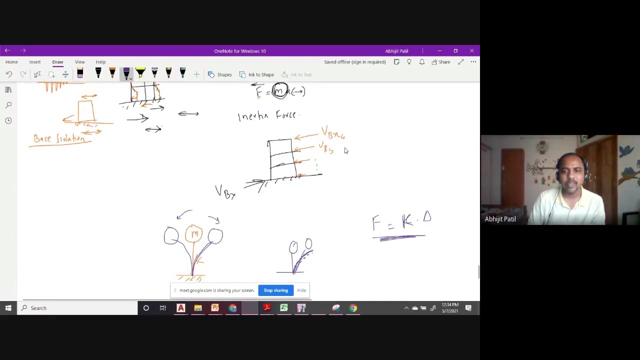 so for next floor, you will use this value in numerator. for next floor, this value, this will, whatever answer comes, just write down here. okay, so this is your story shear or story force design: lateral force at floor level. so 148 kilonewton will be acting. so if you go here, so this is 148 kilonewton, below that, it is 117. 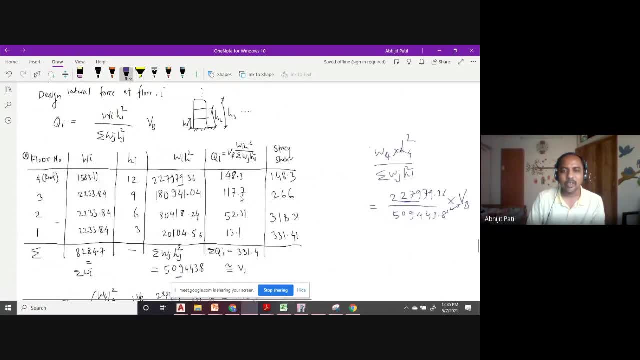 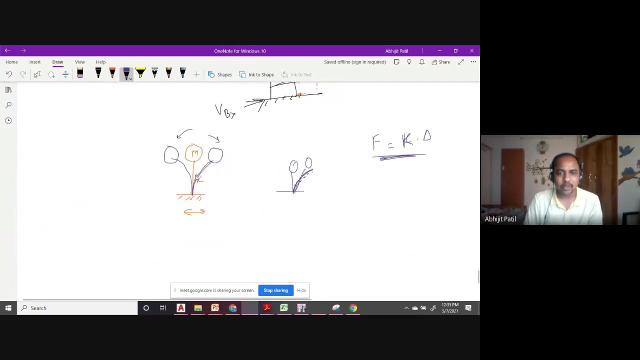 kilonewton. so if you see, this goes on reducing and this reduction is in not linear manner, it is in parabolic manner. okay, if you just put these values in excel and just plot the graph for fun, you will understand that this is not linear. this is parabola. just like this deformed shape, just like 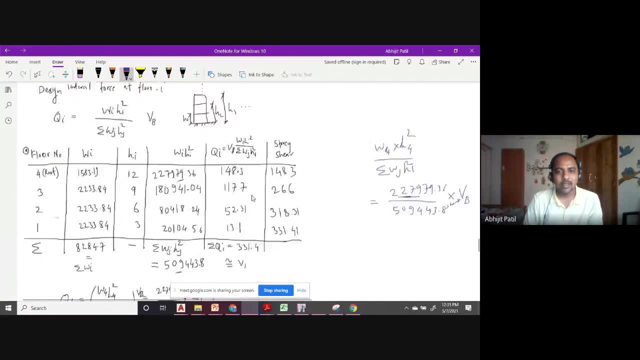 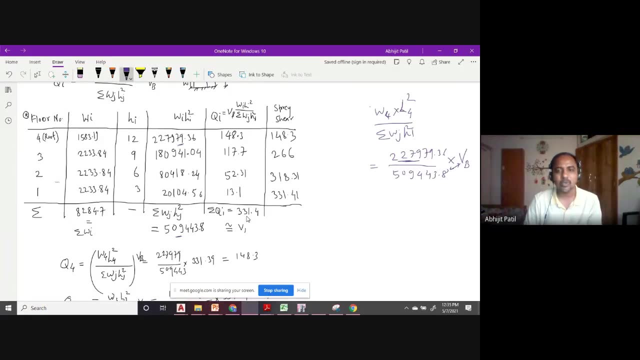 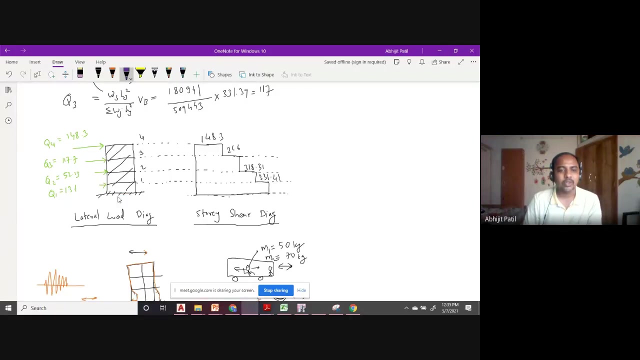 this, okay, and if you get summation of this, this will obviously match with your base year 331, point 4, and this should. that means your calculations are correct, okay, and what is stories? here I will go to this figure. okay, so this is our actual building for storage building. so at first story, level 13.1 here. 52. 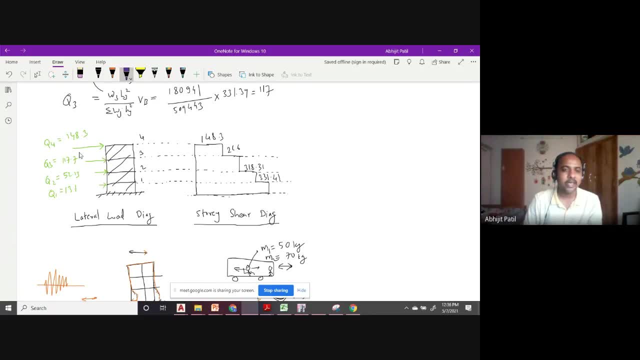 here 117, here 142. so this is the lateral force acting at each floor level and just like, if you remember, cantilever beam, with some forces acting, and if I ask you to draw SFD, if I ask you to draw SFD, what you will do. 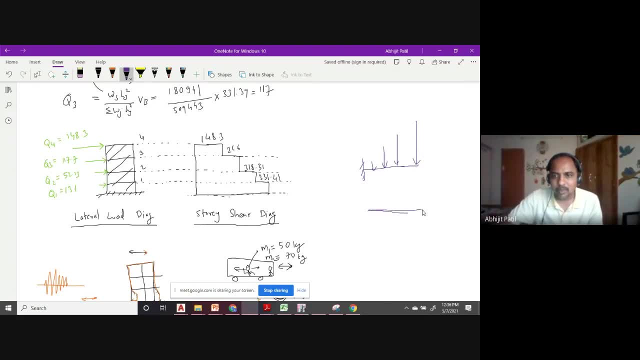 you will do is you will draw shows here which I have dropped. so I am going to, will just go on drawing the assembly like this: so this is 142. then no force travel, travel. then this: I will add 117 here. so this is 142. sorry, 148 something. 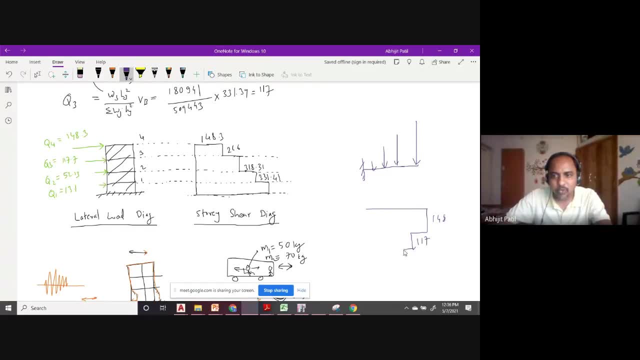 here it is 117, then no force, then 52, no force, and 13- sorry this too far you- to no force, 13, no force, and then this will be reaction. so it seems this: this is cantilever, so addition of all these three, it will action and addition. 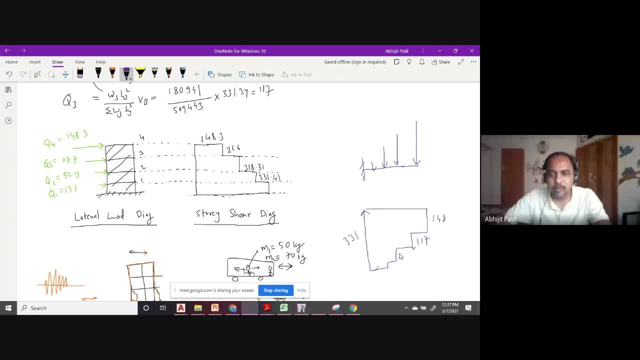 of all these three is nothing but your is nothing but your 331 base here, 52 and 13, right. so this is the way you will draw the SFD. so story share diagram is nothing but accept the off your earthquake forces. only thing is our building is standing. 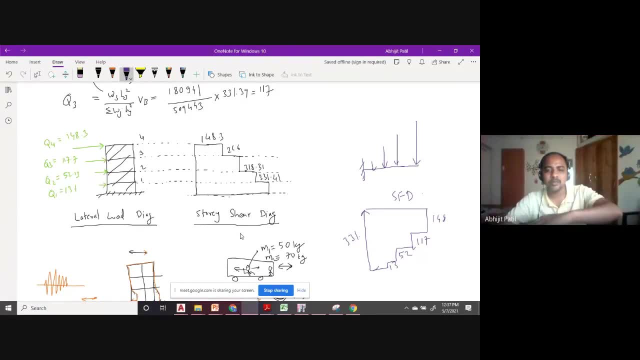 vertical. you, up till now you must have drawn a simply for horizontal beams here, SFD, for just consider this as a vertical cantilever where the support is at the foundation level, okay, and just go on drawing. so this is what we have done. 148, then no story share, then addition of 117, then addition addition. okay, so that. 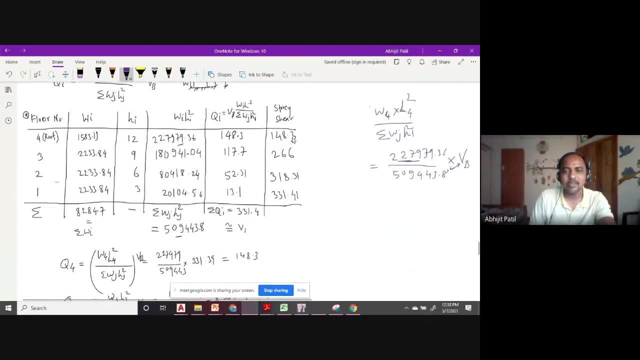 is what we have done. so first value, right as it is. next value: just addition of this 142 plus 117 i have written here. then addition of this 318, then addition of this 331, and this will obviously be equal to total base year. okay, so i hope you have understood. so this is. 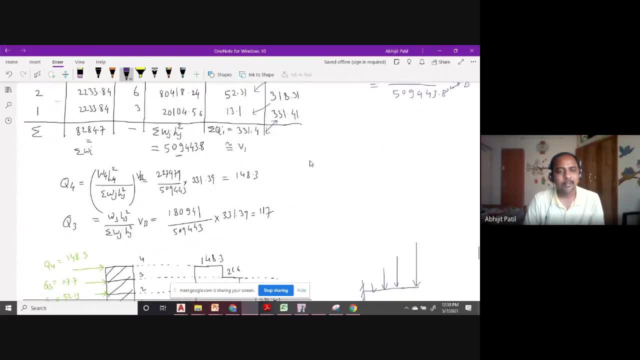 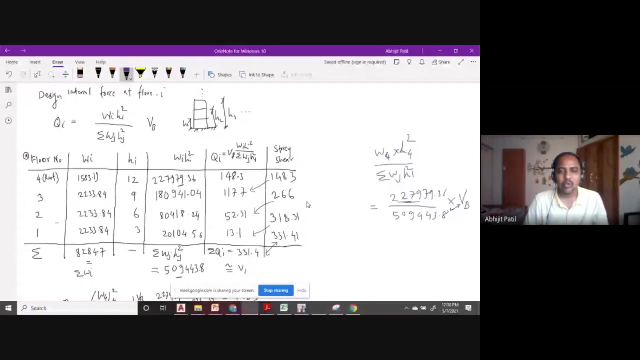 in x direction same thing, since the earthquake force is same in other direction, same table will be repeated. if the earthquake force value is different, these values will be different, but the pattern table, etc. everything will be same. okay, so this is the way you calculate the earthquake force coming on a structure, whether 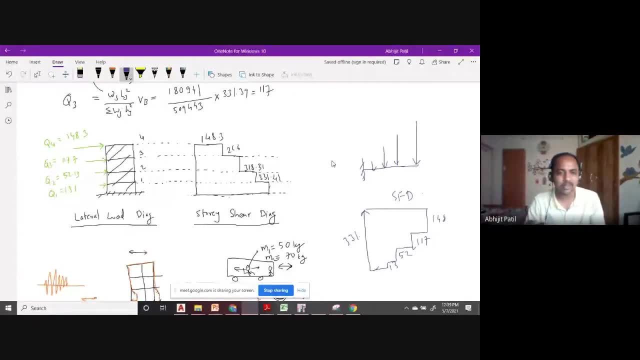 it is a, a, a single storage structure, or it is 100 storage structure. okay, so this is very basic uh, simple codal. uh equivalent static method, it is called. now next step. obviously it is not in uh at ugc levels, but you or you just have to analyze this structure. okay, so, because of these forces, there will 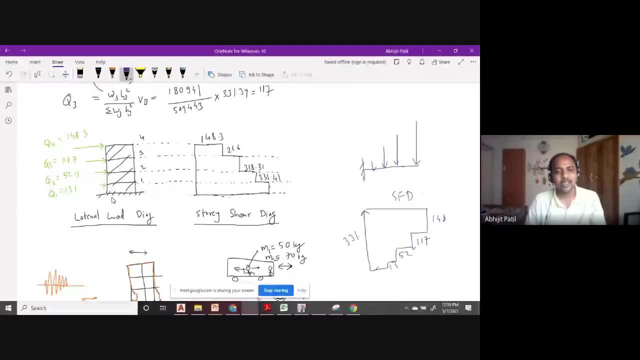 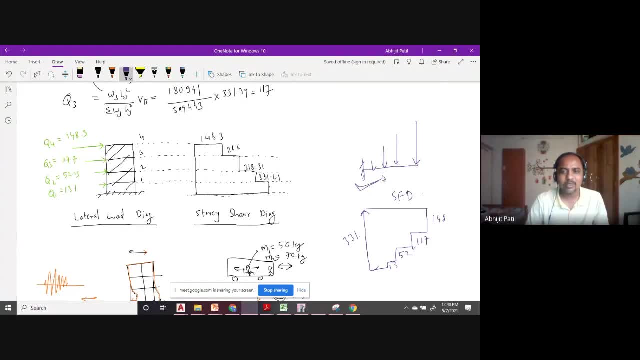 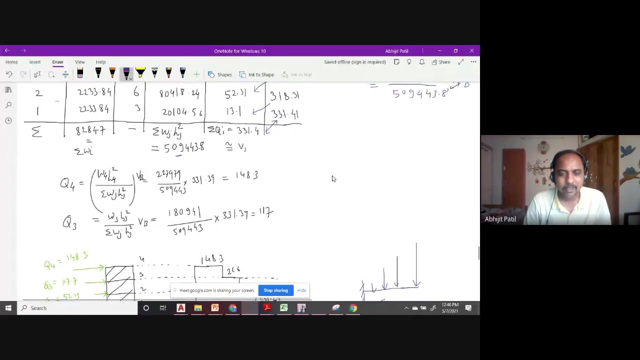 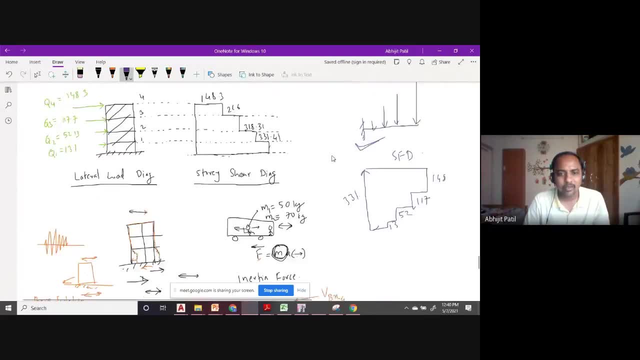 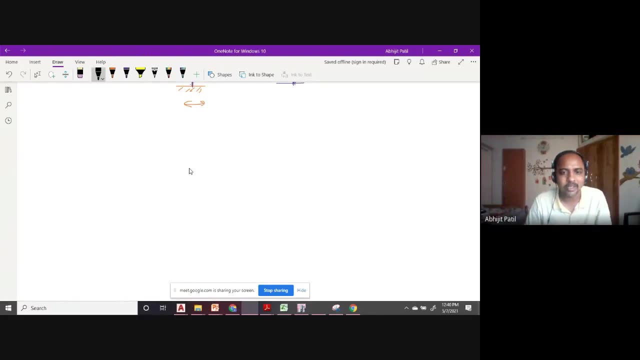 the height. yes, yes, yes, it is along the height. very good question, so i will just. of course, this is again not part of syllabus, but you must know what exactly is happening. so, basically, i will draw a floor plan, okay, and uh, i will not. okay, i need to draw columns also. so let's say there are a few. 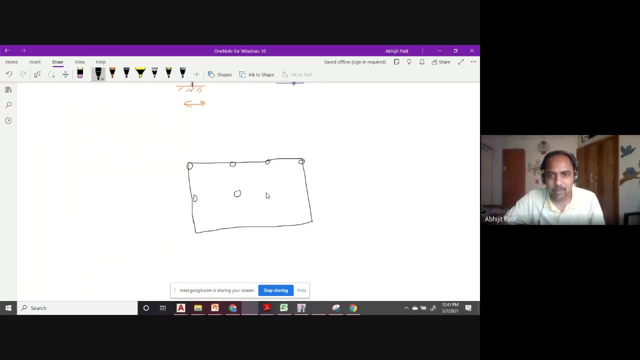 columns like this. okay, so let us say that. uh, this is floor number three, where the earthquake force was 117 kilo newton. right, so we have separated that floor. so this is what is happening now. where exactly is this force acting? okay, so there are. there is a concept called. 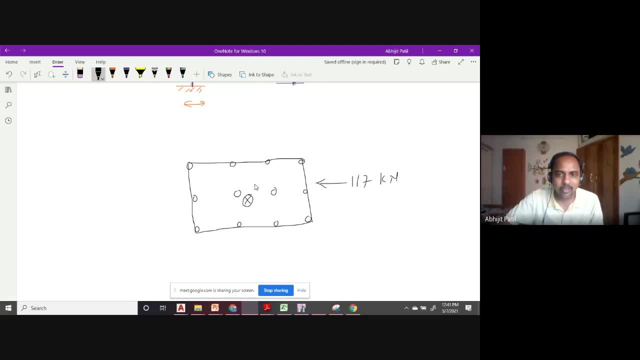 center of mass and center of rigidity. so typically, ideally, if all the columns are round, all square, all the beams, it is very symmetric. the center of mass and center of rigidity will collide with each other. so what is center of mass? it is basically center of gravity, of whatever mass. 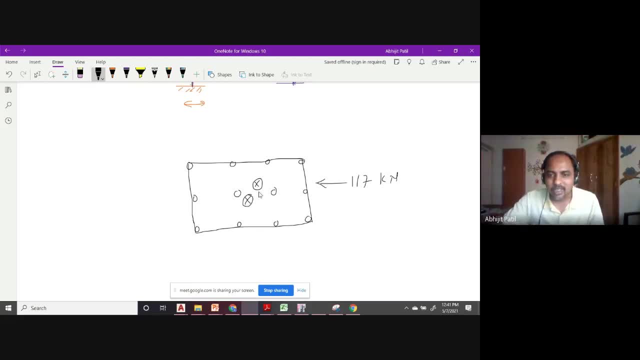 is present on that floor. okay, and what is center of rigidity? it is the center where, the center of stiffness. you can say. so how to calculate center of stiffness? it is very, very easy. you calculate the uh stiffness of each column. so let us say this is k1, k2, k3, like that, k4. okay, and 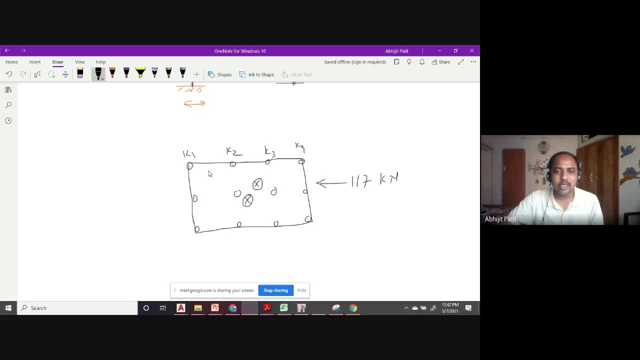 by using this you can just calculate the relative distance. so how to calculate that summation of yeah, yeah, x, i. so it will be again in x direction. it will be different in y direction. it will be summation, sorry, it will be numerator k, i, x, i like that. okay. so you calculate for each column and then divide it by a total. 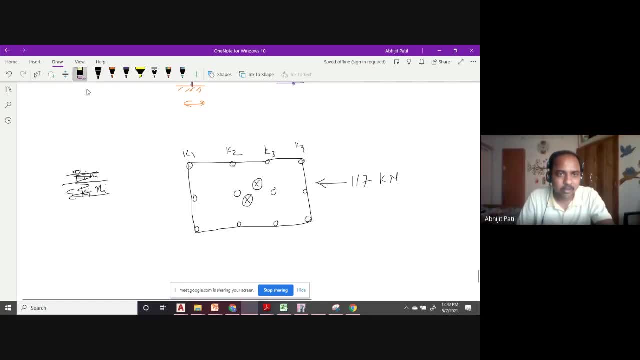 sorry, it's not like that. just a second. so with refer with respect to any reference point. let us say: this is my reference point and i am calculating x in this direction. okay, so from that direction, summation: k, i, x, i. so what is k? k1k2k3, what is xi? from this point, it is to the center. it. 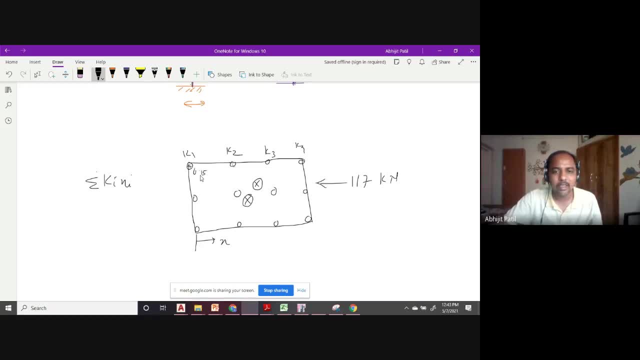 is suppose 300 column, so it will be 0.15 from this side, because this is my zero here. suppose your base spacing is 5 meter, so it will be 5 plus 0.15. 5.15 will be my x2 like. 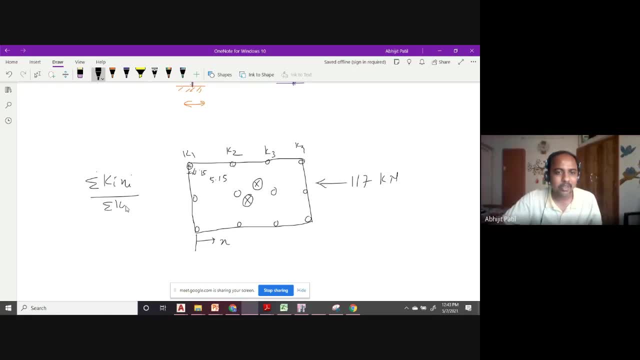 that. so you have to just multiply that, divided by summation ki, you will get x bar. okay, so x bar is my location of center of rigidity. so this is i am calling my center of rigidity, okay, similarly, in y direction you can calculate. so cg, or center of mass, is where my earthquake force is acting. 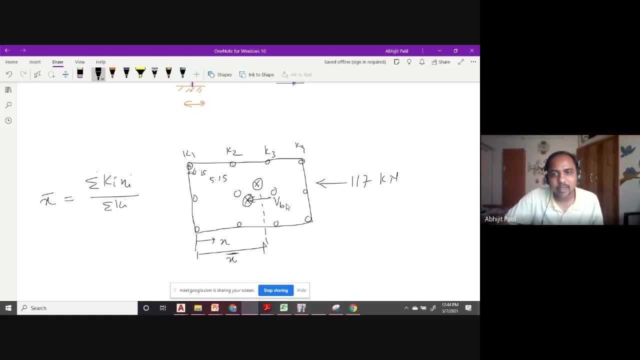 the, the x3, let's see, because we are considered third floor and center of rigidity, is where the resistance force is acting. so i'm calling this as i let us say. this is r x3. okay, so if these two are matching, no problem, but if these two are not matching, there will be 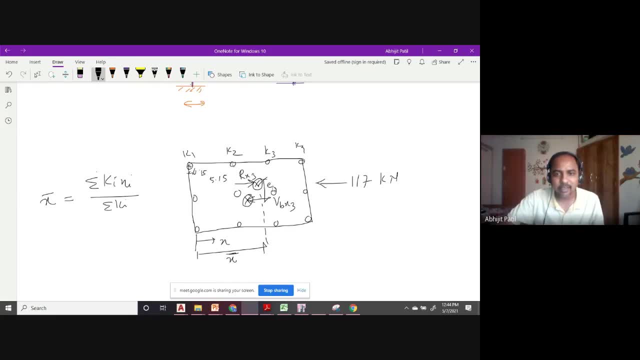 some eccentricity. e. okay, so 170 multiplied by e. this movement additional moment will be acting on this floor. okay, and this force and these moments are distributed along the columns. okay, because this is rcc slab. okay, so rcc slab what it does, although the forces as you. 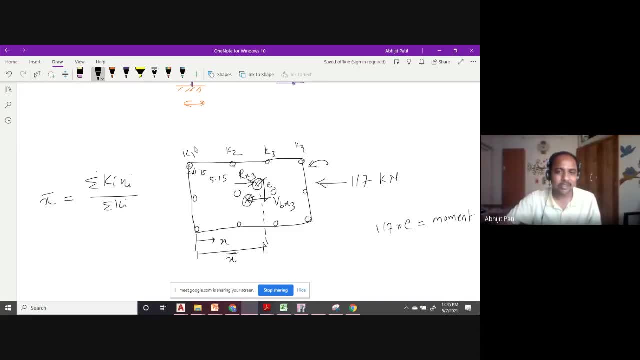 believe my rcc means the whole rcc will be acting along the column right. so rcc slab, the force is to be acting at the center of gravity or center of mass. this distributes the force along all the columns. and how this is distributed again using this. so what is the suppose? k1 by summation k. 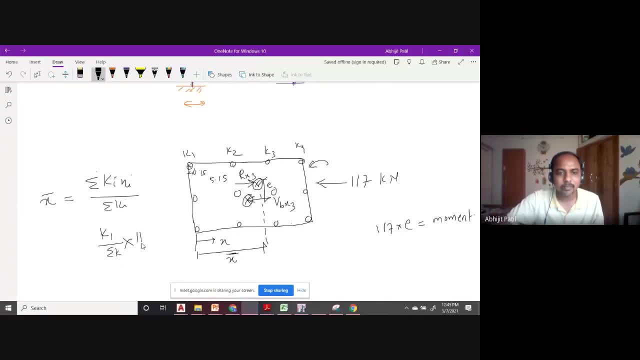 is multiplied by 170, understood. so, depending upon the stiffness in x direction, because stiffness will also vary in extension will be different. if you remember, in stiffness formula there is I right. so if your column is like this, this is B and this is D, let's say so in. 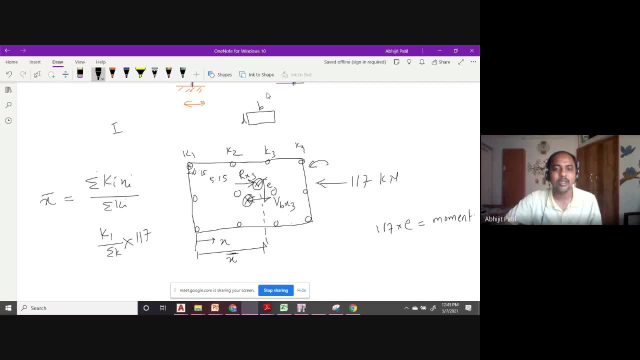 X direction, the stiffness will be different. in Y direction the stiffness will be okay. so what is the stiffness of your column in the particular direction divided by the total stiffness of the column or that flow? to multiply this fraction with this force, you will get the actual force coming on this column in addition to that there. 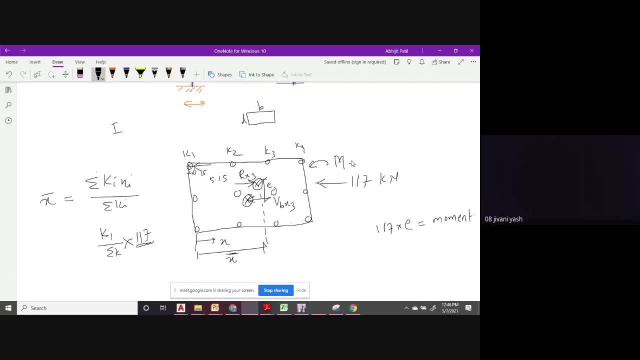 will be this moment. the movement is also distributed. yes, moment is also distributed. moment is also distributed in the same pattern. okay, so in whatever, if you are using start or it apps, any latest software, so all these calculations are then automatically in the software. even there is provision you can provide this eccentricity if you are not satisfied with. 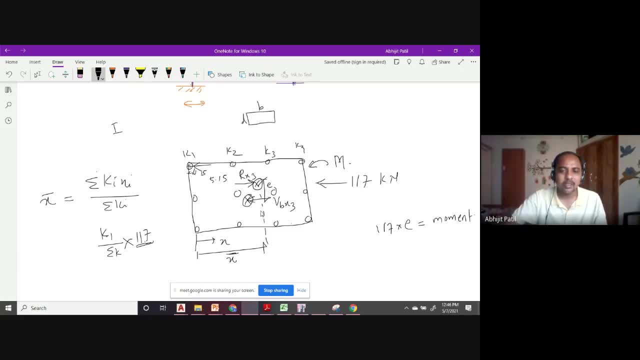 software's calculation. you can manually you put some eccentricity at each floor level, different these in the cities also at be put okay. so once you get this now imagine the whole structure. it is like this. so fourth, third- I'm just drawing this column- second, first and foundationally so. 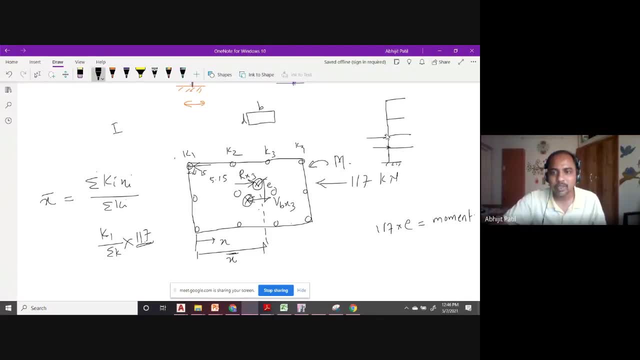 at each floor level, be having some force on that particular column in that particular direction, plus moment okay, and this is happening with every column. so along with gravity load, now your structure becomes a few. uh, even in this scenario also, you can solve the frame. there are some manual methods available. 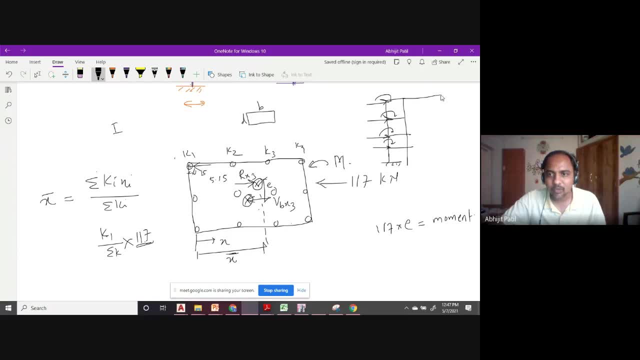 so in x direction. if i take there are four columns here, right, okay, and each column or each joint will be subjected to such forces like this. even this, okay, so you can use any of the, for example, khani's method. okay, so to solve the portal frames, such manual analysis methods are available, so if you want to, 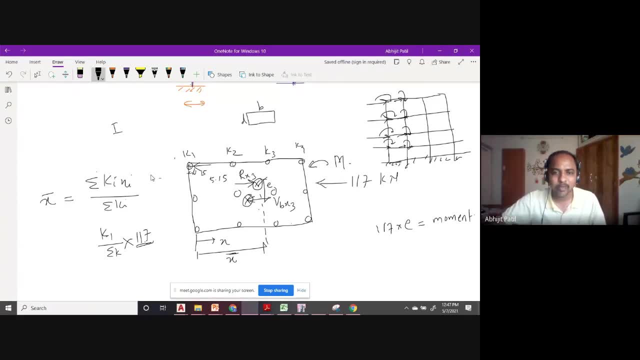 do it manually. you can consider the frame frame by frame. so this first frame, this is second frame and third frame, like that, okay, and you will calculate force coming on each column and you just apply those forces. so this will this will become a structural mechanics problem, or add on structure mechanics. 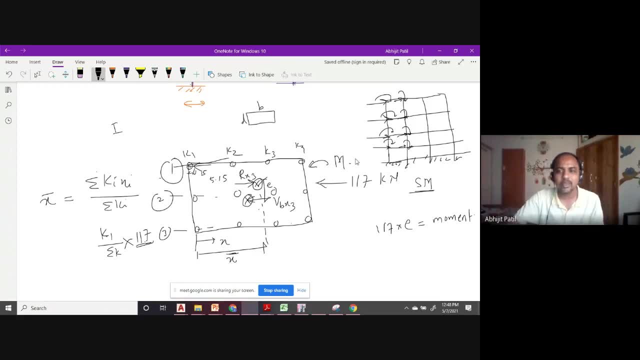 problem and you can do it manually or you can use matrix method, any method to solve. so once you solve that, then you will get what is the moment coming on this, what is the actual force coming on the each and every column or beam. so this is the way to do it manually. okay, any other doubt? is this clear? yes, 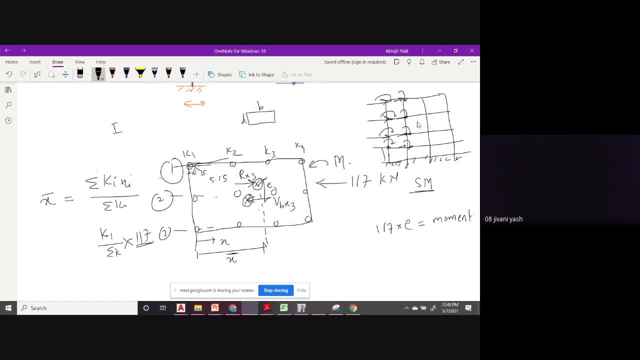 okay, any other doubt? is this clear? yes, okay, any other doubt? is this clear? yes, so any? yes, yes, I mean calculating fundamental time period. so we have to take height from Flint to top of the water tank in case of RCC or no. no, no water tank. it will be from Flint to topmost floor roof level. roof level: yes. 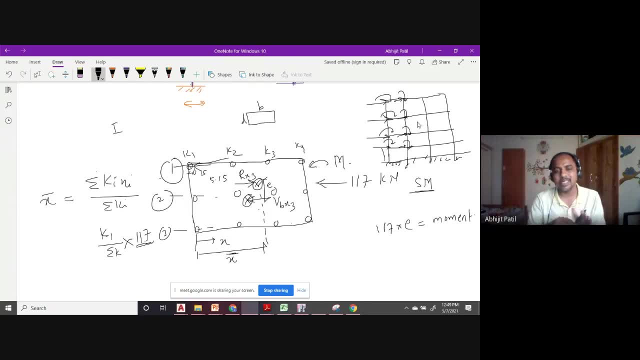 because are the water tank location generally. what is typically what happens. you have a small staircase cap and above that water tanks are pulled, or you will provide a separate structure where the water tanks are put. so you neglect those normal projections because, as compared to the floor level that those projections are very small. 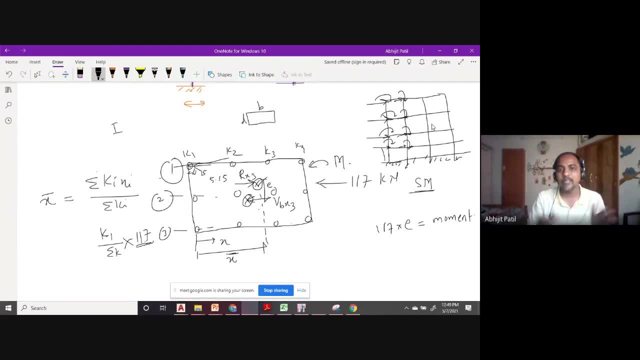 so up to roof is sufficient. but if more than 50 percent part is elevated- sometimes that may also happen that the client wants covered terrace and they want to cover it with rcc, so more than 50 is covered- then that floor will not be called as roof. now the above floor will be called as roof. 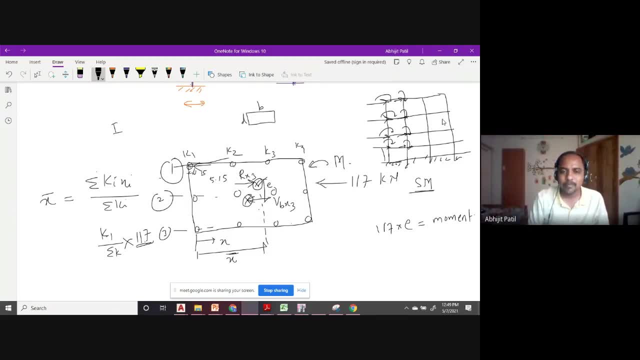 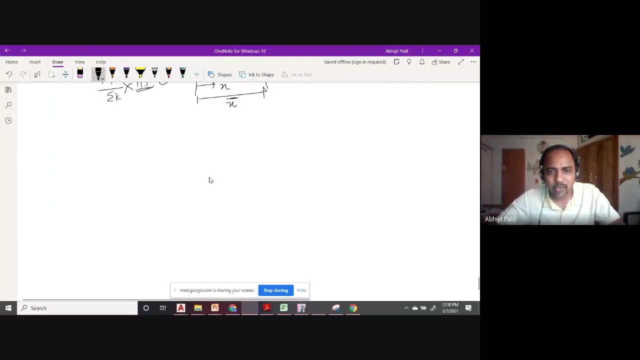 and you have to consider that height. okay, okay, any other questions, sir? yes, in the structuring of irregular shape, then we take the average length and the breadth. uh, of which shape? irregular shape? okay, okay. so for irregular shape, okay, so again, there are different, different possibilities. i will just go with some shape like this: 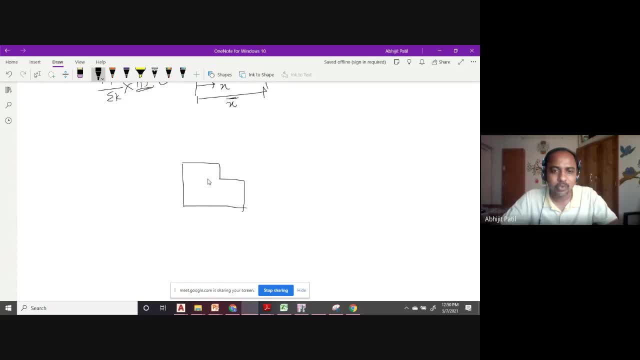 right. so in plan your building is looking like like this, or even elevation your building is looking like this, so you take not average, but the longest. so this may be your dx, and if it is uh, same way but in height like this, sorry, more than 50 percent. 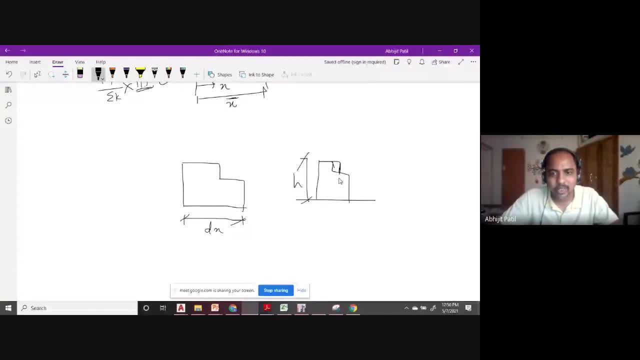 so this will be h, not that h1 plus h2 by 2. no, you take the highest and going further, there can be buildings like this. this is a very special case, it may not happen always- and your columns are located like this, so this is called a non-parallel system. normally, we provide beams and columns in parallel grids. 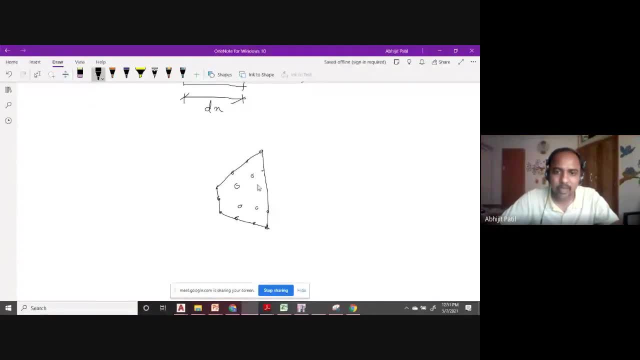 but this is a non-parallel system. you may have some additional columns here like this, so this is like this, but this is not parallel, so this may happen like this. okay, so here, normally what we have seen, that we consider only x direction force and only y direction force. 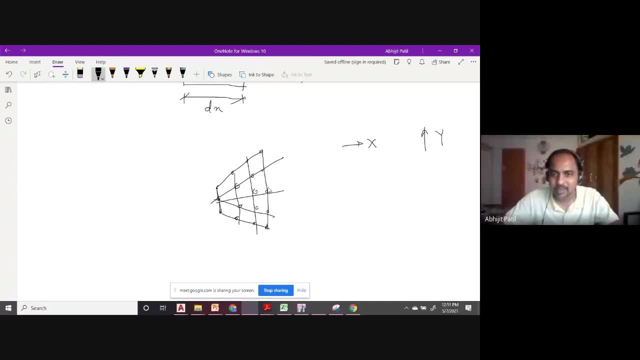 separately in load combinations okay. but in such non-parallel systems, when we are considering x direction force, so 100 percent x plus 30 percent y, and when you are considering y direction force- 100, 100 percent Y plus 30 percent X- you have to consider: 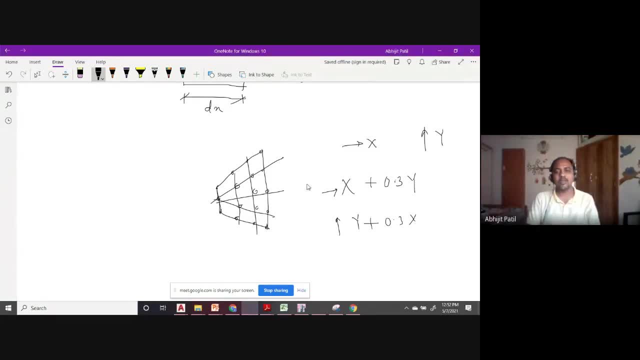 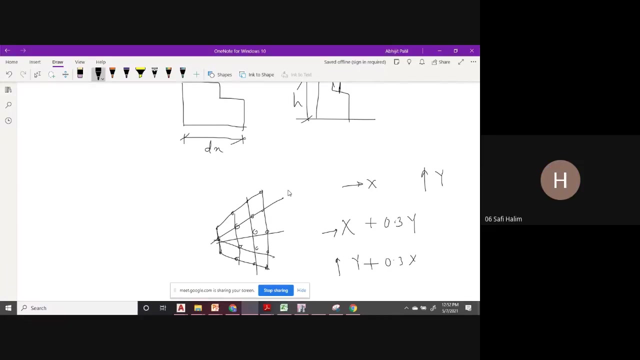 OK, so this is the way you tackle irregular or non-parallel systems. OK, any other doubts? Can you tell us any doubt you can ask? Can you tell me about the other two methods for calculating the process? OK, that is the dynamic method. 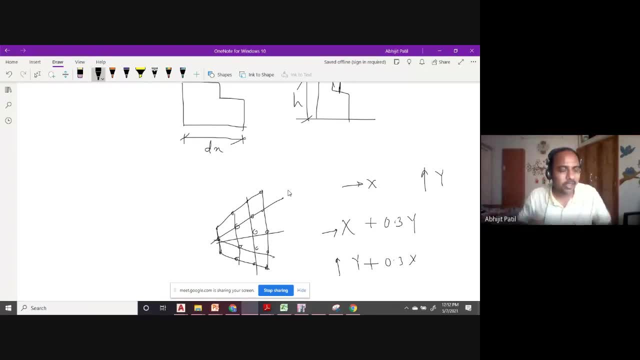 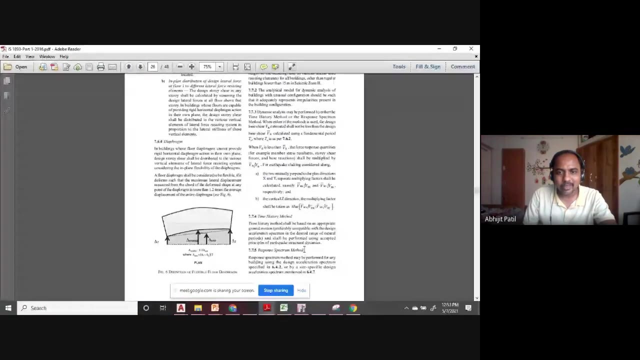 OK, to tell you in brief the dynamic method, that is, response spectrum method. OK, here in code also. Now they have mentioned: yes, we are on that page. OK, so there are two methods: time history method and response spectrum method. 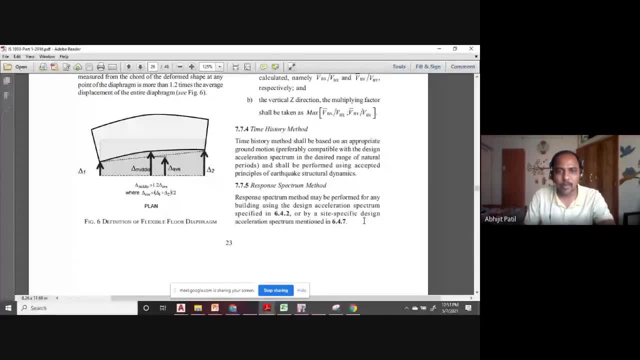 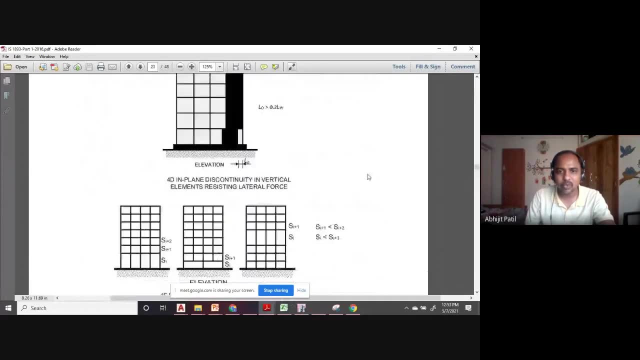 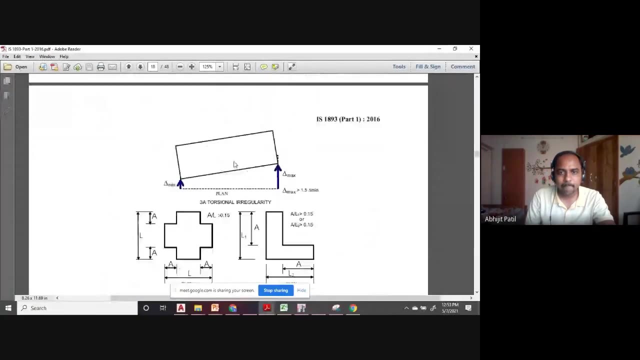 OK, so what is the response spectrum method? Let me see if we calculated SA by G using some formula or that graph. So I will just go to that graph. There lies the difference. OK, this graph. So this is what. 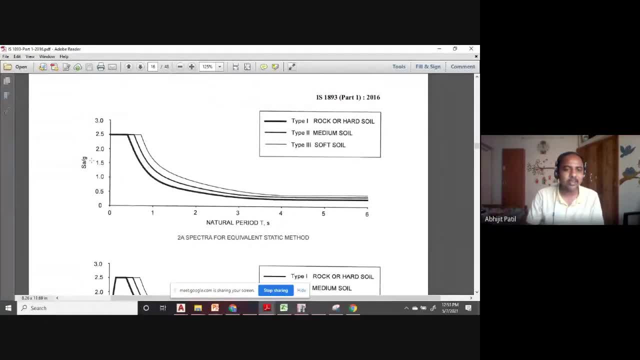 Natural time period, and this is SA by G. So what is this SA by G? This is just acceleration response. OK, that means when, if a particular building is having some time period- one second, one point, five second, two seconds, et cetera- what will be its? 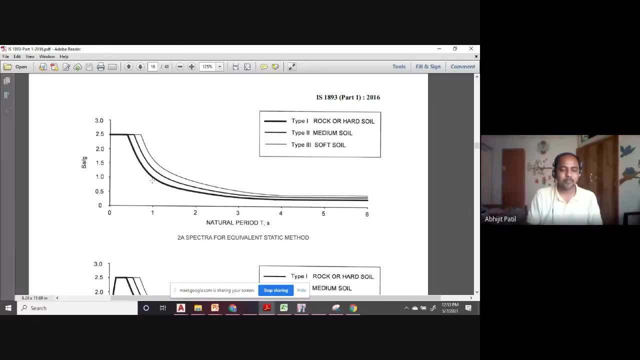 response that is already decided by the course OK, and that decision we are just accepting because it is based on some research. It is not baseless, It is based on some research. but we're designing a very small building. We cannot allow or allow some that much time. 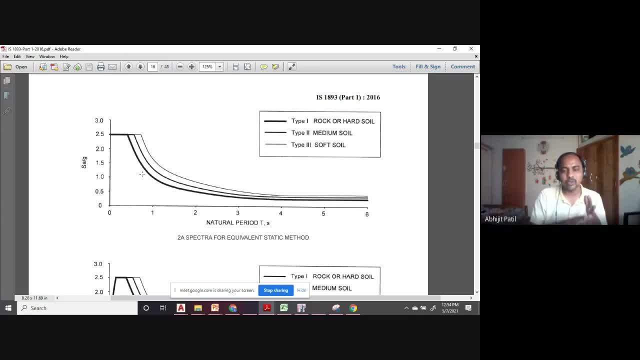 to do, or time also and money also to research, to do the research. So that is why we follow code guidelines. So code is just minimum values. If you want to do something different, you can always do research somewhere in the clauses. It is in every code. 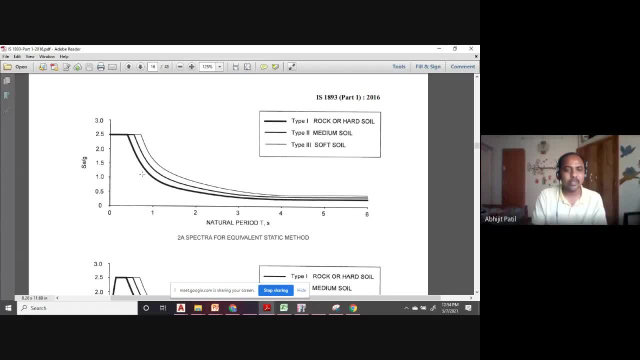 It is mentioned that these are just minimum values. If you want to do something extraordinary beyond this, you do your own research, prove your results and then you can utilize that. OK, So this is what- how this graph is calculated. now by response: 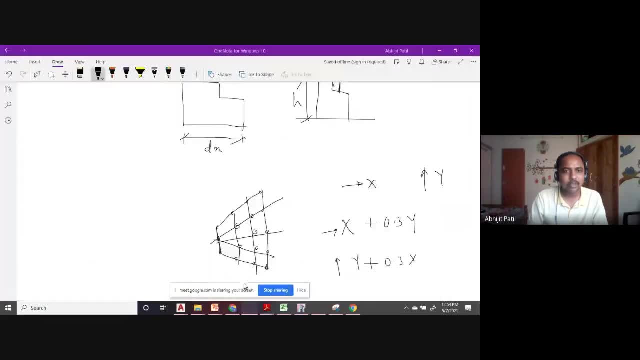 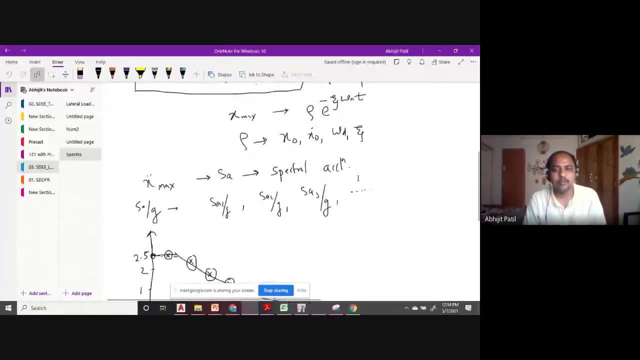 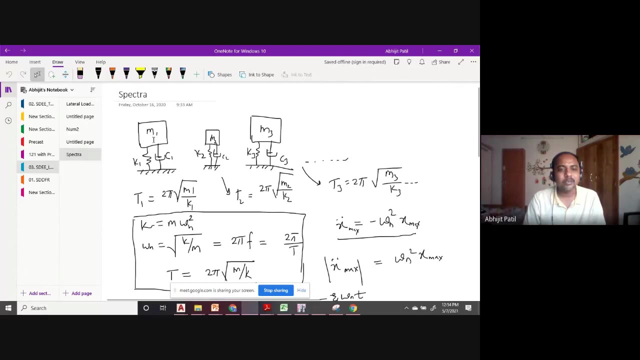 I mean, let me see if I have explained. Yes, exactly. So what? what is done by code? So these are some different differences to know. this spring mass dashboard system is nothing but your building. so having some different properties of mass and stiffness, having some different properties of masses. 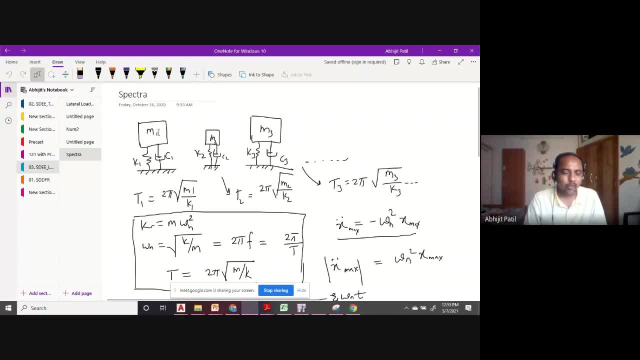 So these are a number of buildings. So obviously, because of different properties of mass and stiffness, the time periods will be different, to be one, two, three, et cetera. OK, and you start vibrating this building. So you just start the vibration. 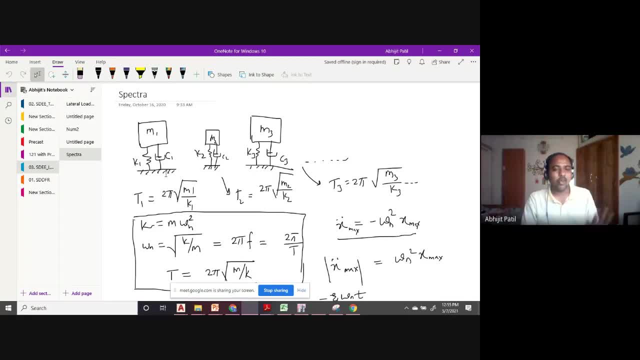 So there is a basic law that if you give vibration to the building, it will give you its own time period. So that is called mass, mass time. And that is what is this: One, two, three et cetera. So you just vibrate that and calculate what will be the maximum acceleration. 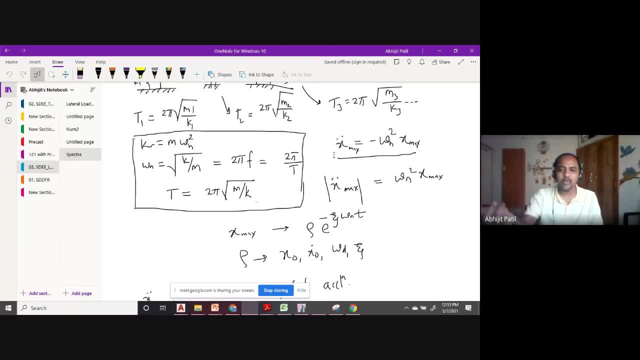 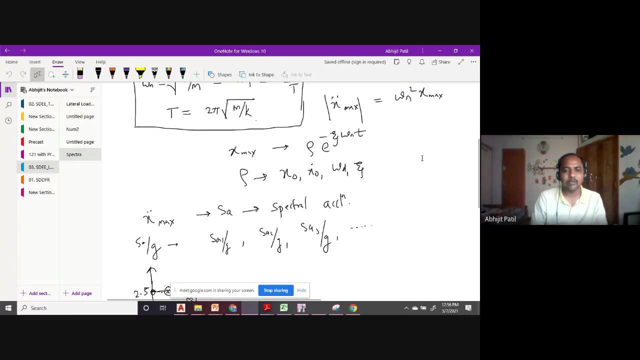 OK, so we can do this theoretically also, or we can do this in lab also. What code has done? It has done this, and this will be the maximum acceleration. OK, then there is a concept called spectral And absolute, So I will not go into that. 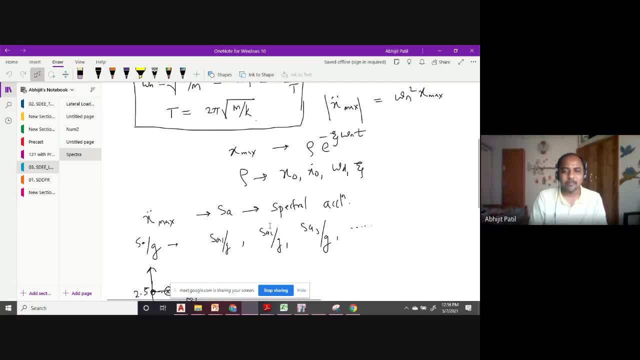 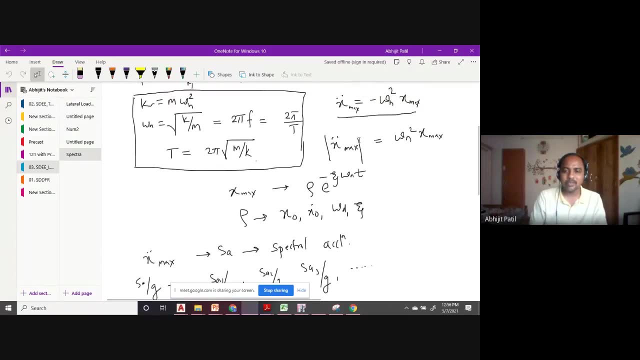 But you record the spectral acceleration, Maximum spectral acceleration of that building. OK, so always the acceleration and response, they can be interchanged. OK, so you just go on doing this. vibrate the building- record maximum acceleration. vibrate the building record maximum acceleration. 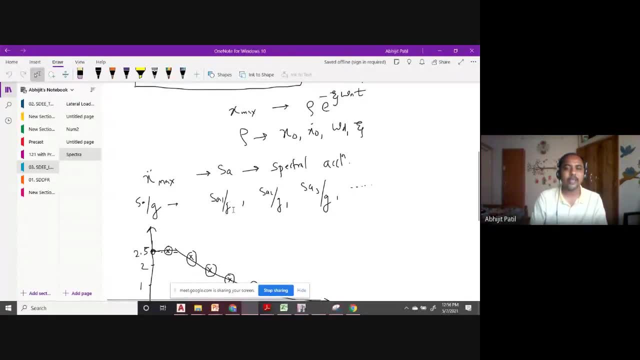 Divide that with G, The acceleration due to gravity. OK, and you just go on plotting. So for time period T1, this is the value of a time period T2, T3, T4, like that, And for different, different foundation. 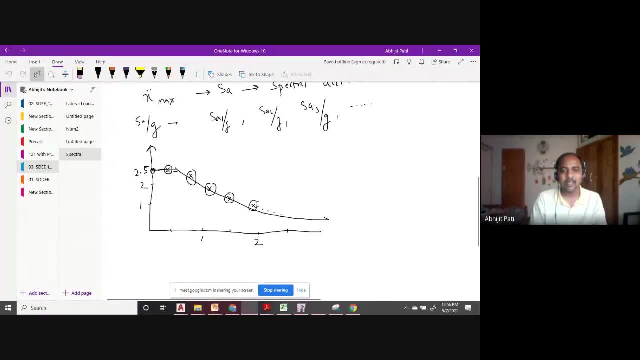 strata condition. you just, they have just calculated this data, large amount of data, and then this pattern is found out: OK, and this is what we call it as spectral, OK, response spectra. So this is standardized and we use this for our building. 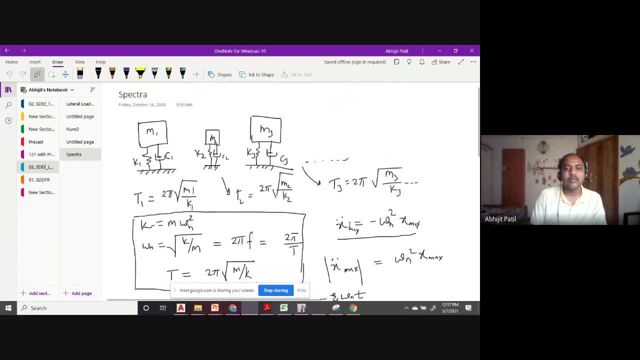 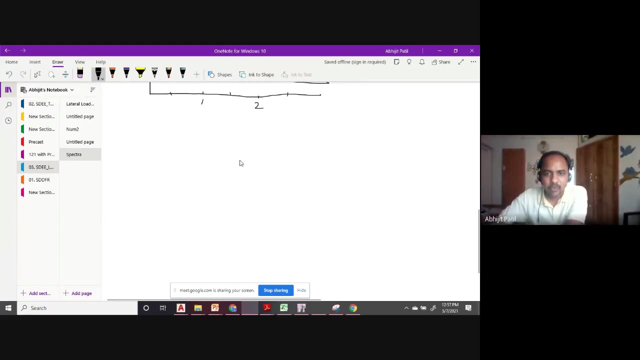 What is assumption here is static method, that building will vibrate only in that mode, only in that one direction. But If you consider, Let's say, two storage, three storage, If I will just Demonstrate, Suppose you have three storage building. 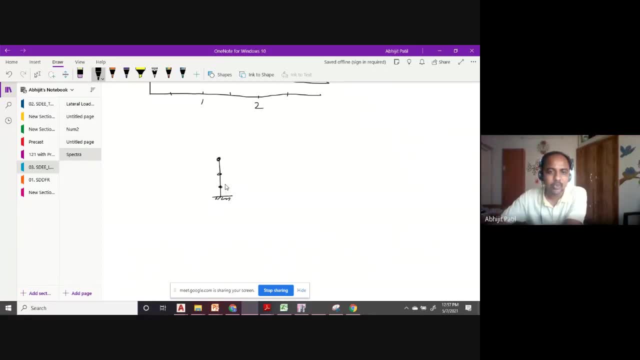 OK, so this is usually denoted. So this is first storage, second storage and third storage. So how will you vibrate in first mode Like this, that we have seen these masses, because they are different masses now, so they will move like this: 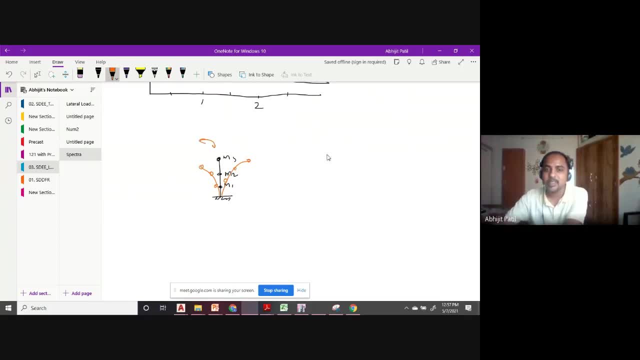 OK, so this is my first mode of vibration, But it is not the only mode. It will also vibrate in this direction, So suppose this is the main position. OK, so what is the difference here? Here you see the mass: M1, M2, M3. 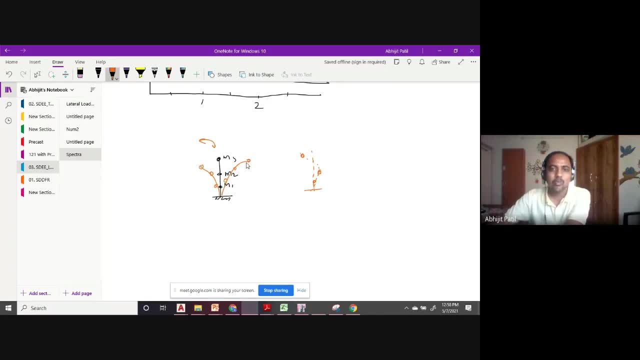 They, at a given time, they are all in the positive X direction, Then they will all achieve the main position and then they will go to all together. We go to negative direction. OK, so positive, negative, They are always in the same phase. 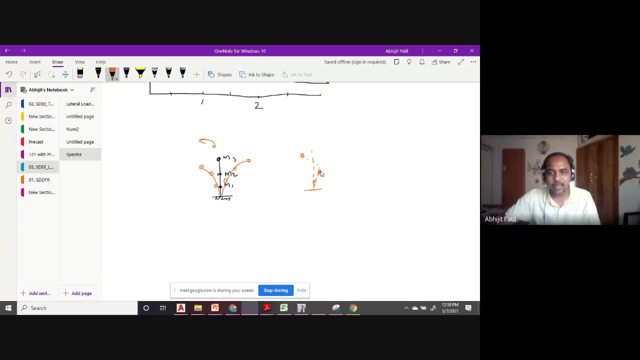 This is called a phase of here. in this case, What is happening? So few masses are going in positive direction and few masses are going in negative direction, And it will be mirror Like this. So when this mass goes here, this mass will go here. 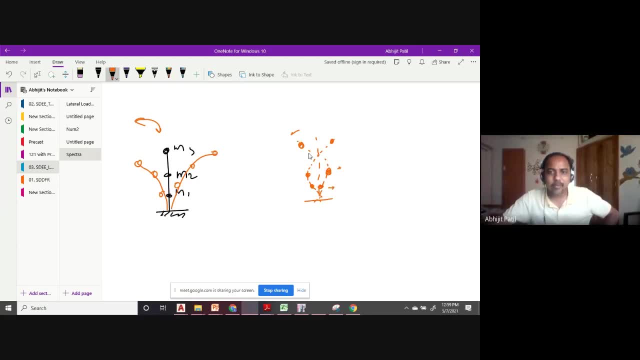 But the other ones are there. So this is happening. So this is the way it is vibrating. So this is called as the first mode of vibration. This is called a second mode of vibration Then. so what is the another thing? this: there is one point where the building is. 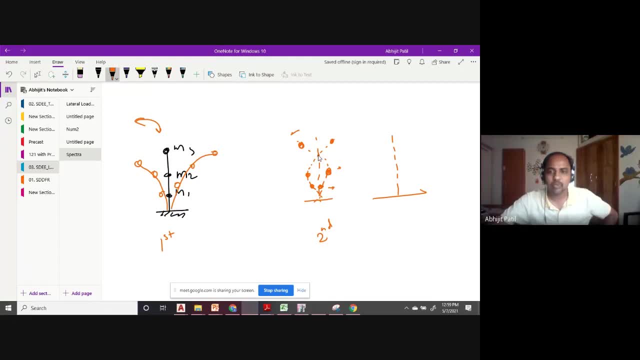 not at all vibrating. This is not leaving its main position. So this is the identification of second mode. So number of mode minus one is the number of neutral points. So these are neutral points. So here it will be third mode. There will be two neutral points. 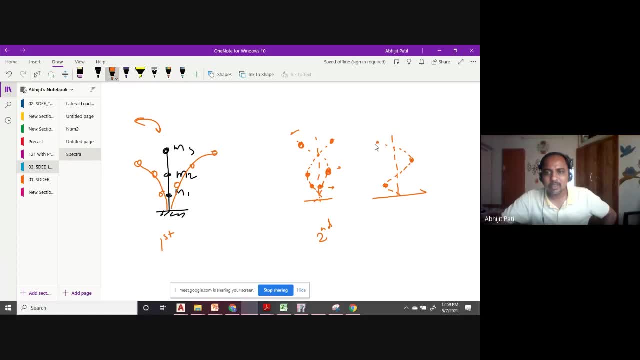 So maybe the mass is here, Mark is here, And OK. So this is the extreme position in negative direction, extreme position in positive direction. So when this mass is here, this mass is here and this mass is here, Or the other way. 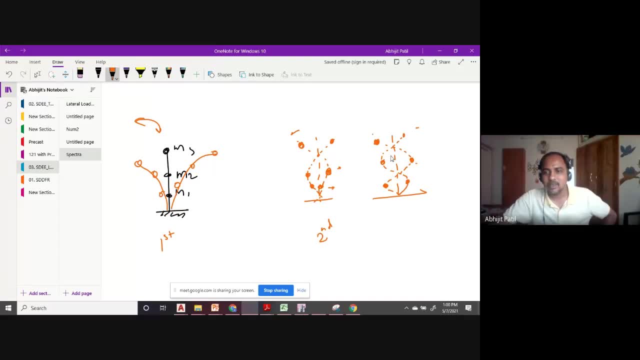 So nobody is seeing each other, They are out of it. And here the points are two. This is your third mode. OK, So this is called as only three masses are there, So maximum three modes it can achieve in particular direction. So this is the next direction. 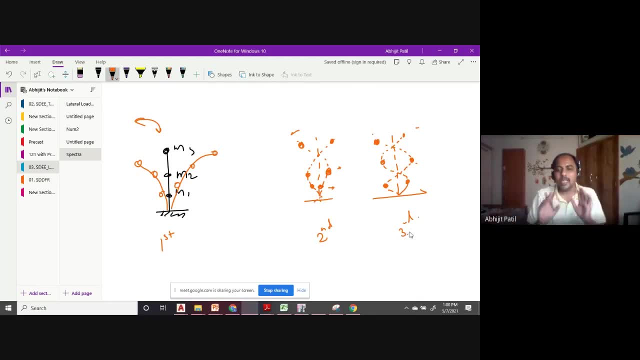 Same thing will happen in Y direction. OK, Have you understood these modes of deformation? What equivalence static method does is that it says, or it assumes, that building will vibrate only in this fashion. It will not vibrate in this fashion. Maybe they will be in same phase always. 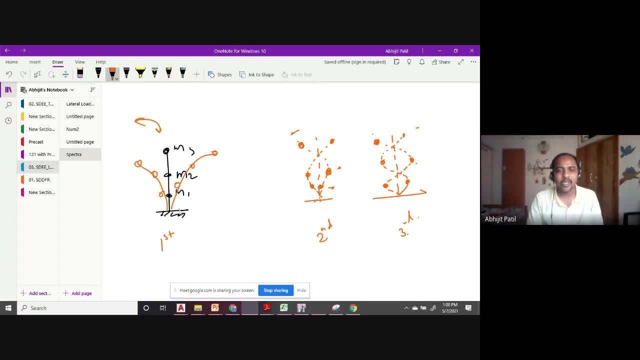 So that is the basic assumption in equivalence static method. So that is why we distribute the force using that parabolic formula. But in actual case there can be out of phase, second or third mode of vibration. So to capture that we are using the response spectrum method. 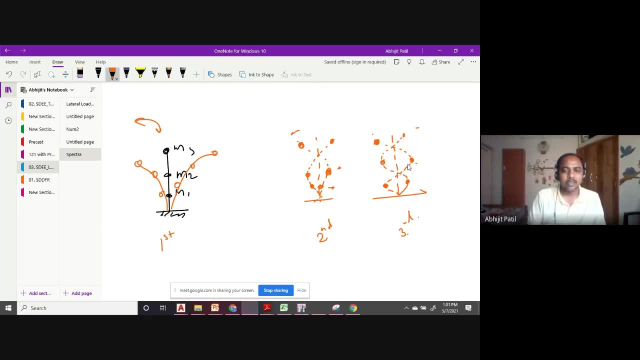 So what response spectrum method does it combines? It will not only calculate for first mode, as we have done in static method. It will calculate what first, second, third or whatever number of modes we desire. OK, so up to that modes we can consider. 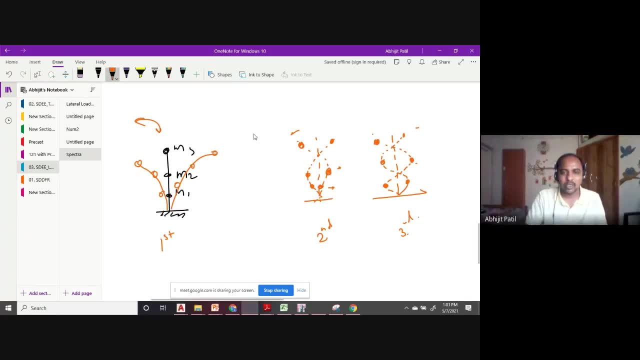 And then we have to combine those results together. So the earthquake force here at this story level, Let's say Sorry, we Be X, OK, now it becomes complicated. now at floor level three and more than one. OK, And this would here it will be: we be X at floor level three and more to. 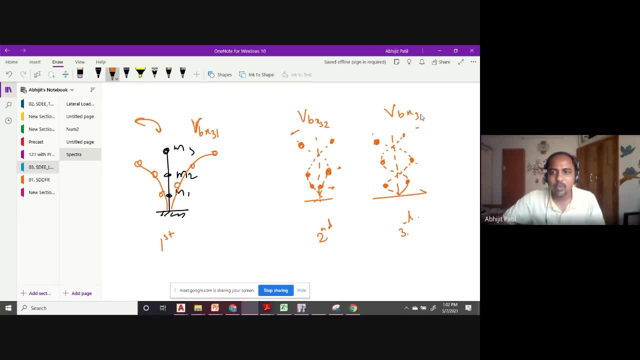 And we be X at floor level: three more three. OK, so we were having just only we be X, three. Now we are: we be X three, one, two, three, And then we have to combine these three. So there are also some standard methods, SRS. 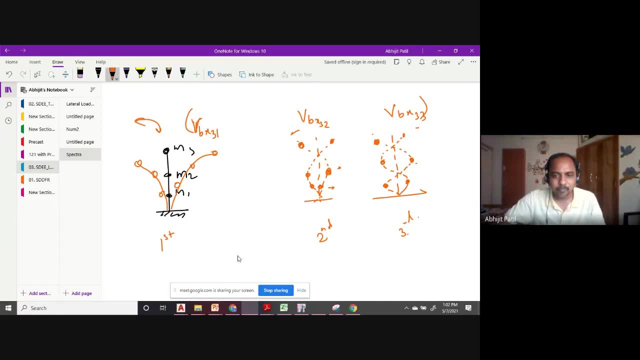 So what is SRS? is some of square roots, So we be. I will just write Now: one square plus two, square plus three square. If you are considering more than number of modes, then then And just take the square, that value, add all those values and take a square. 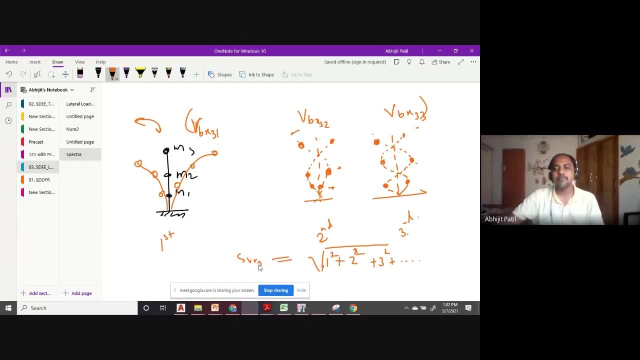 So that way you get the VB X three OK. so there are again different combinations, So this is the way we are Dealing in response spectrum with it. So this is dynamic method, Although we are breaking down and simplified it to a static method. 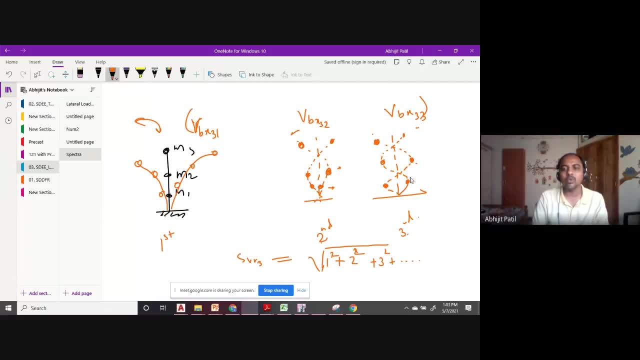 But we consider dynamics by the help of these modes. OK, so modes are nothing but the way building will vibrates, And these are standard modes, be it a building or be it a string of a guitar. This is very natural. This is the way it vibrates. 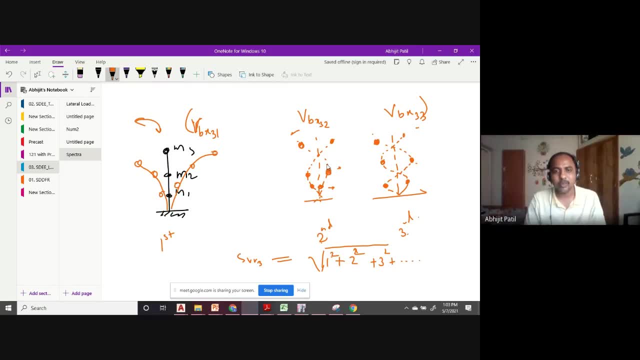 OK, so This is response spectrum, And what is time is the method. So in time is the method. We consider one earthquake record. So in each and every case here we have considered only one particular value of best year. the best year value will not change. 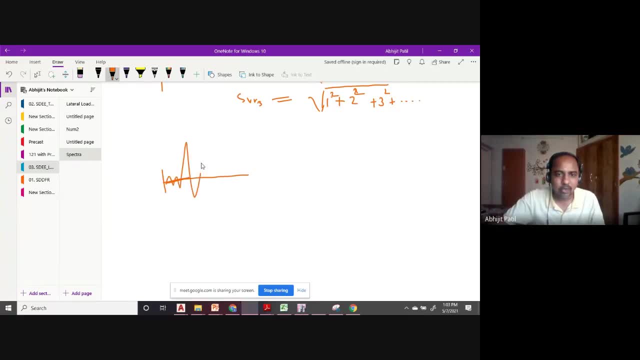 But here We know the records of earthquake are like this. So at each and every time second the value of earthquakes will be different. OK, so the forcing value is different And we analyze that for each and every time period. So we have to consider the delta t at what time interval we are going to analyze. 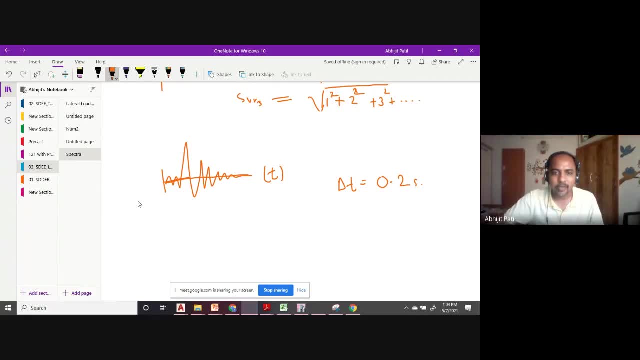 So let us say I'm going to analyze that point, two seconds. So I will divide this at each and every point: two OK, and I will know the value of this is the value of earthquake force. Then I will analyze our structure, The structure. 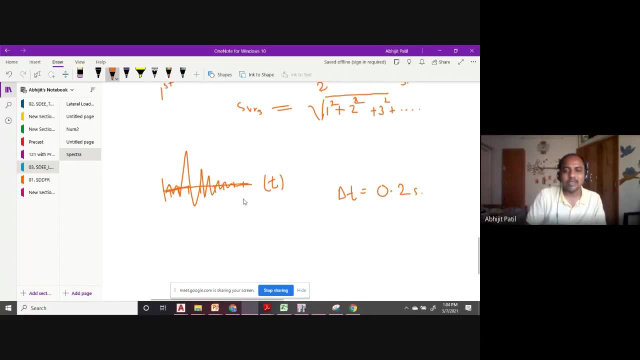 Is deformed by some value. OK, so in our response spectrum method or static method, the structure is not deformed. OK, it is at a stationary position. But here, For first step, it will be in stationary position, but for second step, 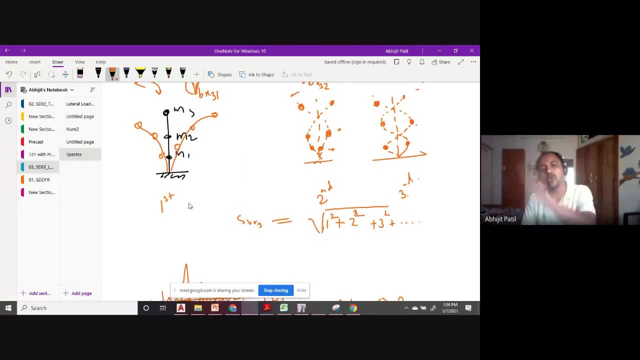 the structure may be already deformed, and from that point onwards we will have at: So T1 is zero seconds, T2 is one, two seconds, T3 is point four seconds. So here maybe earthquake force is also zero. So no deformation here. 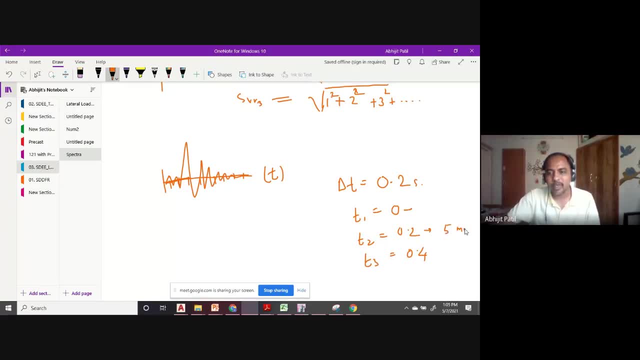 There will be some deformation. Let's say the structure has deformed by firemen. So when we are going for next step, the structure here is already deformed by firemen. And then we apply this force at T3 equal to point four seconds. 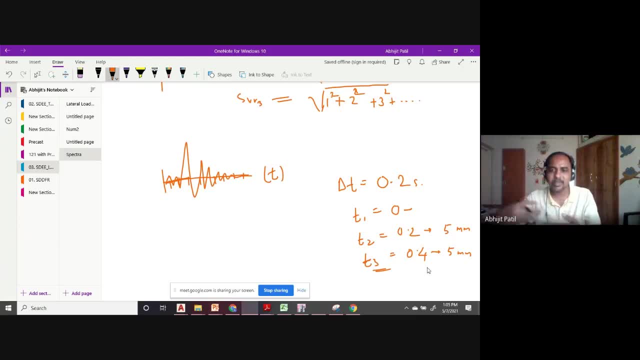 So, likewise, this is One step, step by step, step by step, This analysis and this is. you can see how complicated it is OK. so if your total time is to, this is called as time history. if it is divided into a hundred parts, you have to analyze your 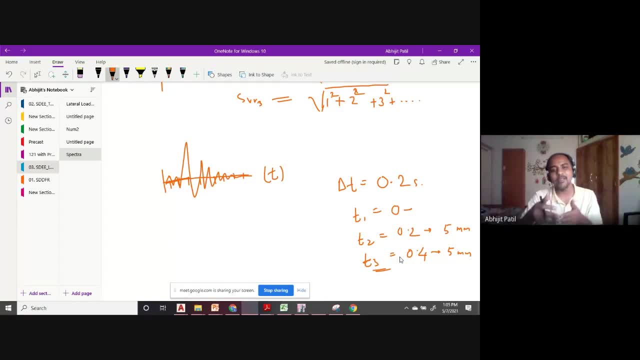 structure for a hundred times and then again combine the results to get the maximum value. OK, so this is called as time history method and this is more rigorous, more accurate. So this is generally used for very critical or important structures, not for buildings. 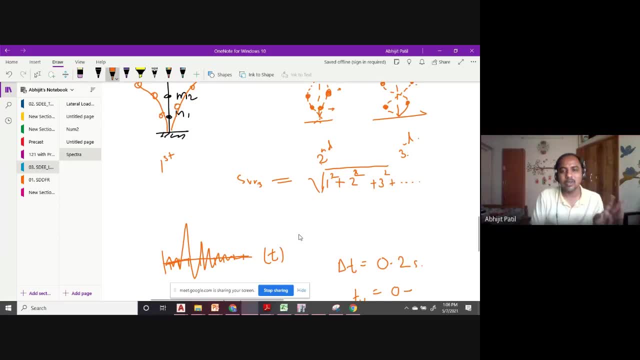 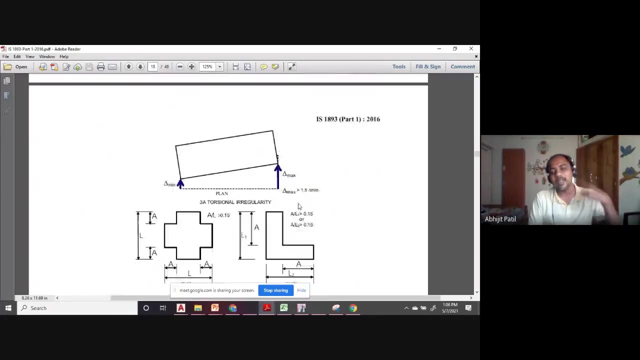 For buildings. we can go with static method or now the board has made compulsory to use a response vector method. OK, so these are the. of course there are some other methods, also push or analysis method, so that will be again very advanced topic. 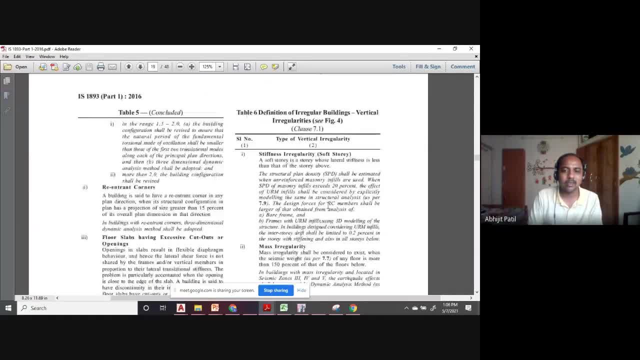 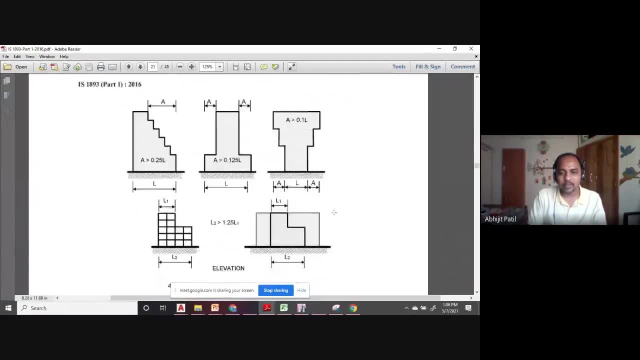 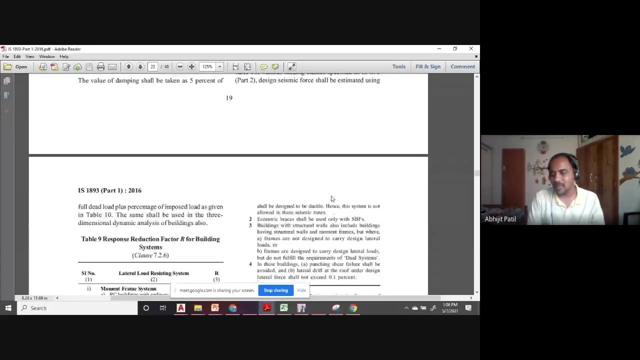 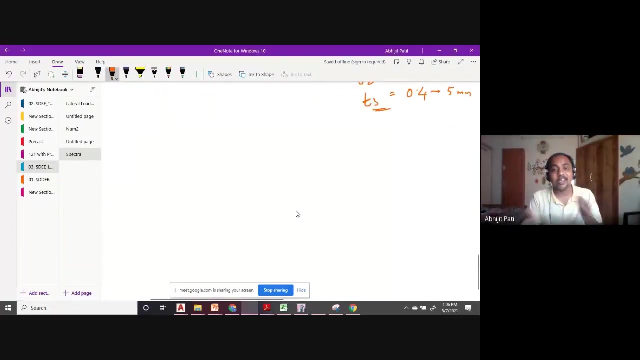 You have a new board coming up for us is design, called as performance design. So there you require that push or method, The freedom. OK, we don't have. very simple. That is also nonlinear. Yes, that will. Yes. Again, linear and linear, that is different thing. 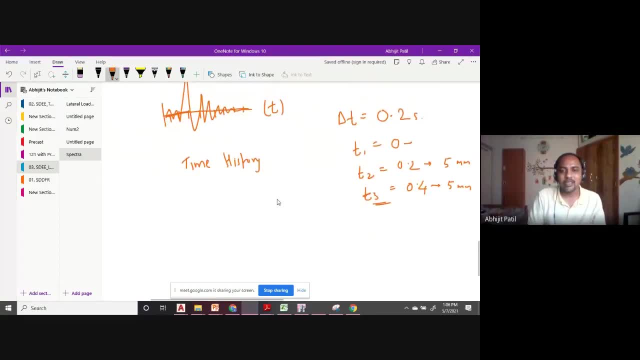 I'm just thinking of setting and dynamic. OK, so these, all these methods are linear, static as well as dynamic. but linear methods. Linear means what we consider, that the material is in linear zone. Elastic- Yes, elastic, That means if I apply a load, it will deform. 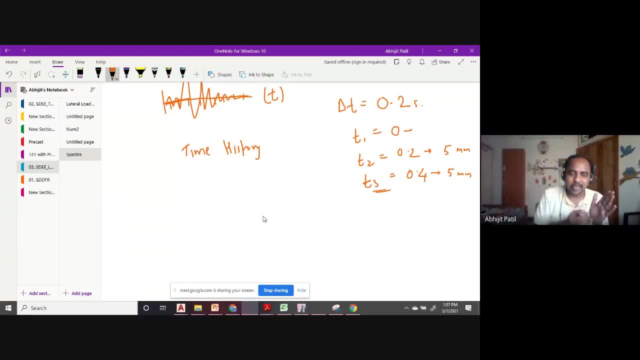 If I take away the load- take out the load- it will again regain its original size and shape. There is no permanent deformation. under these assumptions, All these analysis are done. The push or analysis or analysis, though those come under nonlinear analysis. 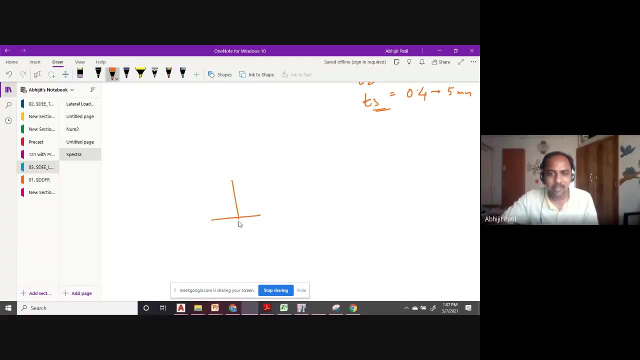 Speed delta is again a very simple. I will just explain the concept. We have this column with some Load and we also have some lateral load because of earthquake. Let's say it is we. So when we analyze using any static or dynamic method, 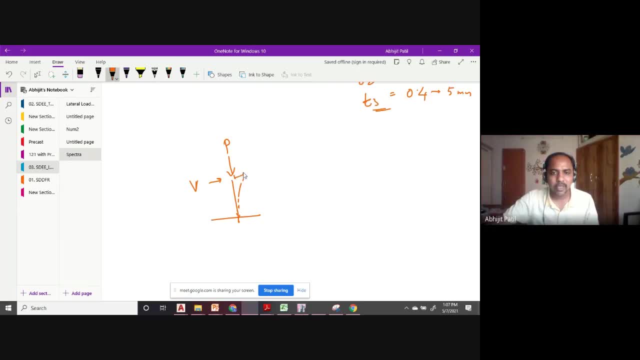 We say that it will be formed by some amount known as Delta. OK, now the new thing is: So this was the original, but now it is deformed like this: In case of earthquake, Now this actual load is acting here and this force is acting. 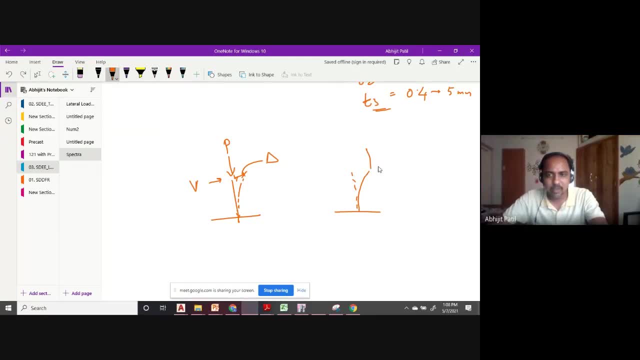 OK, not the case. OK, so the actual load is acting here and this force from here to here, we can transfer, but we have to transfer this actual force here. So how do we transfer? This is deformed by Delta. So if you remember the rules of statics, we can transfer any force. 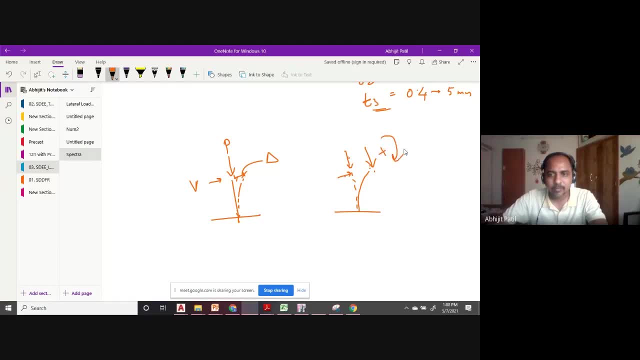 By actual force plus A movement, and this movement will be equal to the into Delta. OK, so this additional movement is acting on this call. So generally, what is done? this is not very of high importance In case of short columns. short columns means L by D or L by B. ratio is less than 12.. 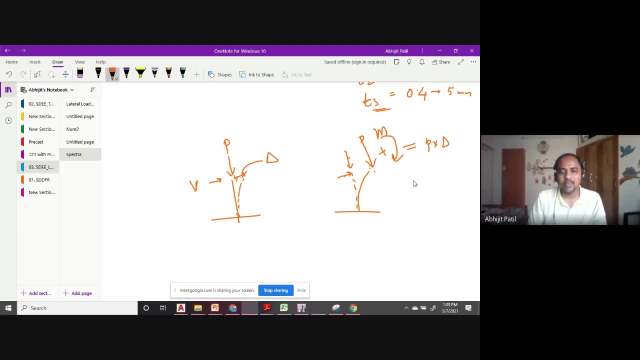 OK, but it is very important in case of long columns. So we have in IS456, we have two options: either consider additional movements in case of long columns by using some empirical formulas or charts given in IS456, or there is another option. This is called a secondary effects. 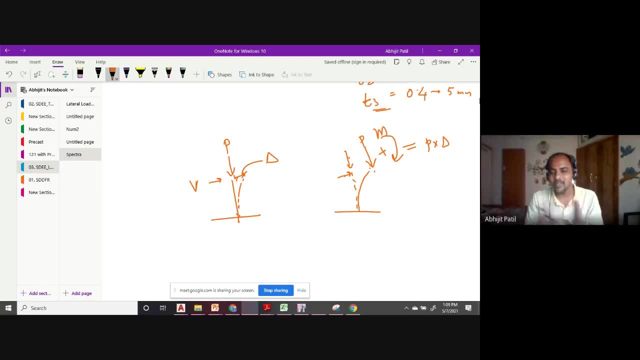 You analyze your structure By using this: secondary effects. So the secondary effects are nothing but this, leader. So you now have to consider not only actual force and the lateral force. You also have to consider this additional moment because of this, during earthquake, When it is deforming. 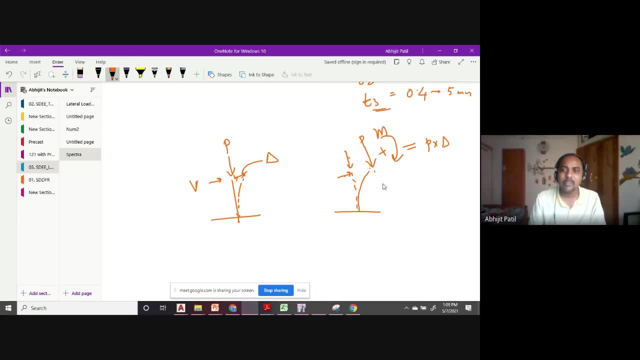 So it is subjected to actual force, but also some additional movement. OK, but it is not a single step analysis. So you analyze this and then you will find That because of this additional movement, it is going to further deform, like this: 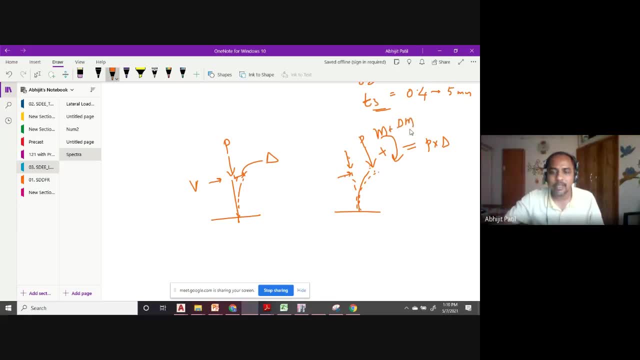 So again, some small additional movement will get added, So you have to use iterative methods to find exactly how much movement is added. OK, and again, this lot of softwares are providing this option of doing the analysis. So this is the basic concept of 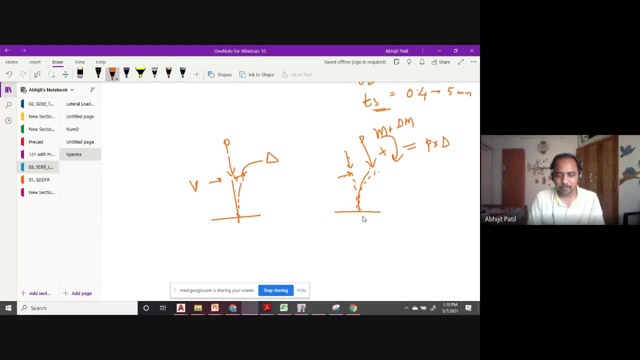 Delta analysis. Any other queries? So how do I think the vertical forces would work? Vertical forces: OK, so vertical forces basically see the effect of. Again a very good question where I will explain where exactly it's critical. 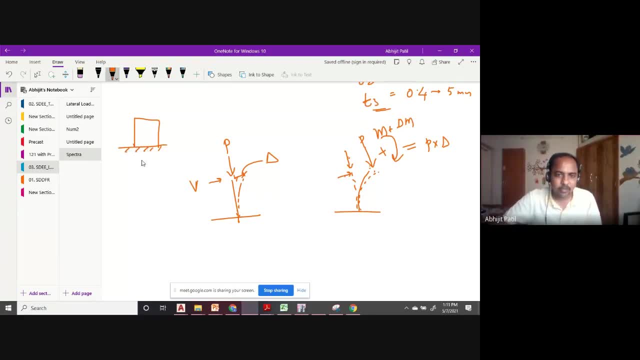 So we have up to now seen horizontal forces. So vertical force will be like this: OK, so it will be in upward direction or downward direction. So when the vertical force is in upward direction, the already gravity forces are there here, right, they're acting downwards. 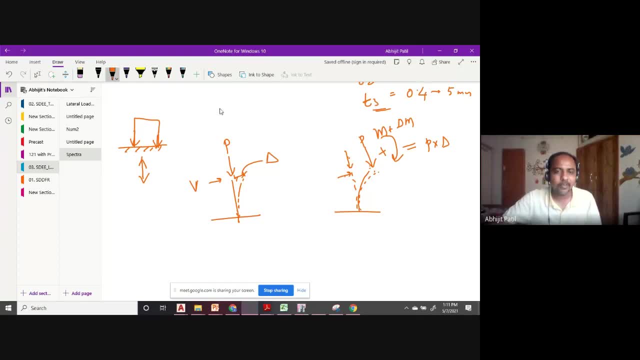 So they are. But because we know that force now, we calculated one zero, four times the weight of the building's, weight of the building, so approximately four percent. So four to seven percent or two to seven percent is the range of earthquake force. So you can see here. 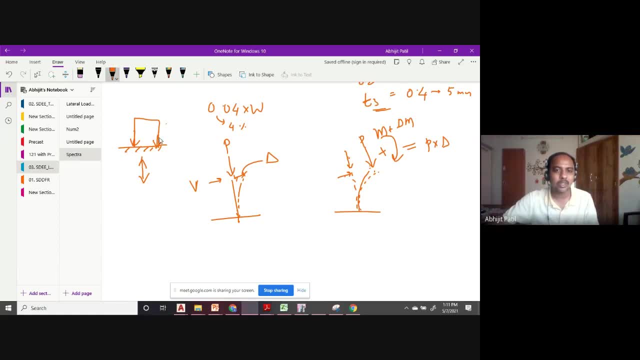 a hundred kiloton force is coming in here. only four kiloton of force is coming, So there is no problem, We have taken care. You say, but I don't know You're talking to get to a hundred. So it will take care of that force. 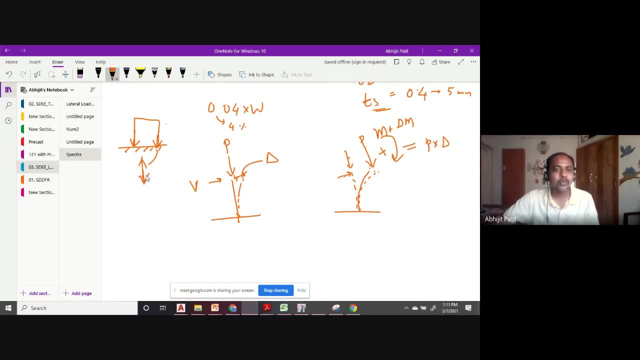 But when it is acting downwards, when it is acting downwards, this will impose additional gravity force. So instead of one hundred, we have one hundred and four. now, OK, but we have tackled with that. by what course is, you can consider, almost. 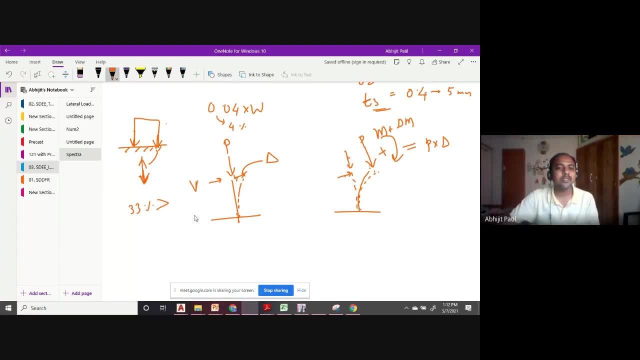 Thirty three percent more for invisible stresses in case of earthquake. OK. so coaxial load of problems the issue, but Foundation, OK. so this will impose additional load on the foundation and the bearing pressure. suppose you have designed cut to cut. two hundred kiloton per square meter is the bearing pressure and your 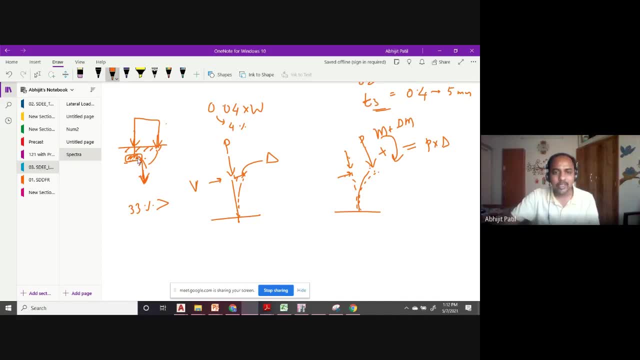 footing size is such that you achieve two hundred. So in that case, what course is, in case of earthquake forces, additional 30 percent permissible stresses are allowed. That means in case of earthquake. So thirty three means hundred. cut thirty three, two hundred. 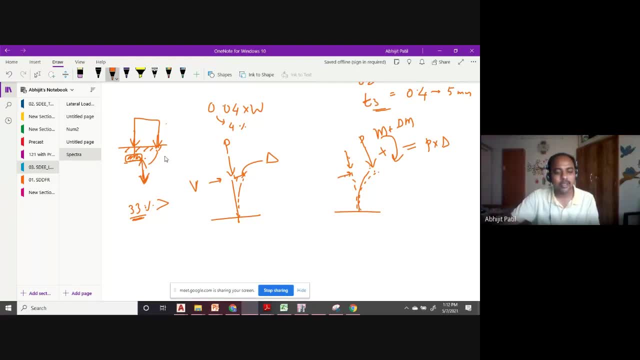 So it will be two hundred and sixty six kiloton per square meter pressure is allowed in case of earthquake loads. So this is how we consider the vertical component of earthquake. But the problem is that means there is no problem in normal buildings, But the problem is in the case of cantilevers. 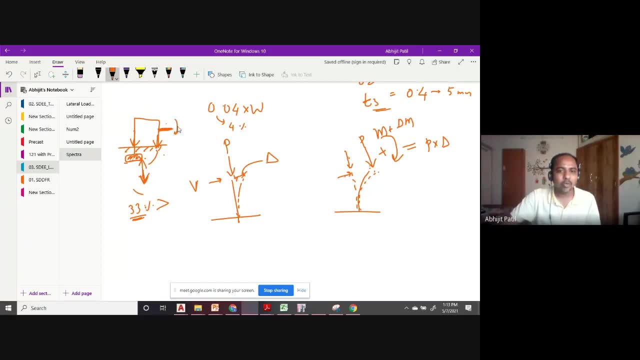 OK, so in cantilevers this vertical component is very dangerous. So what course is designed this cantilevers for a force equal to five times the vertical earthquake force coming? This is so dangerous. that is why the cantilevers need to be designed. 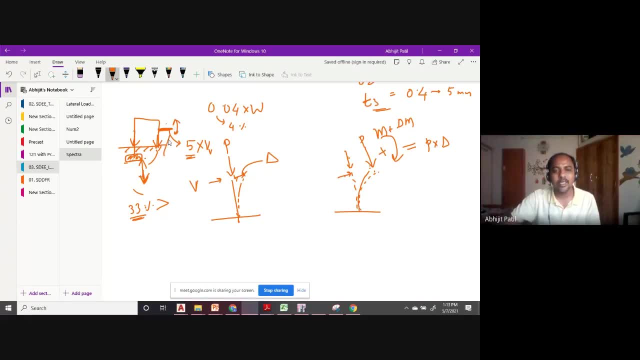 five times more the earthquake force. so that is the only part of concern in case of vertical the cantilevers, Otherwise the court takes care of the other. We did not apply a separate vertical earthquake load for analysis, only for it is that. 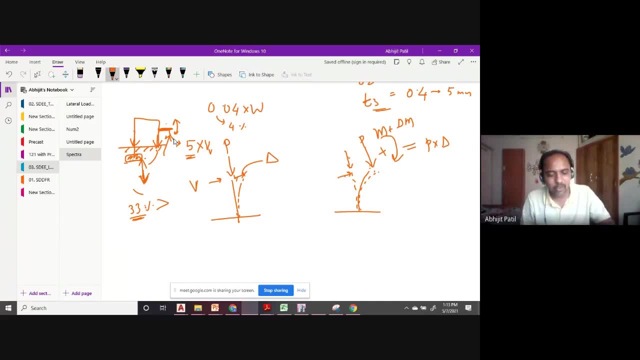 cantilevers- OK. another question, Sir: yesterday, yesterday, you saw some star marks in the convergent and different boundaries. Yes, star marks, OK. yes, sir, Was that the point of focus of our original earthquake? Yes, yes, yes, yes. 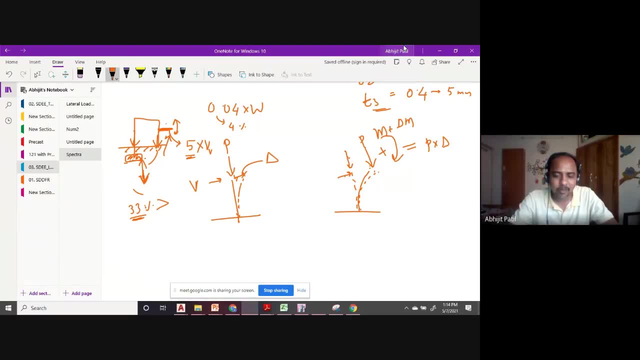 See, the focus is what is deep inside the body of the earth, where the actual rupture starts. Look at that point, because we measure The on ground points. we measure by using latitudes and longitudes. So the point exactly vertically above that focus, we call it as epicenter. 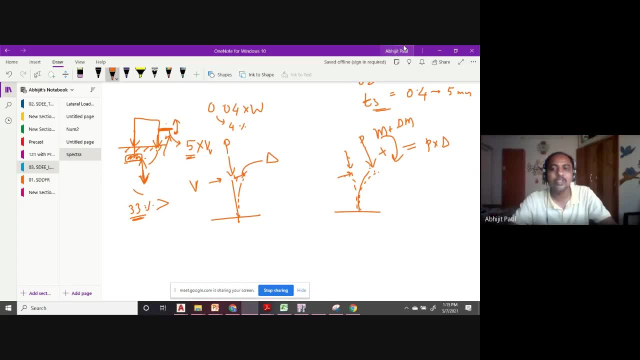 So we never say that Bhoj is the focus. We say that Bhoj is the epicenter of the earthquake, because that is the way we identify on the ground and at that lat and long going down. So let's say then the additional data is mentioned- that below epicenter, at a distance. 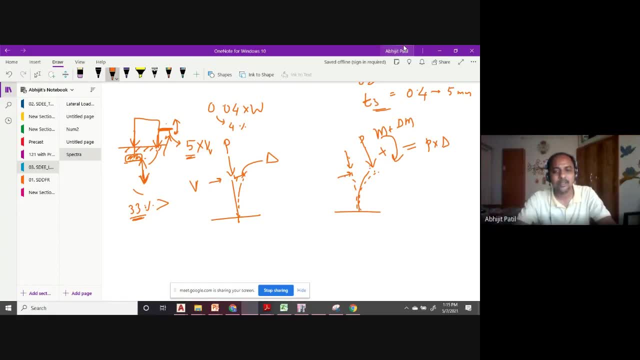 of approximately five kilometers. the focus is located- OK, so this is just terminology: focus and epicenter. So focus is the actual point where that rupture or slippage has occurred And that was the star shown in that particular image And the same magnitude will be in the Bhoj and Ahmedabad, or different magnitude. 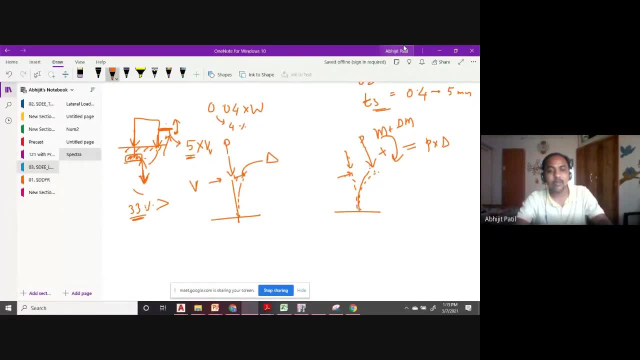 Magnitude? yes, Good question Again. I missed that And I was telling the difference between magnitude and intensity. See, magnitude is measured, particularly the research. Magnitude is measured, It is particularly logarithm of maximum amplitude of P wave. 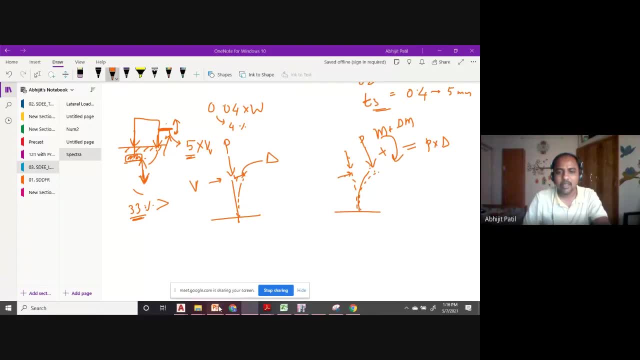 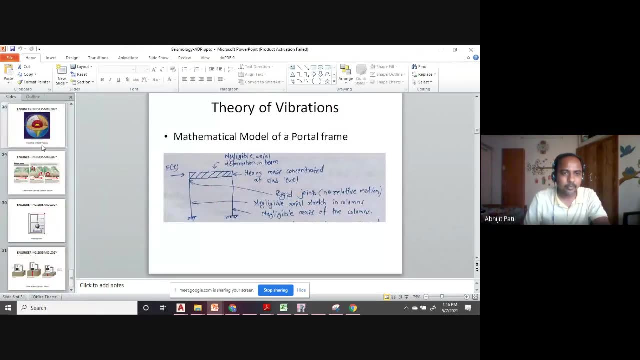 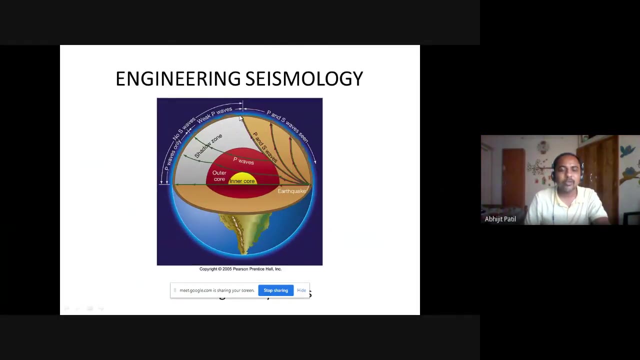 OK, and if you remember that, I can show that graph in the presentation. it was there. OK, so this P wave, it has been generated from here, So the P wave properties will not change throughout. It will remain same on the surface when we measure it. 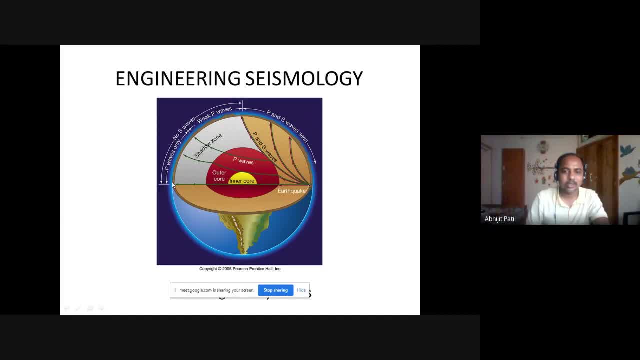 OK, so suppose this is US and this is India, because technically we are exactly opposite on the surface. so when earthquake happens in US and one of our centers, this small graph records it here, and one is somewhere in Europe, let's say So, all these three values will match. 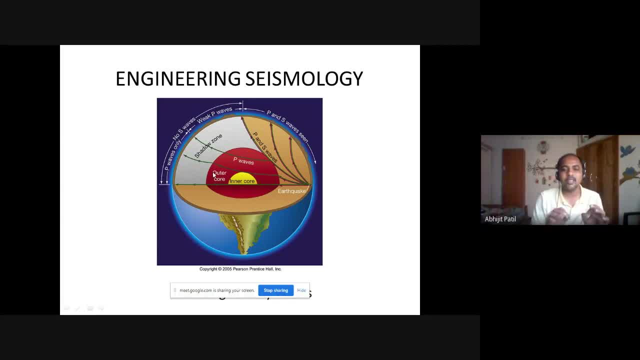 Because everybody is measuring the P wave. So magnitude of the earthquake will remain same, irrespective of the location on the Earth's surface. OK, but intensity of course it will be. very lot of damage will occur near this epicenter of focus, But here no damage at all, or even people. 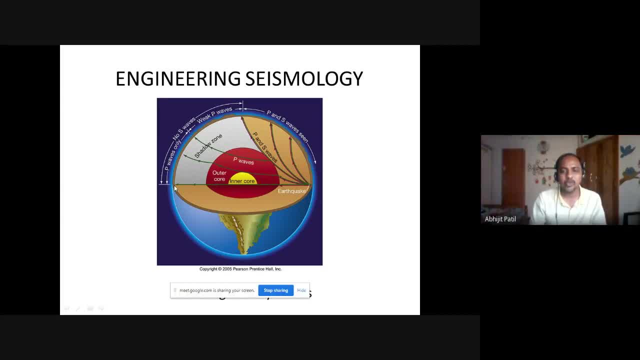 human beings have not felt the vibrations at all. So intensity will be zero year and it will be maximum year And usually it will go on. It will be increasing as you go away from the epicenter. OK, so remember, magnitude is always for any given earthquake event. 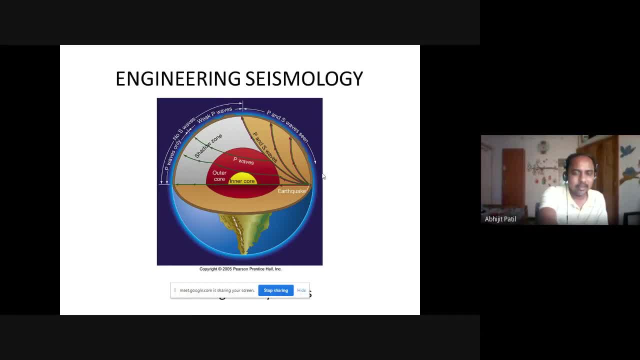 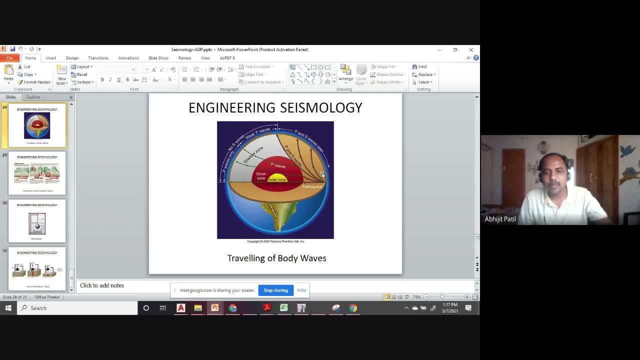 Magnitude is constant. It will not change. Yes, any other questions? So one more question, sir. So in the IS core you've shown that three different types of soil- hard soil, medium or stiff soil and soft soil. Yes, 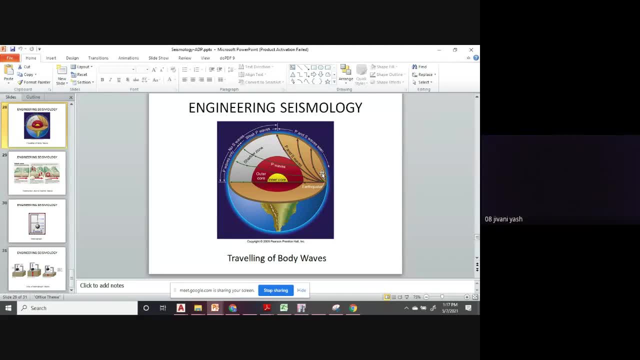 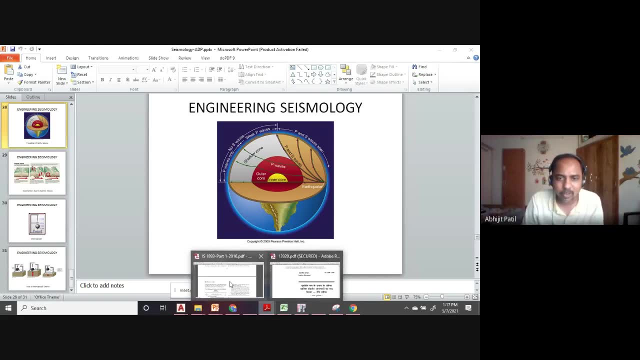 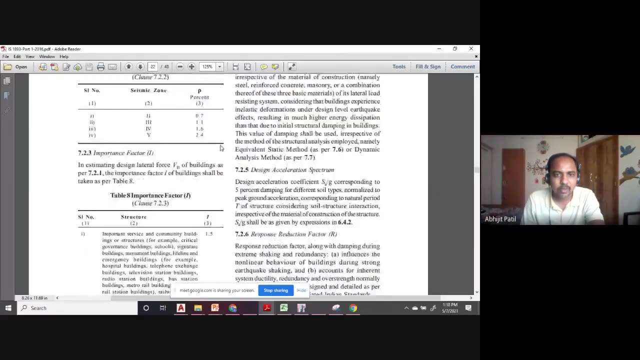 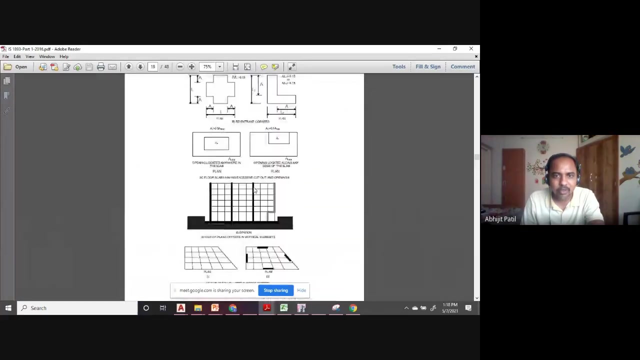 What is the basis of this category, of these three soils? Is it SVC or N value or something? Yes, that that is given here. It is dependent on N values. One table is given exactly Basically it depends on the N values. 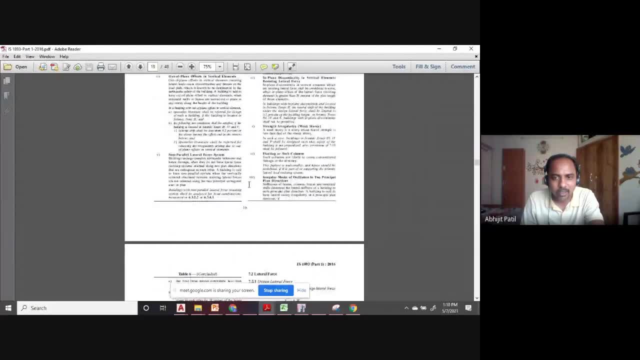 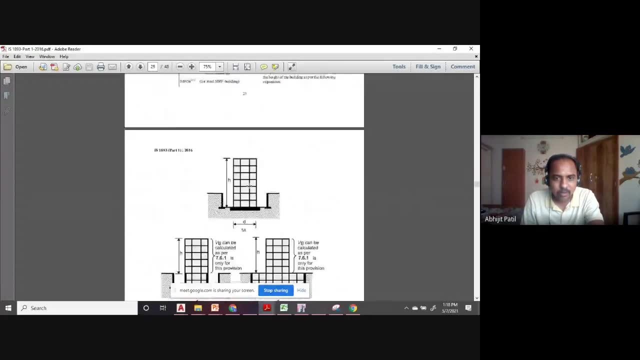 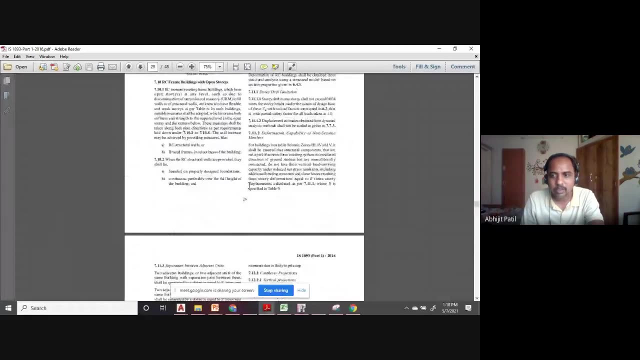 So in the case of, for instance, there's a portion of the N value. it depends on the temperature. It depends on the temperature of the soil. So it is not decided by the temperature, It is determined by temperature, So it can be defined by the temperature of the soil. 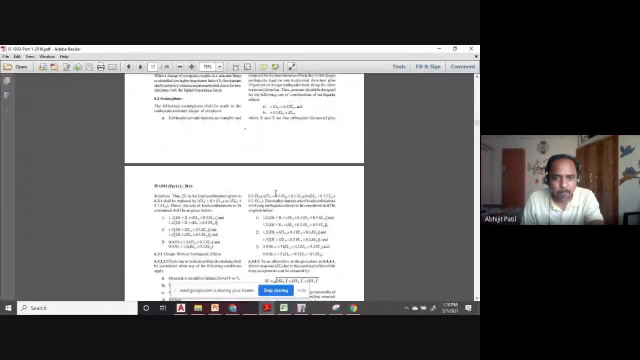 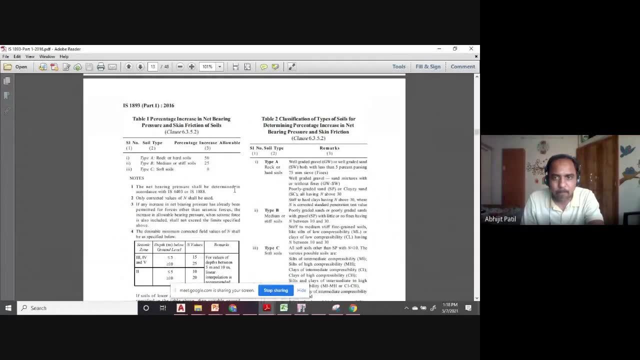 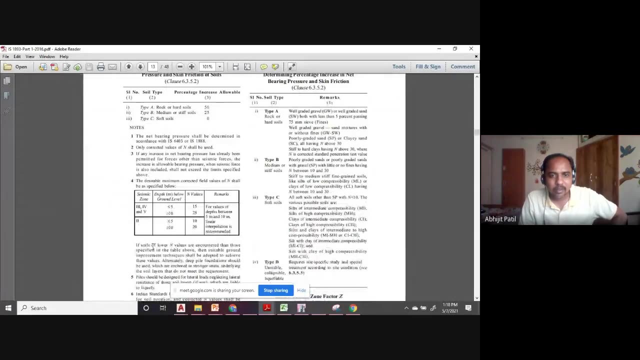 So the temperature of the soil is determined by the temperature of the soil. So if you think of the sea level, that's what we are discussing. yes, so even in description is given here. here you will see. okay, 33 is sorry that. was old value. so here you can see the percentage of increase in net soil bearing pressure, or hard soil it is 50, medium soil it is 25 and for soft soil it is not allowed. previously it was averagely 33% for all soils and here is. 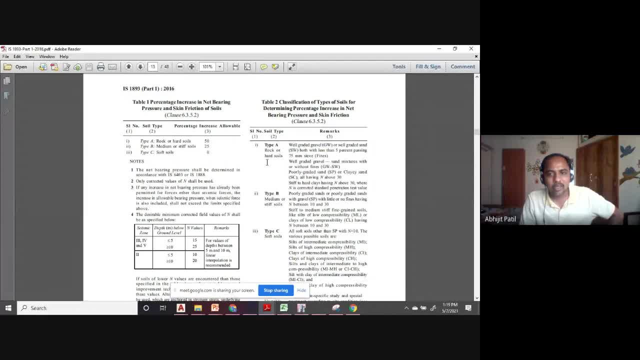 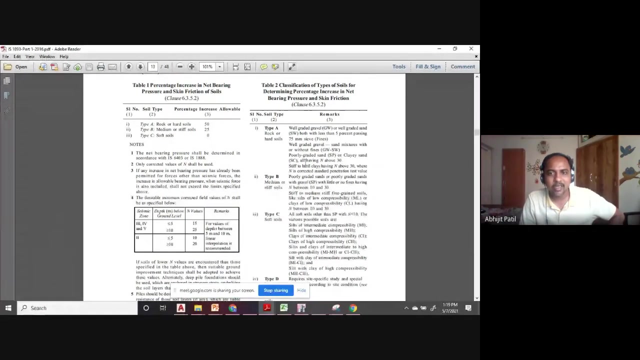 that type of soil, so type a rock or hard soils, so well graded gravel or well graded sand, both with less than 5% passing 75 MC. okay then, well graded gravel and sand mixtures, with or without fines. yes, yes, so descriptive this, and all having n value about 30. so you know, in previous code it was only 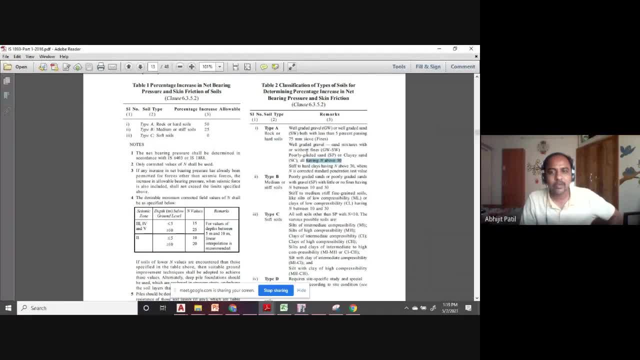 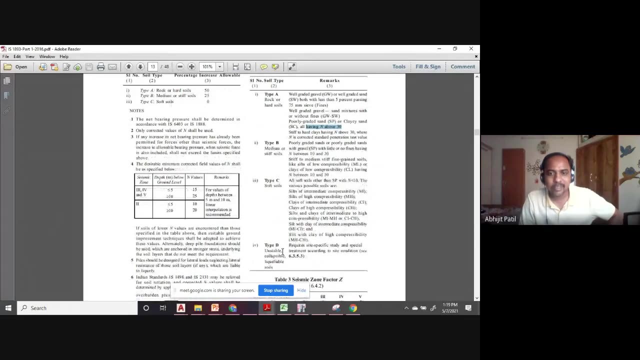 based on n value. but now they have given a very good descriptive, distinct soil description: 10 to 30 and less than 30, okay, so this is. and again they have type D collapsible soil. so again that becomes very specific. this requires site-specific study, so we cannot use our response spectrum, we have to use the. 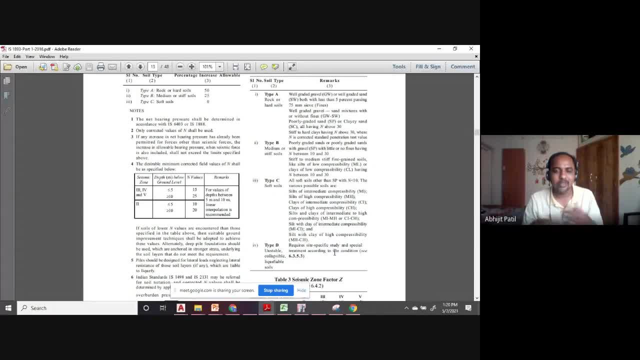 site-specific spectrum. okay, so this is again a part of systemology where, instead of using general graphs, you study that particular area and you generate your own response spectrum related to that particular type of soil in that particular area, and then you can use that. okay, so this is table 2. 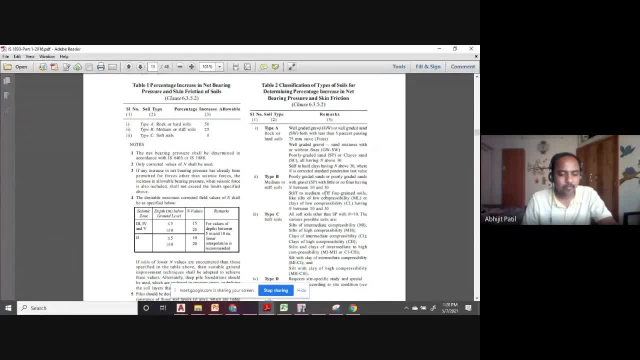 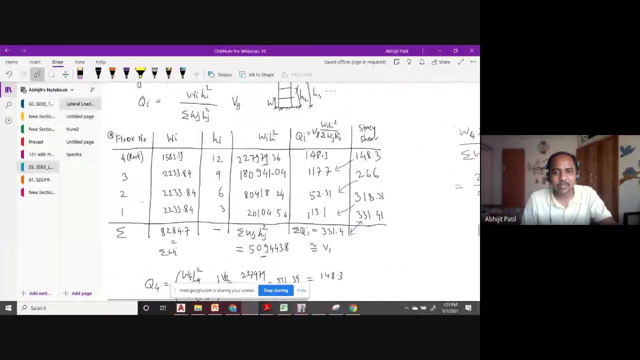 cell so you can, Meinard, then start by finding all the critters of those passes f or any other queries. students, if you can us what I will do, I will share this as to numerical which I have sought, So if in case somebody has missed something. so, step by step, they can please bear with my handwriting. 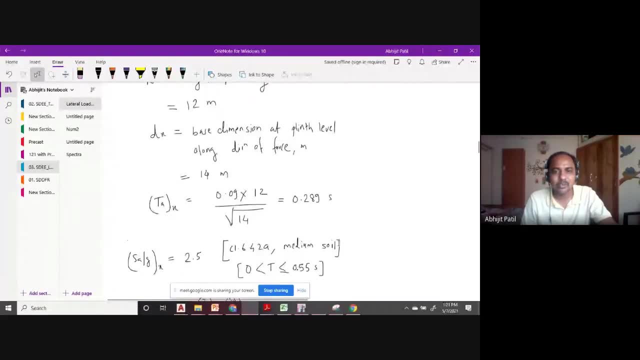 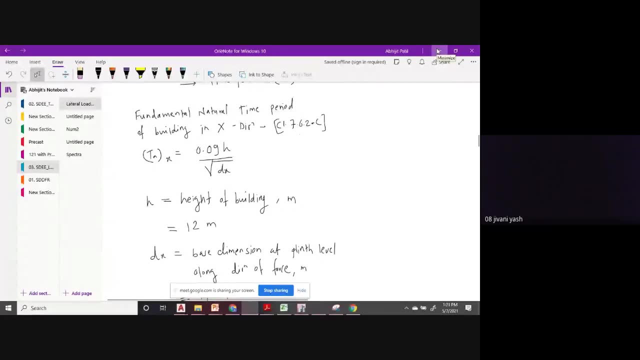 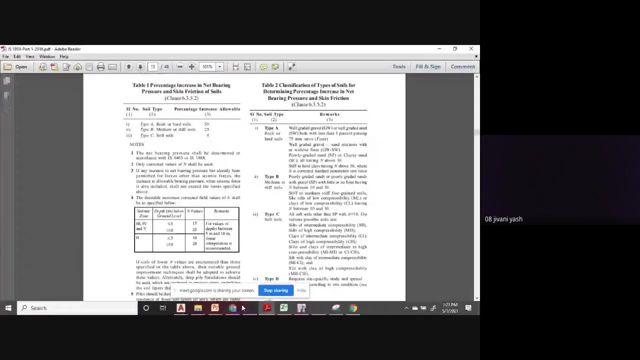 because i have been using this writing pad so it's not, but it's readable. you can refer that, sir. you have taken your hs 12 meters, sir, yes, yes, so it will be nine. no, sir, sir, you, you said that the h is from plinth to top. 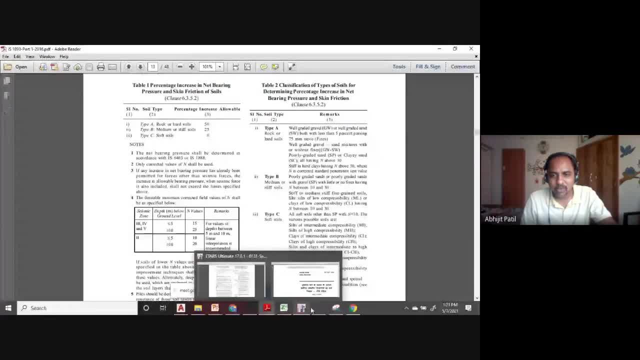 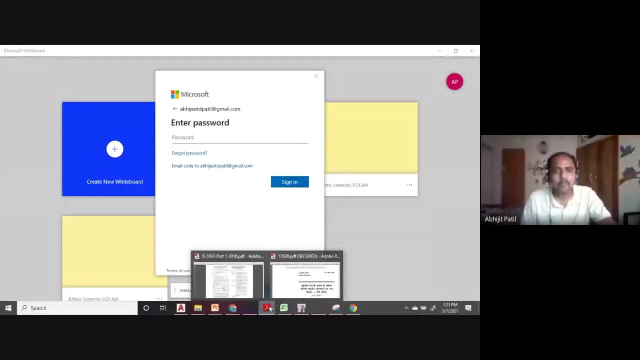 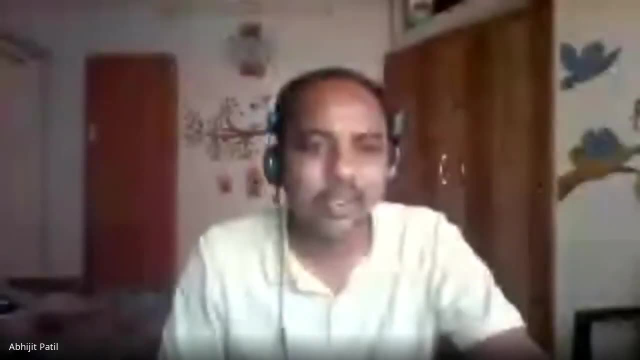 yes, so whatever section i have shown is actually above plinth. okay, just let me go back to that. okay, so this is not actually a foundation level, this is plinth level. so if you see four storage, so this is first story, slab, second story, third story and this is actually. 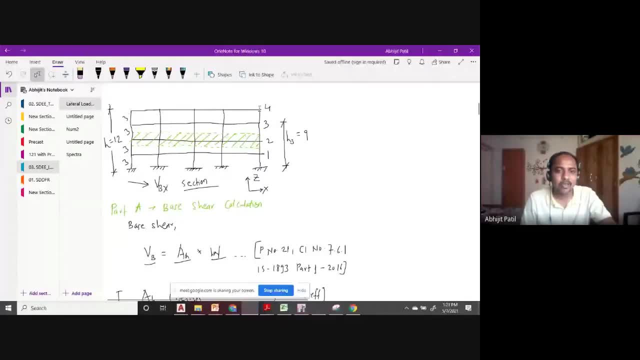 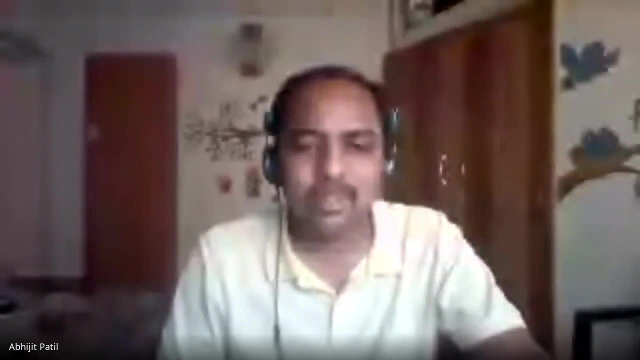 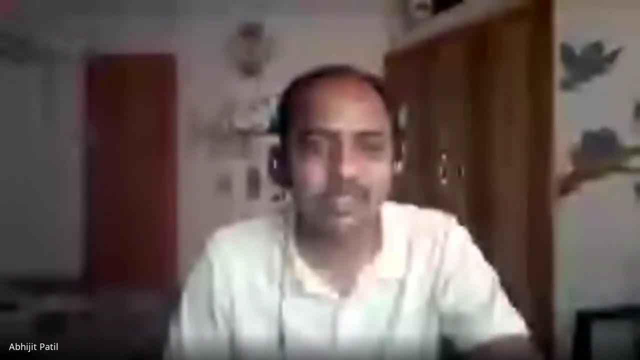 your ground level. okay, and at ground level we don't consider the earthquake form, because this will move with the ground. this is usual confusion. i i can, because generally we see, uh, we draw a cross section from foundation, but here, in this case, this is actually your ground level. first story, second story. 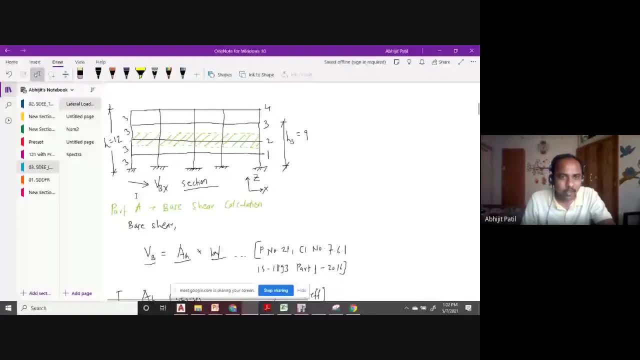 uh, yeah, i will mark that. so this is your ground level and below this you will have your foundations. so this is your ground level, okay, and above this first story, second, third, so fourth is your roof. it's a four story building means ground plus three actually, so this will be five story building. no, no ground plus three. 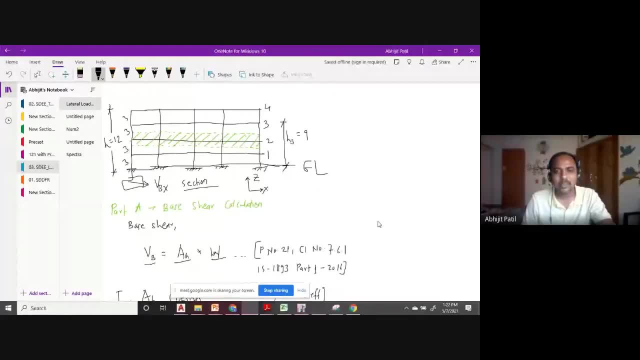 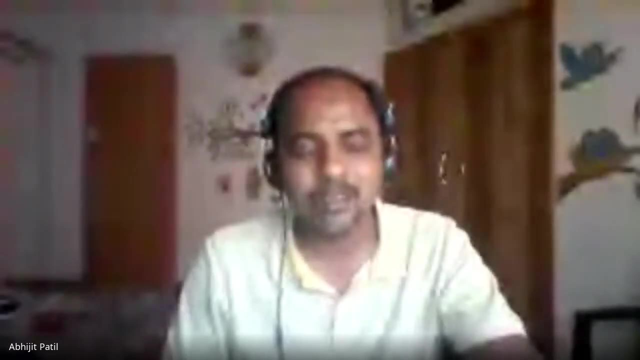 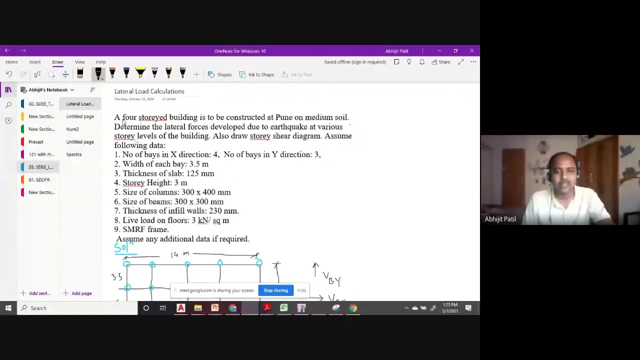 okay, please not consider. yeah, so usually actually this is from our university question paper, so usually some mistakes are there in data. but generally if i take questions i directly say it is because of course there can be a confusion. your point is also right, but i usually give ground plus three or down plus four, like that, so that it is very clear. 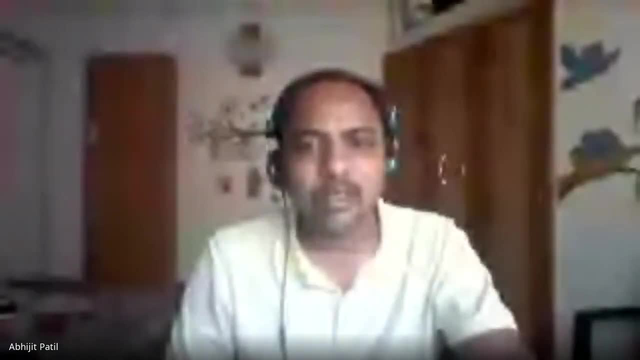 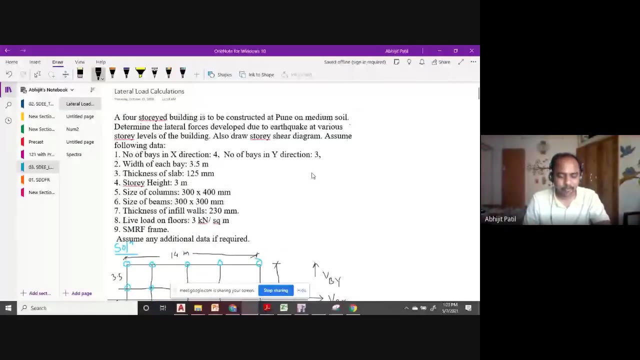 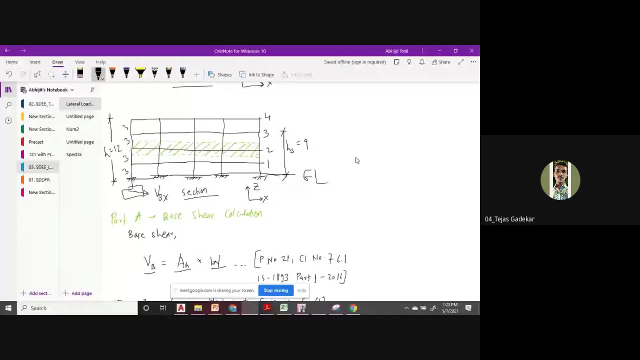 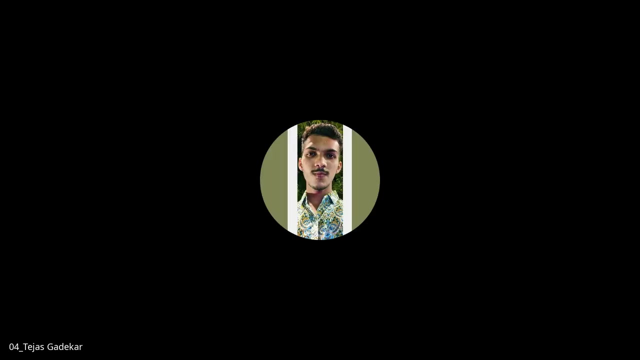 okay, but our students, if it is four storage or five storage, it is generally four- means g plus three, like that. yeah, so then what we have to take here nine meter or 12 meter? no, it's 12 meter, is correct, 12 meter. okay for the four story. uh, yes, yes, yes, yes. uh, jaydeep sir, if you can share their question paper. 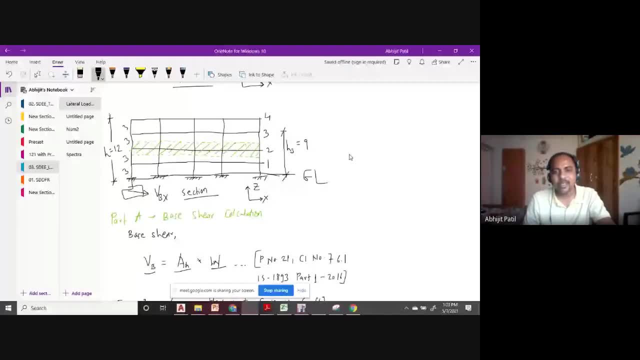 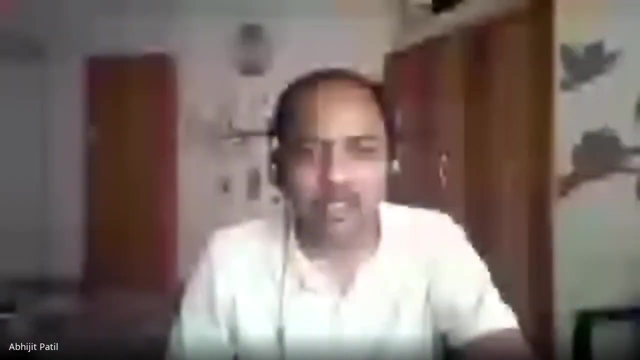 or any sample, one or two, then i can just read out that later on i will just convey the message you can convey to them. yes sir, yes sir, in calculation of story, uh, here, or a lateral shear, in each sir, we consider: h, i, yeah, right, right, yeah, same thing, same thing. i will be. 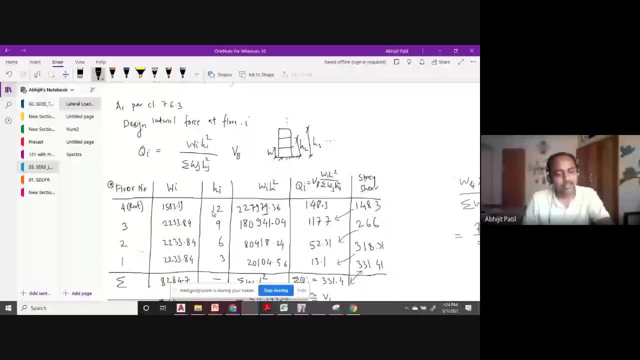 on floor ceiling. HI will be downfloor level, sir Yes, plant level. so this one is at the planet level, first floor, so it is three meter above ground. so this, this is your first story, right, sir? yes, or other basement may to level a three level car parking here. 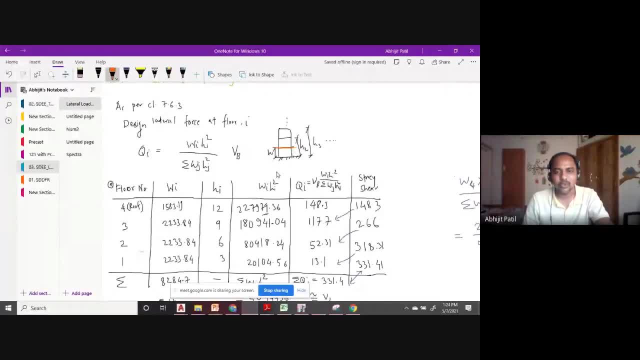 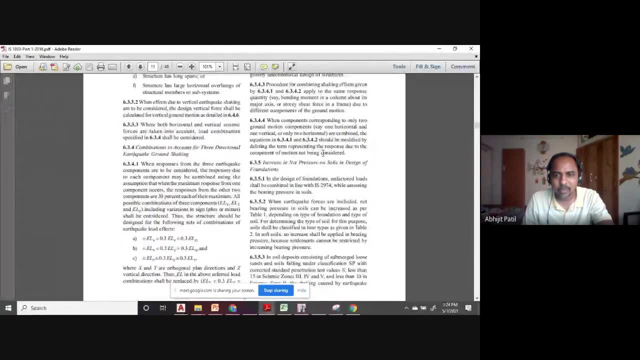 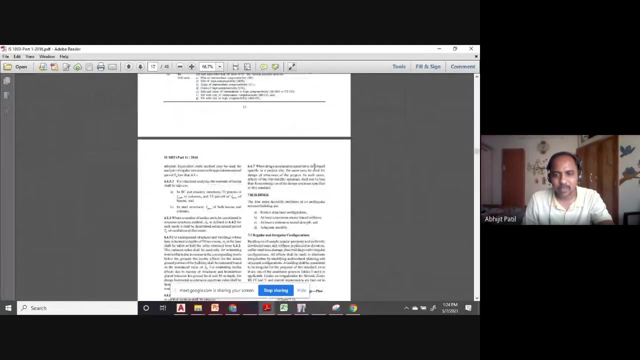 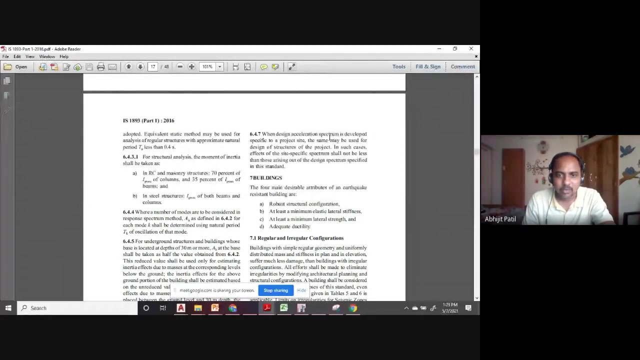 yes, good question. good question. here in code it is mentioned. I will just open that clause. so this was again not there in previous codes. now it is mentioned because usually in Mumbai, where high-rise buildings are there, the basement is common and again you have separate buildings. or I will just answer? 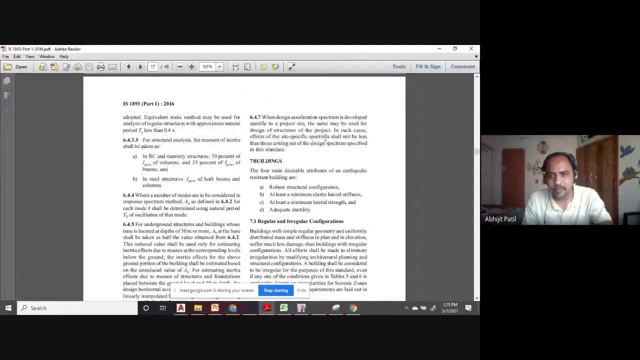 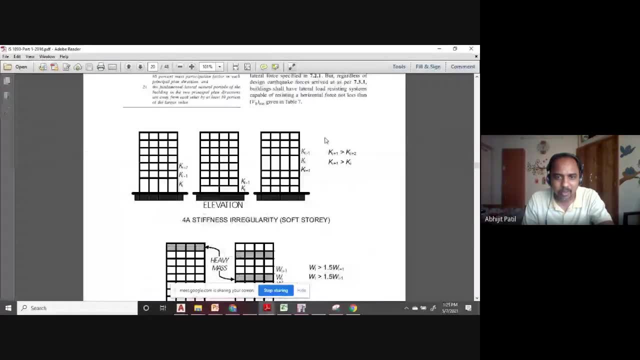 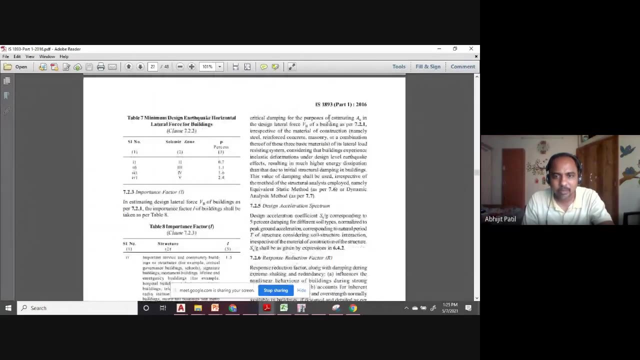 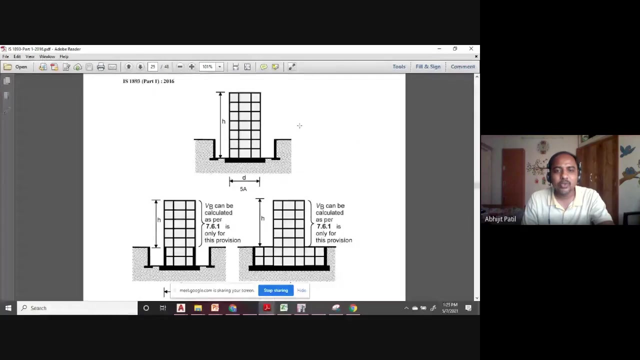 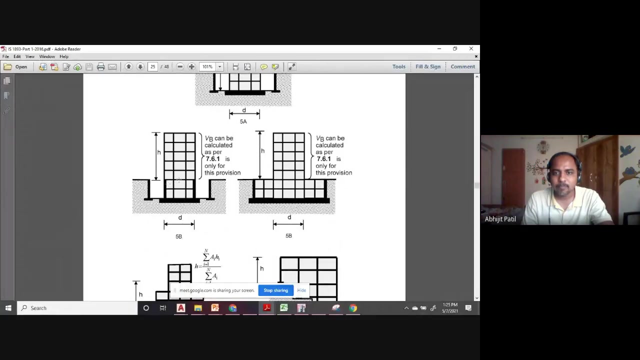 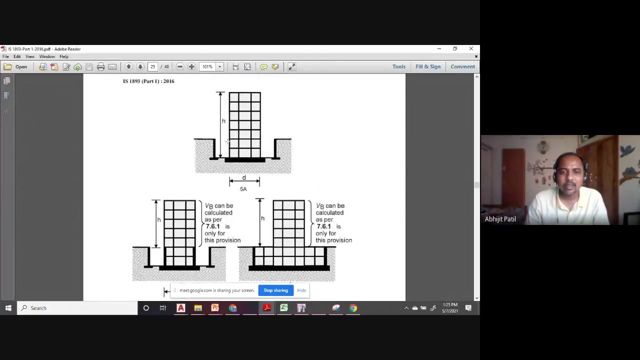 that, basically, if your basement is- I think they have included figure also, so that will be better to explain. I think nine point something. yes, this is the figure. so basically you see there are two types of basements. okay, one case: your basement is separate. okay, so you have a retaining wall. 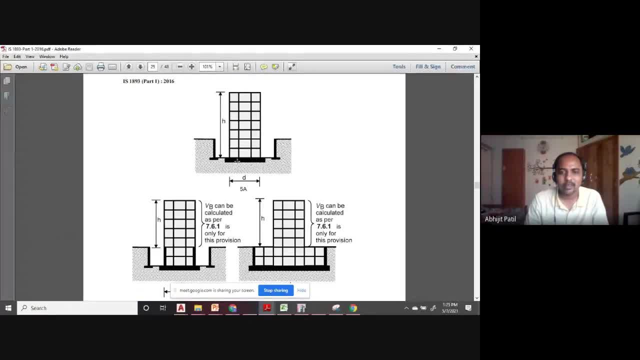 here, you have retaining one here and you have a building here and this retaining wall and this building- they are not at all interconnected. okay, so in this case, instead of the ground level, the top of order, the bottom most story, so you have to measure all your Heights from this bottom most stories, okay, and 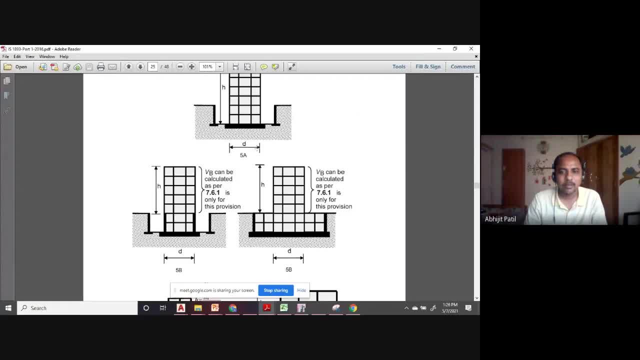 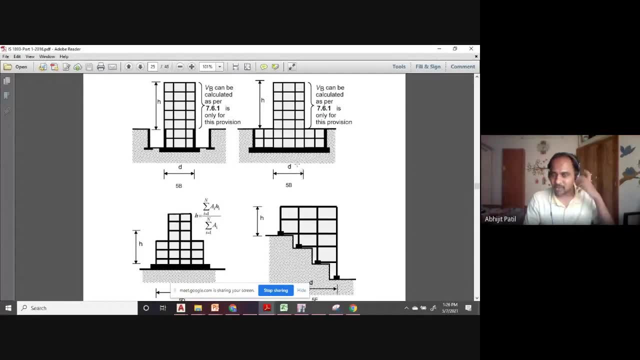 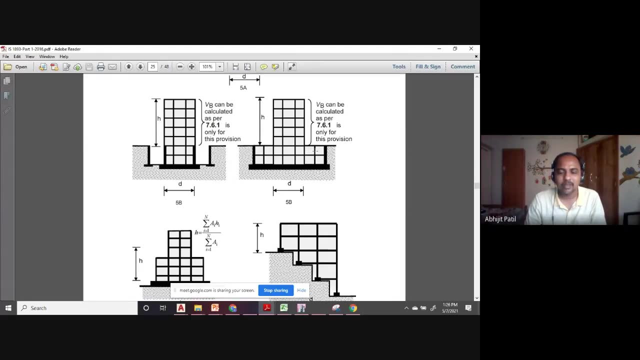 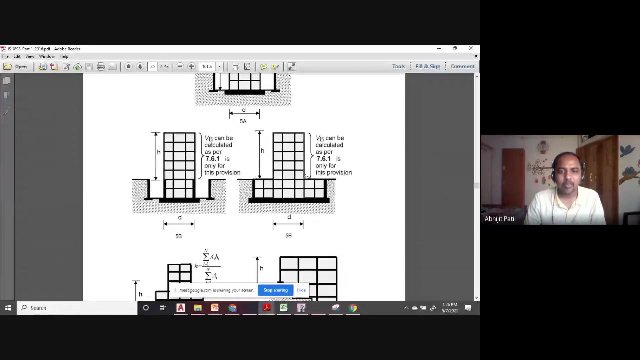 the width of the building is. this, then, is second uh criteria, this, this one, where all your buildings and basements, so they all, are connected like this. okay, so there is no separate structure here, no separate structure, so you have building here and then building dimension expands here. so in this case, you consider the height of the 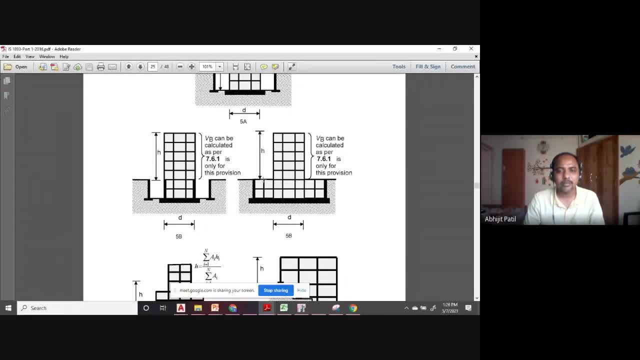 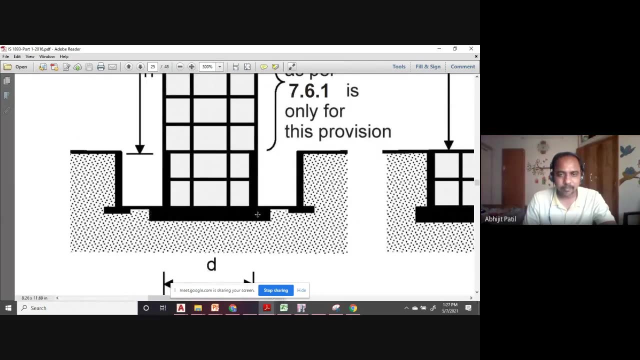 building from this ground level. okay, and you have. what is the difference in this and this? here you have a written wall. if you see, i will just zoom. okay, so you have a retaining wall here, okay, so even though the structure is separated, you still have a retaining wall here. 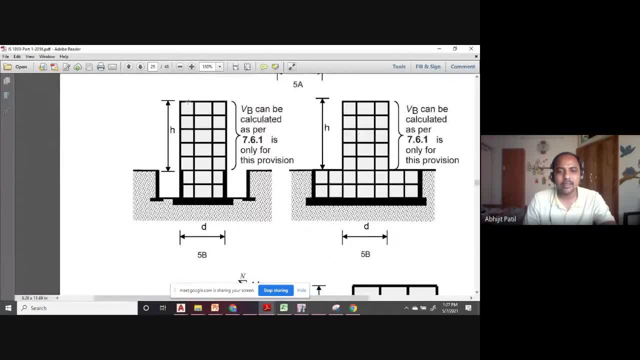 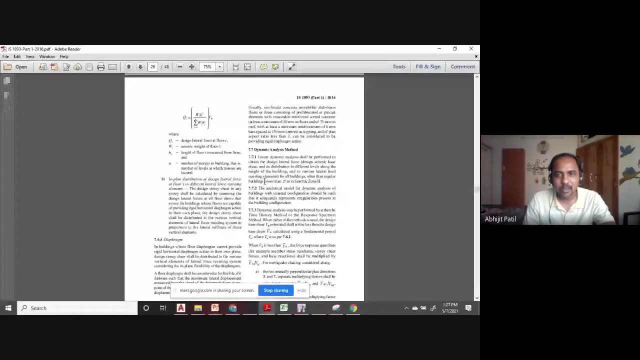 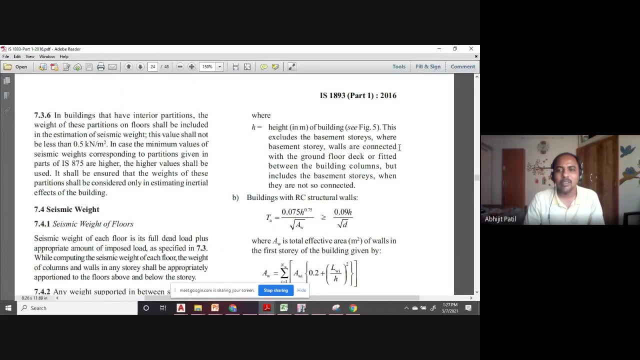 retaining wall here. so in this 5b case you consider the height of the building again from the ground level. okay, so if you see the description plus 7.6.1, i can previous to this. yes, see figure five. so this excludes the basement stories where basement story walls. 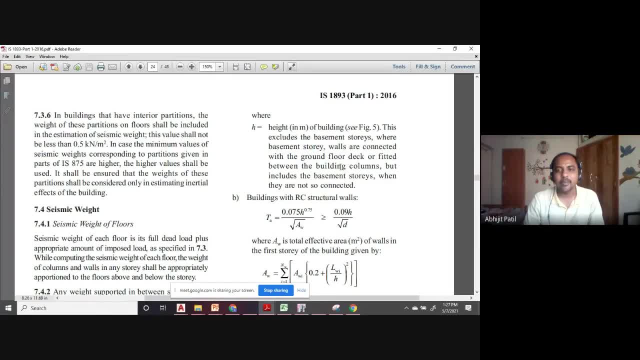 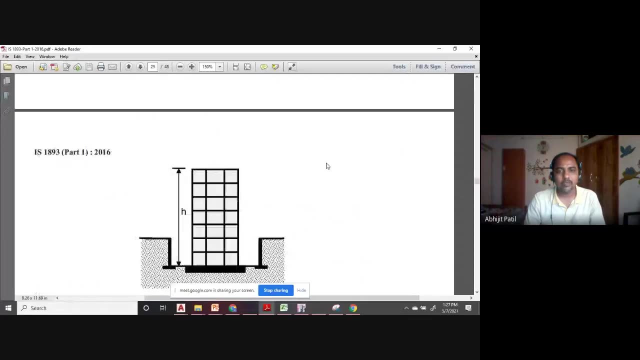 are connected with the ground floor deck or fitted between the building columns. okay, so, this was the case 5b, the below two figures, but includes the basement stories when they are not connect and they are not so connected. okay, so if you have separate basement structure, it is not at all connected with your main building. 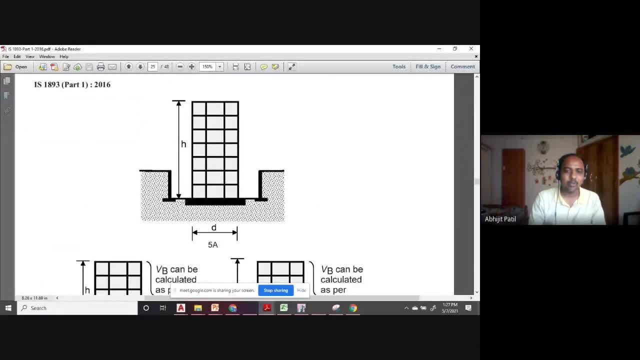 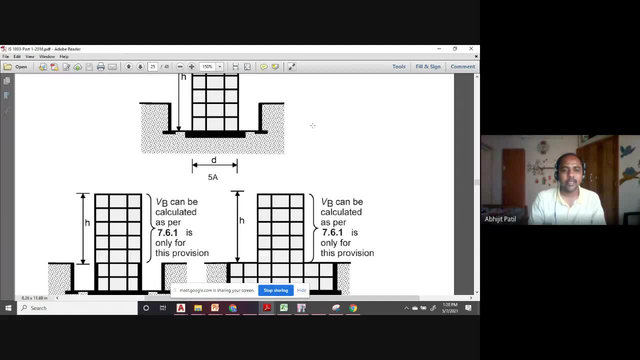 then consider this as ground level and from this bottom most story you start measuring your height. so it is applicable for h as well as h- i, but if they are connected like this or like this, your height of the building will start from this story, and obviously no. 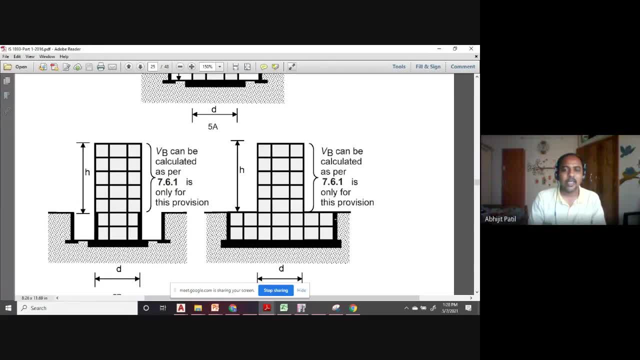 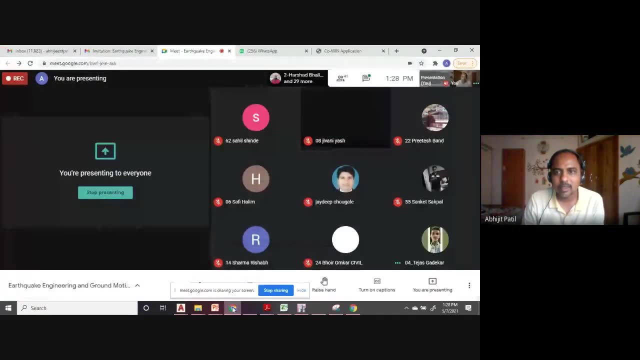 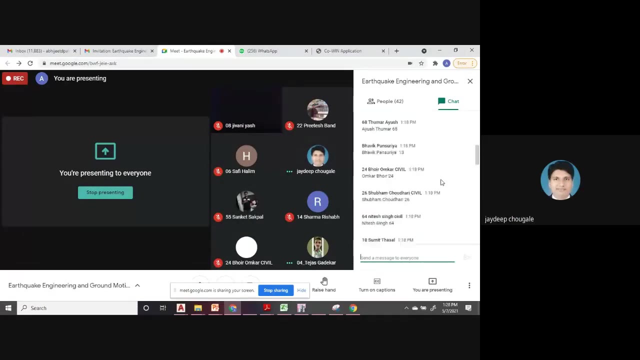 earthquake force will be uh applied on these basements, because this is this- will move along with the ground. okay, yes, any other questions? no, sir, okay, so good, i hope that. uh, of course, this is very uh. this was very extensive in a short time period. i tried to cover most of the points. uh, one part remaining is is 13920, so that uh, ductility. 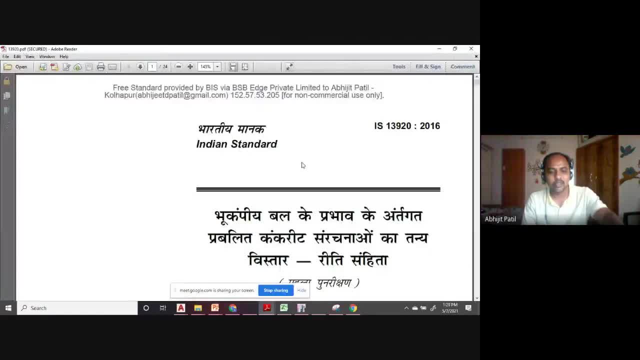 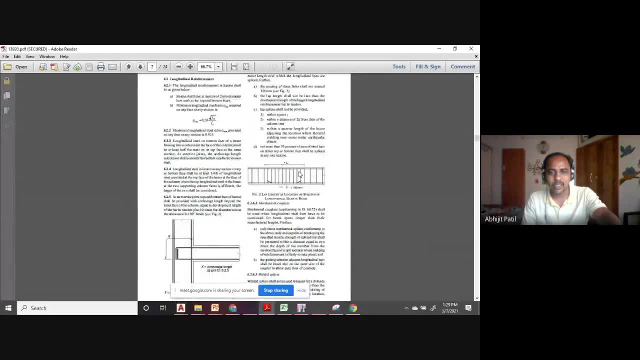 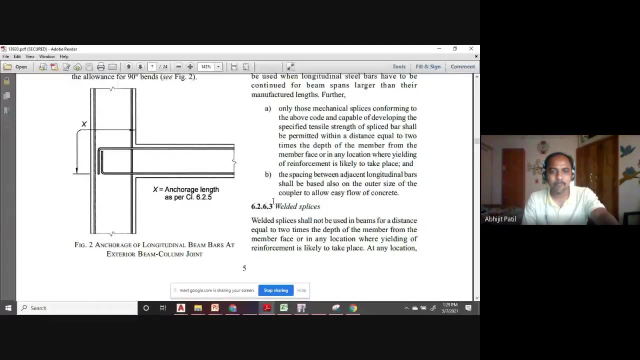 detailing is actually nothing but uh code. so this is the code and few figures are there which are self-explanatory. you can go through that. so just like: how should be at lap length? what should be ld? what should be the spacing? it should not be more than 150 mm. the beam column joints, this should be like this: the l's. 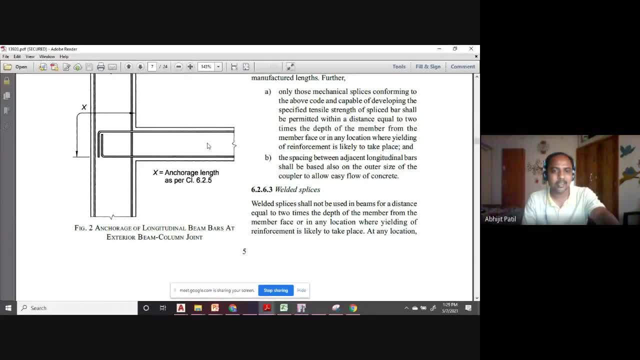 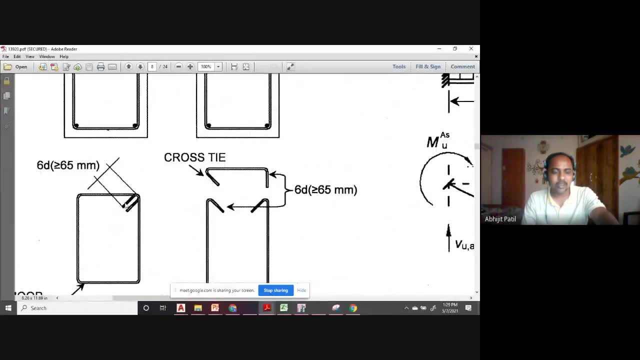 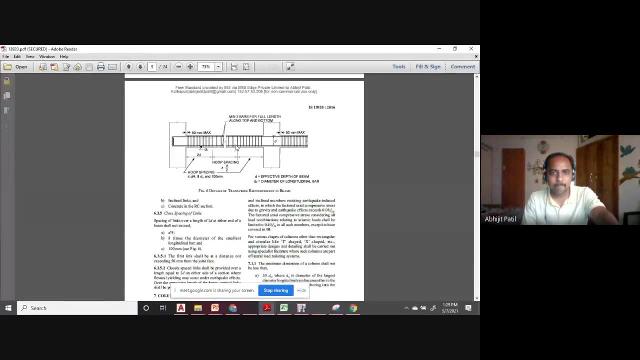 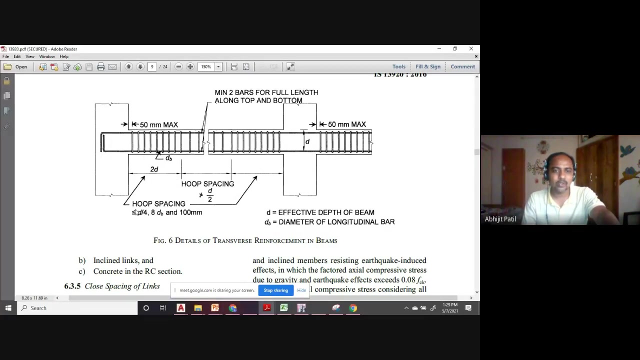 of top bar as well as bottom bar. the anchorages should be provided like this: then, uh, this cross tie or this should be: uh, this is a correction. now it is 75 mm or 10d typical beam cross section, so 2d distance. the hoop spacing should be different and in between it should not be more than d by 2.. 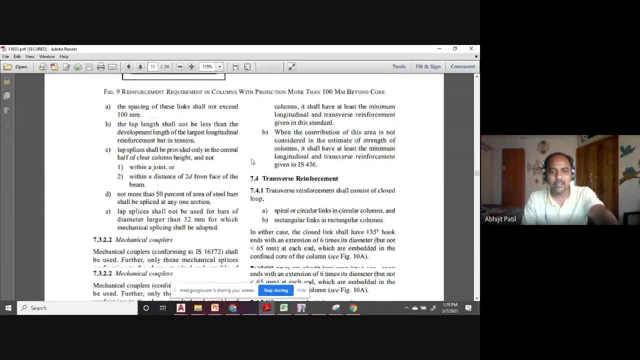 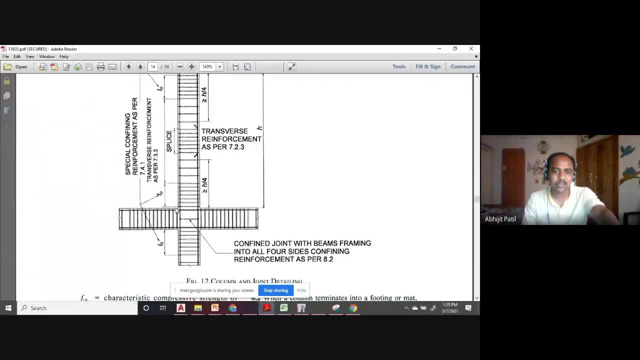 same thing. these are very important guidelines. these are to be followed. so, with the help of figures, you can just go through that. browse through those figures. yes, this is very important section. so, near the column beam junction, this is a elevational section of column, so this is. 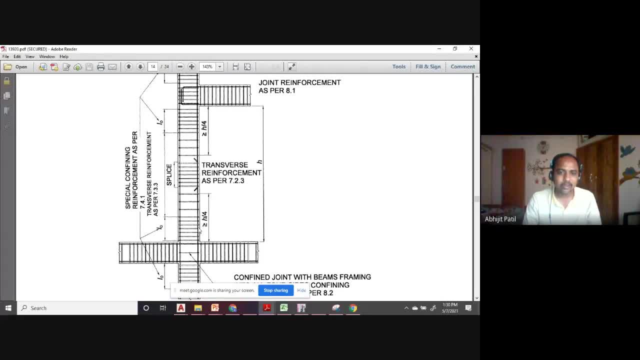 one floor level. this is another floor level, so here the whole spacing is very close inside. also you have to provide column links following the same spacing here, then wherever there is splicing. so remember this- the splicing is not at the floor level but somewhere in middle, the middle third of the column H, by 4 H, by 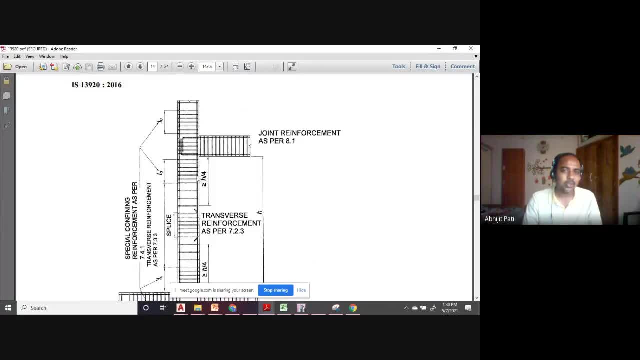 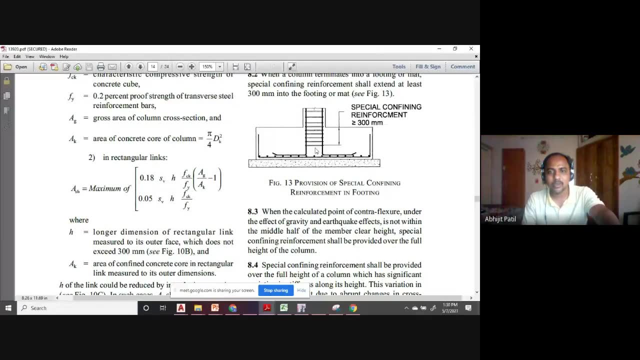 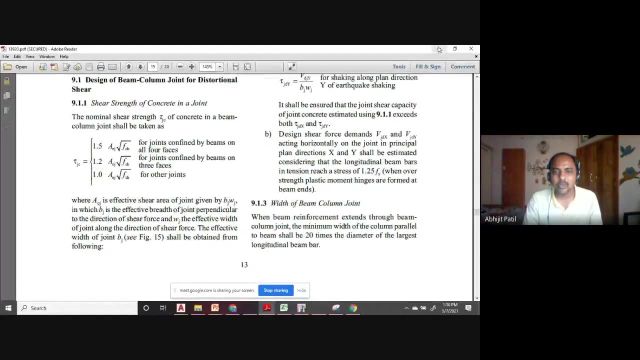 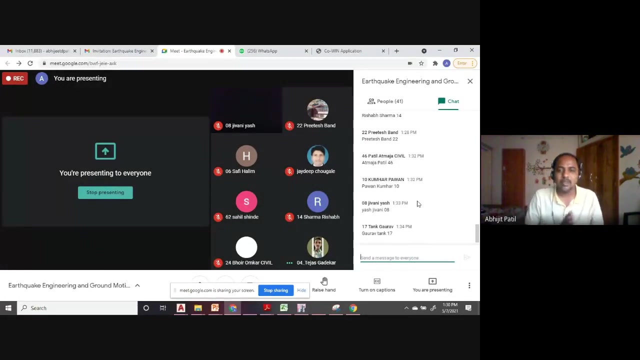 four, except that you can provide splicing. so these are a few important guidelines you just refer that will be even in the footing, these stirrups, which is usually not done. so this should be continued like this. okay, so these guidelines you can just refer and we'll be able to understand, okay. 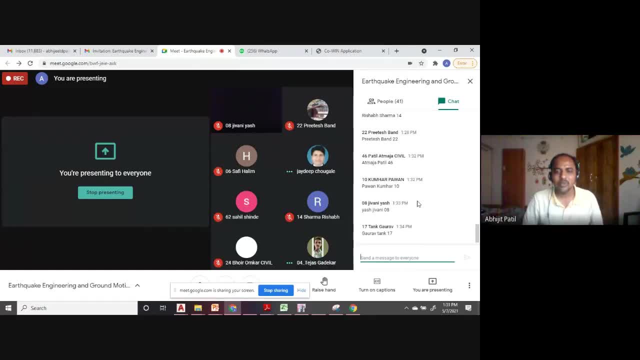 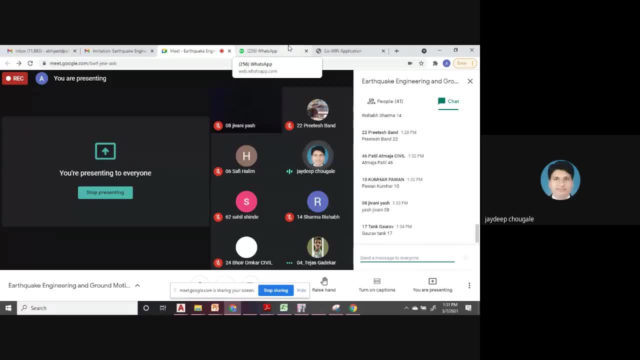 Padil sir for your sharing your. Padil sir, for your sharing your knowledge and spend your valuable time knowledge and spend your valuable time knowledge and spend your valuable time with our students and motivate them to with our students and motivate them to with our students and motivate them to think on the Arctic region structure. so 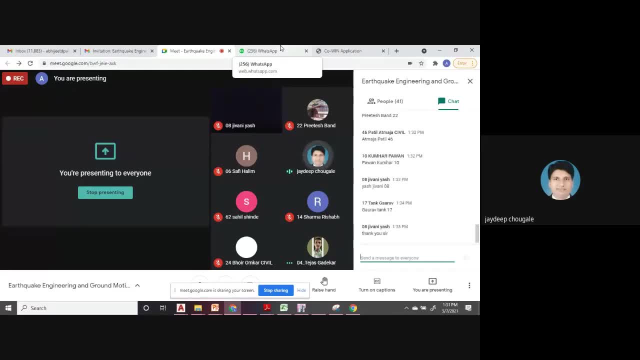 think on the Arctic region structure. so think on the Arctic region structure. so thank you once again, British, and you thank you once again British, and you thank you once again British. and you would have thanked, yes, sir, yes, sir would have thanked, yes, sir, yes, sir would have thanked. yes sir, yes sir. good afternoon, sir. I would like to 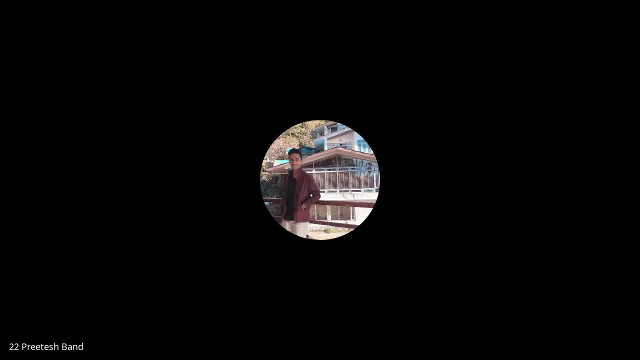 good afternoon, sir. I would like to good afternoon, sir. I would like to thank you for the thank you for the thank you for the behalf of all the be civil students and the behalf of all the be civil students, and the behalf of all the be civil students and the civil department. the session was. 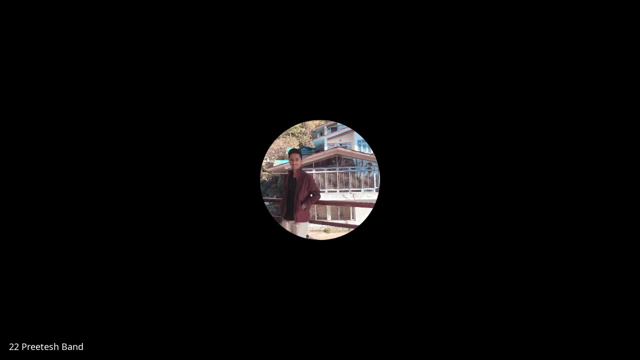 civil department. the session was civil department. the session was very informative and also interactive. we very informative and also interactive. we very informative and also interactive. we really appreciate the fact that you really appreciate, the fact that you really appreciate the fact that you started with the very basic of 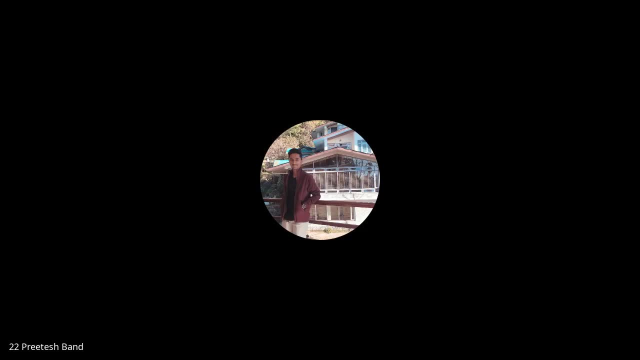 started with the very basic of, started with the very basic of engineering geology, and then proceeded engineering geology, and then proceeded engineering geology, and then proceeded with the actual earthquake engineering, with the actual earthquake engineering, with the actual earthquake engineering design procedure which helped us in. 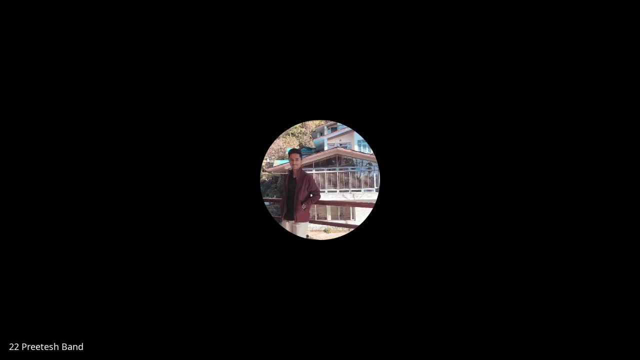 design procedure which helped us in design procedure, which helped us in understanding the topic quite easily. so understanding the topic quite easily. so understanding the topic quite easily. so we are quite grateful that you have. we are quite grateful that you have. we are quite grateful that you have spent some time from your busy show you. 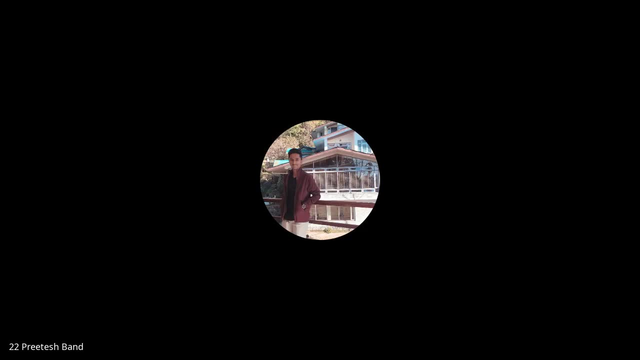 spent some time from your busy show. you spent some time from your busy show you to share your vast knowledge and to share your vast knowledge and to share your vast knowledge and expertise in the field of earthquake expertise, in the field of earthquake expertise, in the field of earthquake engineering. finally, I would also like to 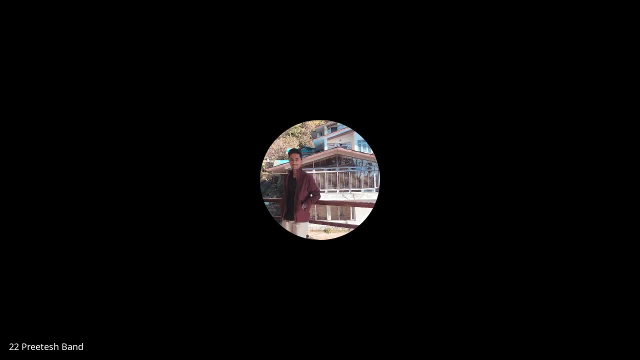 engineering. finally, I would also like to engineering. finally, I would also like to thank a professor, Jerry Toggle sir, for thank a professor, Jerry Toggle sir, for thank a professor, Jerry Toggle sir, for organizing such an informative session, organizing such an informative session, organizing such an informative session. thank you. 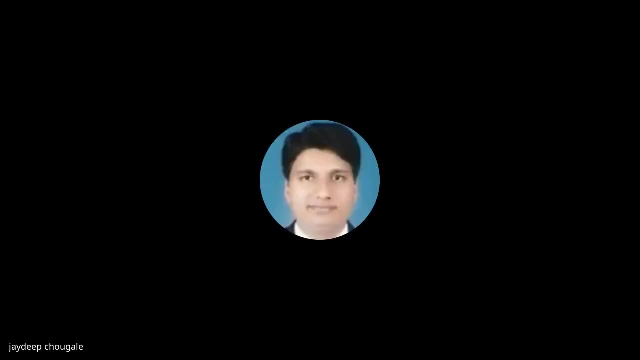 thank you, thank you okay. thank you sir. thank you, thank okay. thank you sir. thank you, thank okay. thank you, sir, thank you, thank you. good and much yeah, student you you good and much yeah student you you good and much yeah student. you mentioned your roll number in chat box.